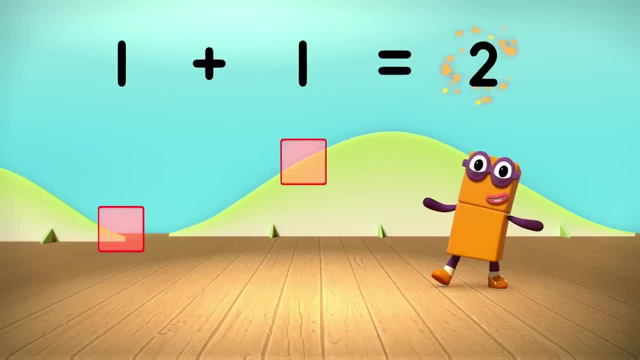 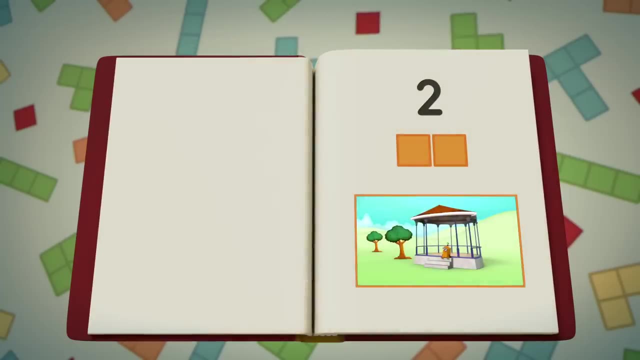 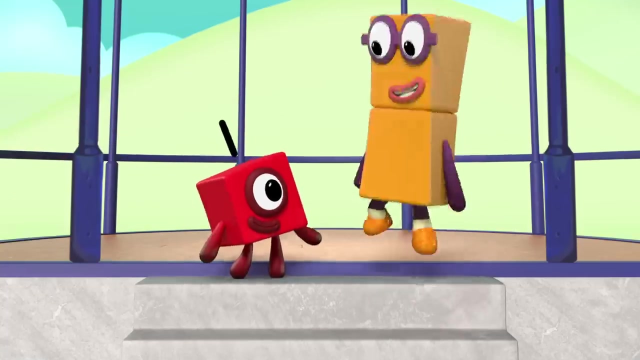 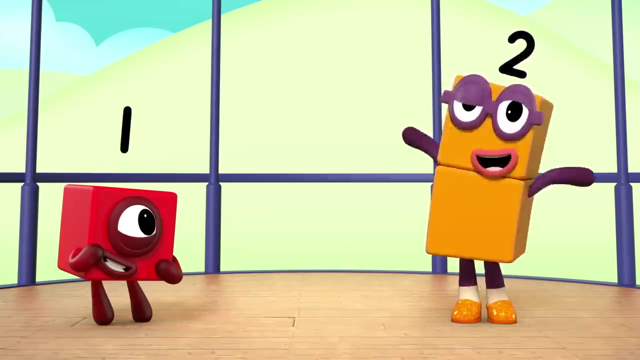 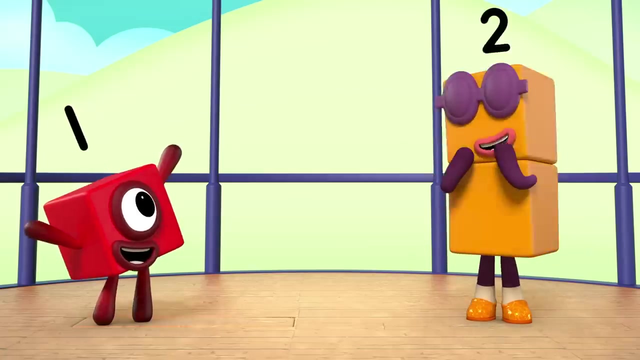 Plus one Equals two. I am two. How do you do Chapter Two? Me and You, Me and my best friend. I am two. I am one. two, Two blocks, And this means two, Two. I love things there are two of. 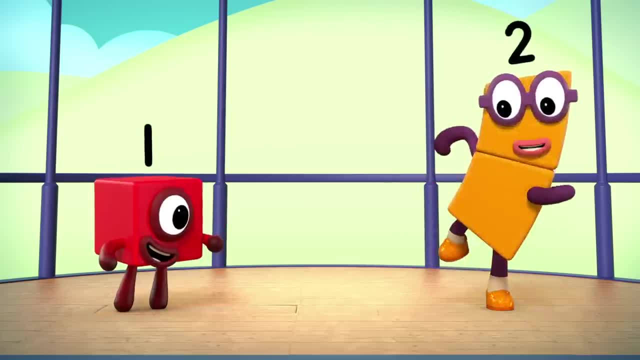 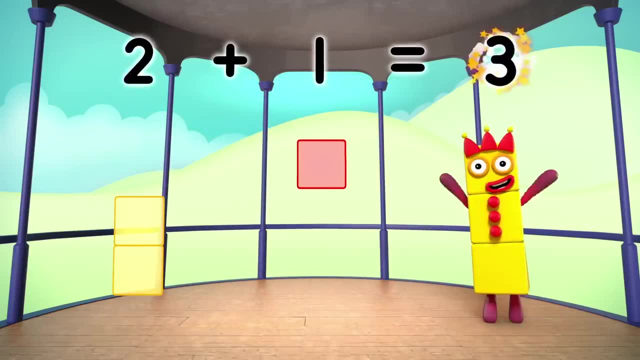 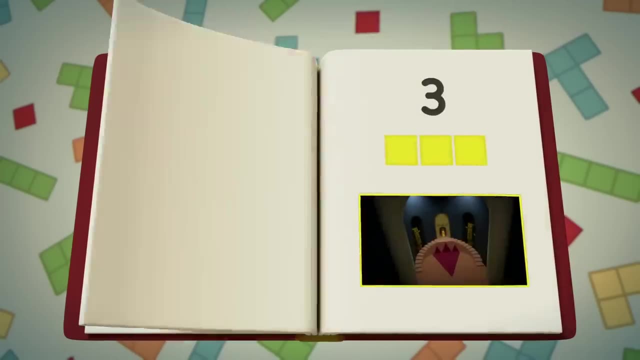 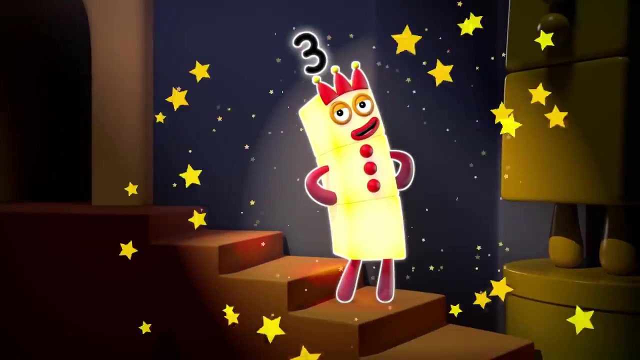 One, two, Two. dancing shoes: One, two, One, two. Oops, Two Plus one Equals three. I am three. Look at me. Chapter Three: Me, Me, Me. I am three. I am one. 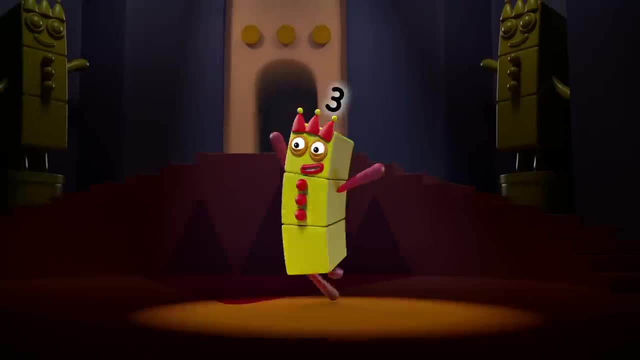 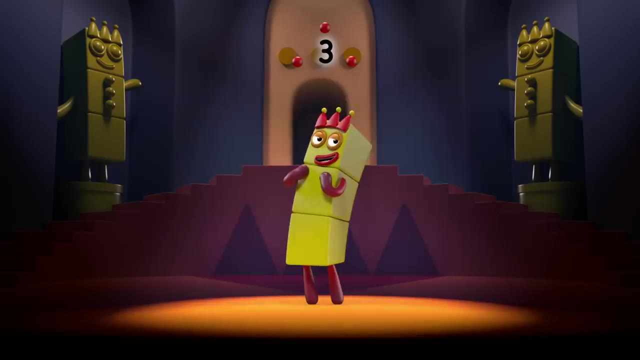 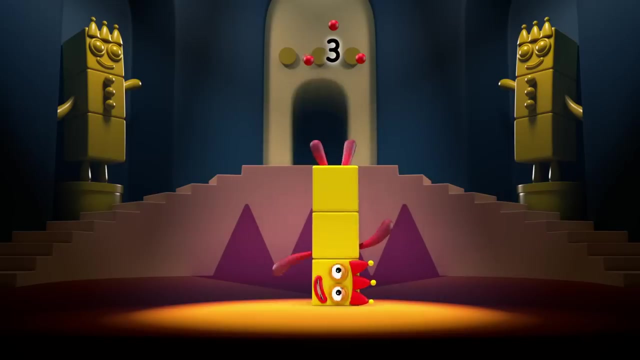 One, two, three, Three blocks. I could juggle one, two, three, Three balls, And this means me Three, Three, Three, Three, Three, Three, One, two, three. I'm so amazing Who could possibly follow me. 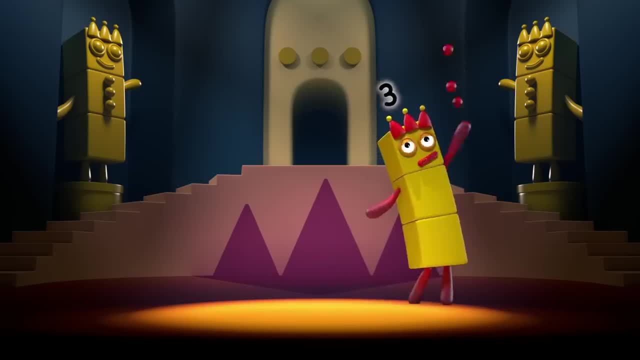 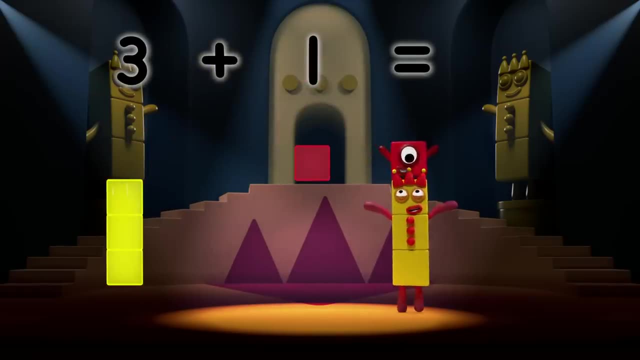 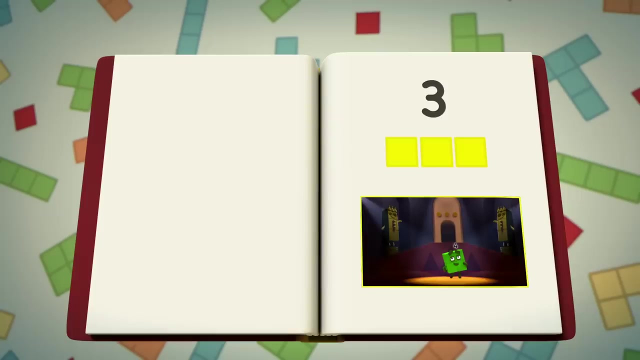 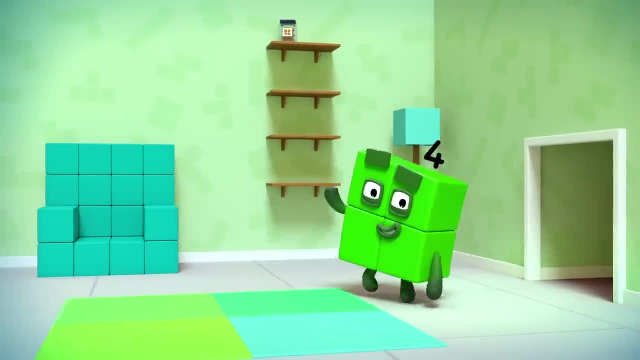 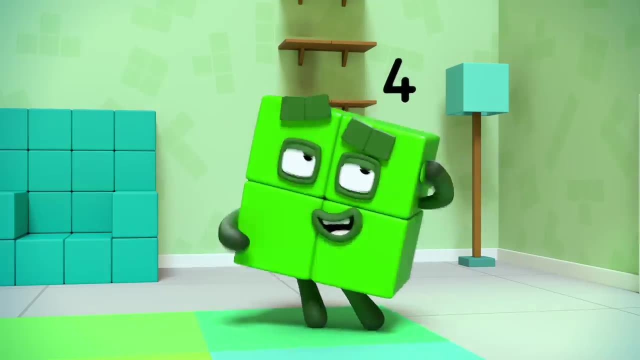 One, two, three, four, Three, Three, Three, Three, Three, Three, Four. I'm four. I am four. Have we met before Chapter Four, Thor's House? Hello, I am one, two, three, four. 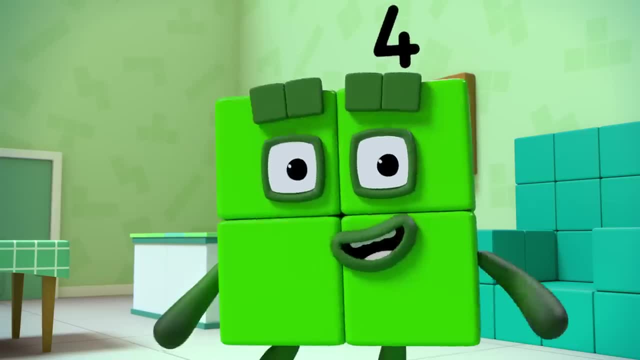 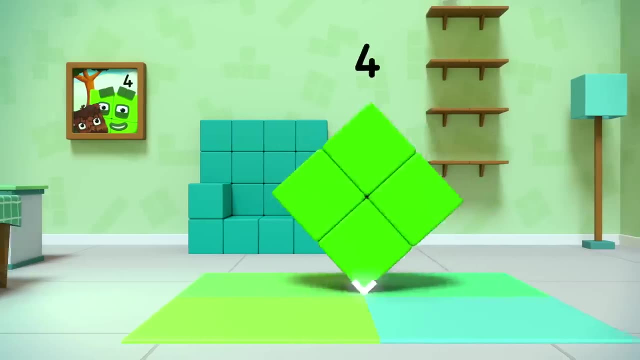 Four blocks, And this little fellow means four. Can you guess what my favourite shape is? That's right, A square With one, two, three, four, Four sides And one, two, three, four, Four corners. Whoops, Oh no. 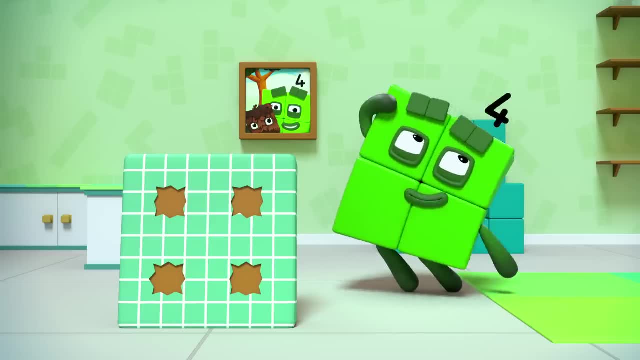 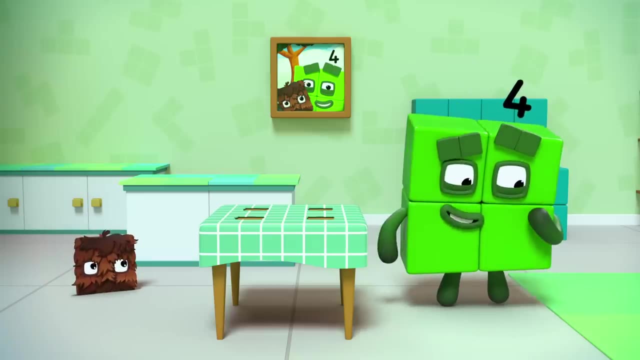 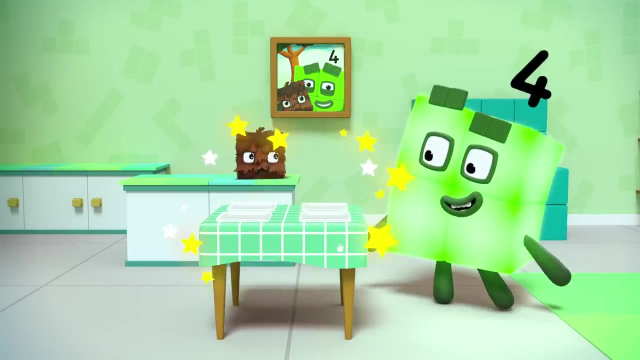 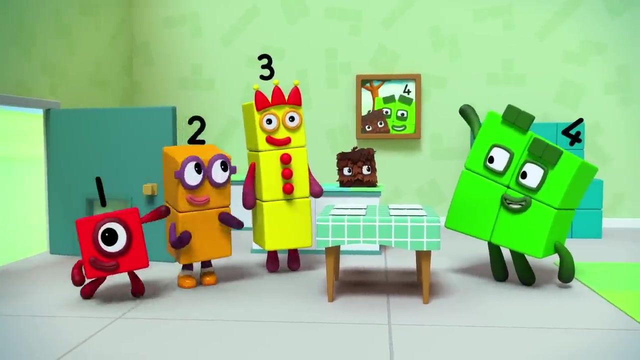 Someone's nibbled four holes in my tablecloth Squarey. You cheeky little square. How can we fix this? One, two, three, four, Four plates. Hello, everyone Who wants a square cookie I can't reach. 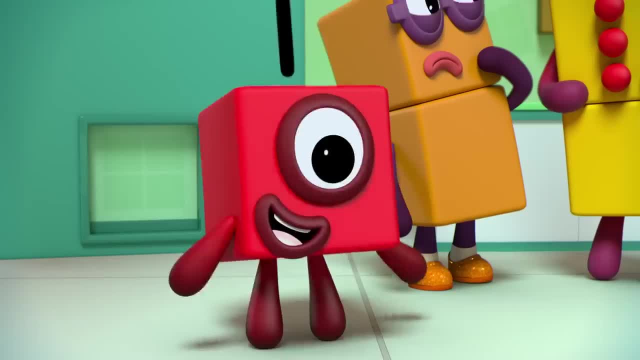 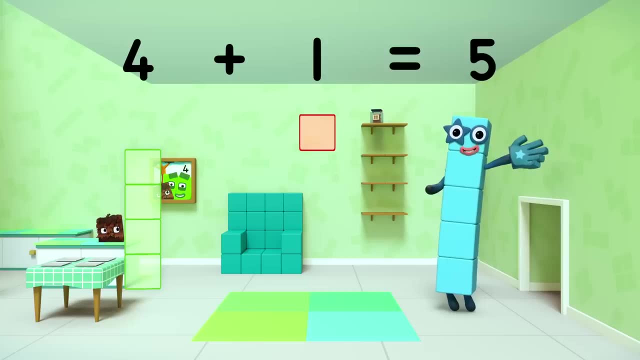 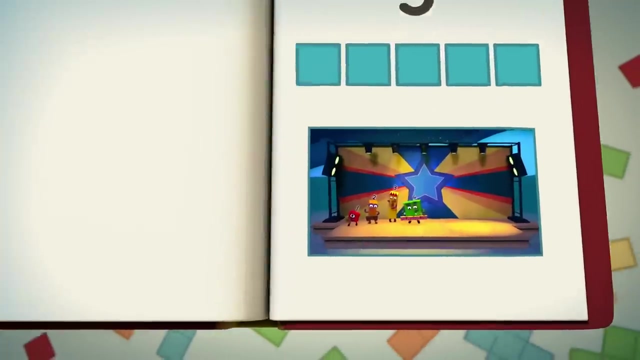 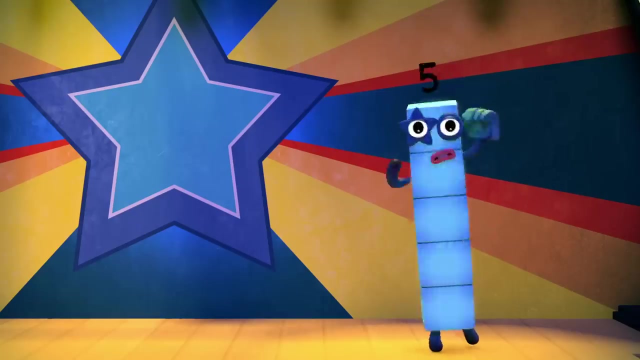 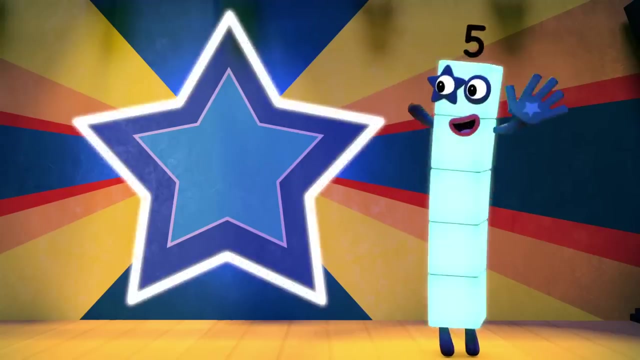 Aha, Four Plus one Equals Five. I am five, I feel alive. Chapter Five: The Star Turn. I am one. two, three, four, five, Five blocks, Five, Five. I love stars. They have five points. 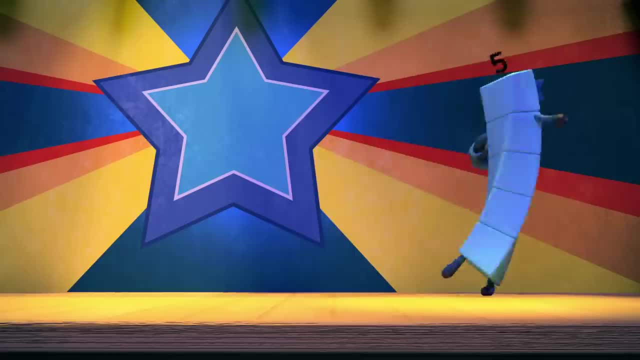 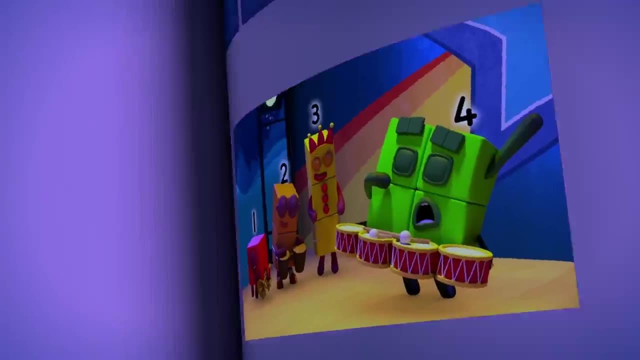 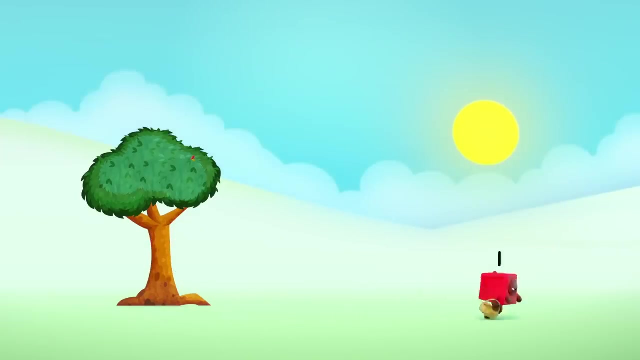 Making me a rock star. Thank you And good night Me Bloxzilla. Me like big things. Which is bigger? Tree is bigger than flower. Me like tree. Nice to meet you, tree, Will you play with me? 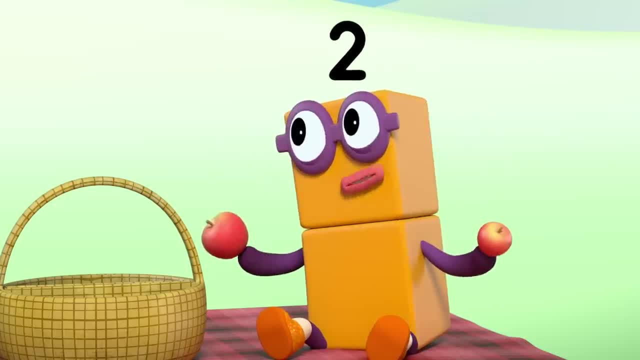 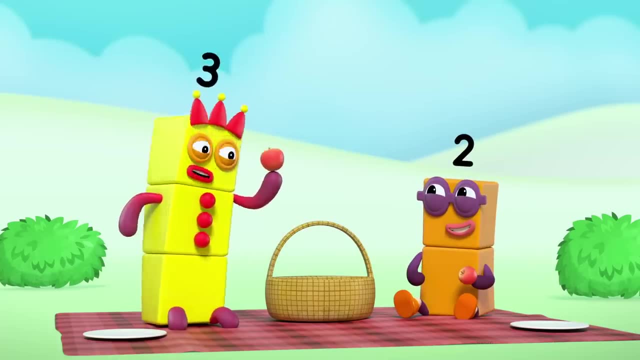 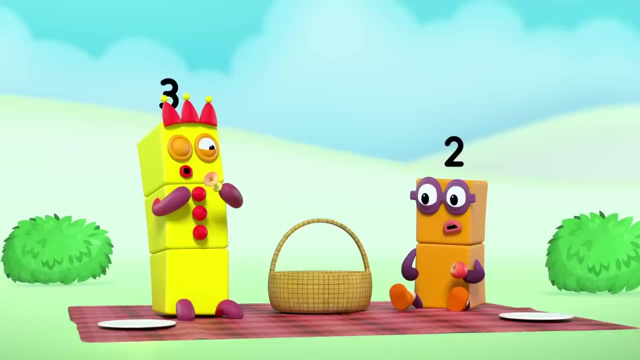 This apple is bigger than this one And you're bigger than me, So you have it tree. Thank you too. I like apples. I like to munch them And crunch them And gobble them up. Me like lots ofіти. 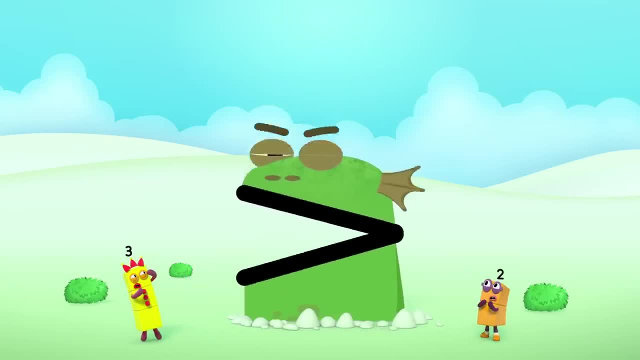 My name's Bloxzilla, So do I Please? Ah, Ah, Ah, Machitos, easiest move God, not just goodbye. I'm so happy That was sudden. Ow, My legs are catching on. It hurts, Oh. 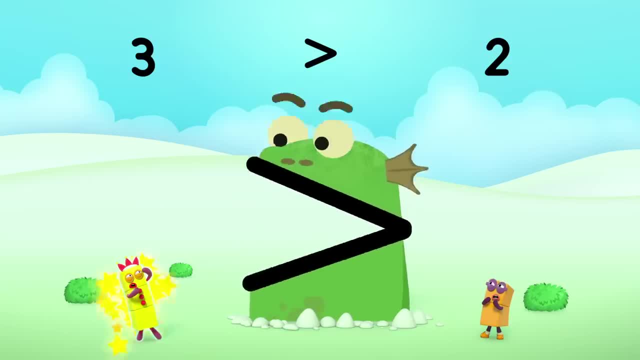 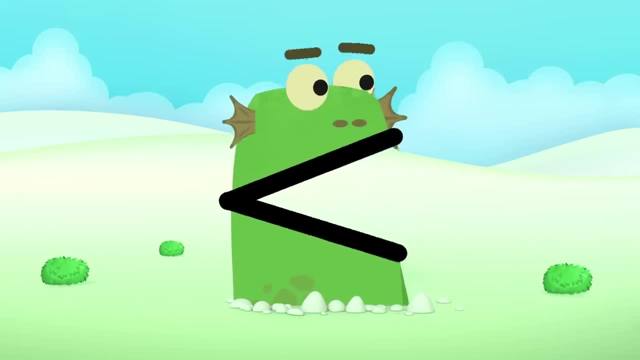 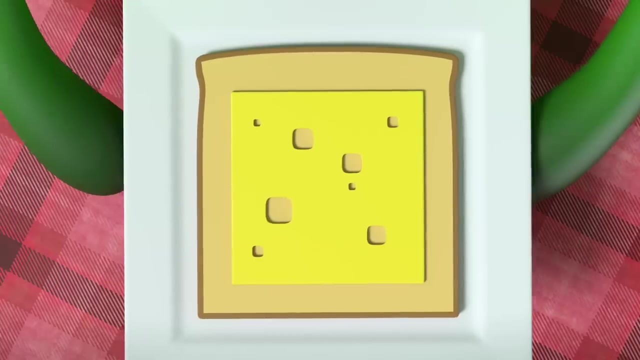 Ah, That's the dose you need. Sounds good. I think it's capable of doing it, But I need to stay strong to stay alive. Please take that irrational measure. Eat you silly. We like you. I like square cheese. 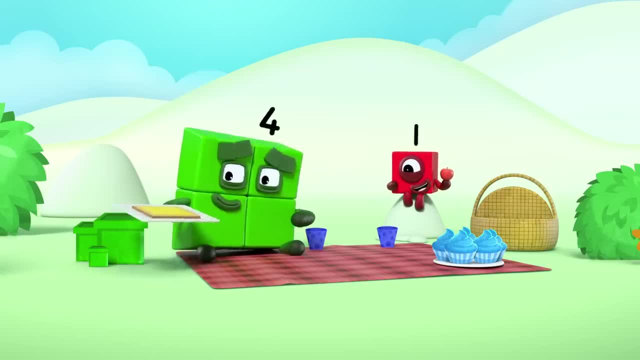 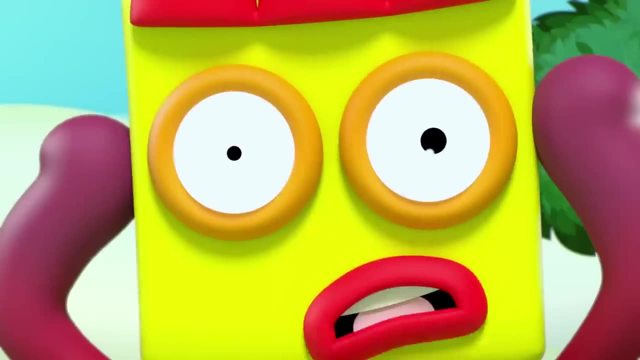 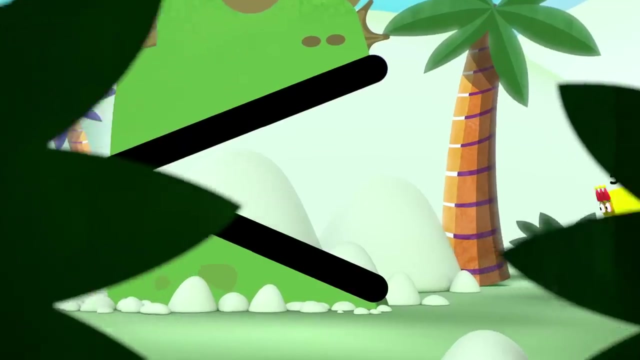 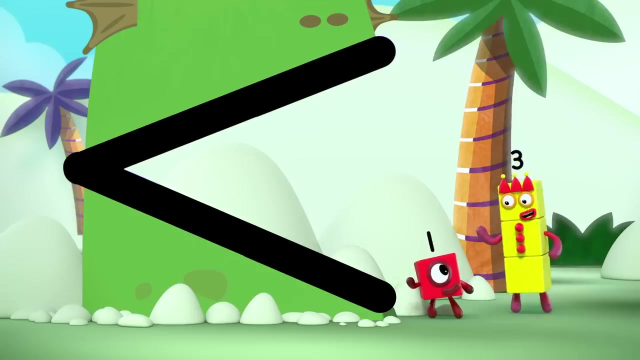 I like it. in my tummy There's a monster. It wants to munch us, crunch us, gobble us up, Run hide. Look a cave We can hide in there. You go first one. You're smaller than me. 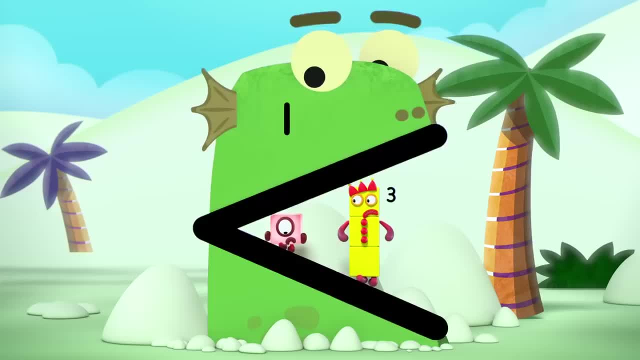 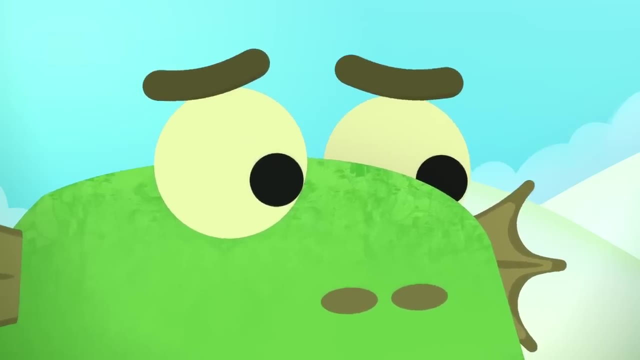 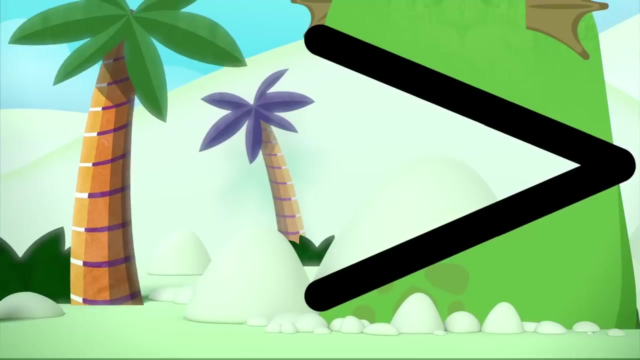 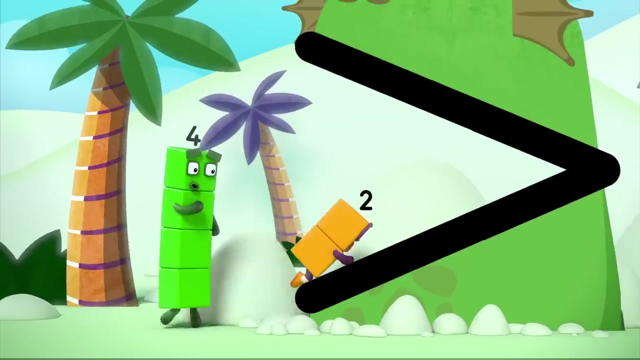 We should be safe in here. One is less than three. Me like bigger numbers, So me like three. Four: Me want to meet you, not eat you. Where can we hide? Look a cave, You go ahead. two: I'm bigger than you. 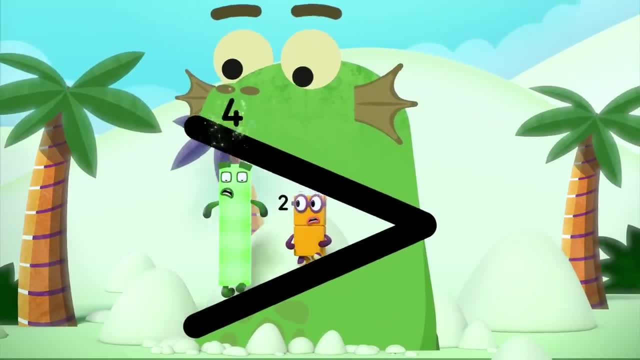 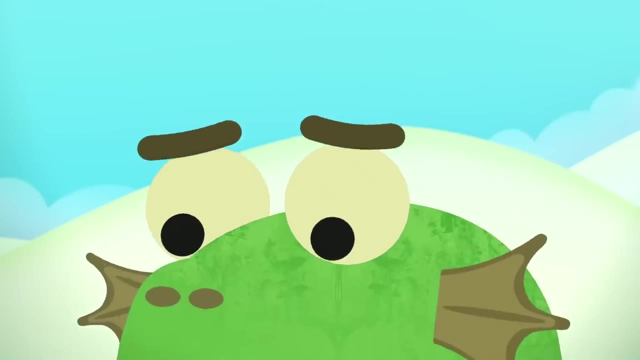 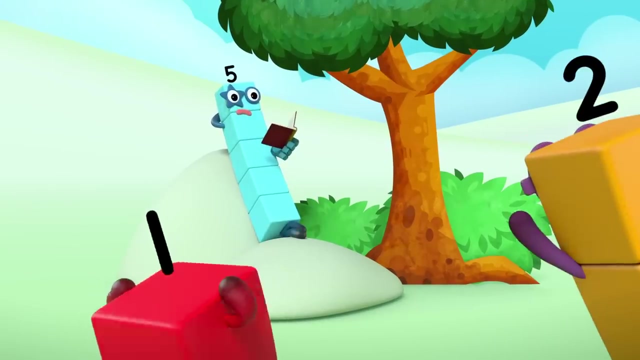 We should be safe in here. Four is greater than two, So me like four, Like I like square cheese in my tummy. No, Stilly, There's a monster that wants to munch us, gobble up us up In its tummy. 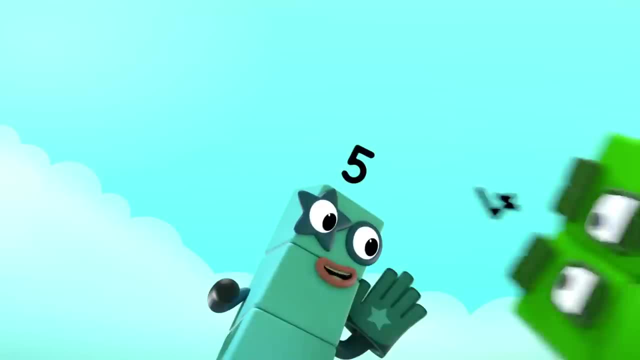 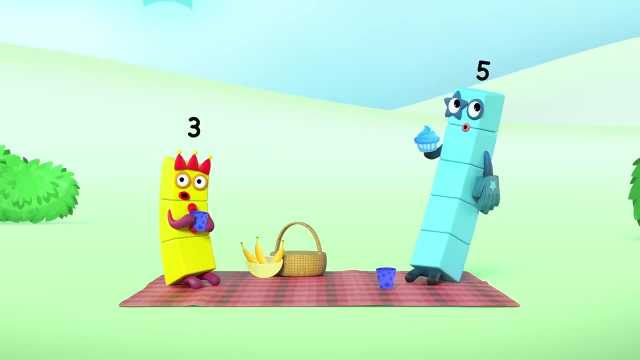 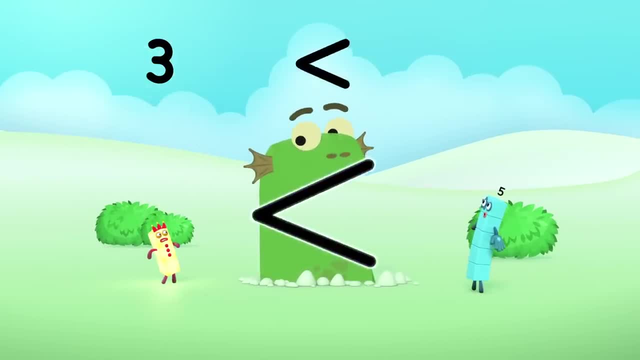 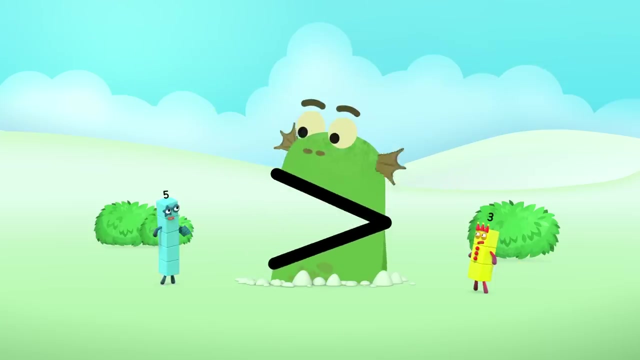 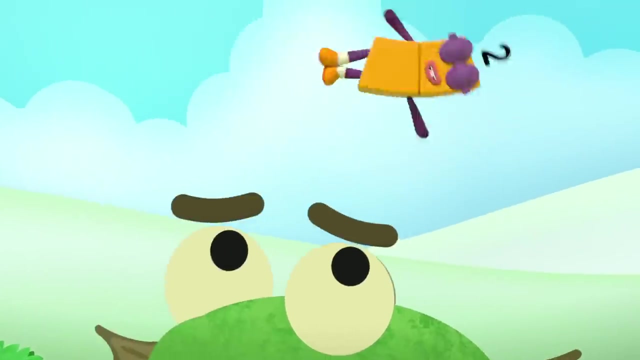 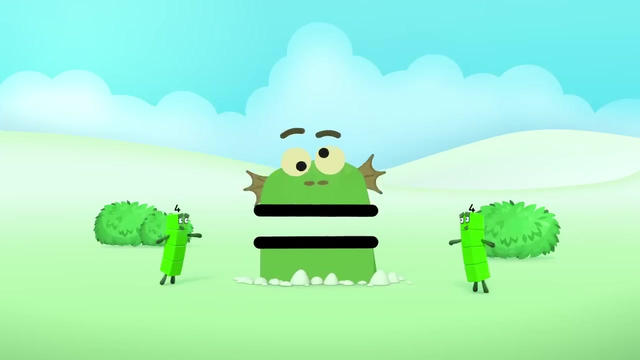 Ok, Ok, Ok, Ok, Ok Ok. Three is less than five. me like five. Me mean five is greater than three. me like five. Three is less, Five is greater, Three, five one. We're both the same. Four equals four. 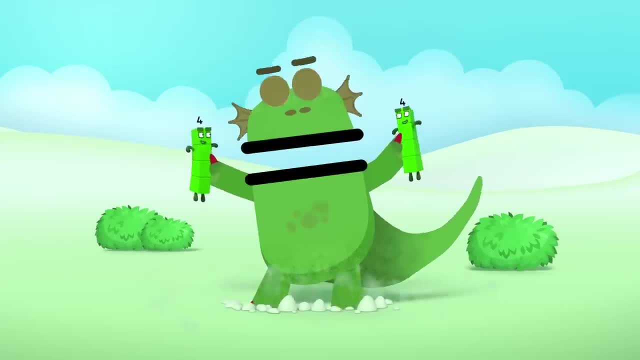 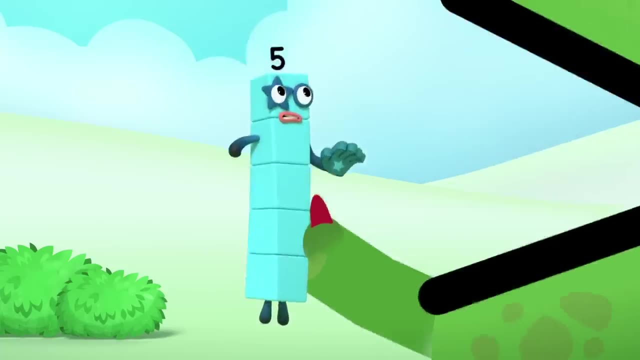 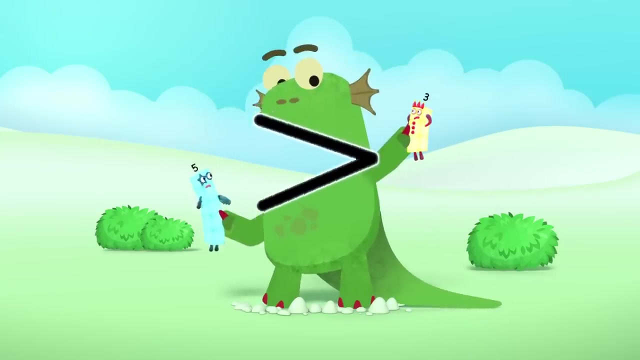 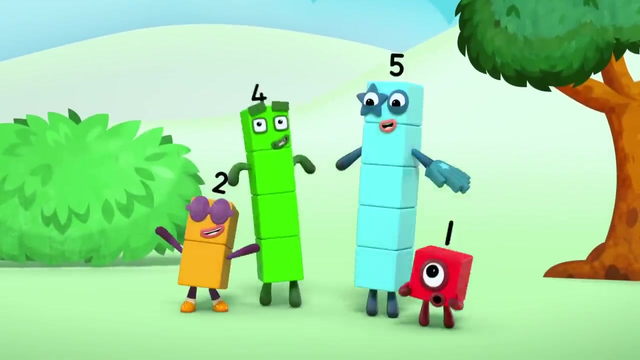 You can't eat us now. Me no like to eat you silly. What me like to play with you? Play with us. Five is greater than three, so, Bloxilla, play with five. What Hooray, Play with me? Play with me. 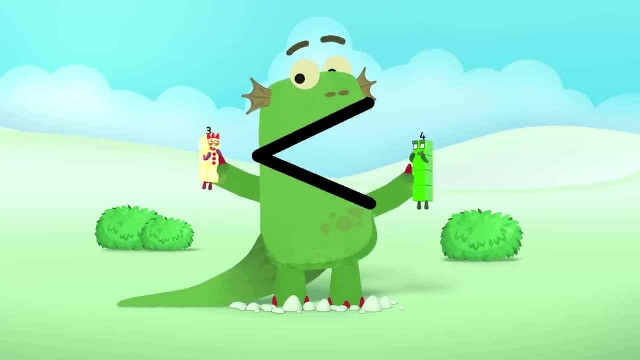 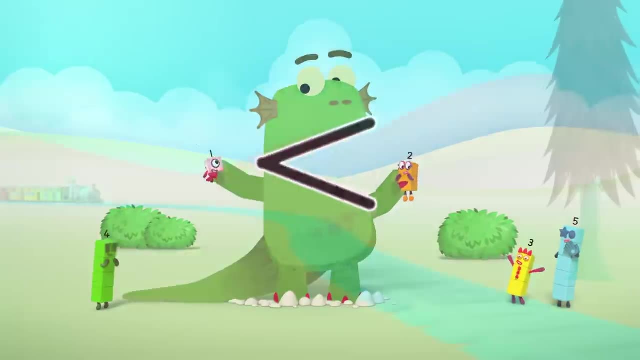 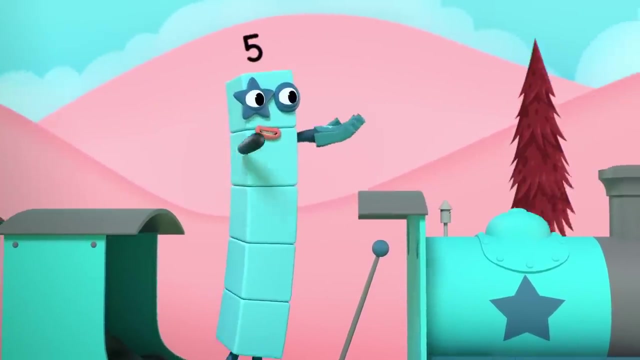 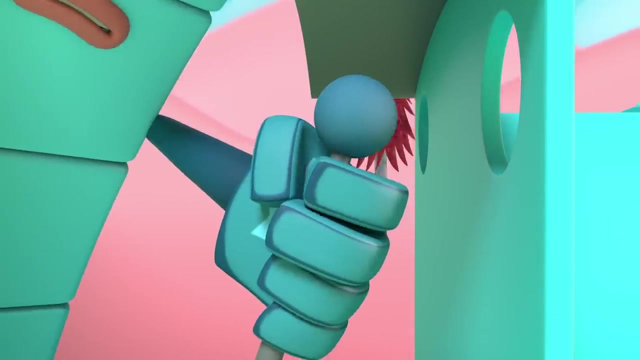 Bloxilla play with number blocks. Three is less than four, Three is greater than two, One is less than two. I am five. I feel alive whenever I can drive my train. Only five, no more, no less- can drive. the number blocks express: No, I'm getting on the train. 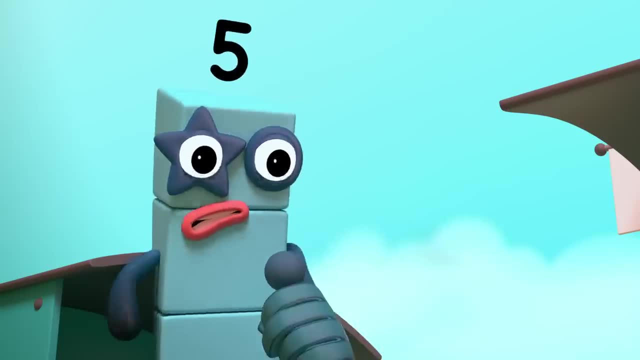 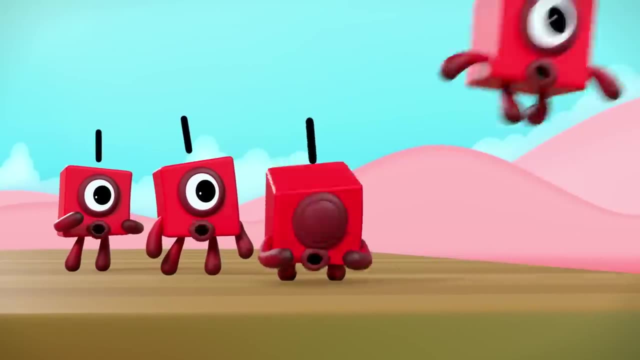 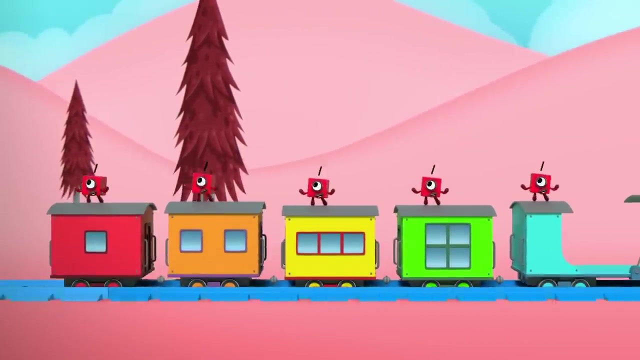 Let's be on our way again. boo-hoo, We have to get the train to stop, So hop, hop, hop, hop, hop on top. Only five can stop the train. So how do we make five? again, Only five, no more, no less. 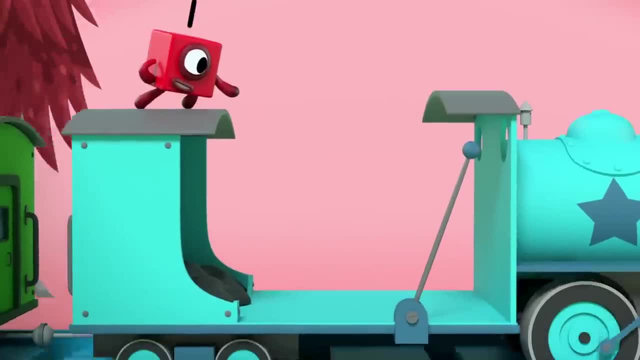 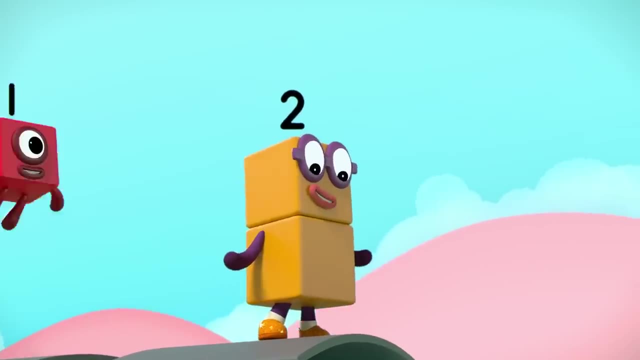 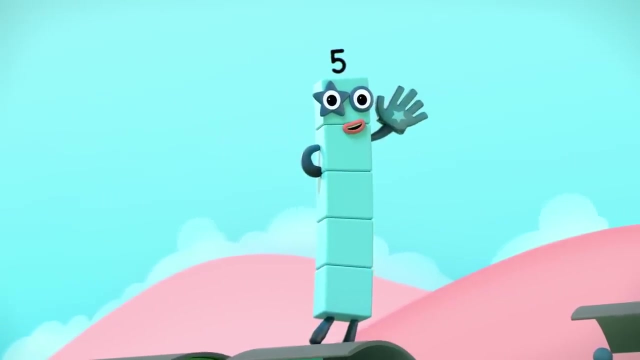 And to stop the number blocks express. I think I know what must be done. Let's stop the train by adding one. One plus one equals two. Two plus one equals three. Three plus one equals four. Four plus one equals five. Only five can stop the train And I am back to five again. 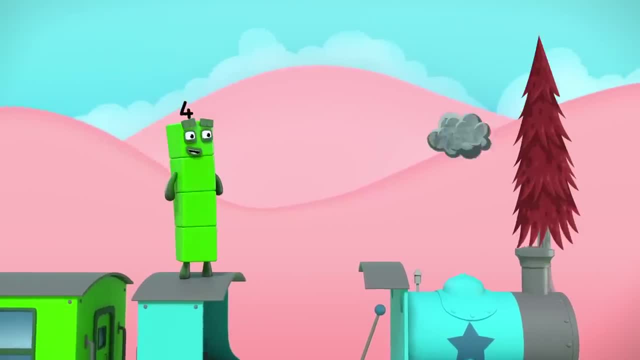 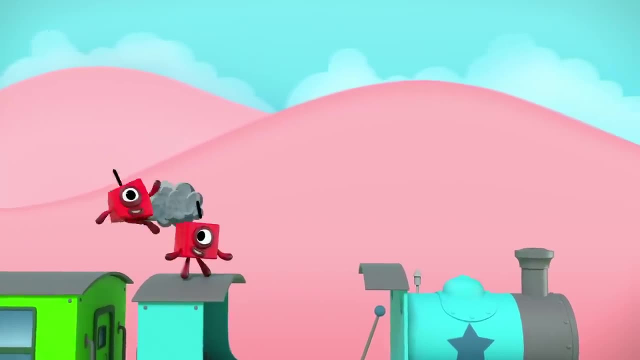 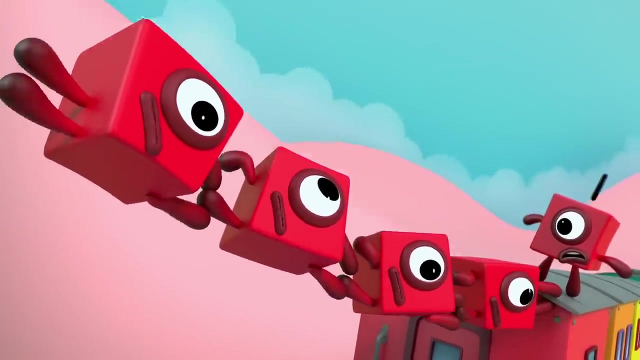 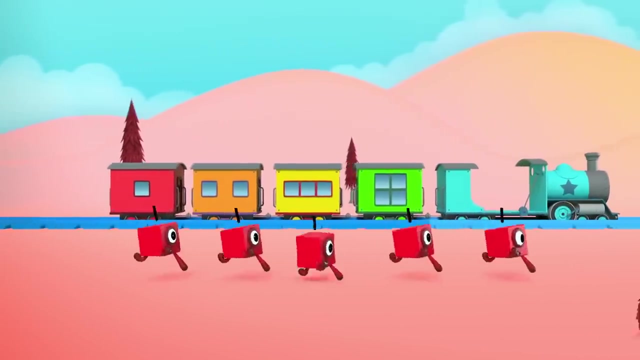 Five minus one equals four. Four minus one equals three. Three minus one equals two. Two plus one equals three. Two minus one equals one. Can you help us, pretty please? We need to get back on the way. Only five can stop the train, So how do we make five again? 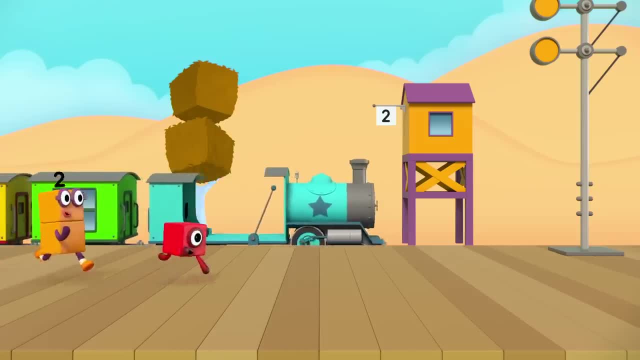 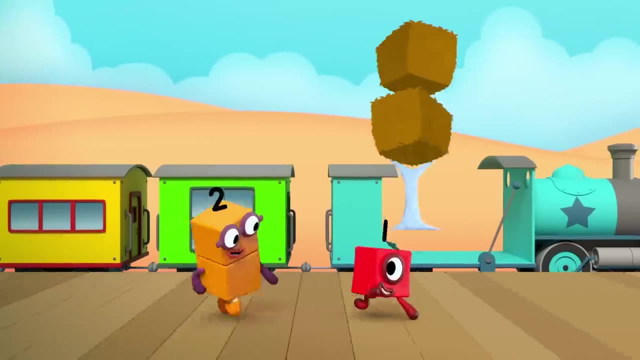 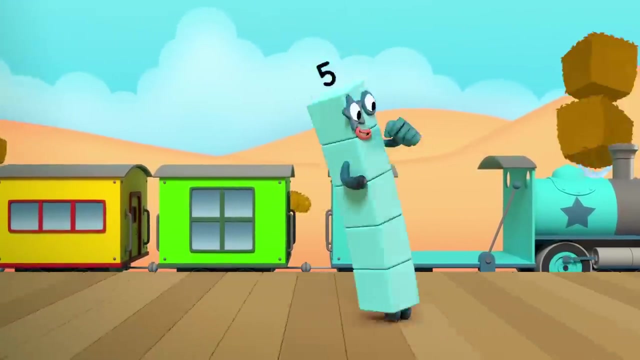 Only five, no more, no less. And to stop the number blocks, express Boo-hoo. We know what we have to do. Stop the train by adding two. One plus two equals three. Three plus two equals four. Four plus one equals five. Only I can stop the train. 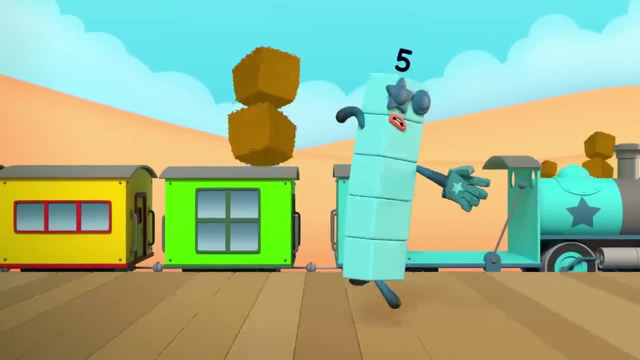 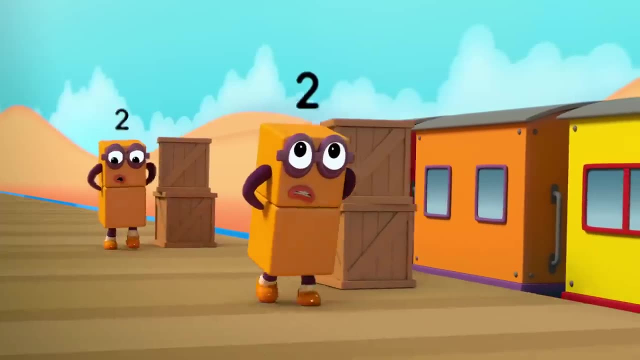 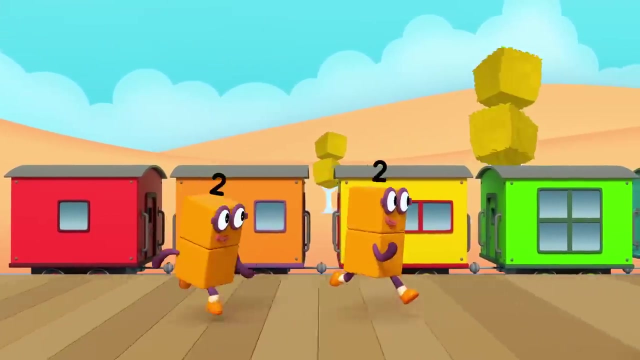 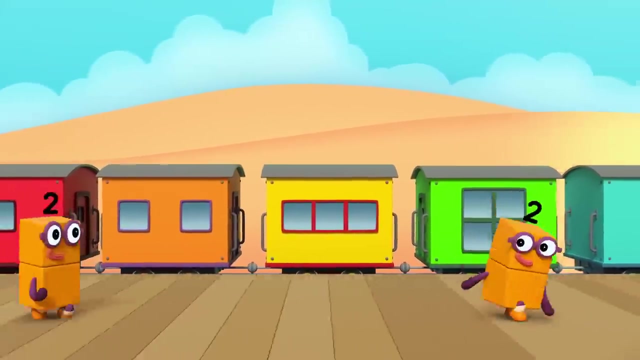 So I am back to try again. Five minus two equals three, Three minus two equals one. Ouch ow, come on twos Time to act like kangaroos. Hop, hop, hop, hop. Two plus two equals four. Four minus two equals two, Especially matte fourth. 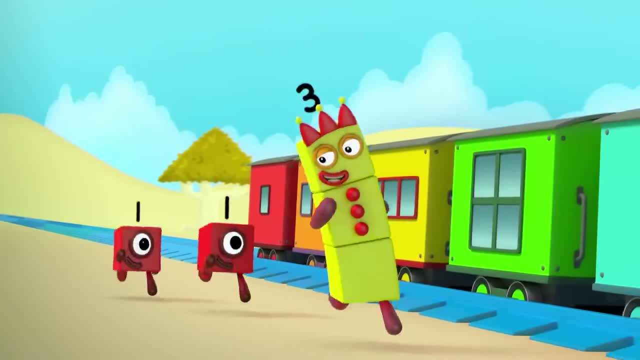 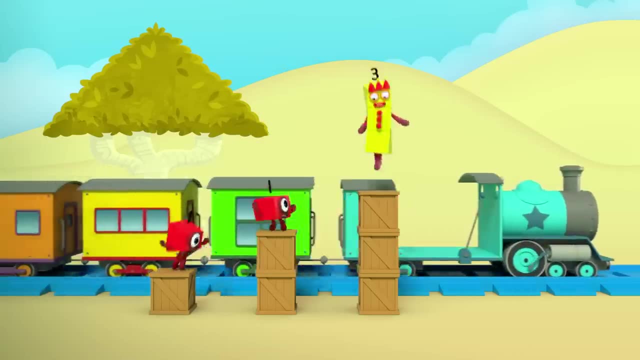 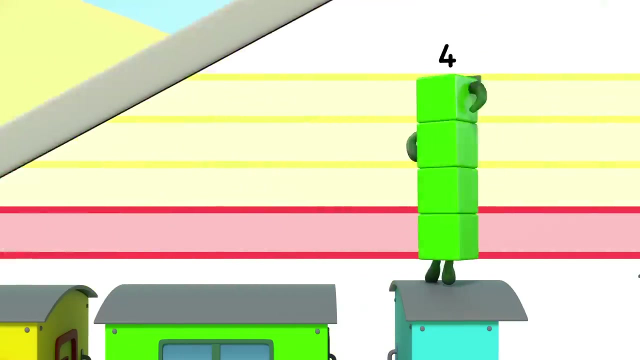 Five minus two equals three, 자기 spirited. And I am back to five again. Five minus two equals three. Three plus two equals four. So I am back to five again. Three minus two equals three. Three minus two equals three. Three plus two equals three. And to stop the train by adding three. 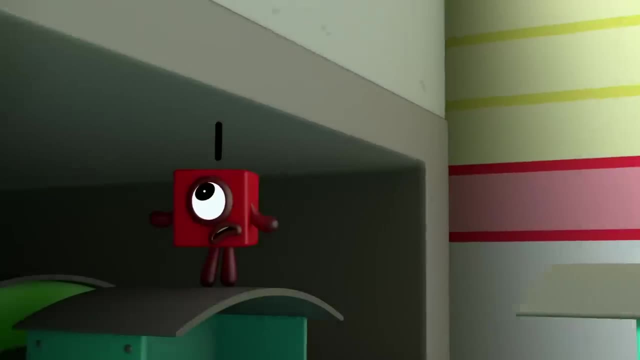 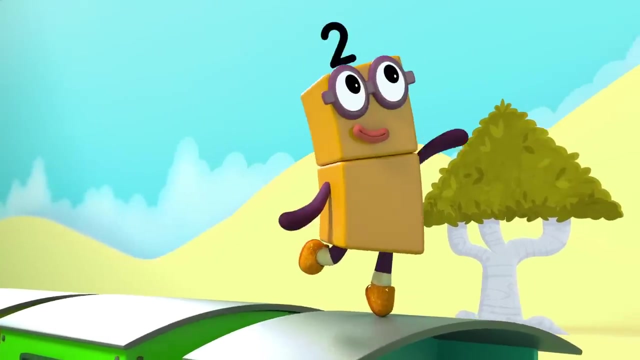 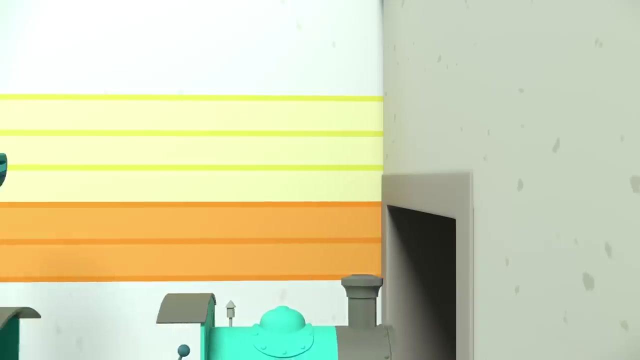 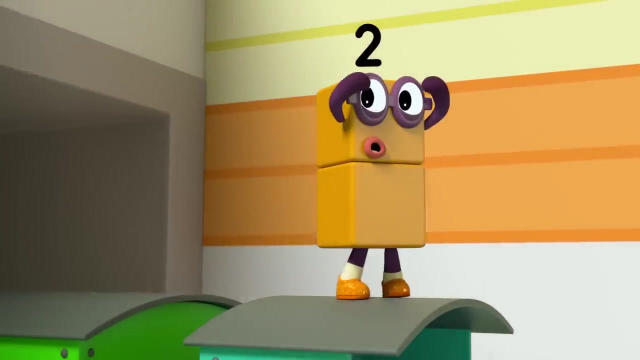 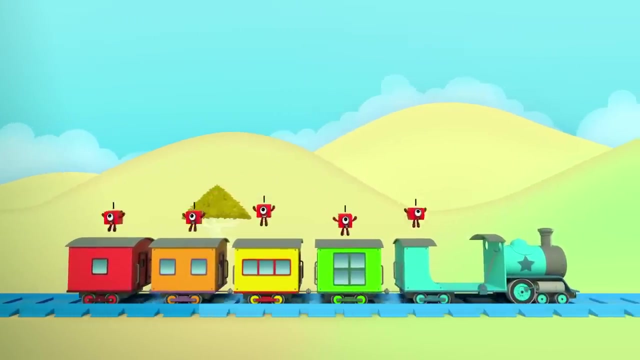 Three minus two equals three. Two minus two equals three. 2 plus 3 equals 5. Only I can stop the tree. and I am back to 5 Minus 3 equals 2. Only 5 can stop the train. so how do we make 5 again? 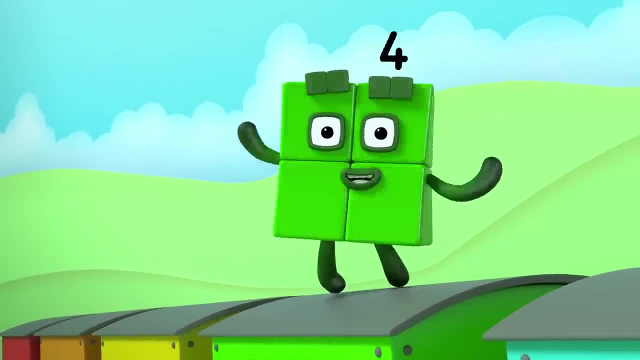 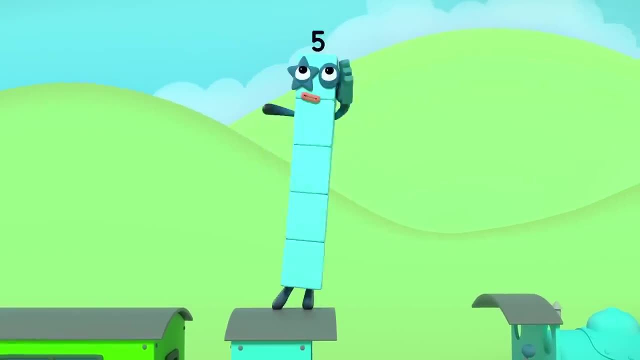 I am square, you mean 4, let's stop the train. by adding 4, 1 plus 4 equals 5. Only I can stop the train. so here I am to try again. Only 5,, no more, no less, can stop the number blocks express. 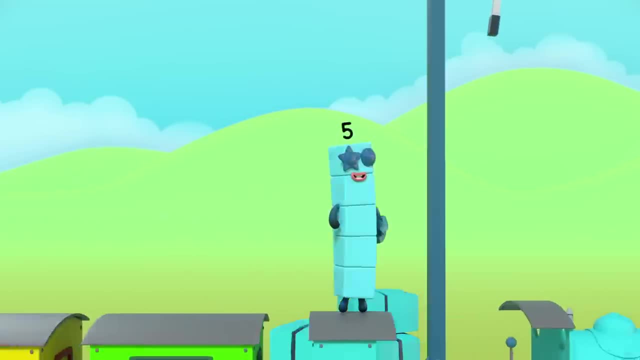 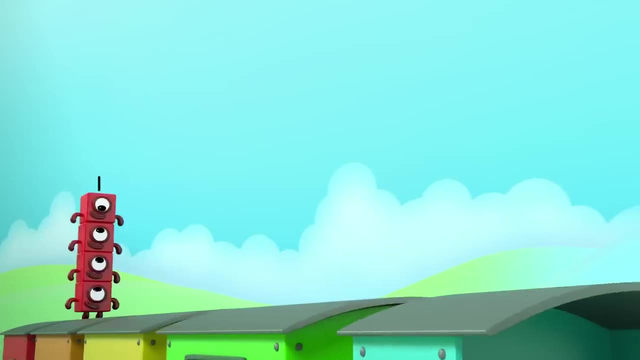 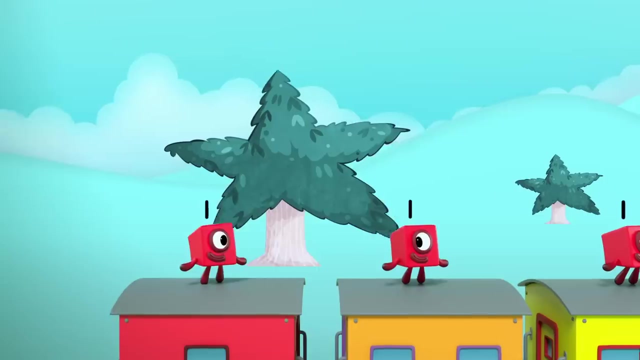 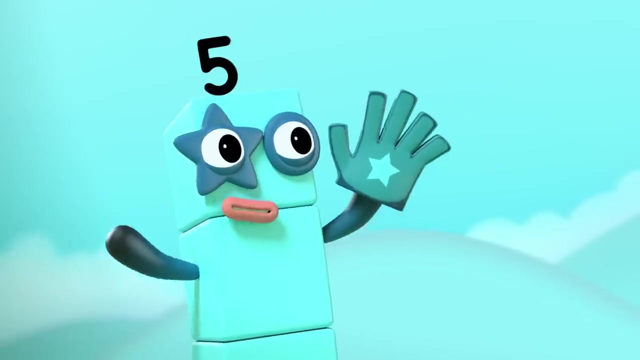 Woohoo Minus 4 equals 1. Only 5 can stop the train. so how do we make 5 again? 1, 2, 3, 4, hi, Only 5 can stop the train. so here I am to try again. 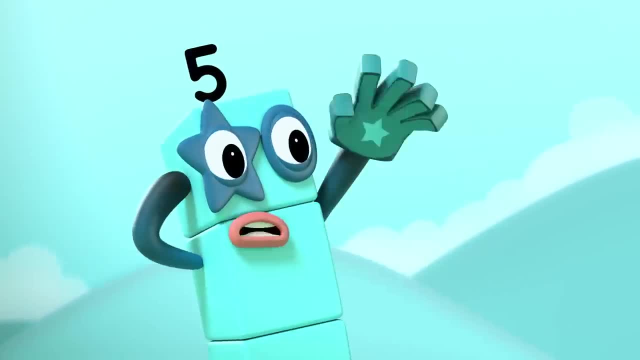 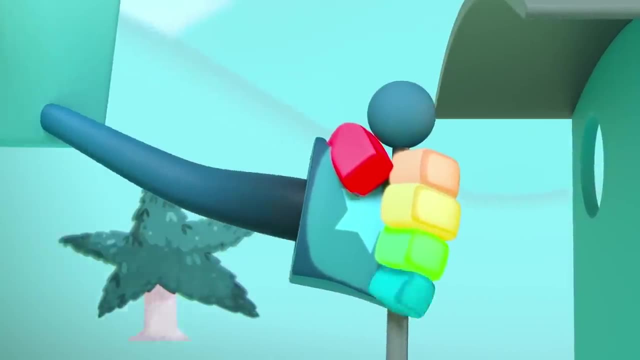 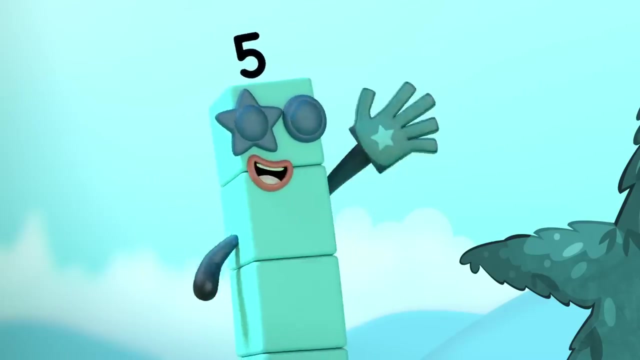 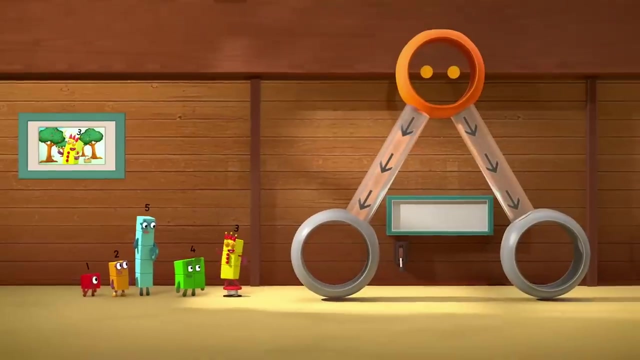 Uh-oh, no, we're in a mess. Stop the number blocks express 1,, 2,, 3,, 4,, 5! High five, Success. I stopped the number blocks express Woohoo, Welcome, welcome, welcome to my fantastic Bun Fruit Factory. 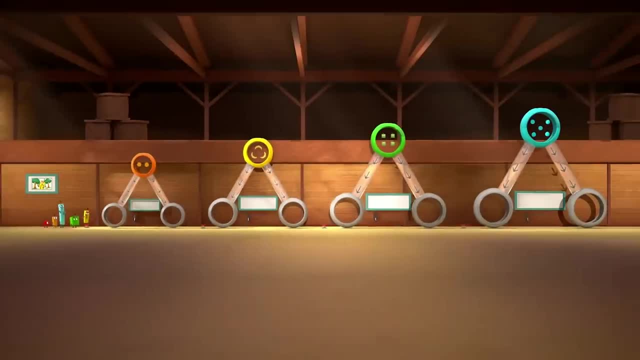 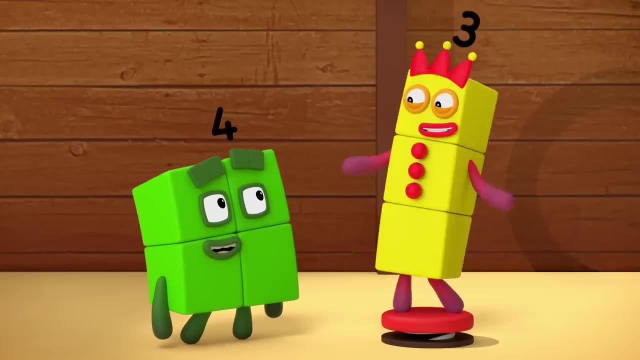 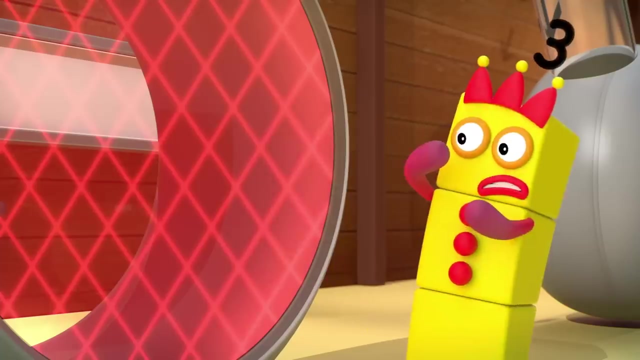 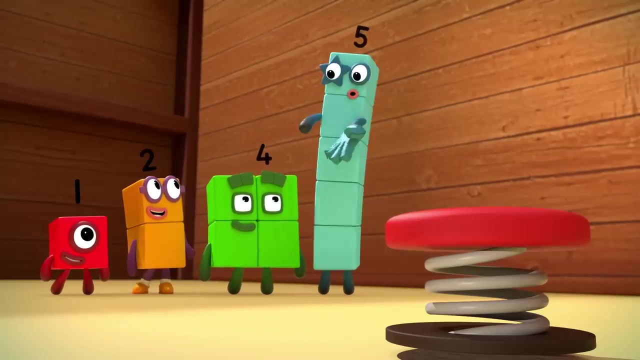 Where we serve up fresh fruit all day. Ooh, Wow, How do they work? Oh, easy peasy. lemon squeezy, Obviously. I just Oof, Silly thing's broken. There are two oranges in there, Maybe if 2 tries it. 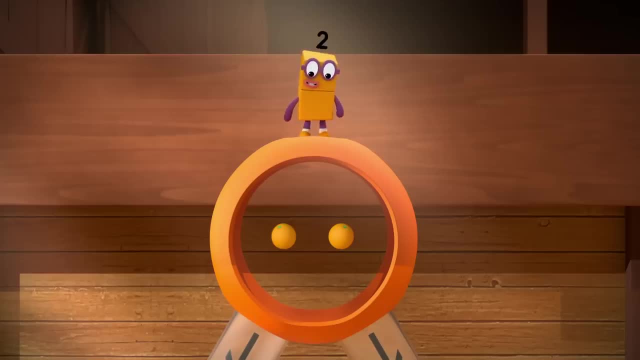 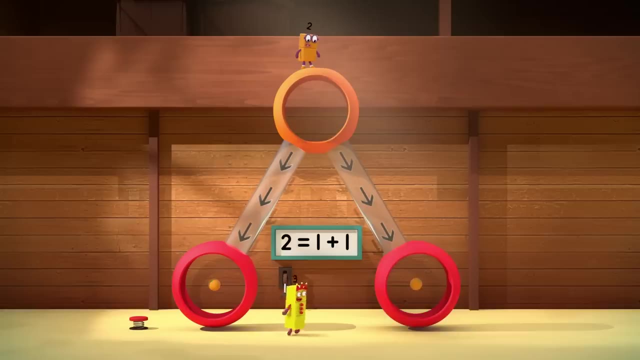 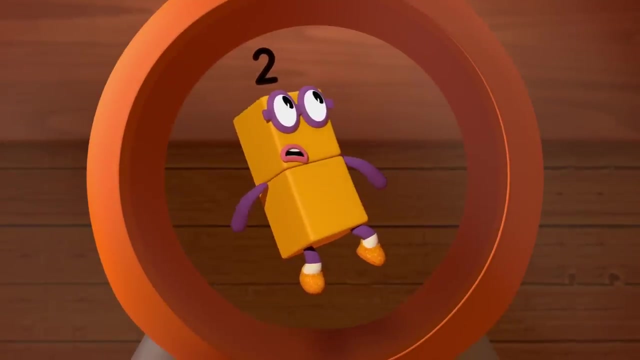 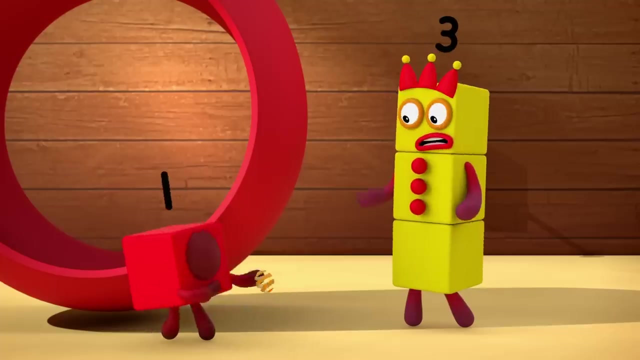 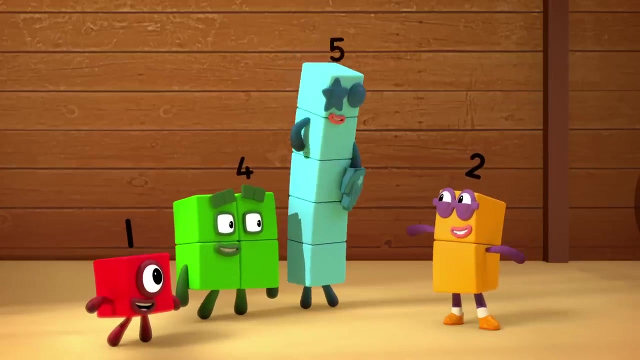 Ugh Ugh. 2 equals 1, 1 plus 1. Oof, How do I? 2 equals 1 plus 1. Yum Ta-da. Look. 2 at the top Splits into 1 and 1 at the bottom. 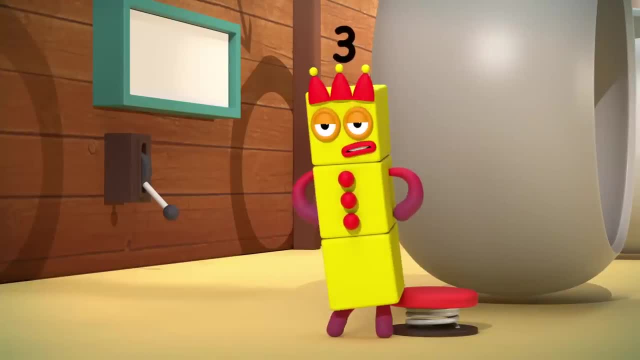 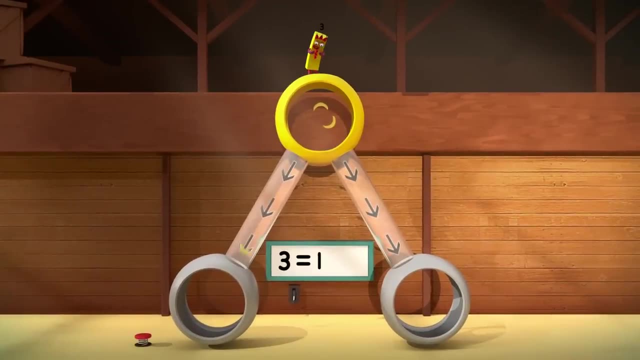 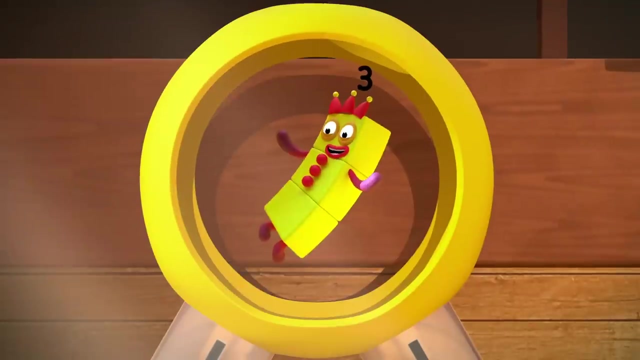 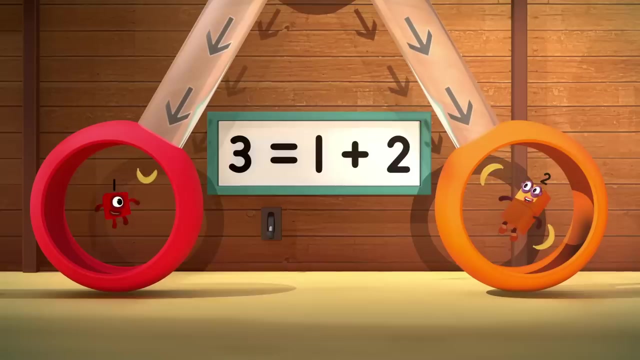 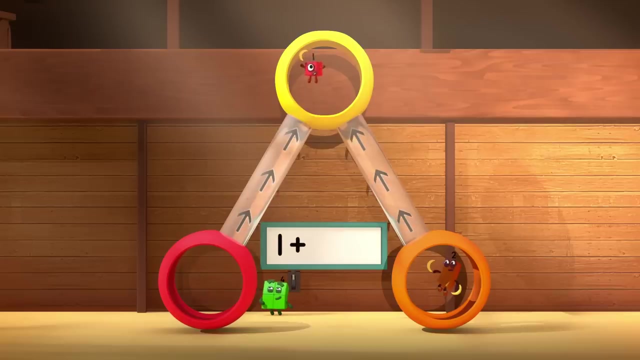 Ahem, I want fruit. It's my turn. 3 equals 1 plus 2. Yummy, yummy, yummy. 3 equals 1 plus 2. Oh, Where's 3?? Let's try this lever. 1 plus 2 equals 3. 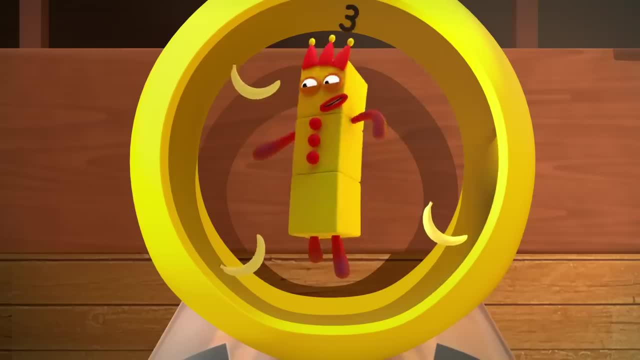 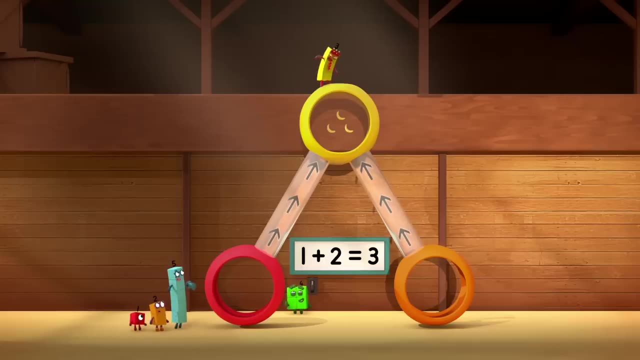 Oh, It works both ways. Oh Hey, Those are mine. 3 equals 2, 2 plus 1 plus 2. 3 equals 1 plus 2. 2 equals 1 plus 2. 2 equals 1 plus 2. 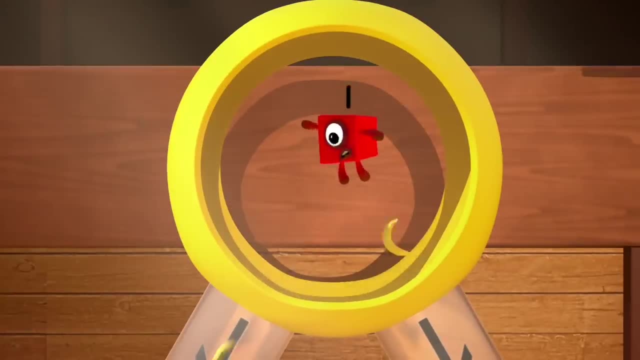 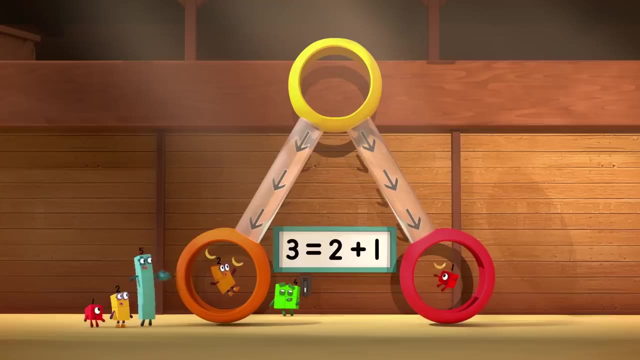 2 equals 2, 2 equals 1 plus 2, 2 equals 1 plus 2, 2 equals 1 plus 2, 2 plus 2 plus 1 equals 2, 2 plus 1. Now there's 2 over here and 1 over there. 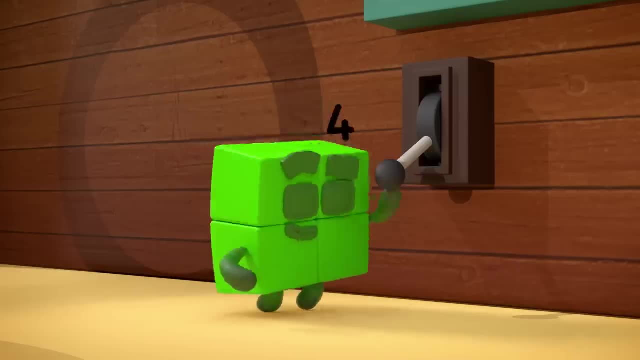 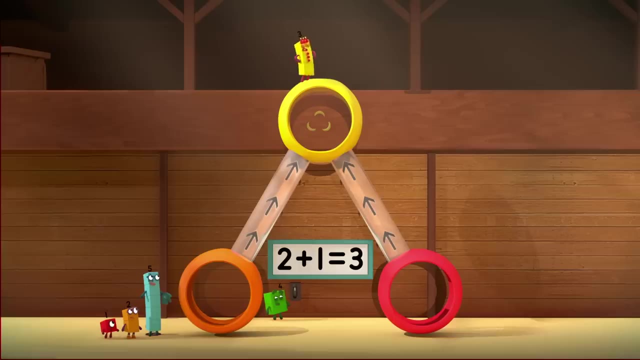 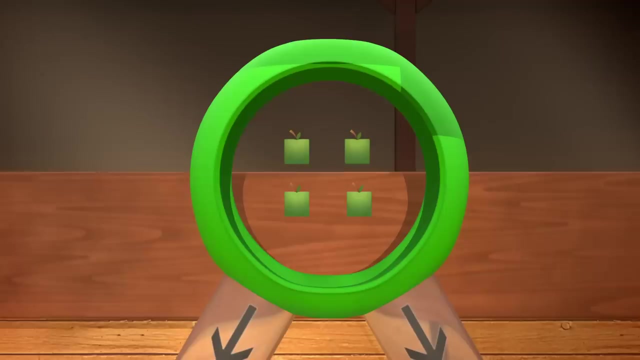 But 3 doesn't get her Bananas again. 2 plus 1 equals 3. Hey, I'm still hungry, Mmm. Look, Apples, Square, apples, Huh, Energonum, Yum-yum Huh. 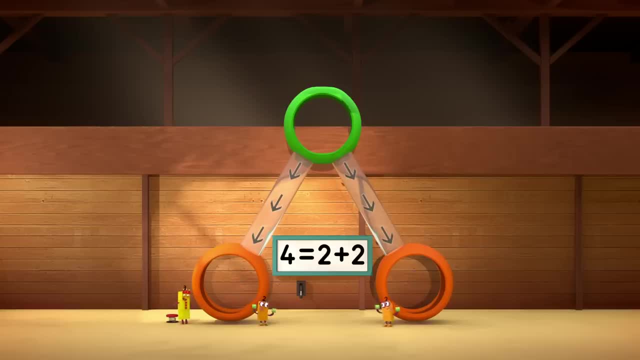 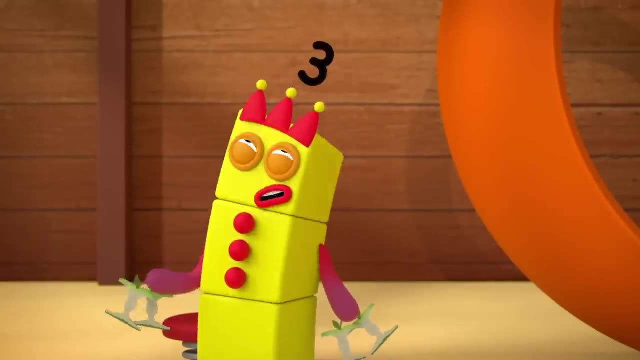 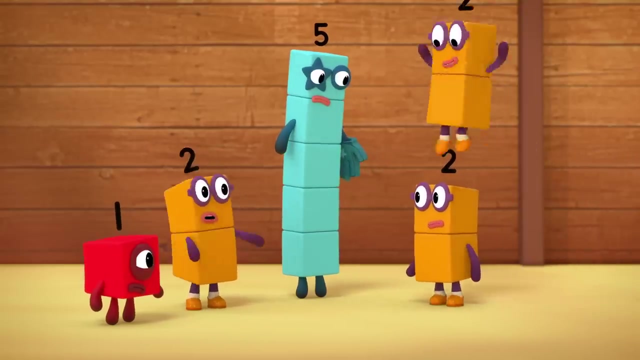 Yum-yum, No, no, no, you silly machines, Poor Three. We need to find a way to make three apples come out. Look Four new apples at the top. I know how to make three, Here you go Three. 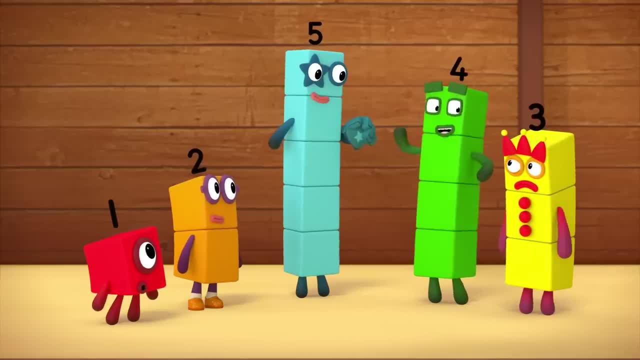 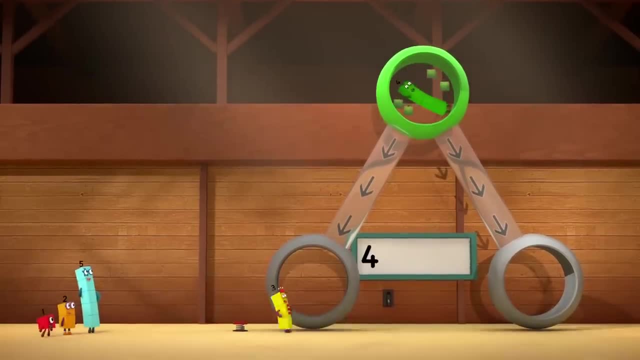 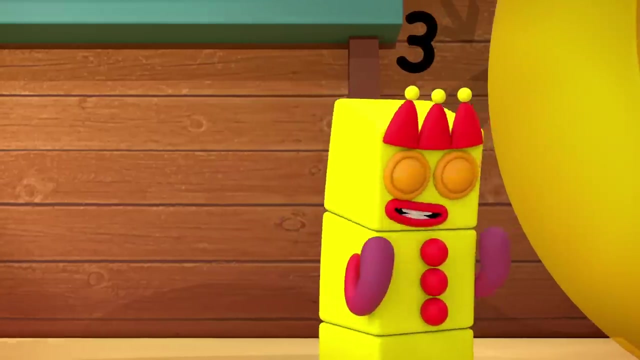 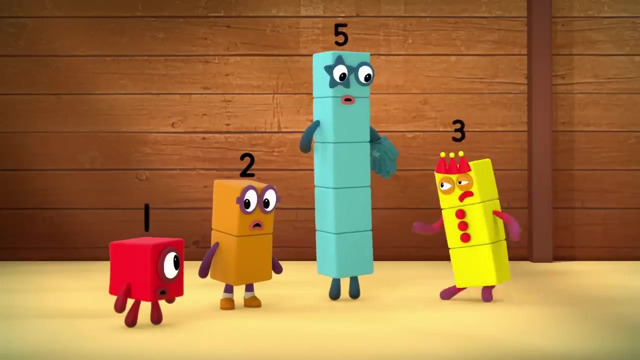 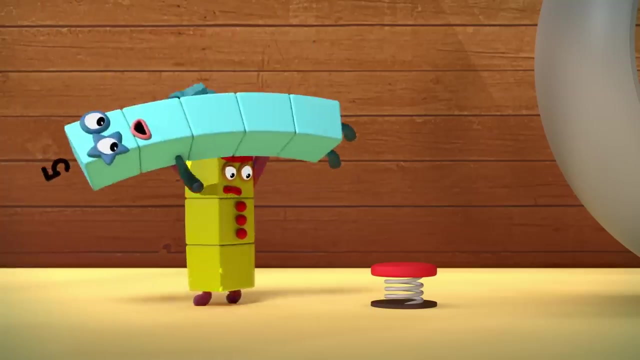 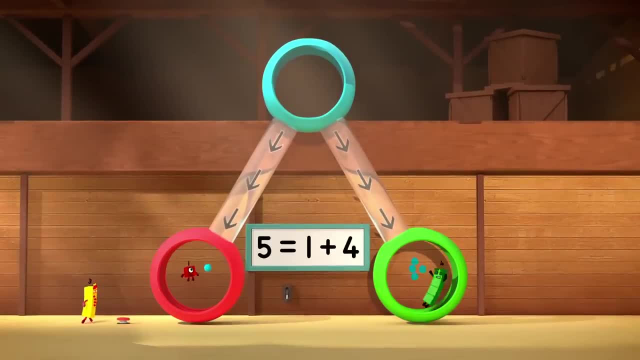 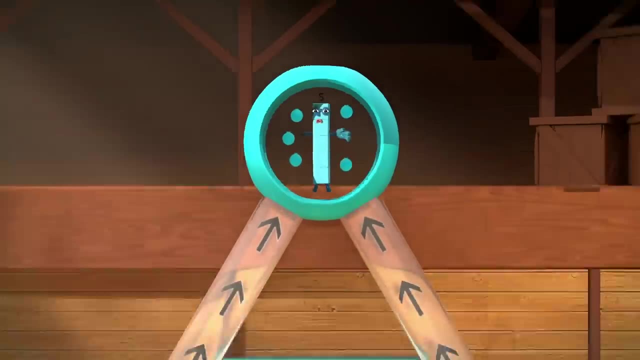 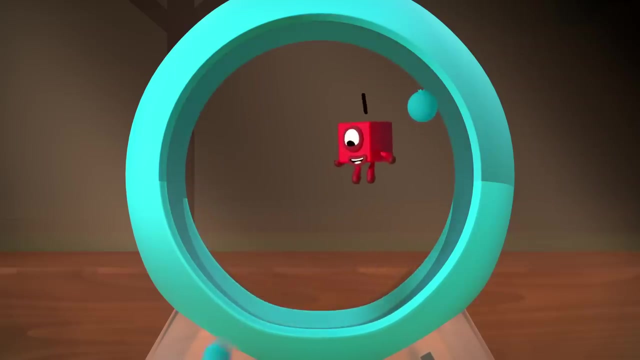 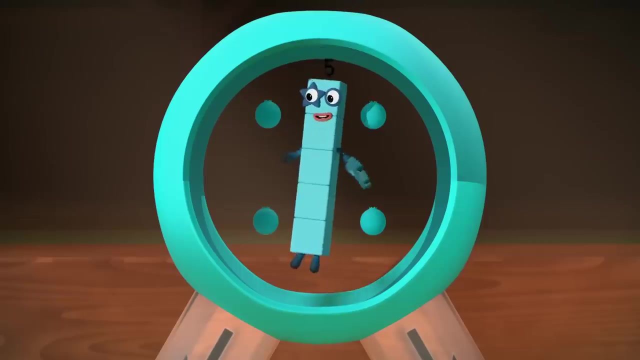 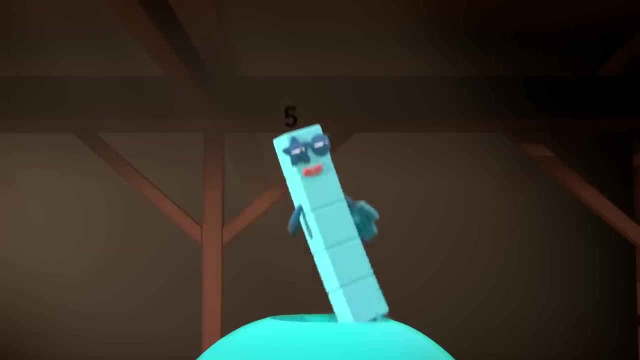 Five equals one plus four. One plus four equals five. Yikes, Five equals four plus one. Four plus one equals five. Five equals two plus three. Two plus three. Two plus three equals five. That's going far too fast. Five equals three plus four. 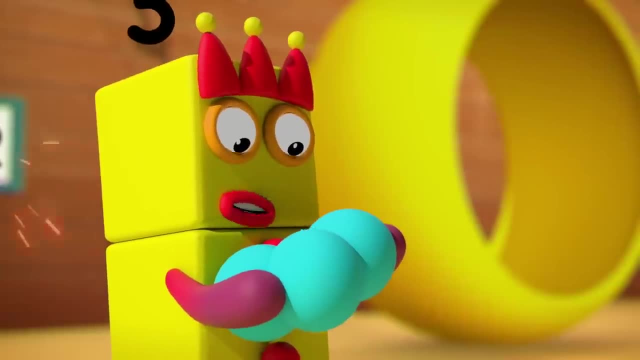 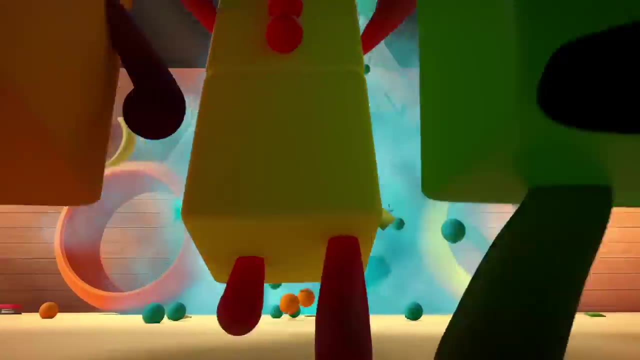 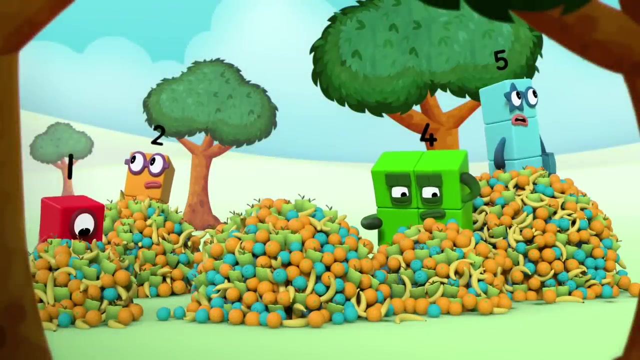 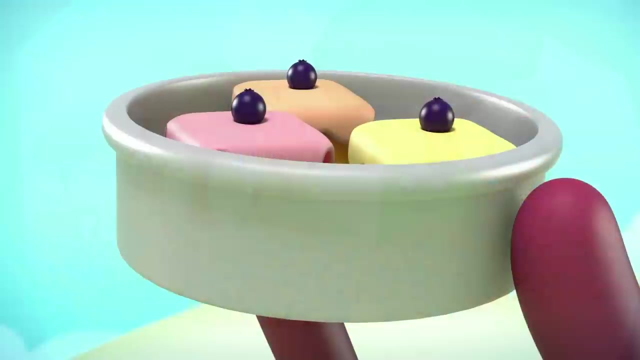 One, two, three, Three blueberries, Run, Run, run, run, run, run. Huh, I told you, Easy peasy. lemon squeezy: Oh, Oh, Uh-uh-uh, Ready Oh Yum. 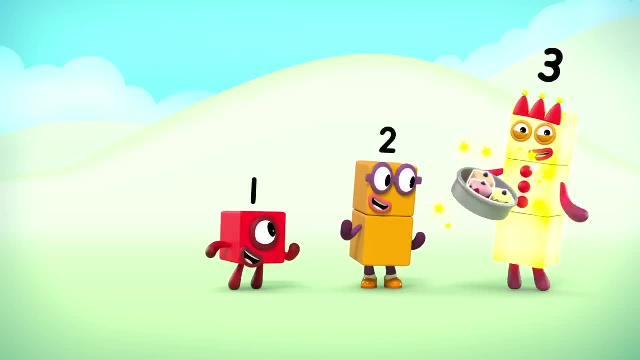 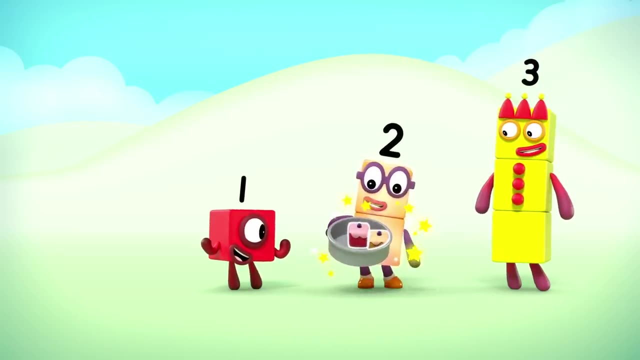 One, two, three, Three block cakes. One for me, Nom nom nom And one less than three is One, two, Two block cakes. One for me, Nom nom And one less than two is One One block cake. 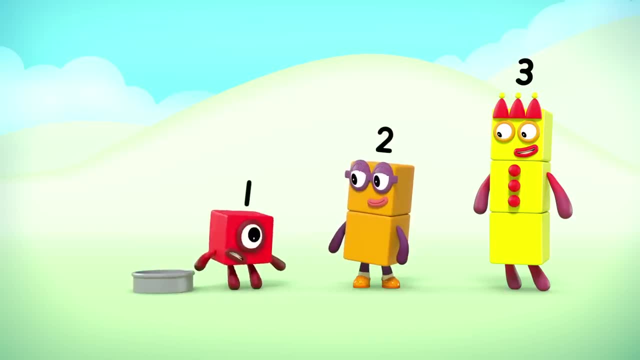 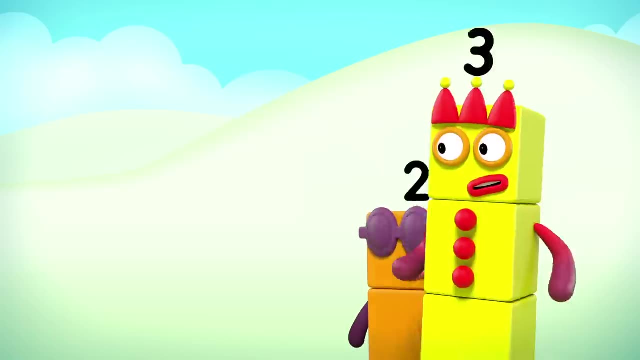 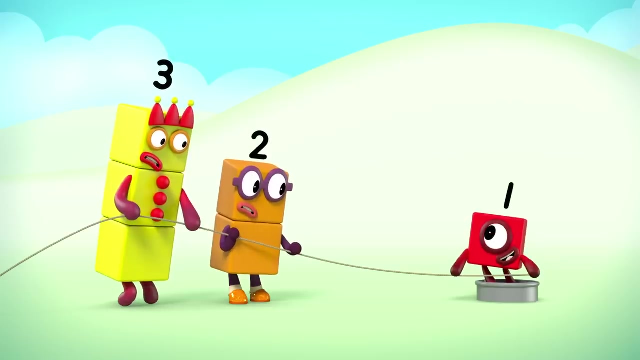 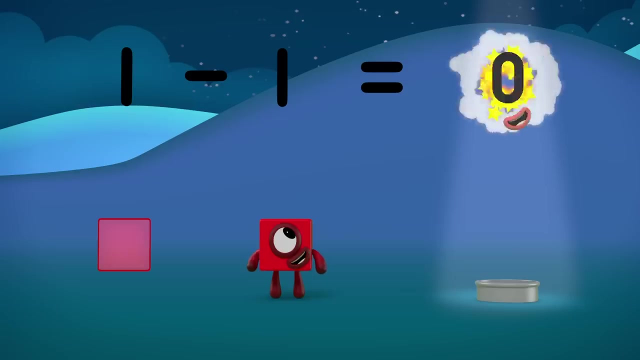 One for me, Nom, And one less than one is. Is What's one less than one? Only one way to find out: Oh, How many blocks are in this tin? One Ready Pull. One minus one equals zero. 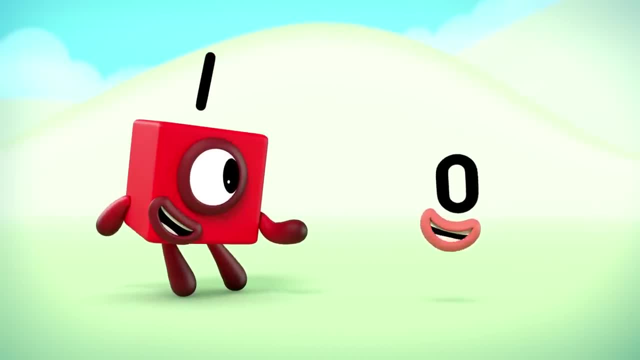 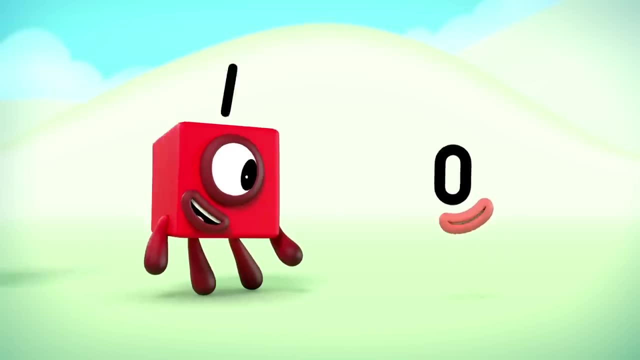 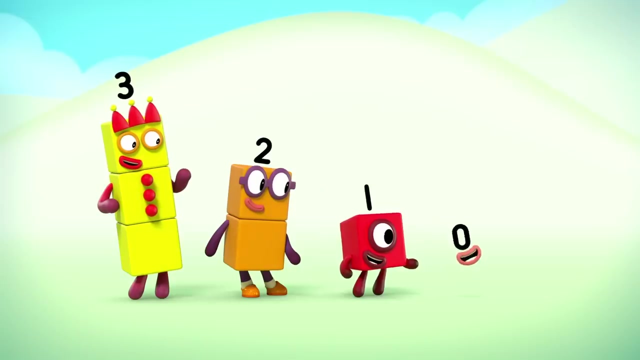 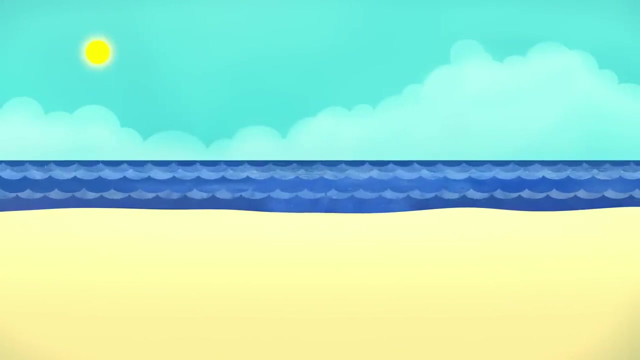 Who are you? I am Zero, the hero, One less than one. Where are your blocks? I haven't got any silly Zero blocks. Wait, is that No music I hear? Follow me. When there are no boats anchored in the bay, you've got zero. 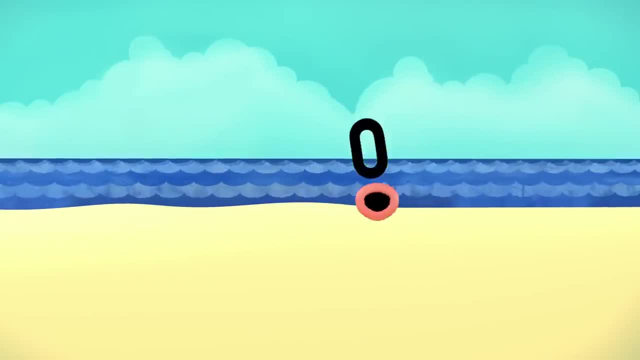 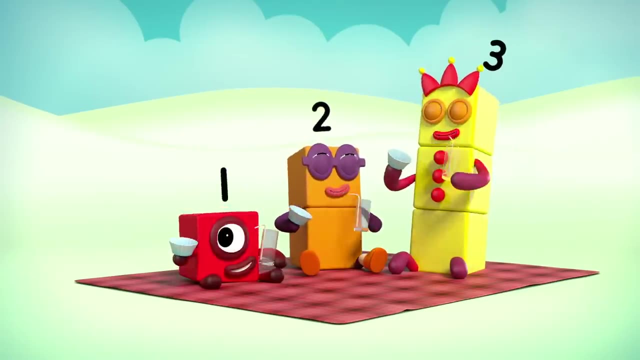 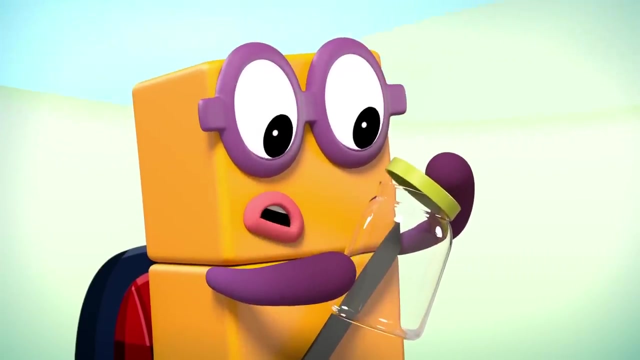 When all the birds have hopped and flown away, you've got zero. When you've eaten all the cupcakes, when you've drunk up all the milkshakes, you've got no cakes, no shakes- You've got zero. When all the sweets have vanished from the jar, you've got zero. 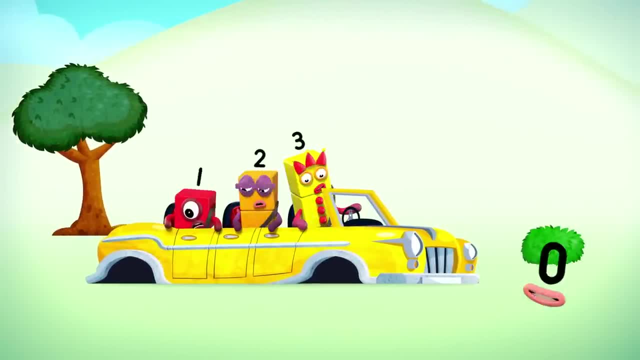 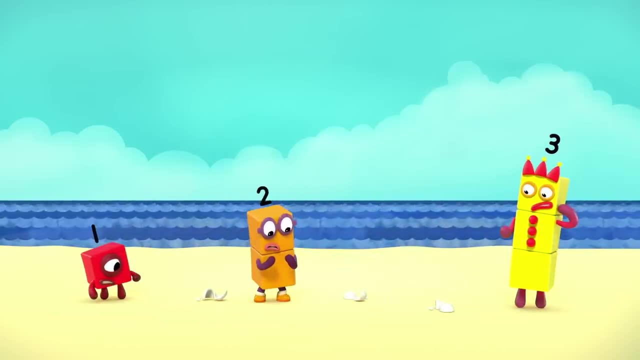 When all the wheels have fallen off your car, you've got zero. When the wind blows down the teacups and you've broken all the teacups, you've got no hats, no cups- You've got zero. I'm the number for nothing. 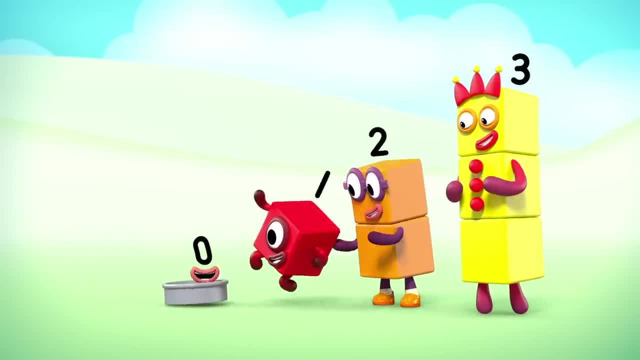 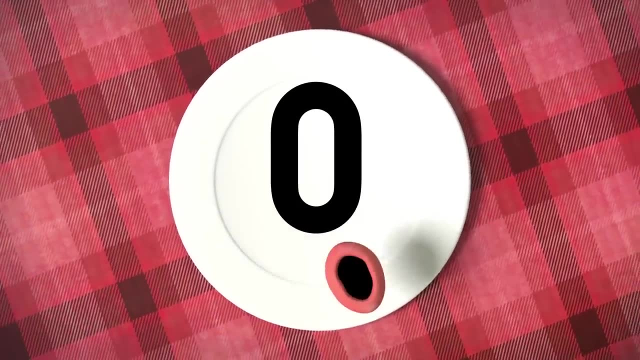 I'm one less than one. when there's nothing or something. I'm the number for none. When there's nothing there to count, none is the amount. You've got zero. When all the bunnies in the field have hopped, you've got zero. 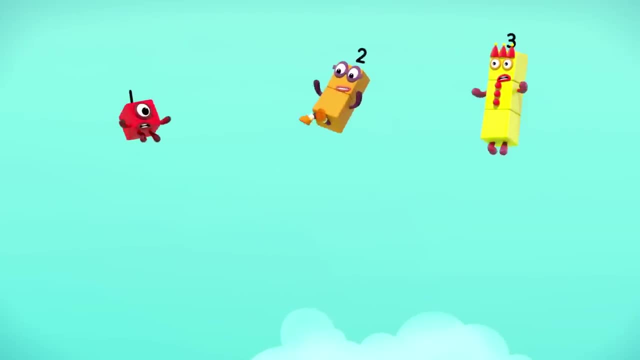 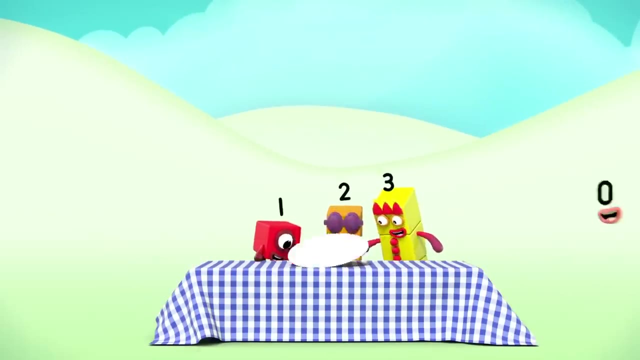 When all the bubbles in the air have popped, you've got zero. When you've jumped in all the haystacks, when you've snaffled up the fluff jacks, you've got no snacks, no snacks- You've got zero. 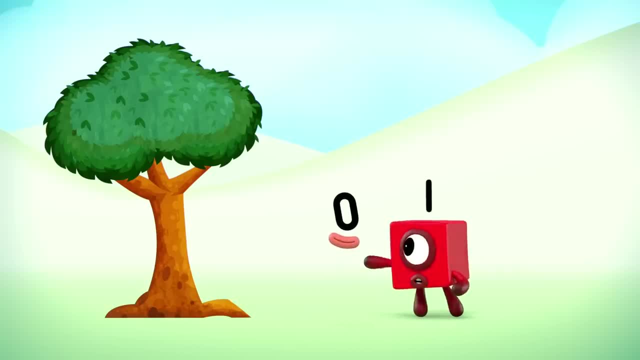 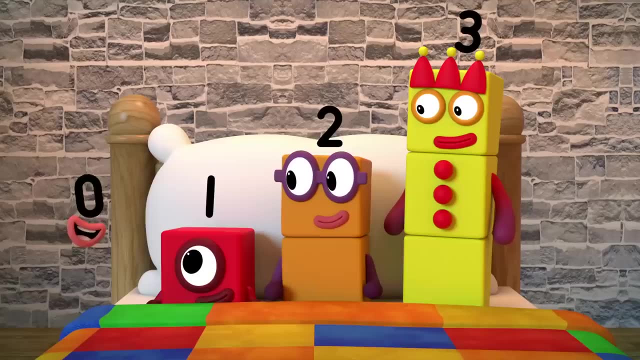 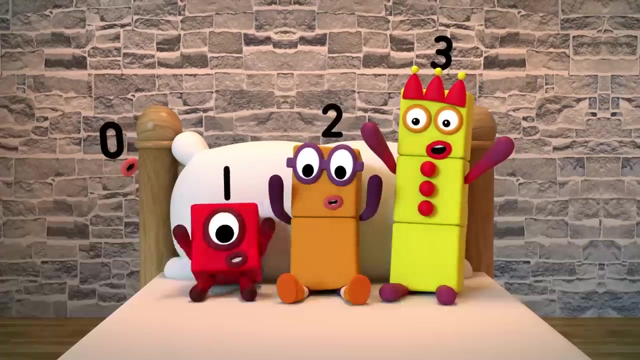 How many elephants in that tree? Zero. How many unicorns can you see? Zero. How many frogs are on your head? How many squirrels in your bed? Zero, zero, zero. I'm the number for nothing. I'm one less than one when there's nothing or something. 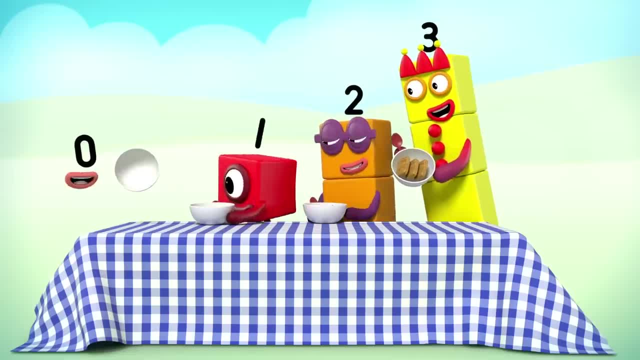 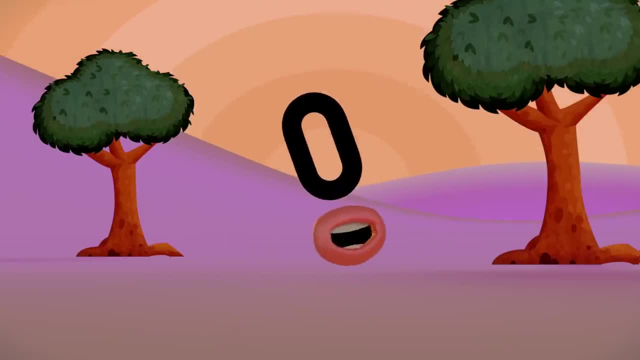 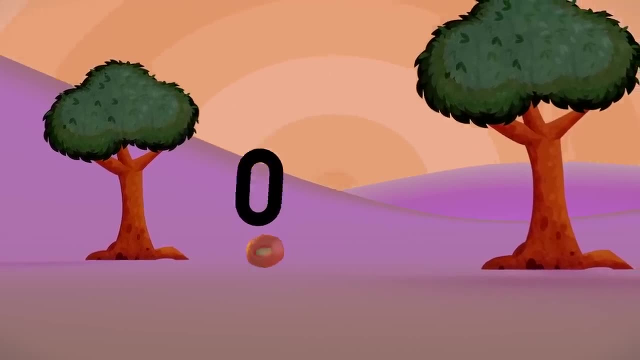 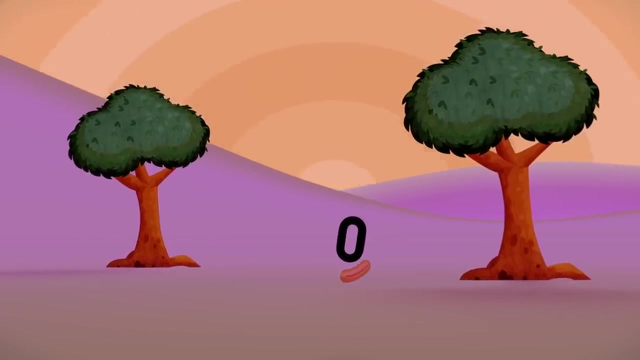 I'm the number for none. When there's nothing there to count, none is the amount You've got: zero. Imagine a world where nothing can bring you down: No one messing around, no one starting a riot, Nothing and no one to stop you from thinking of nothing. 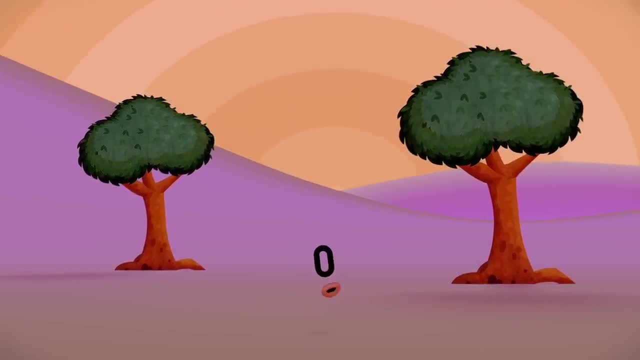 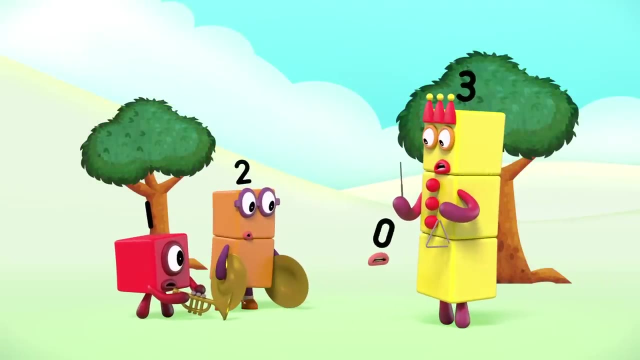 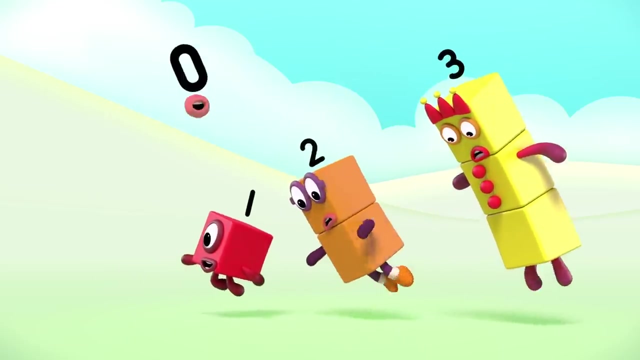 Imagine a world where everything's peaceful and quiet. No, no, no, Zero. zero instruments, Zero, zero trees, Zero, zero gravity, Zero, zero worlds, Zero worlds. Oops, What's this? Nothing. Where are we? 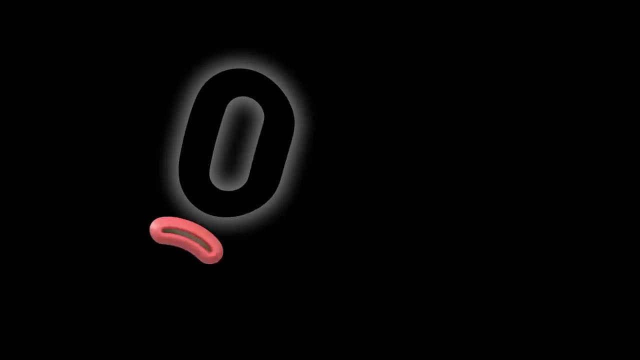 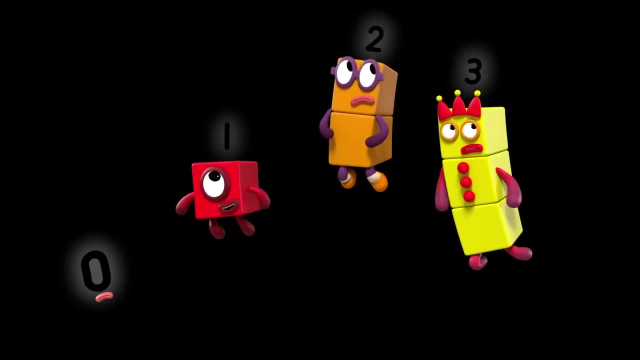 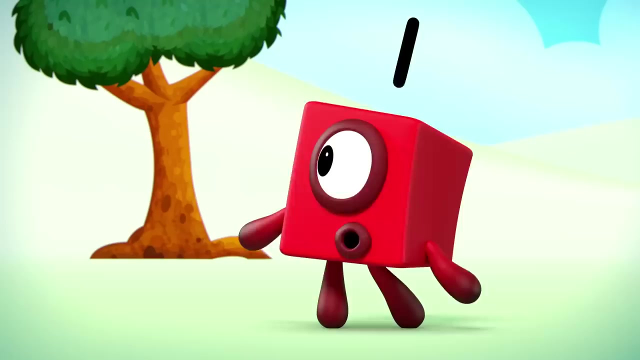 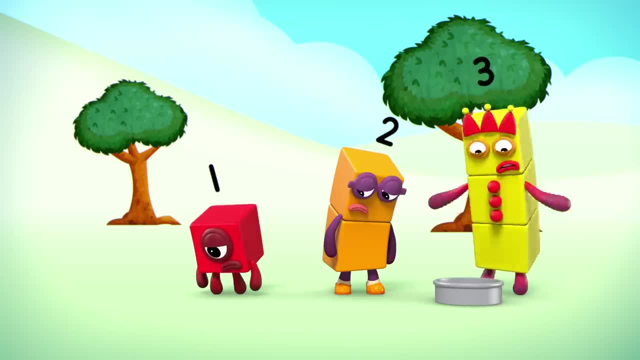 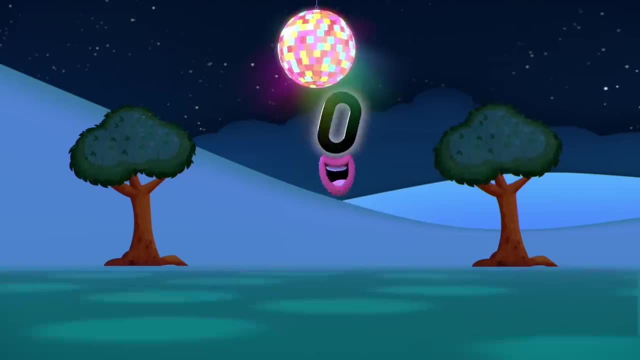 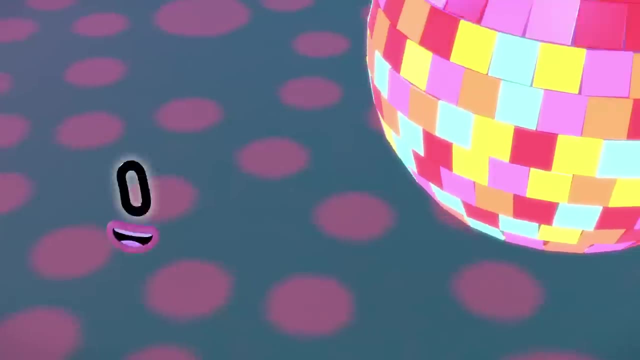 Zero, zeros. Zero was my hero. Ta da. I'm the number for nothing. I'm one less than one When there's nothing of something. I'm the number for none. I'm the number for nothing. I'm one less than one when there's nothing of something. 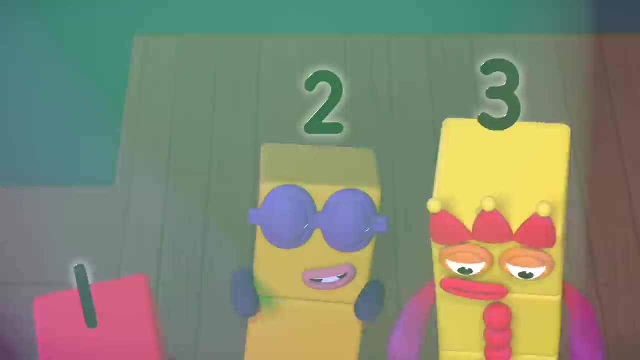 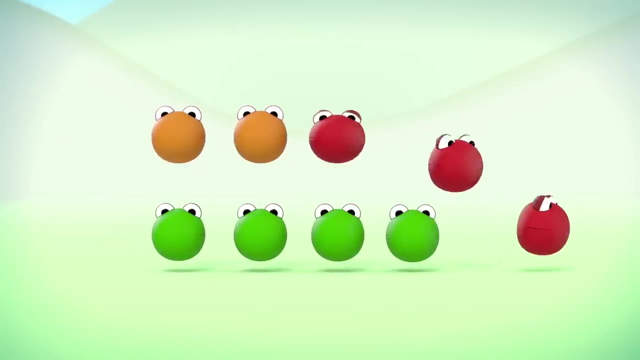 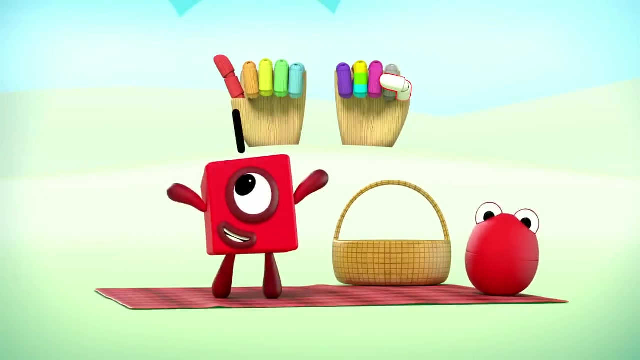 I'm the number for none, When there's nothing there to count now is the amount You've got: zero Number Blobs, One, two, three, four. One number blob and me Counting everything. we see Sharing a bun sitting in the sun. 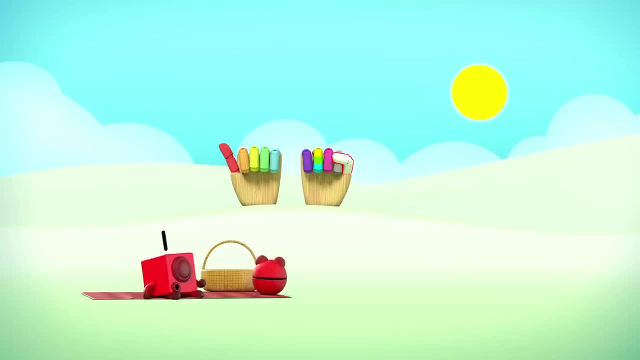 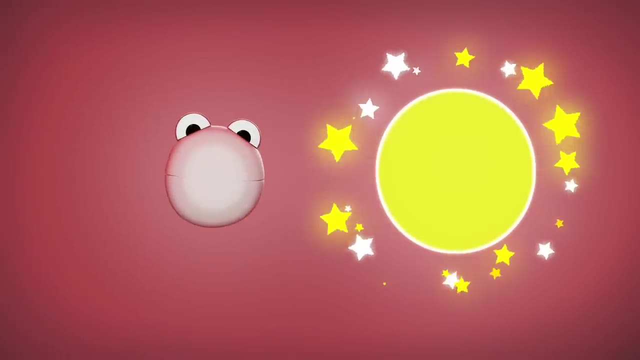 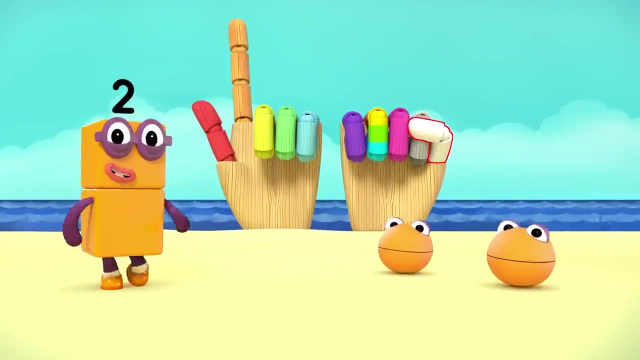 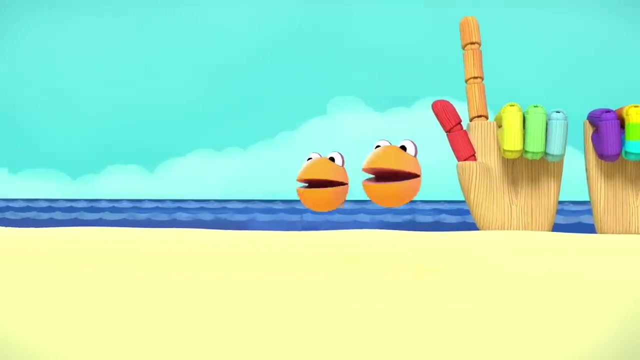 Whistling a happy melody, One number blob and me. One One bun One One sun. One number blob And me. Two number blobs and me Counting everything we see Taking off our shoes, Looking for the clothes. Whistling a happy melody: Two number blobs and me. 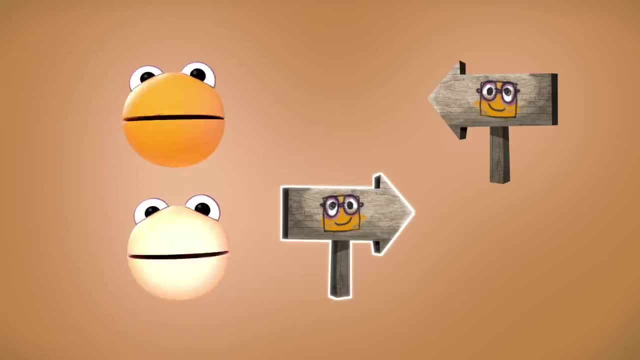 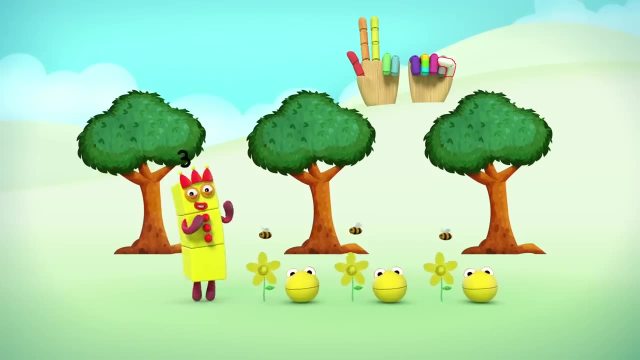 One, two, two shoes. One, two, two clothes, Two number blobs and me Counting everything we see Hiding in the trees, Buzzing with the bees Whistling, a happy melody. Three number blobs and me: One, two, three, three trees. 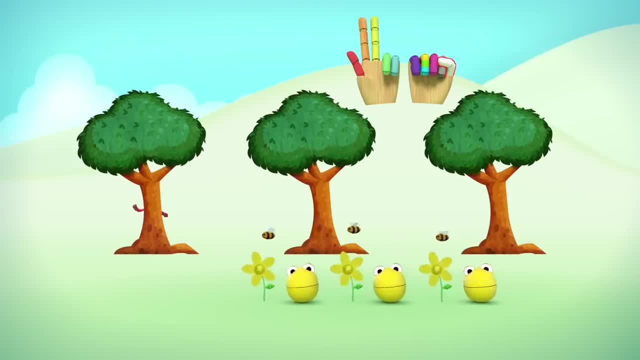 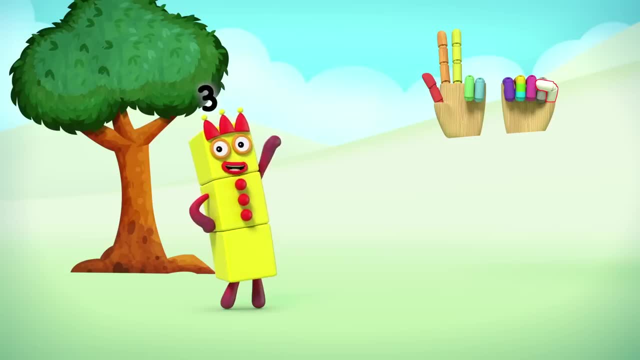 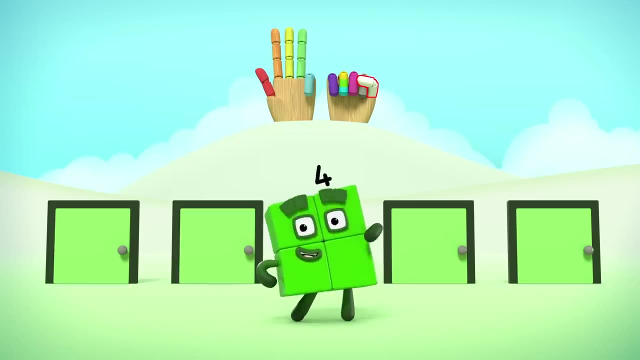 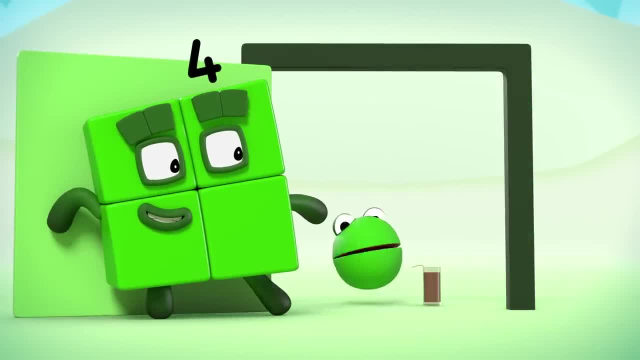 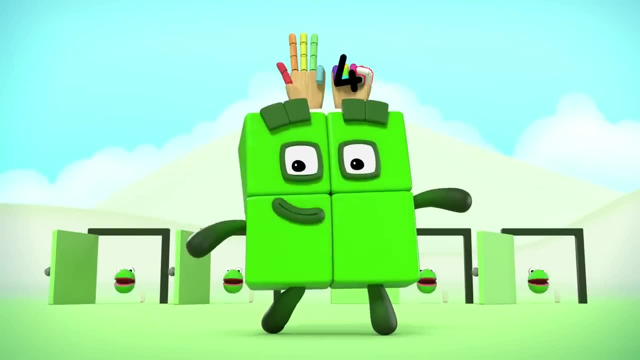 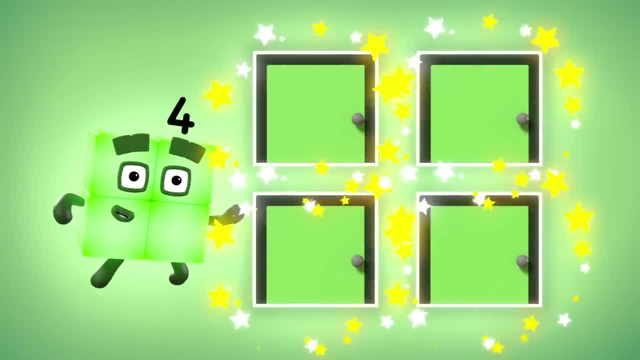 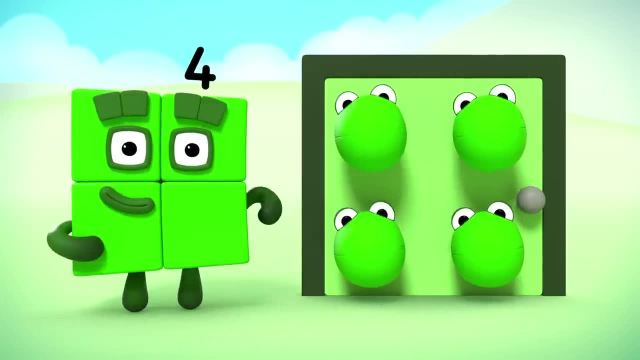 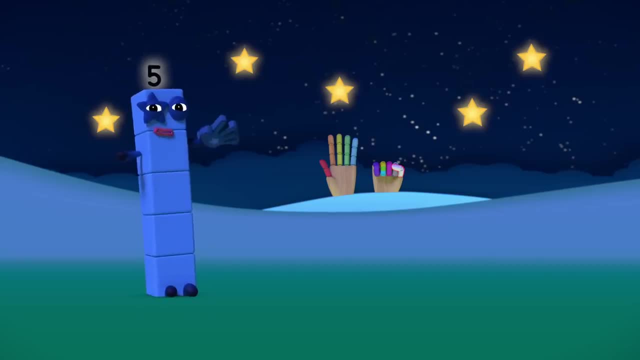 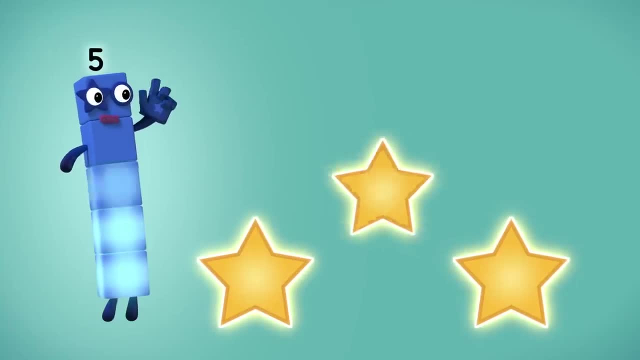 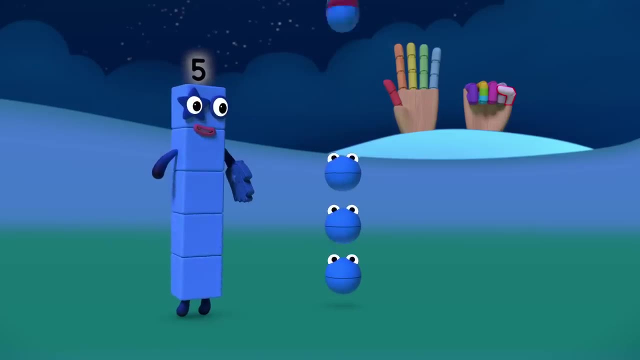 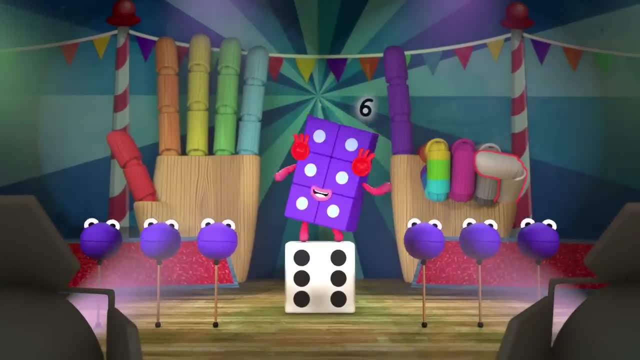 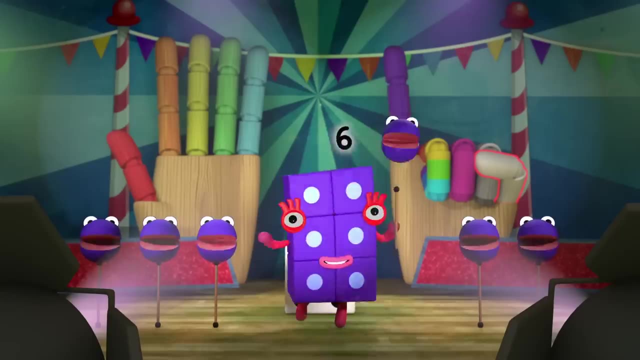 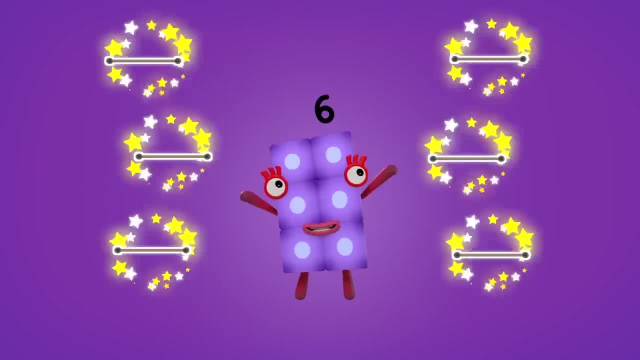 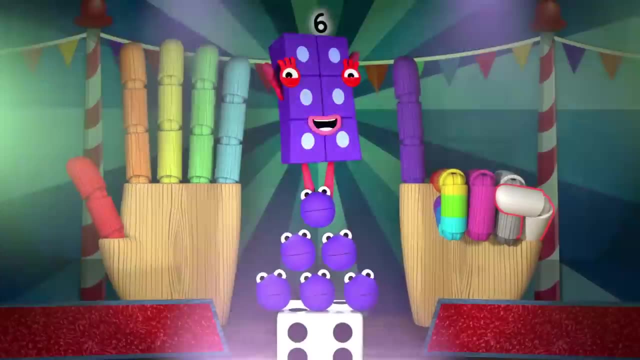 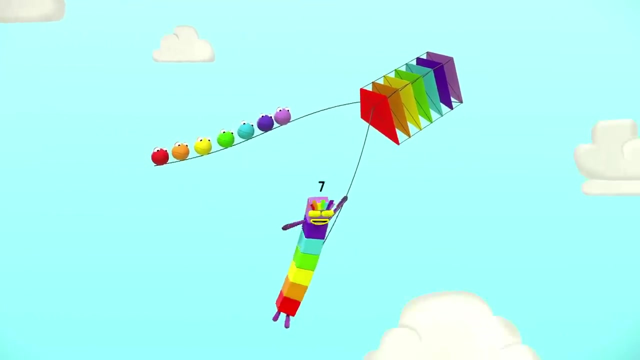 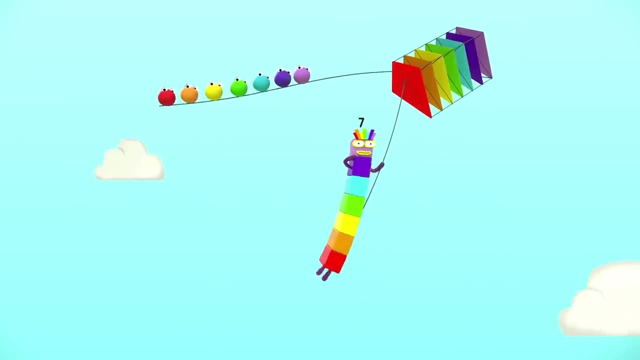 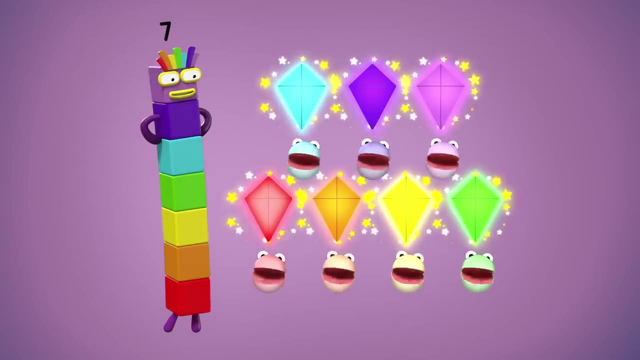 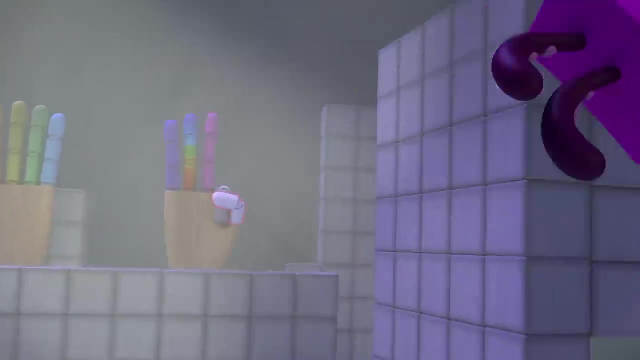 Turning on the lights: rainbow lights, Seven number blobs And me. One, two, three, four, five, six, seven, Seven kites: One, two, three, four, five, six, seven, Seven lights. seven number blobs And me. Eight number blobs and me. 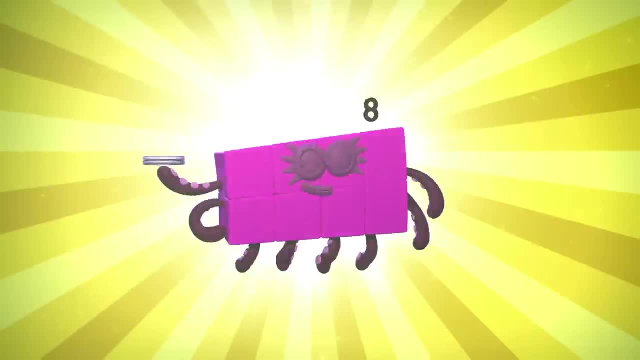 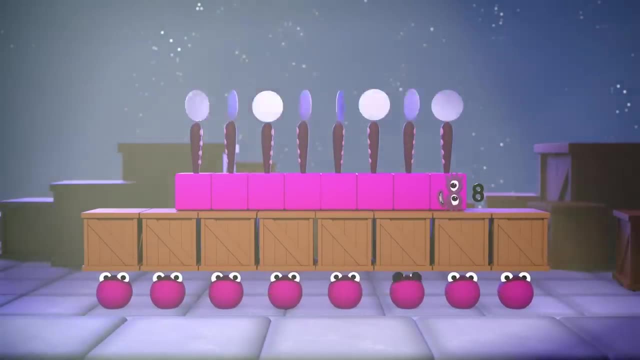 Counting everything we see, Spinning all the plates Off the block, spin, Lifting all the plates, Number blobs, lift Eight number blobs And me: One, two, three, four, five, six, seven, eight. Eight plates: One, two, three, four, five, six, seven, eight. 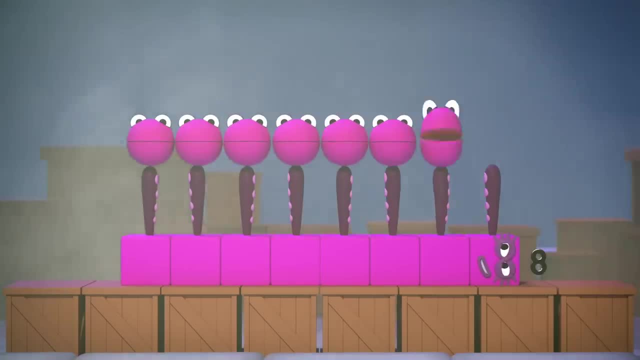 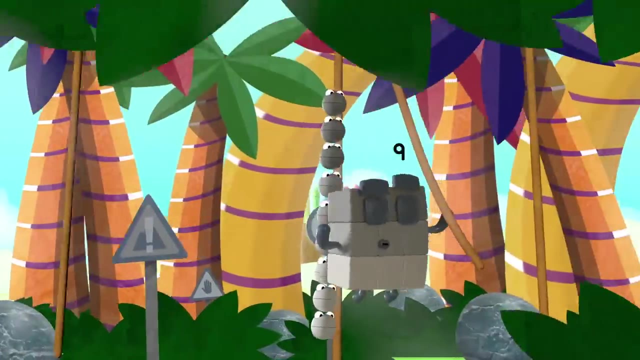 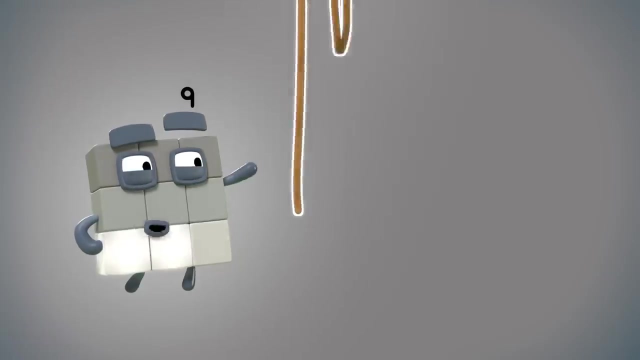 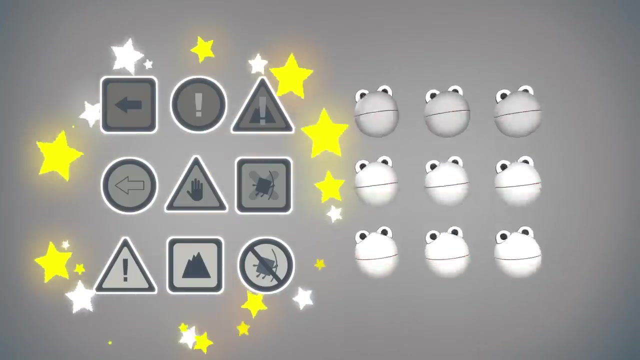 Eight plates, Eight number blobs And me, Nine number blobs and me Counting everything we see Swinging through the vines, Ignoring all the signs. Hey, One, two, three, four, five, six, seven. Eight栆. One, two, three, four, five, six, seven. 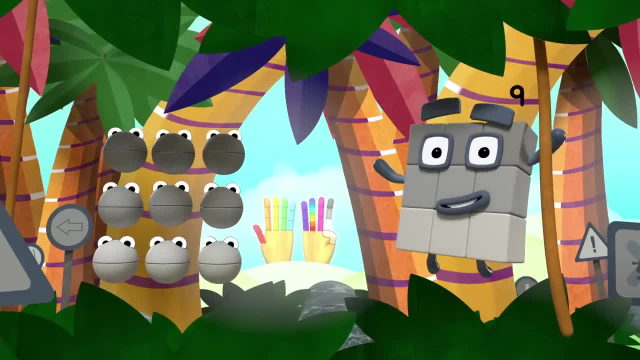 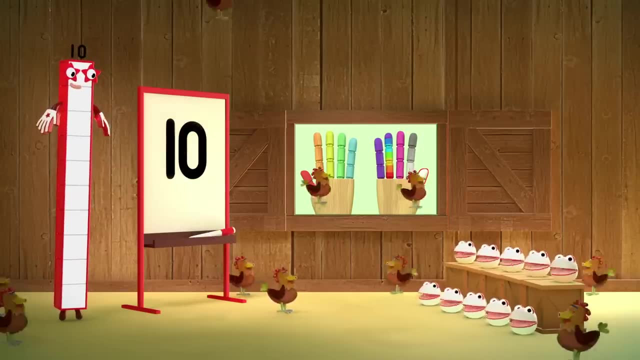 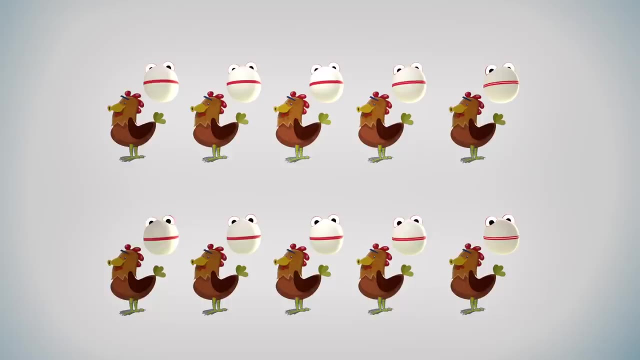 Eight blancs, Nine signs, Nine number blobs And me Counting everything. we see Ten number blobs and me Counting everything. we see 10 number blobs and me Counting everything. we see 10 number blobs. Seven, eight, nine, ten, Ten hens, ten number boats. 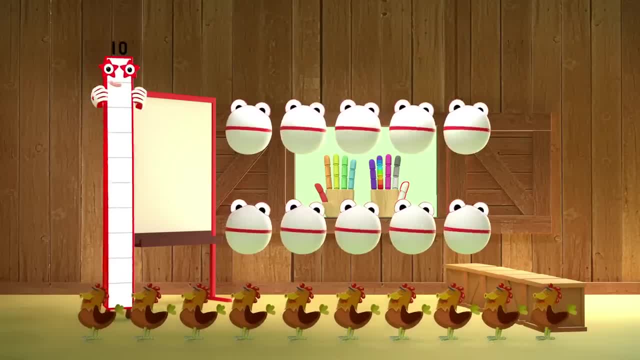 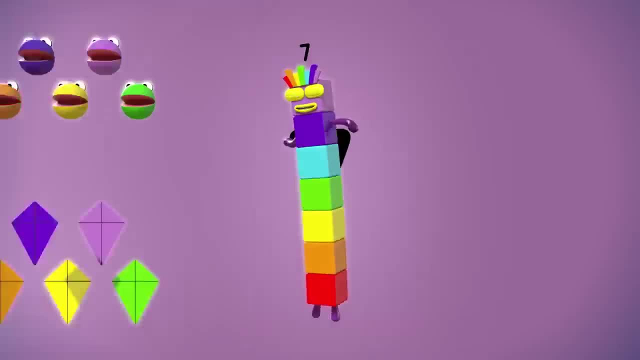 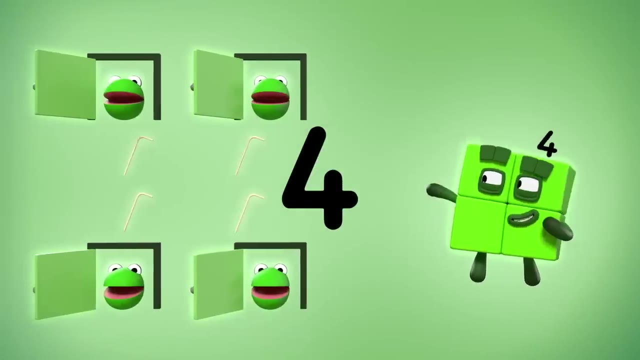 And me. Ten colored pens, ten little hens, Nine swinging binds, nine warning signs, Eight spinning plates, eight heavy crates, Seven floating kites, seven rainbow lights, Six wooden sticks, six clever tricks, Five shooting stars, five motor cars, Four open doors, four bendy stores. 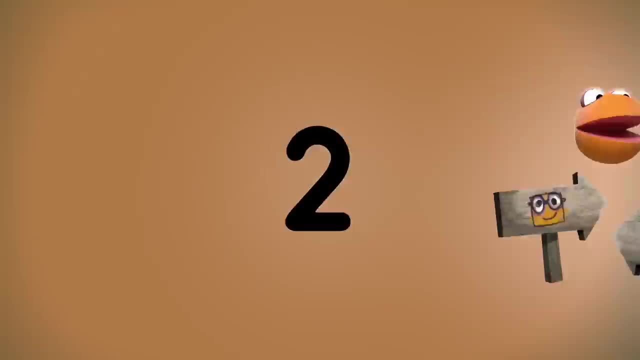 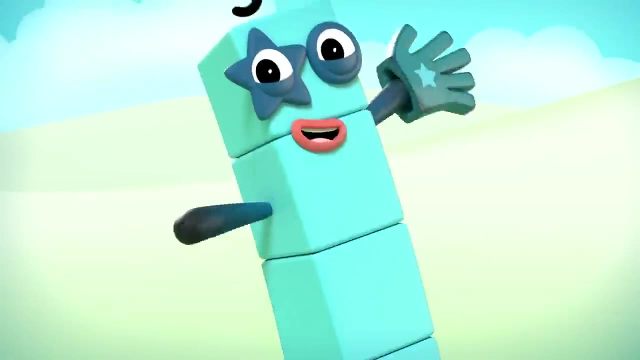 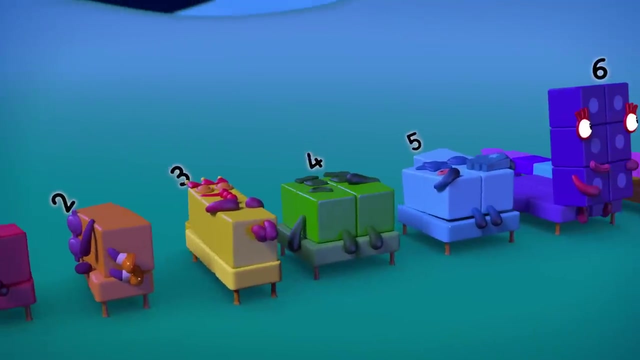 Three leafy trees, three moldy leaves, Two dowsing shoes, two vital clues, One sticky bun, one golden song Time One, two, three, four, five, six, seven, eight, nine, Ten. If you're sitting comfortably then I'll begin. 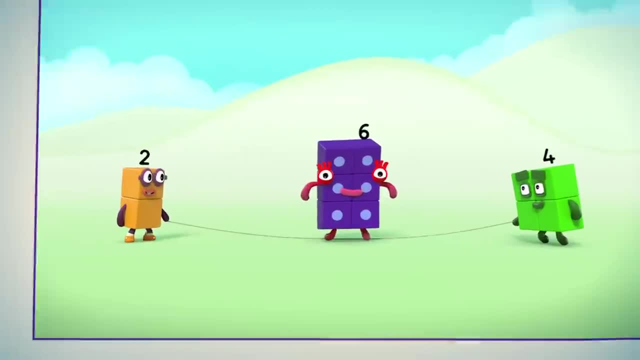 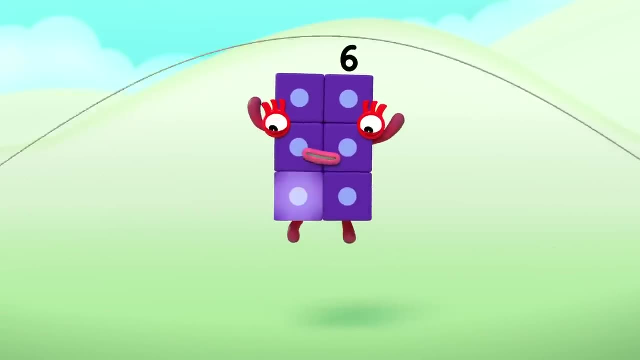 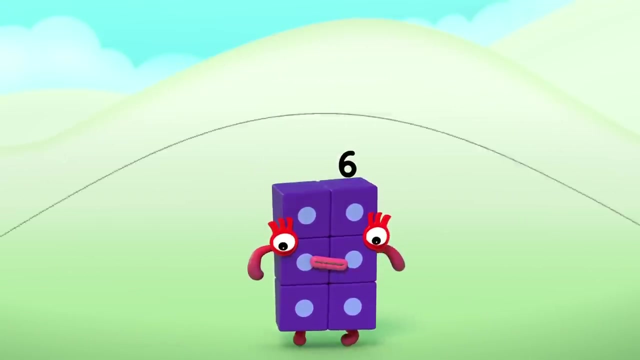 Chapter Six: Skips and Tricks. I am six in the mix Time for rhymes and skips and tricks. Count my blocks: One, two, three, four, five, six And ten. I'm six. you see This up here means six as well, And I love games, as you can tell. 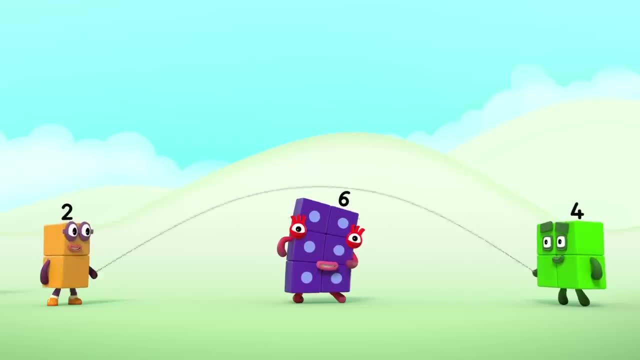 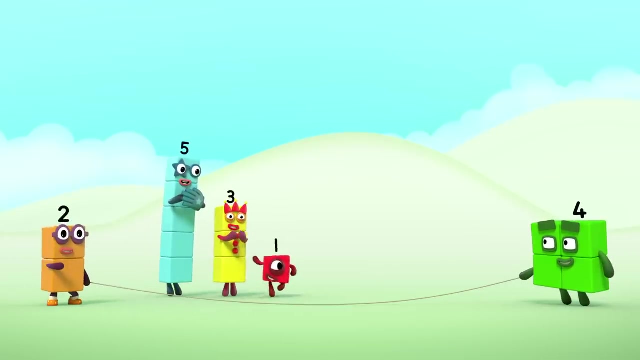 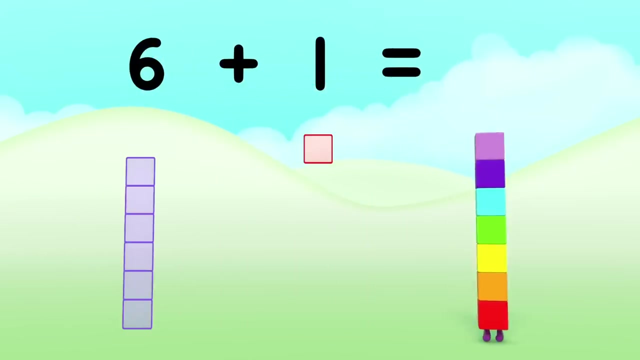 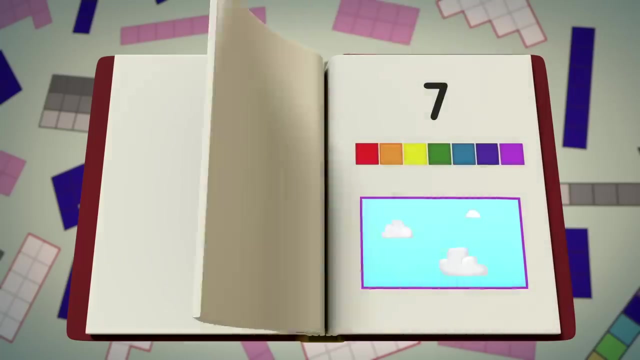 Let's roll. Six, Six tricks coming up quick: One trick, two tricks, Three tricks, four tricks, Five tricks, six tricks, Yay, Yay, Can I join in? Oh, six plus one equals seven. I am seven and I feel lucky, Chapter Seven Falling on My Feet. 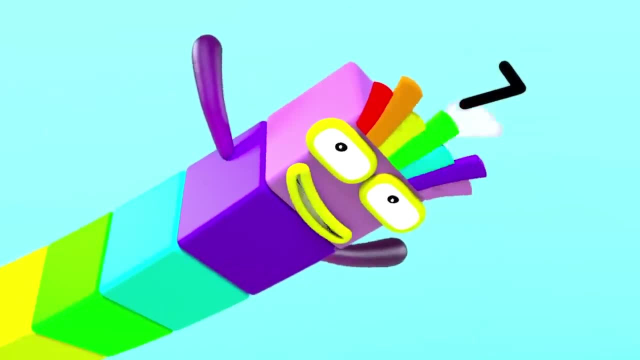 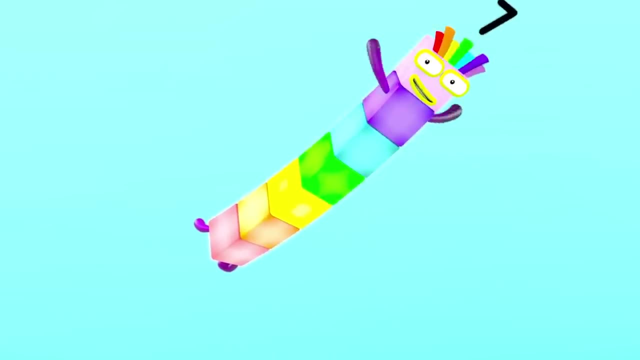 Fancy meeting you up here. That's lucky I'm seven. I've got one, two, three, four, five, six, seven, Seven blocks. Oh, how funny. That cloud is red And here comes orange, yellow, green, Blue, indigo, violet. 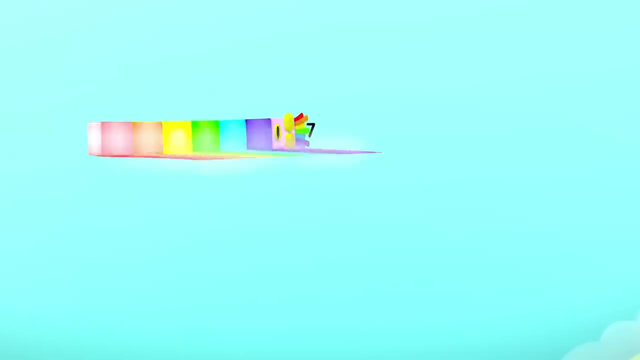 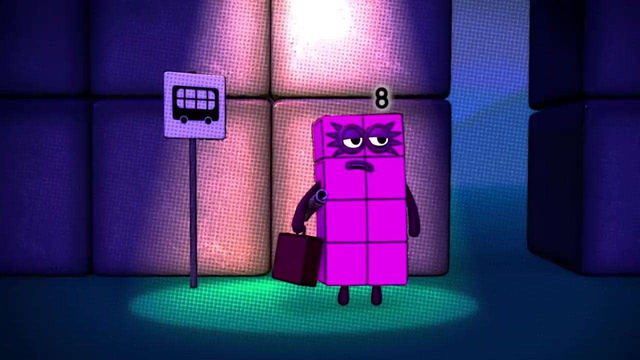 Watch this: Whee, Hoo-hoo-hoo, Oh, Look out. Seven plus one equals Eight. I am eight. This is great. Chapter Eight: The Secret Story of Octoblock. Once, eight was just an ordinary, mild-mannered number, with eight blocks. 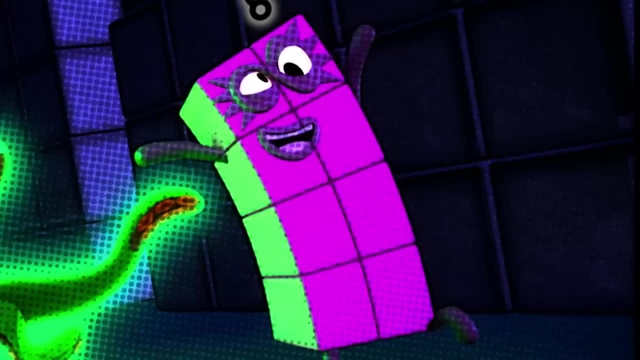 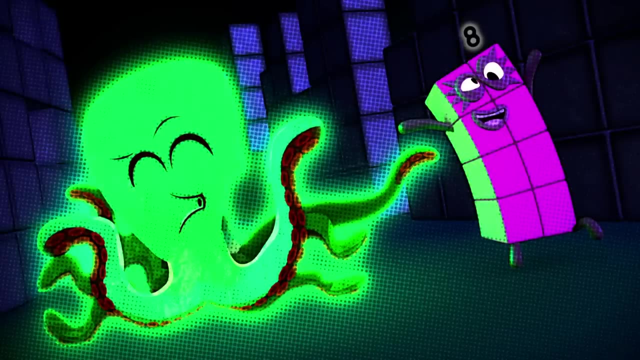 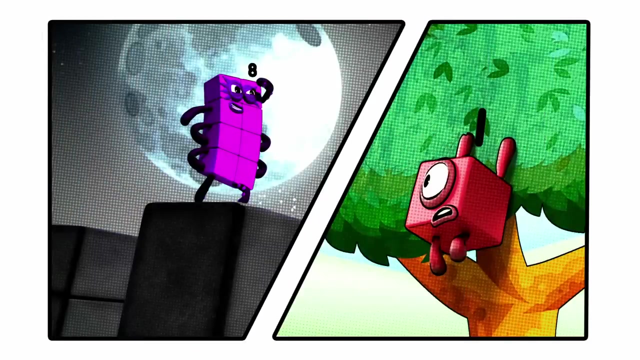 And that means eight as well. But one day eight was tickled by a radioactive octopus Ha-ha-ha-ha. It gave me special powers, So if anyone needs help, they can call on Octoblock To the rescue. 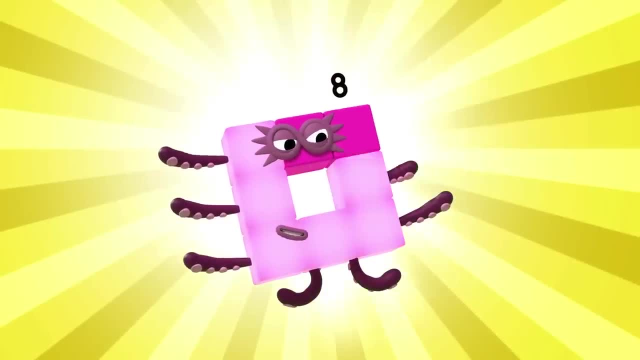 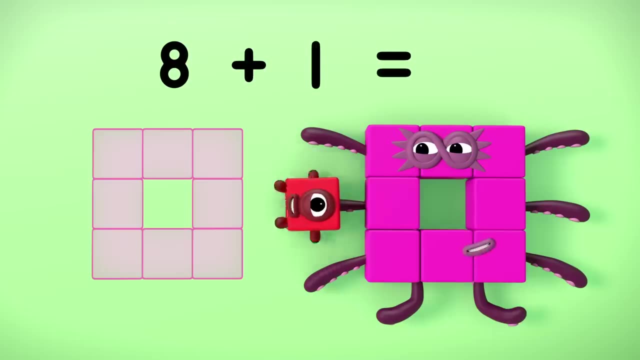 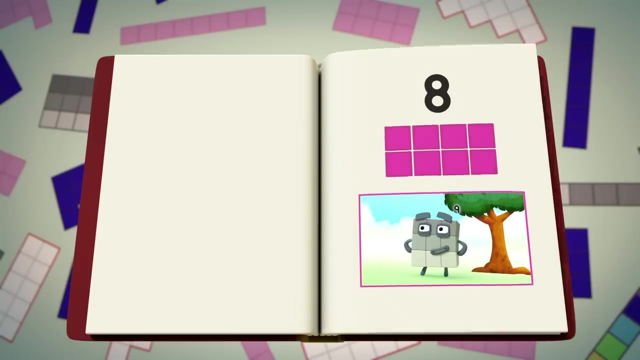 Octoblock. catch One, two, three, four, five, six, seven, eight. Catch. Eight Plus one equals Nine. I am nine and I feel fine. Chapter Nine: Sneeze, a jolly good fellow. 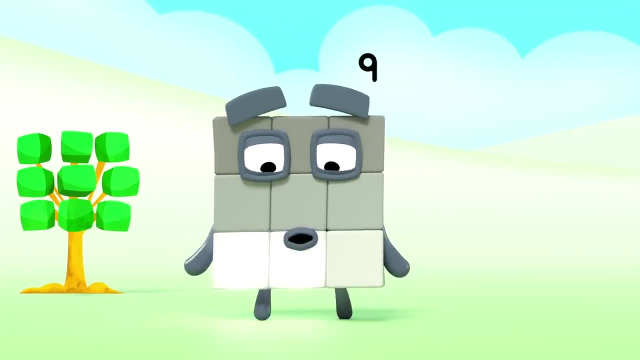 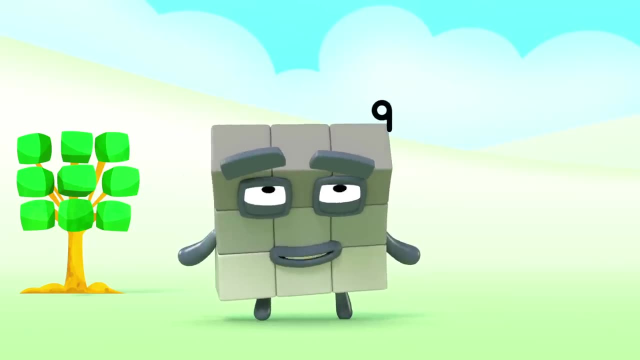 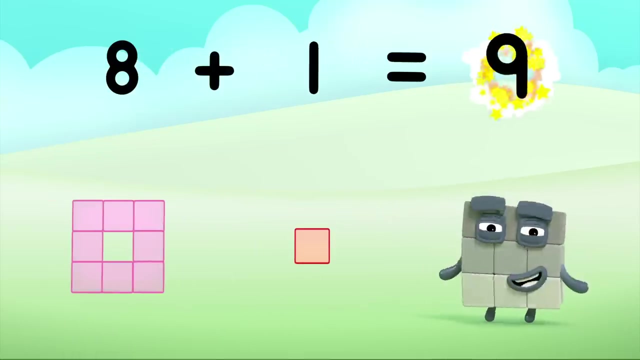 Hello, I am nine. I am one, two, three, four, five, six, seven, eight, nine, Nine blocks. Thank you, Do you need some help? nine Is anything wrong? Eight Plus one equals Nine. 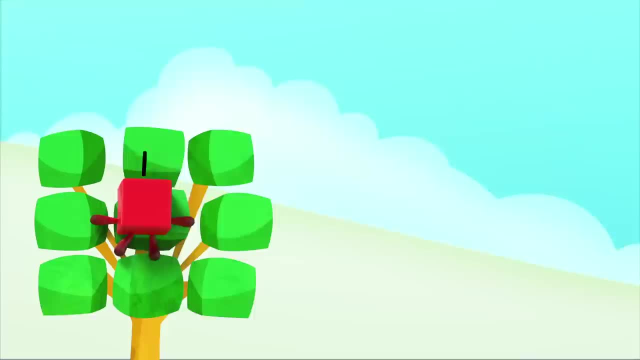 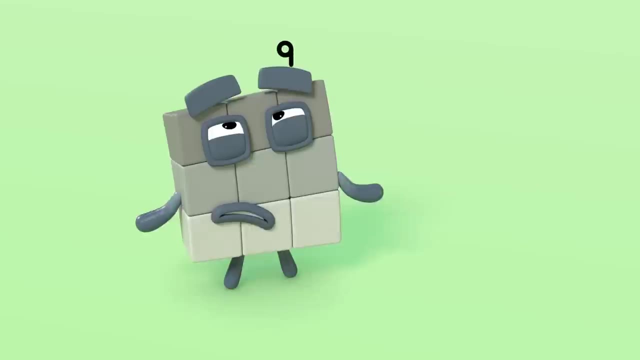 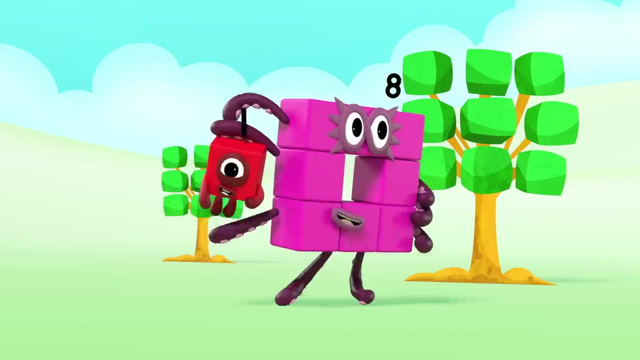 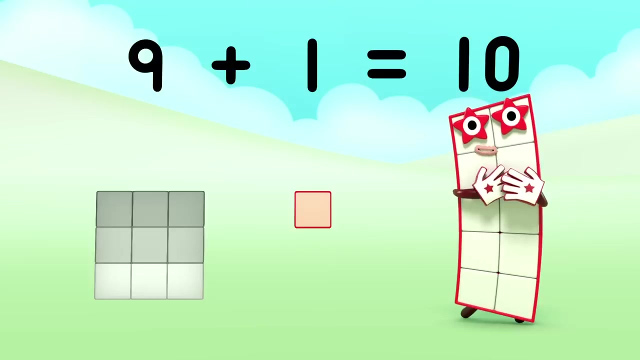 Nine Minus one Equals eight. Eight Plus one Equals nine. Ah-choo, Ah-choo, Ah-choo, Ah-choo. See how you like it. Nine Plus one equals ten. Say it again. 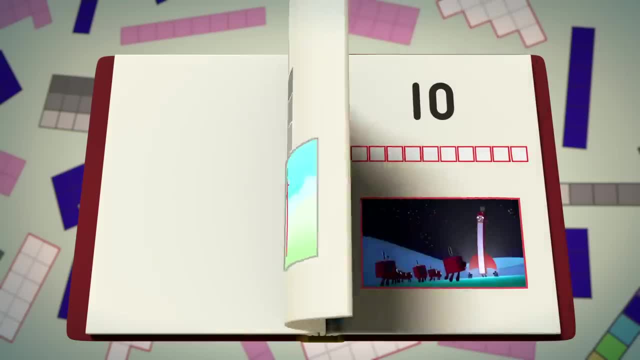 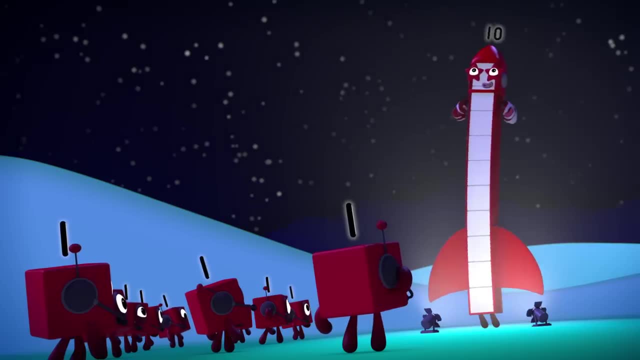 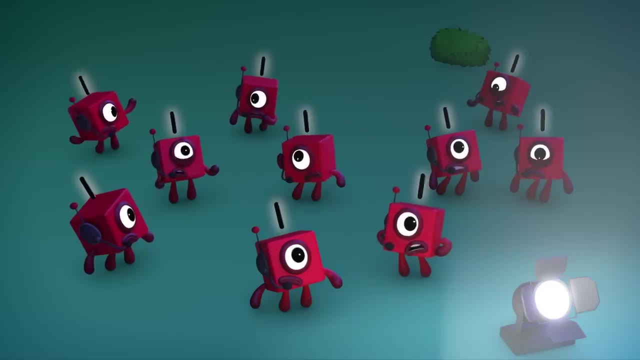 I am ten, Chapter ten, the space race. Ten here, ready for takeoff, Commencing countdown of my ten blocks: Ten, nine, eight, Oh, dear, Calm down everyone. We'll just use the backup rocket. 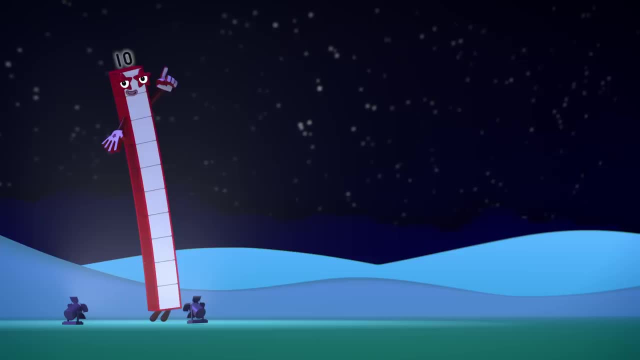 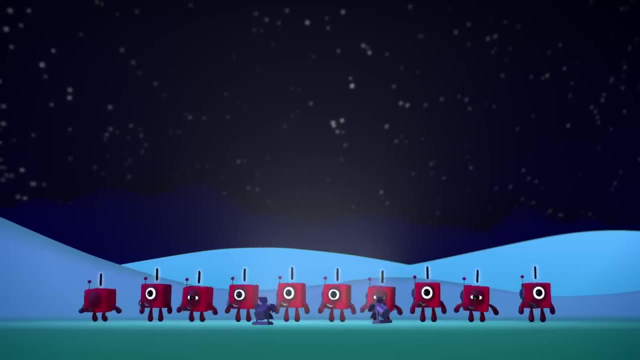 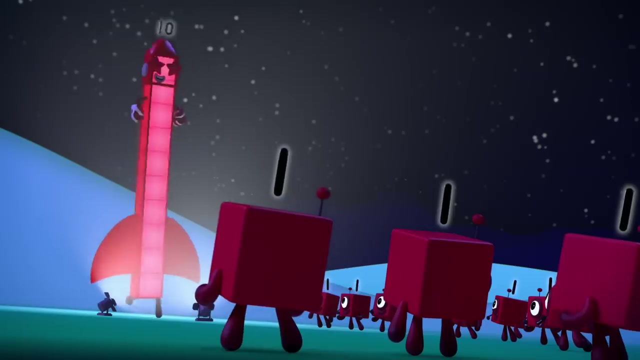 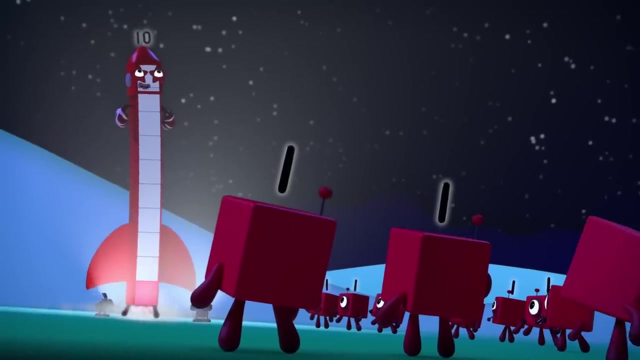 I'm one, ten, which means I'm also ten ones. So it's one small step for ten, One giant leap for ten ones. Hooray, Ten, nine, eight, seven, six, five, four, three, two, one. 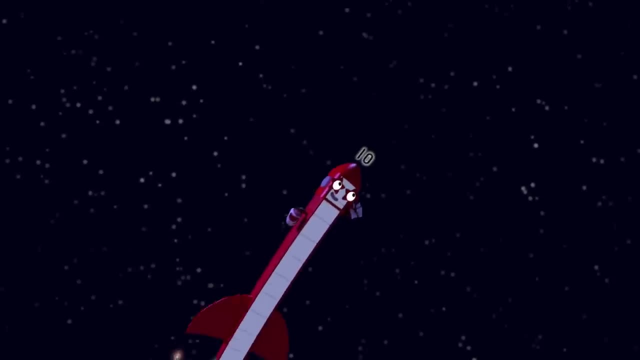 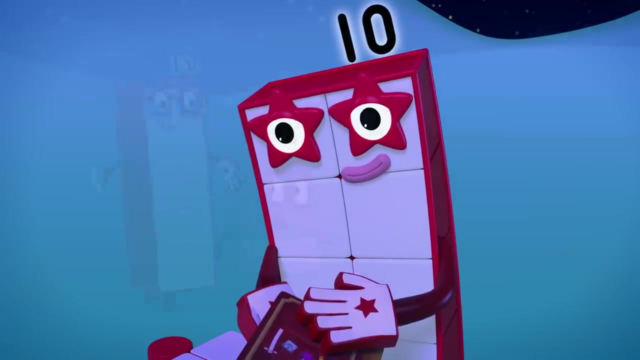 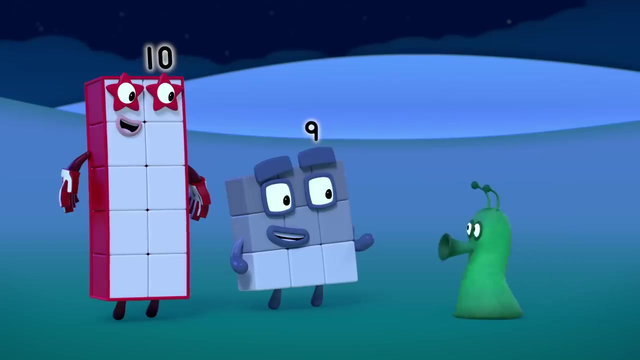 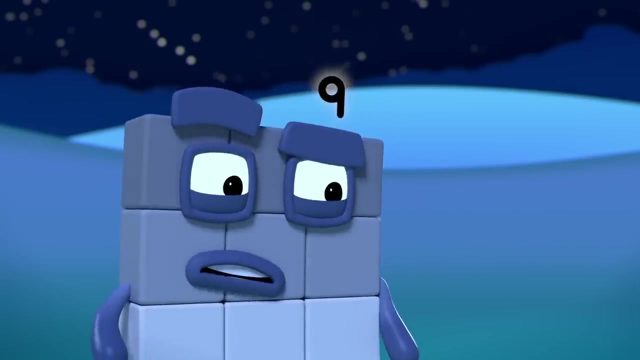 Blast off, Yay, Ah. Now there's something you don't see every day: An alien Up up. Ah, Whoa Is that where you live? Up, up, Up up. Don't worry, fellow space cadet. 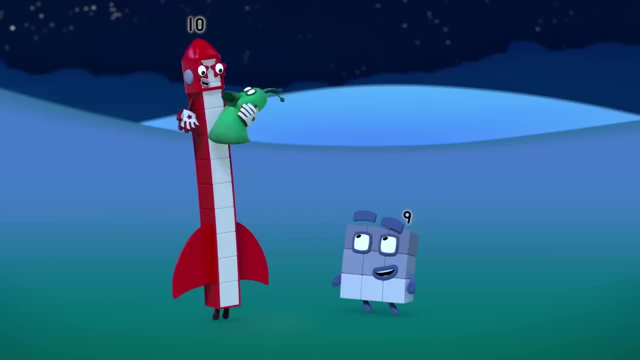 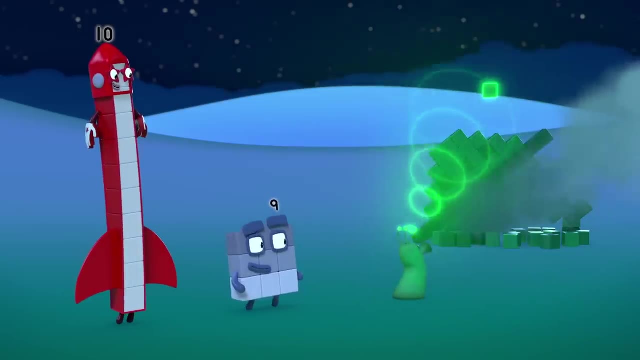 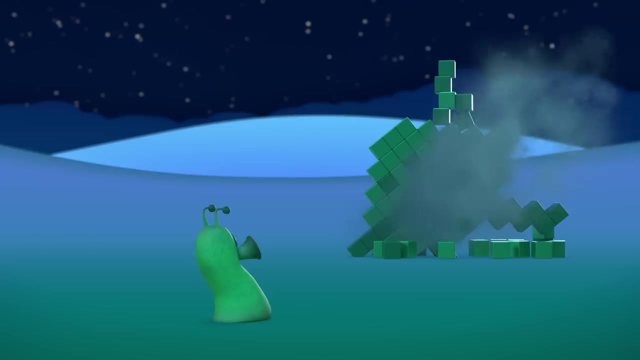 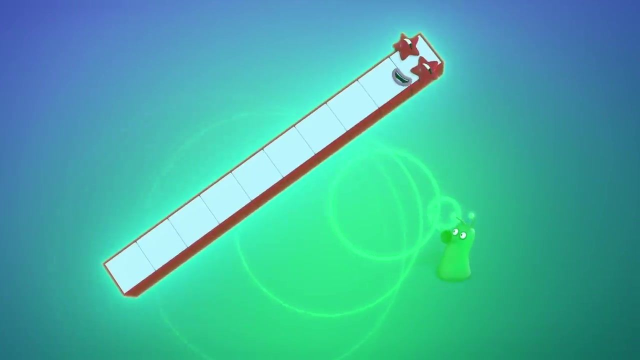 I can rocket you home. Hold on tight. Ten, nine, Eight, Oh, Ah. I think she's building a tower. Hmm, Up, Oh um. I think you'll need more blocks than that. Whoa Stop. 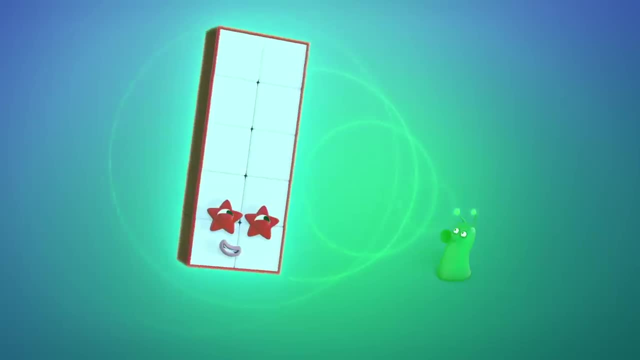 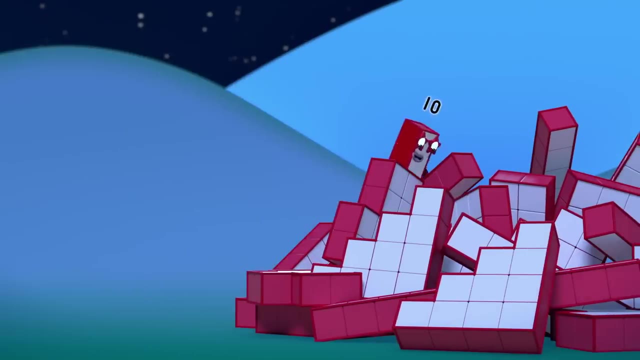 That tickles. Oh Oh, Let's build a tower. Ooh, Oh, Oh, Oh, oh, Oh, oh, oh, All right, ah, All right, I've got the right to get off the rope, All right. 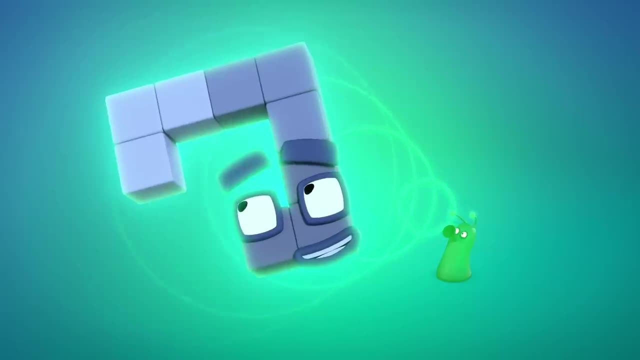 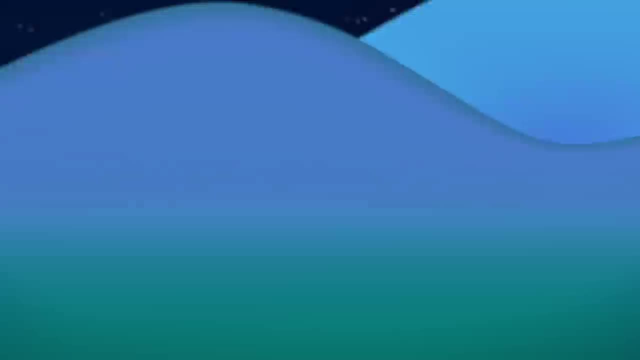 Ooh, Oh, whoops, What a surprise. Ooh, Ooh, Oh, ooh, Oh, oh, oh, Ah, Ooh, Whew, Ooh Ooh, That's, it, Ooh Ah. 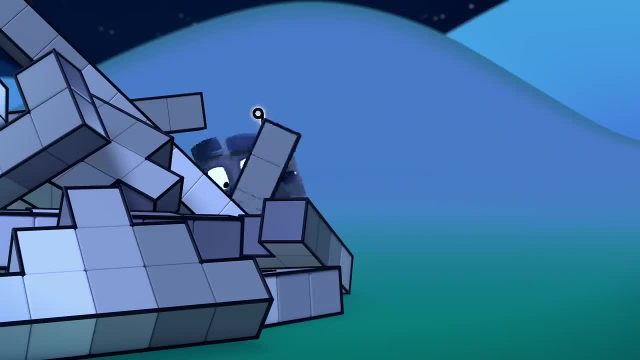 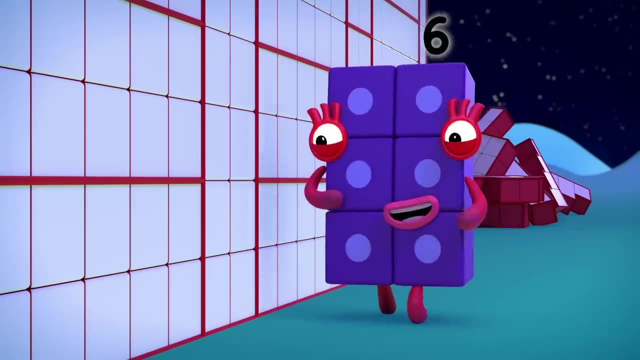 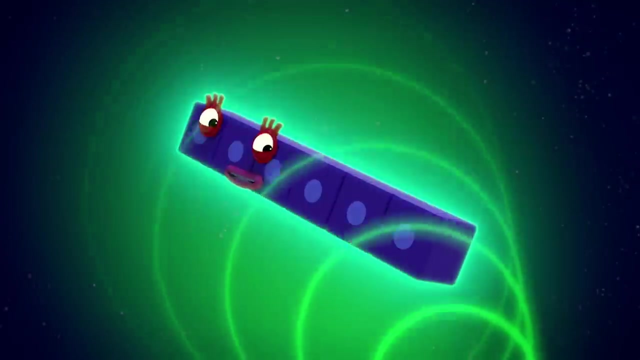 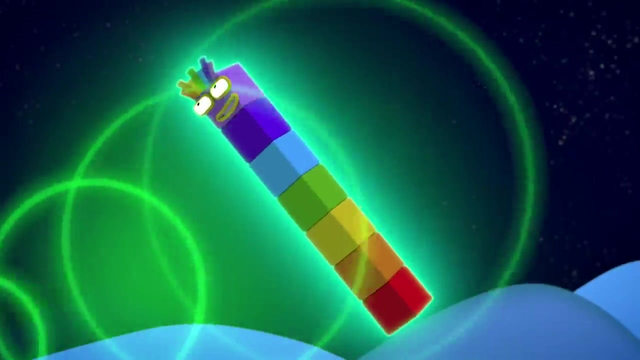 Hey say, can I play One, two, three, four, five, six. Please make me some building bricks. Ooh great Ooh, lucky me Ooh, Ooh-hoo. Hmm, I think I'm going to have to make some building bricks. 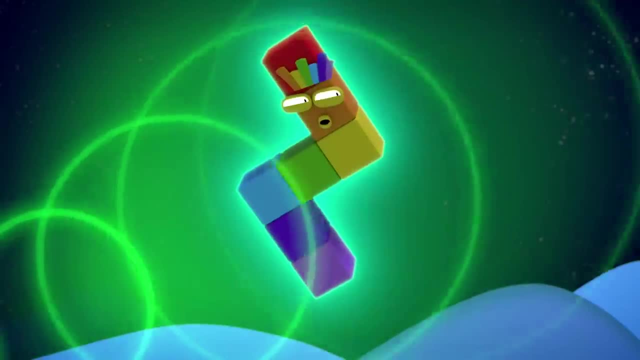 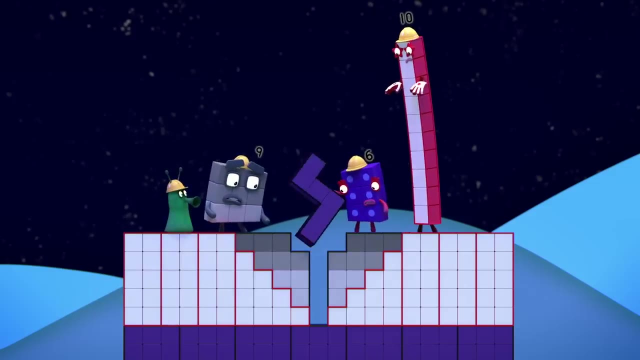 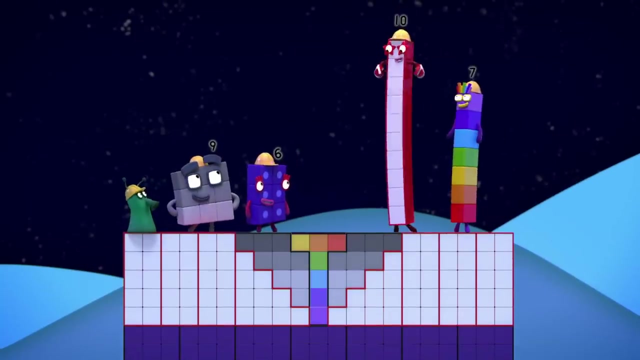 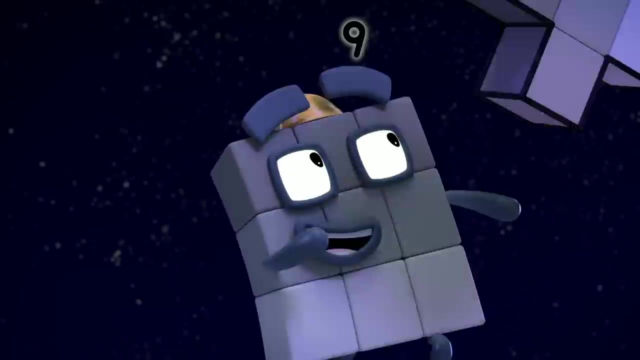 Ooh, I'm going to have to make some building bricks. Ooh, This doesn't fit, Or this Or that, Try this: Yay, Beginner's luck: Number blocks. let's get building. Ooh, That's my favourite. 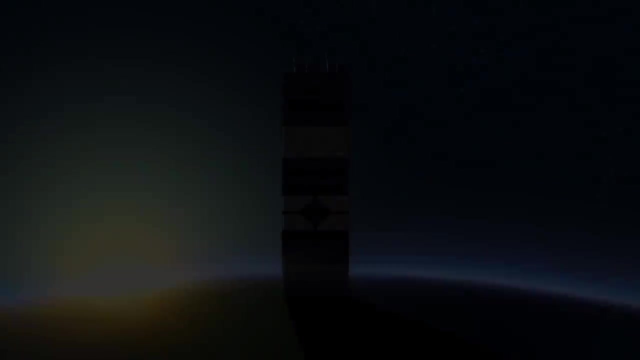 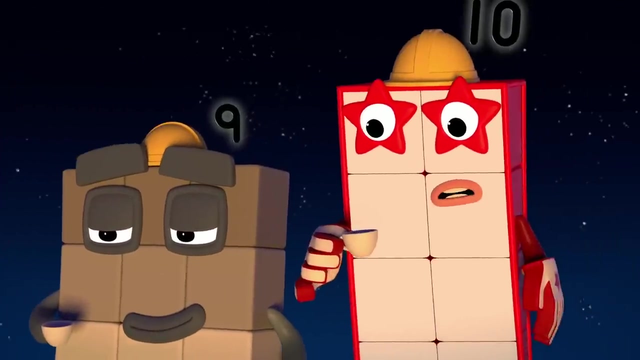 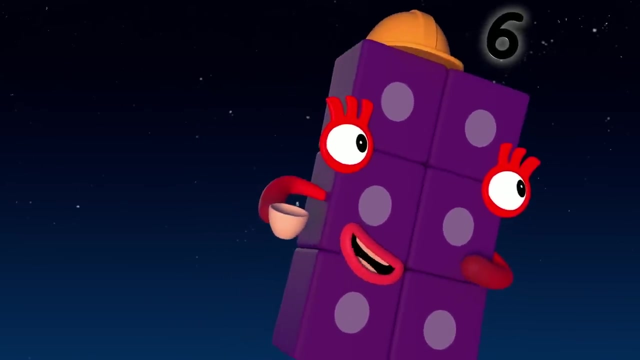 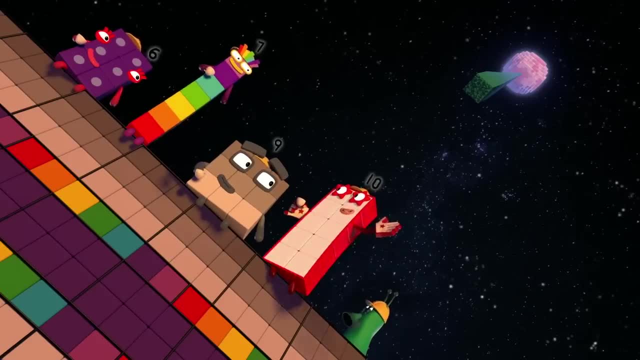 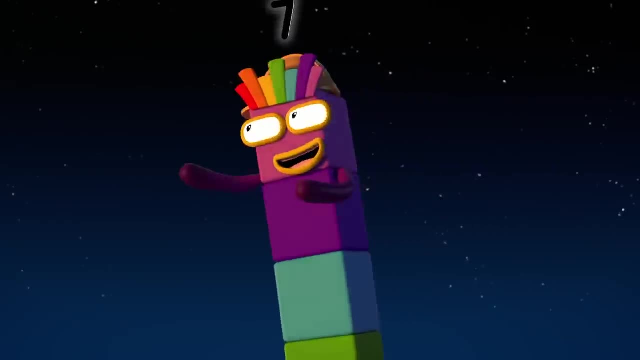 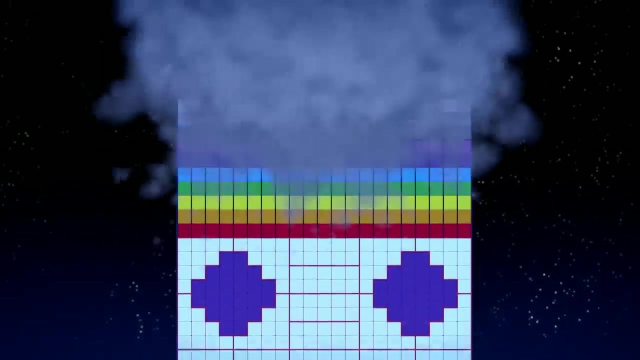 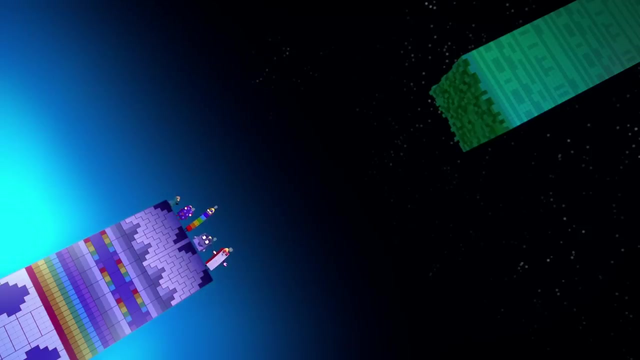 We can meet in the middle. Back to work, everyone, Huh, Ooh, Ooh, Ooh, Ooh, Ooh-hoo, Ooh, Oooh, Ooh, Ooh, Ooh, Ooh. 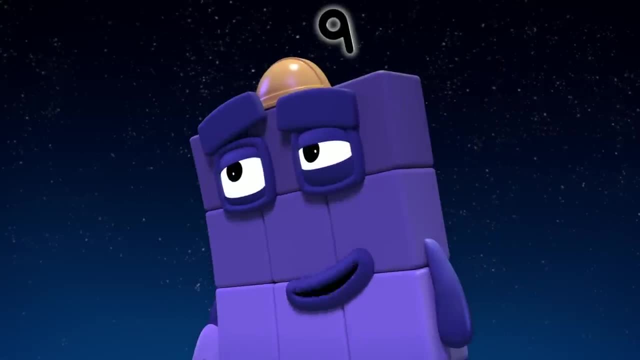 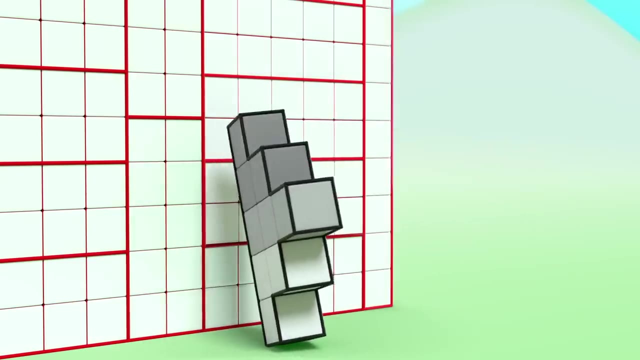 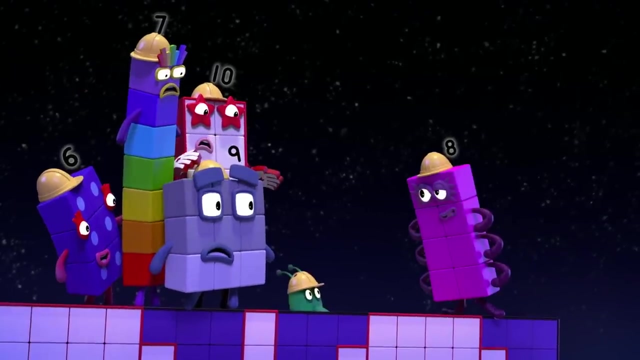 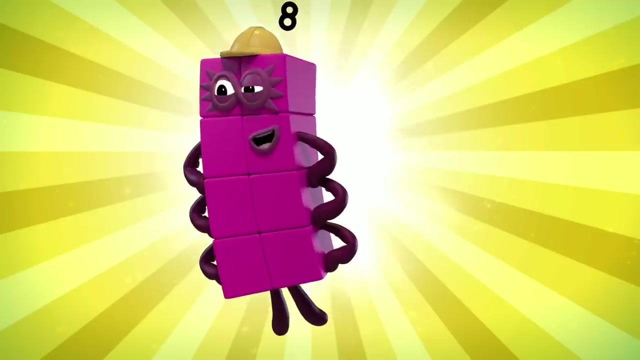 Ooh-hoo, Ooh, Ooh, Ooh-hoo, Ooh-hoo, Aw. Did somebody say help? Octoblock to the rescue, Octoblock, build One, two, three, four, five, six, seven, eight build. 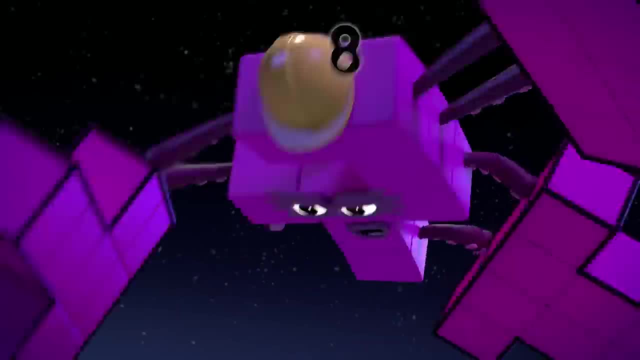 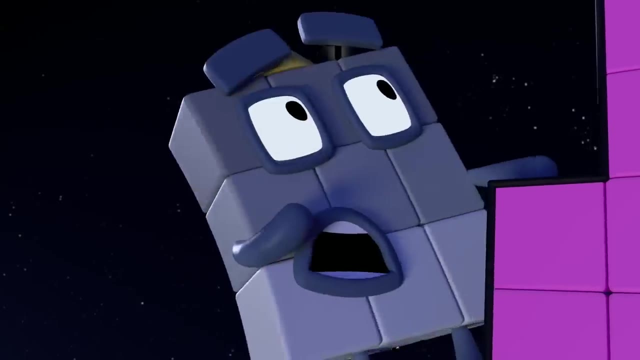 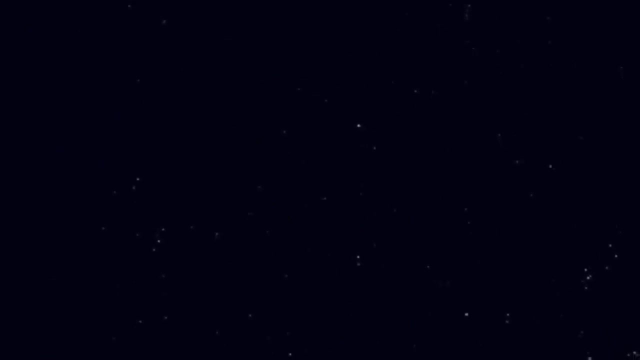 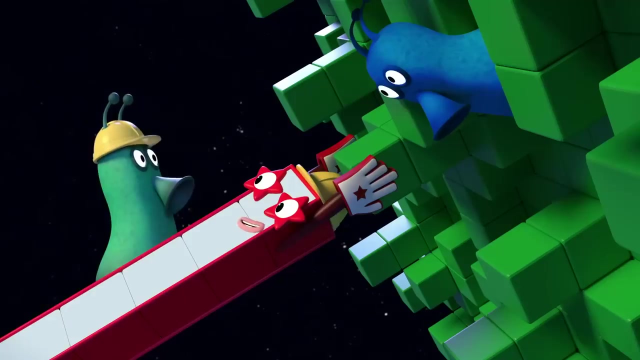 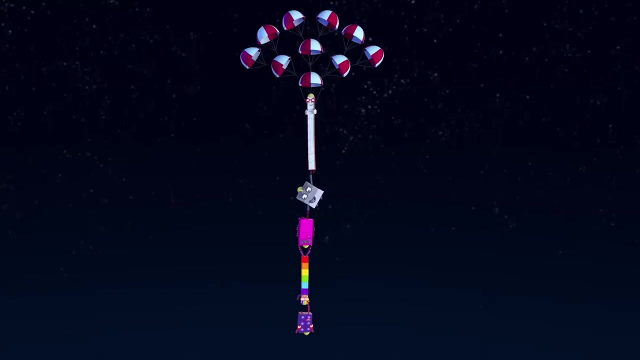 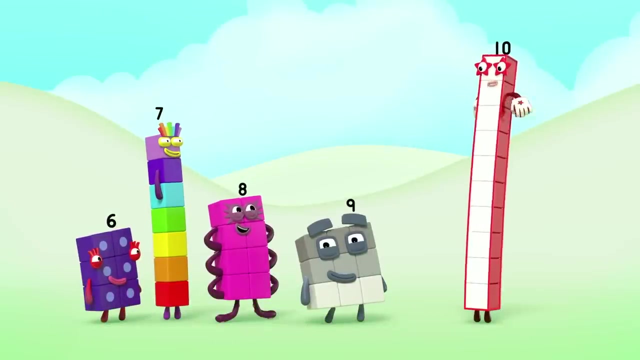 Go Octoblock Nearly there, Timber You go up, we'll go down. Goodbye, fellow space cadet. Yay, Wow, Well done crew, A successful mission. Well, my turn, My turn Mostly successful. 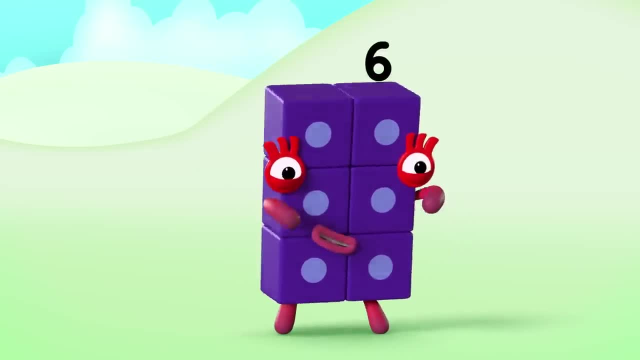 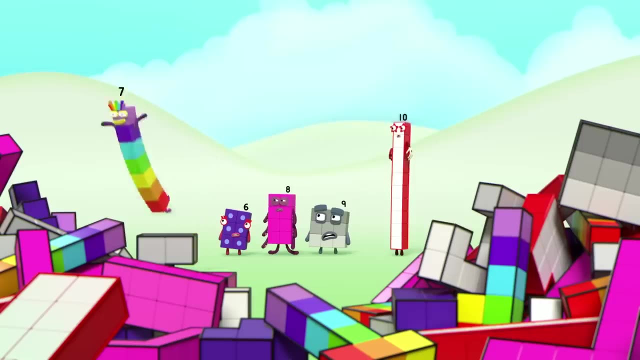 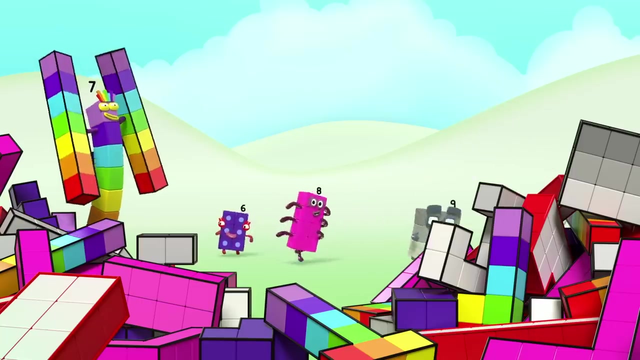 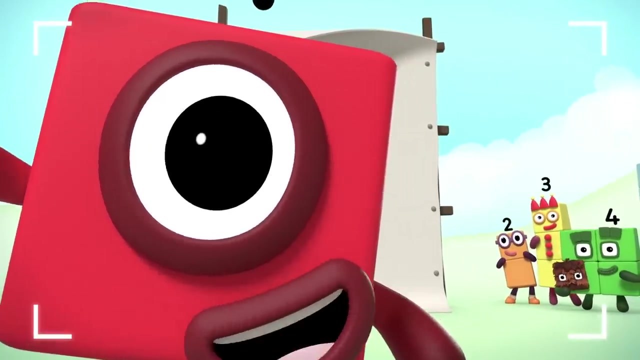 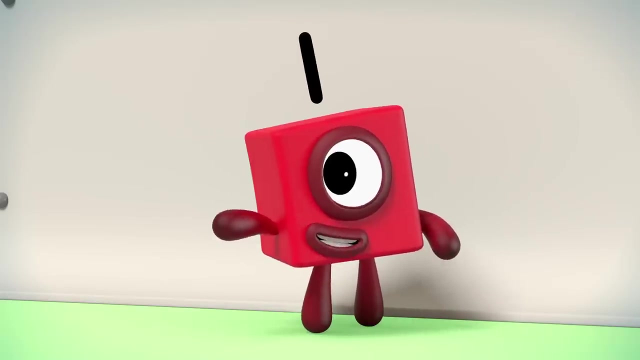 We helped our friend get back to space, but now our tower's all over the place. Oh, that's lucky We get to build something else: A rocket, A house, A rainbow, All ready. Then it's your turn. Just say cheese, and the camera will take a picture. 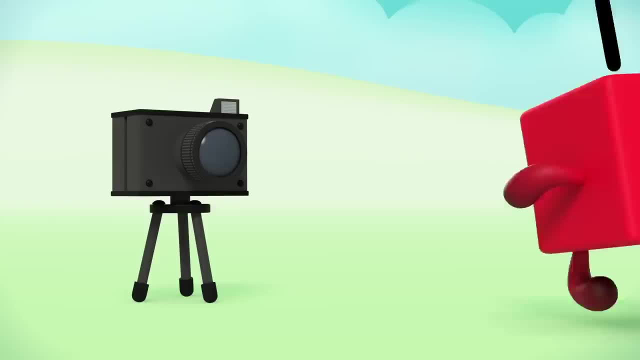 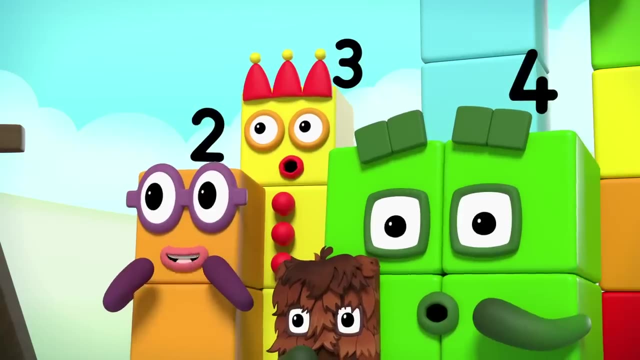 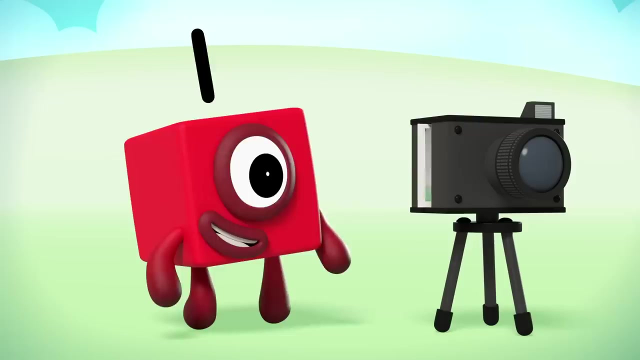 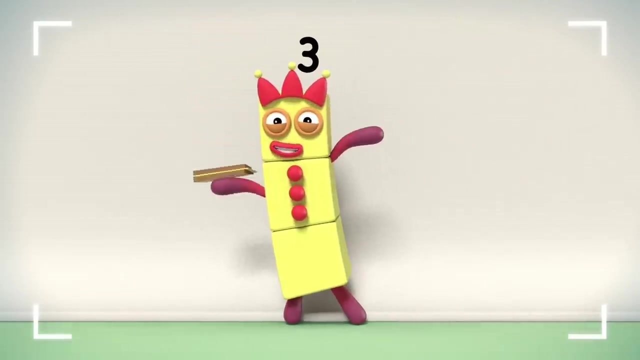 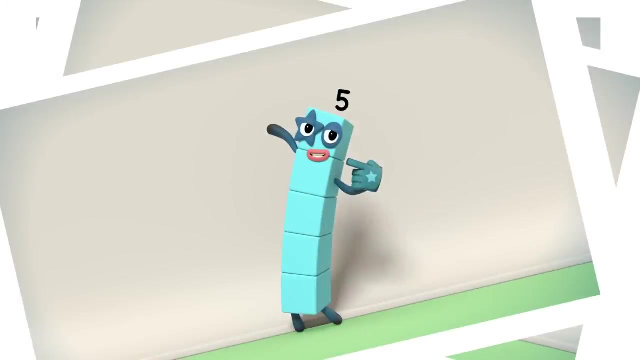 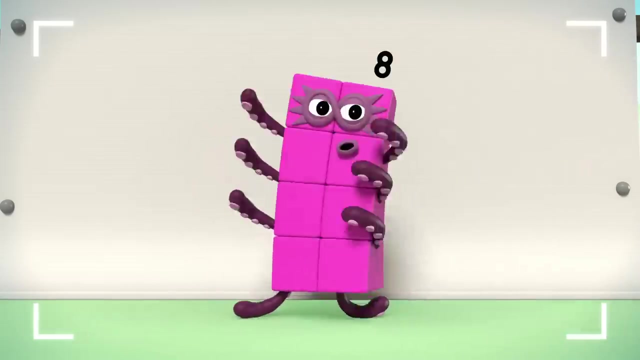 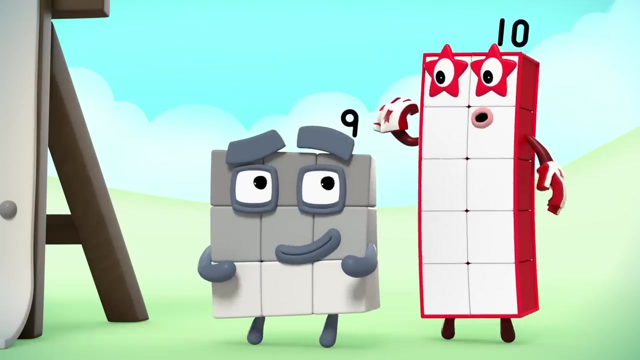 Like this Cheese, Then it pops out here. Cool, My turn. Cheese Bread, cheese bread, Cheese sandwich. Bitch, We have two chances. Cheese, This is life. Cheese, Cheese, Cheese, Three Cheese. 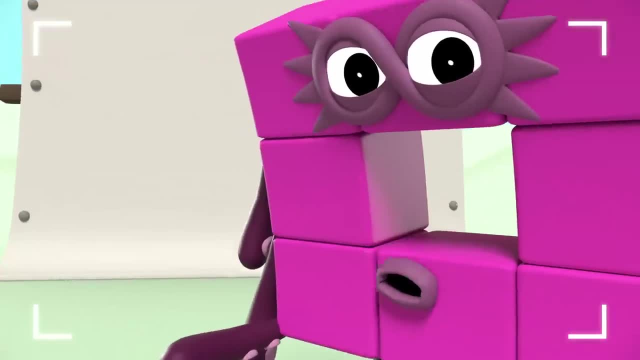 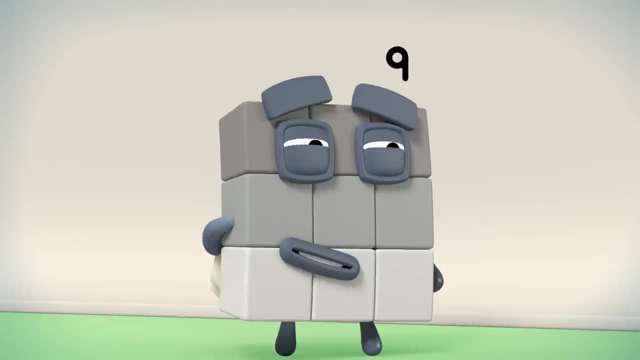 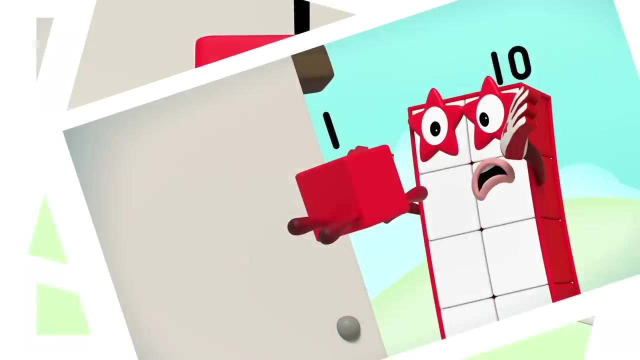 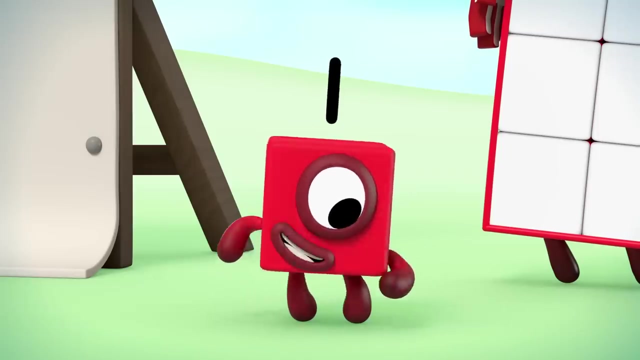 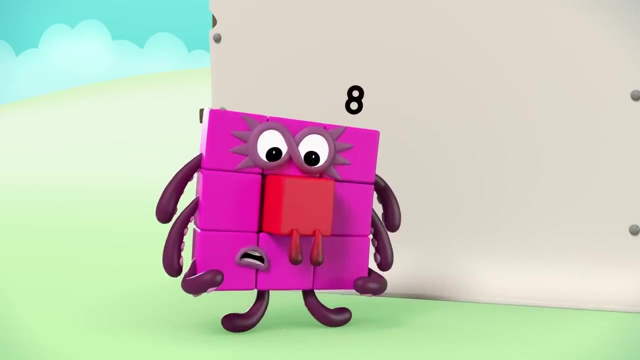 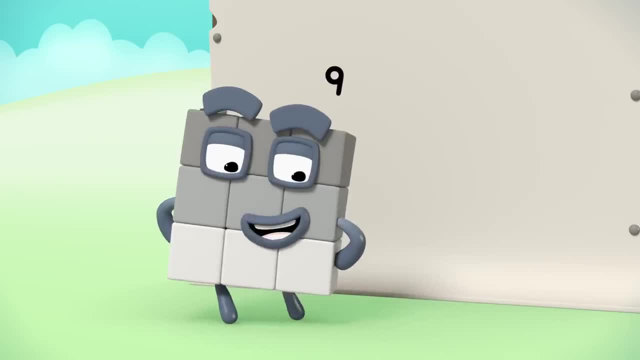 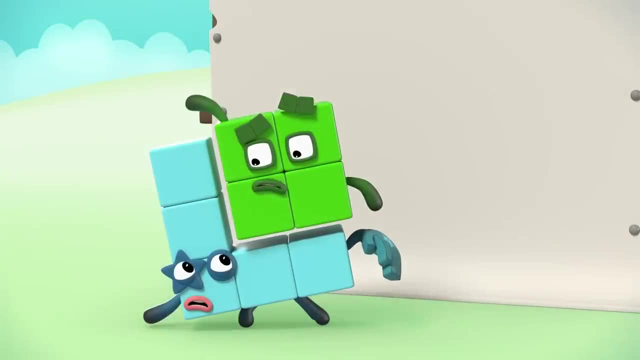 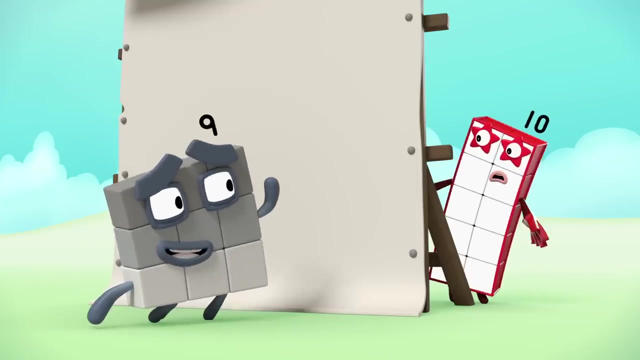 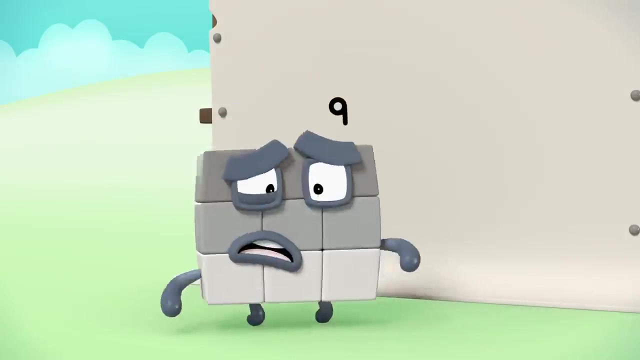 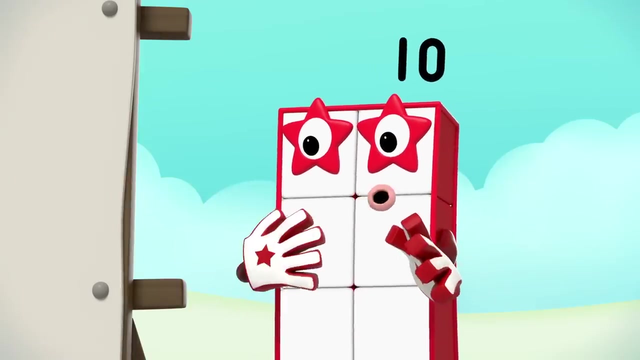 I'm cured. What Hang on? This isn't right. We've got the hiccups. Oh, It's okay. I think it's stopped. Oh, I've got to get rid of these hiccups. Oh, I know how to cure hiccups. 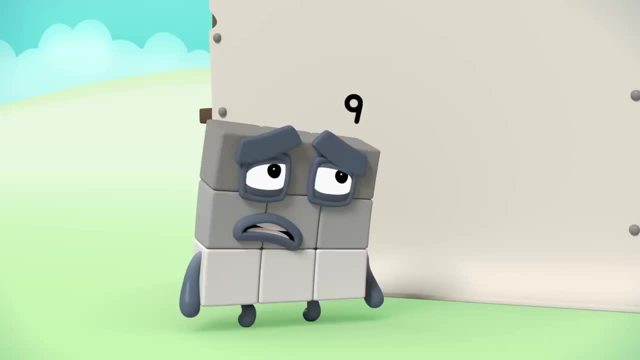 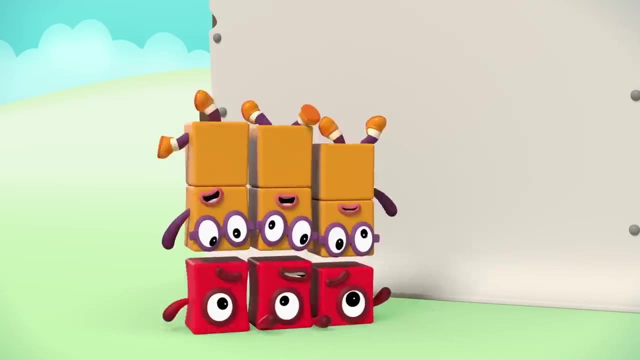 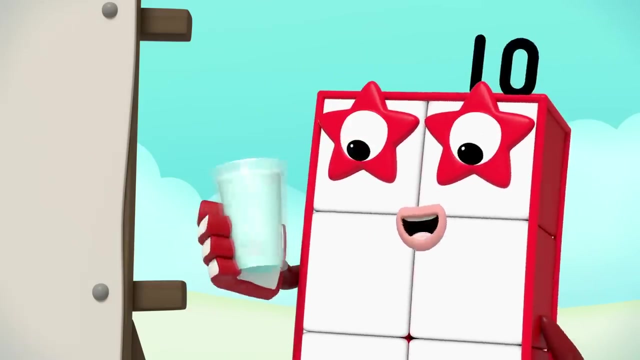 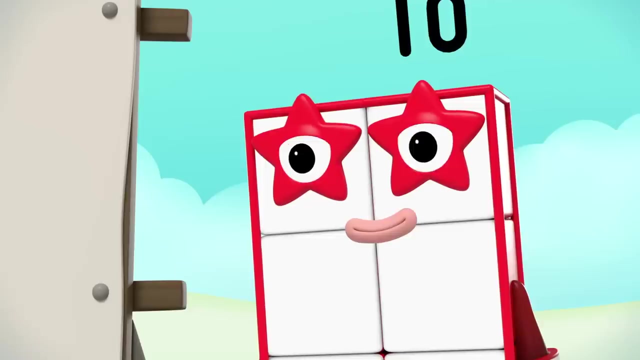 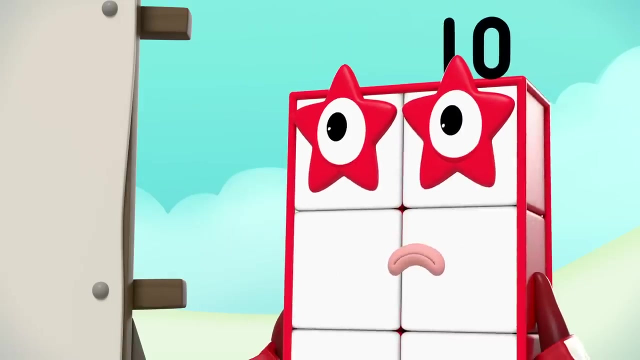 You stand on your head. Huh, I think it's working. Hang on. I know another one. Drink a glass of water backwards Harder. Thanks, Oh, Hang on. It sounds. Oh, We need help, Have no fear. 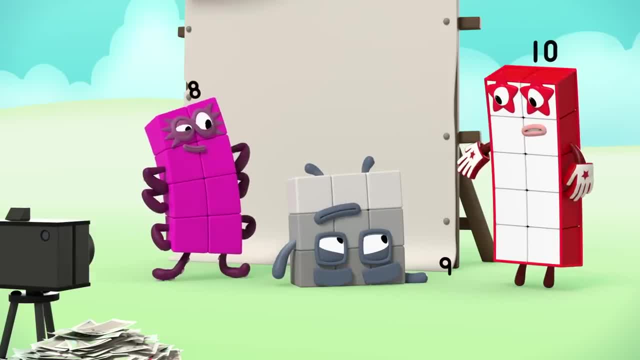 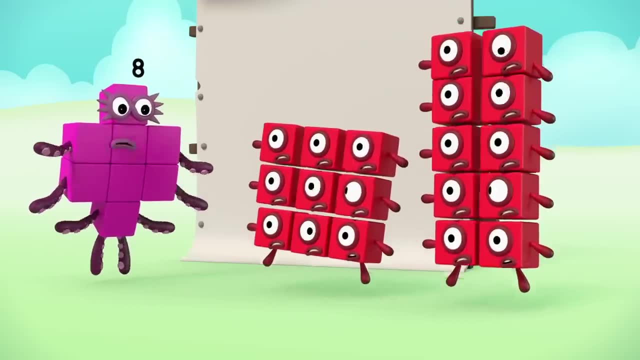 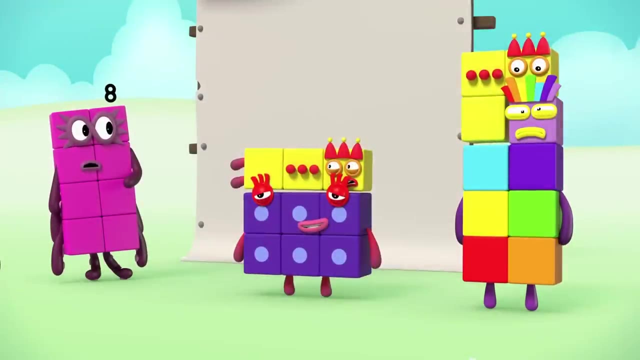 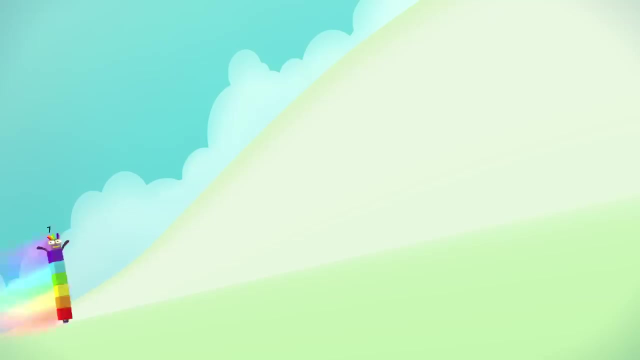 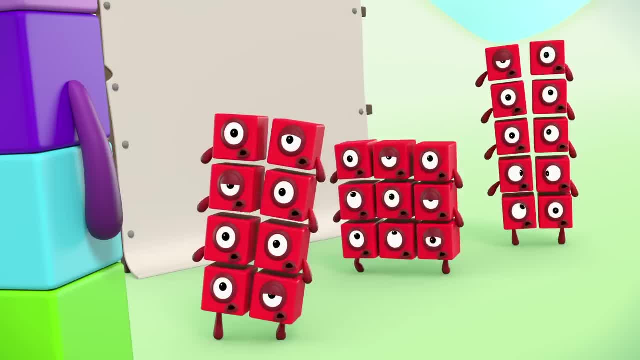 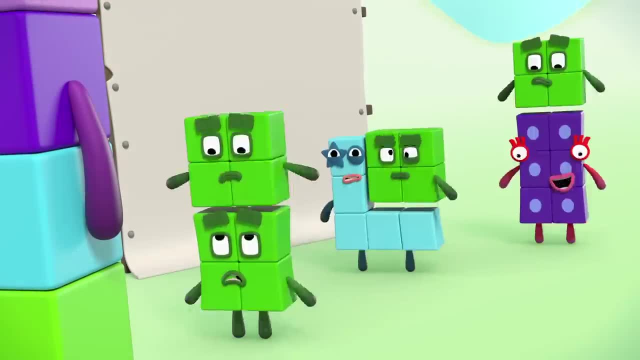 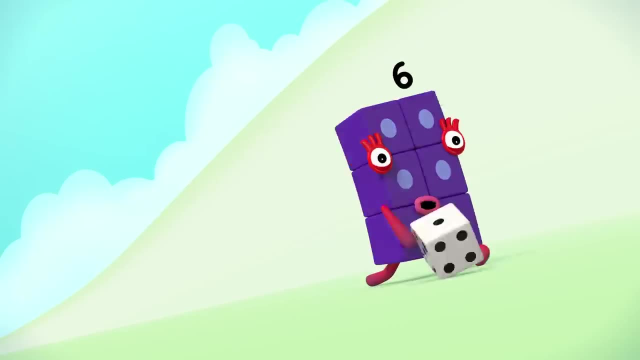 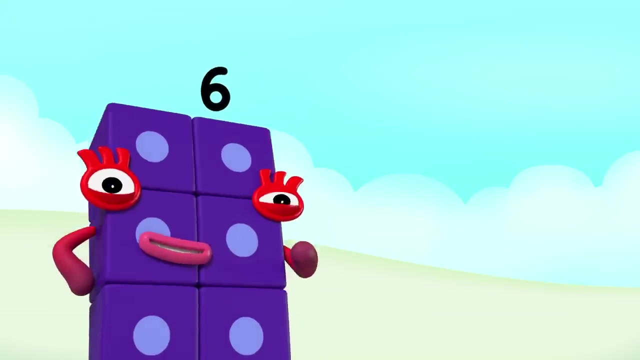 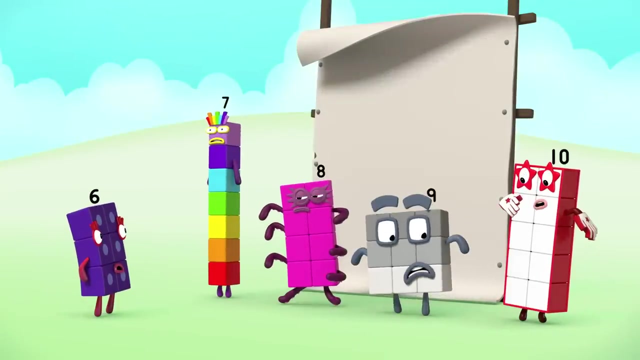 Oh, Oh Oh. I tried that Out of my way Coming through, Got six hiccup cures for you. Let's roll Six. Cure number six: it is Boom, Oh, Boom, Oh, Oh Oh. 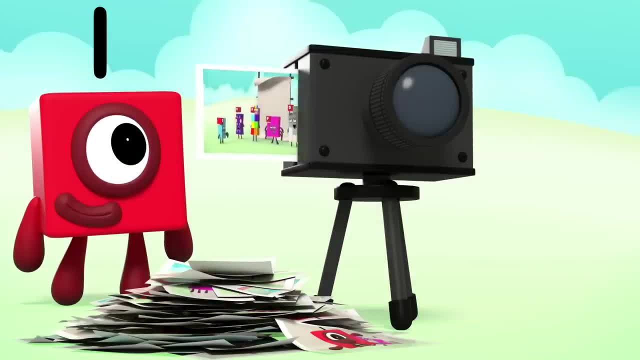 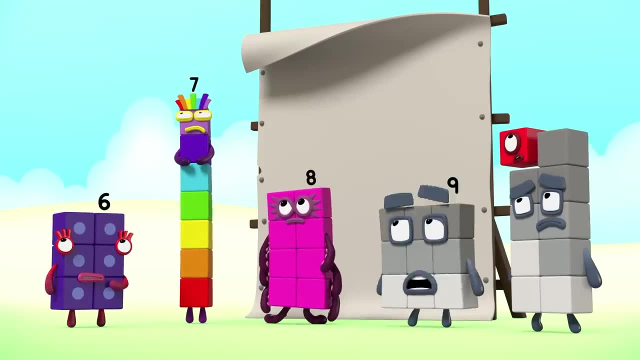 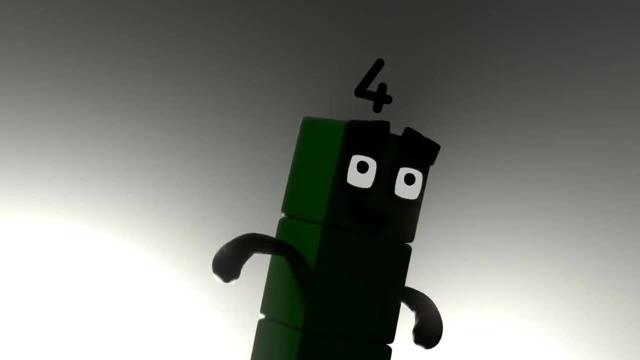 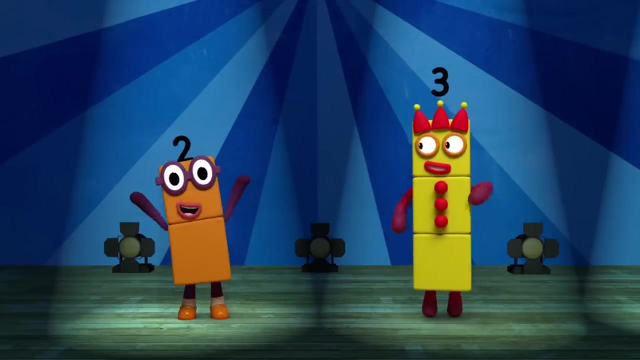 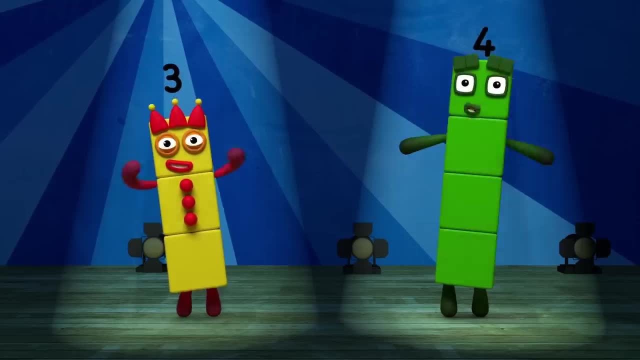 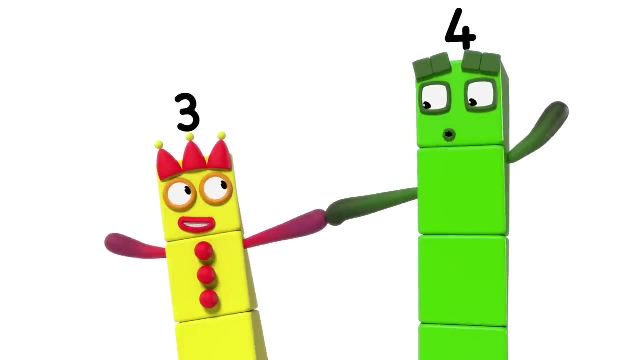 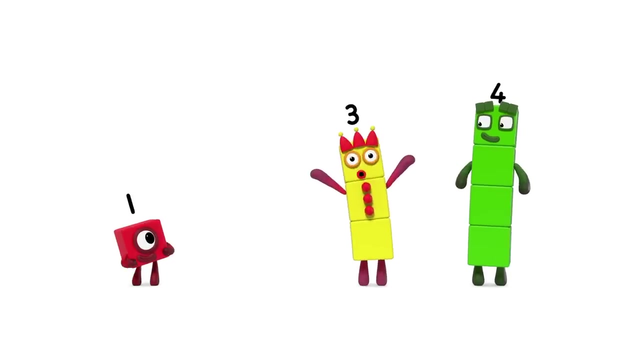 One, two, One two. Three is bigger than two. I can hide behind you. Four is bigger than three. Three can hide behind me. Peek-a-boo, I'm hiding behind you. Can you see me, Peek-a-boo? 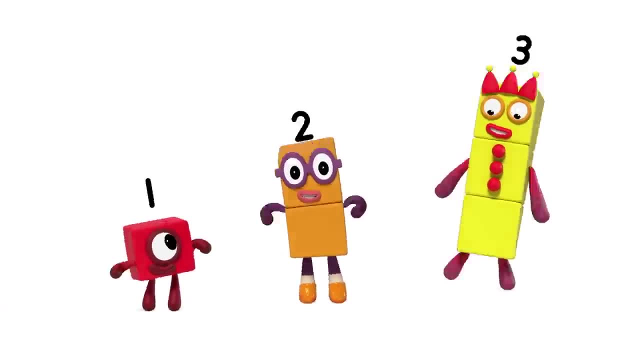 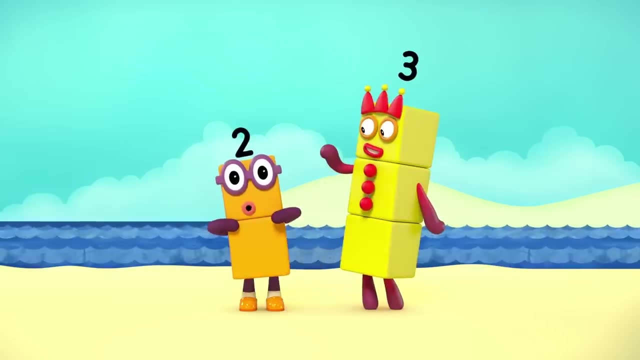 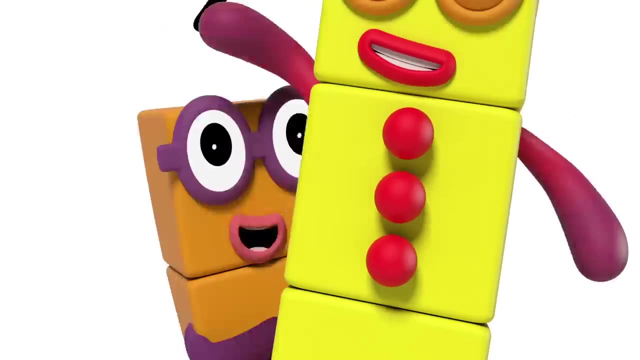 Can you see me, Peek-a-boo? One is smaller than two. I can hide behind you. Two is smaller than three. You can hide behind me, Peek-a-boo. You're hiding behind me, Cause I'm smaller than you. no one will find me. 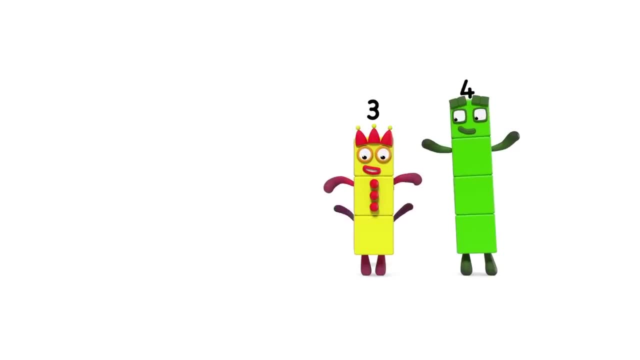 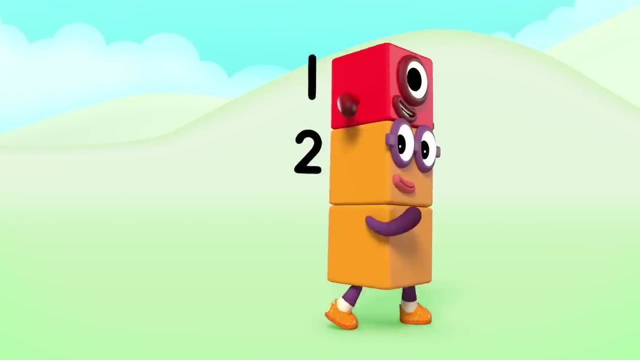 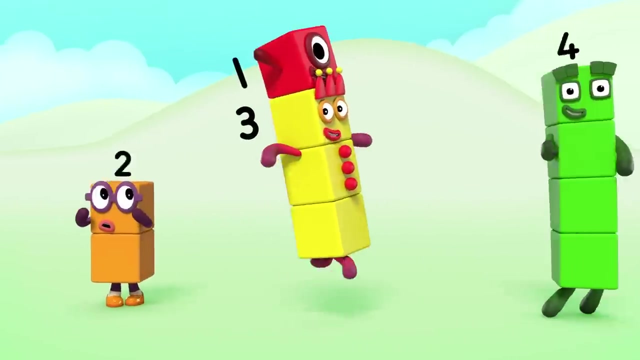 Where have they gone? Go and give us a clue. Can you see me, Peek-a-boo? Can you see me, Peek-a-boo? Two plus one is the same as three. Both of you can hide behind me. Three plus one is the same as four. 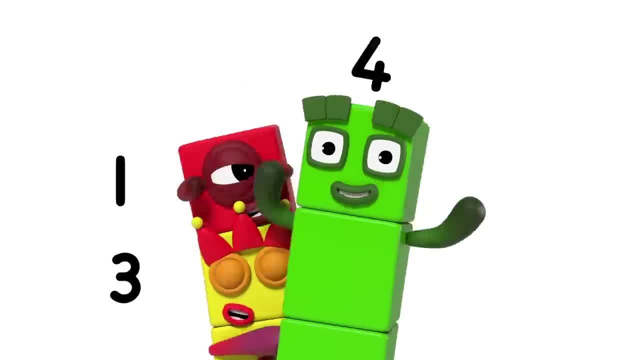 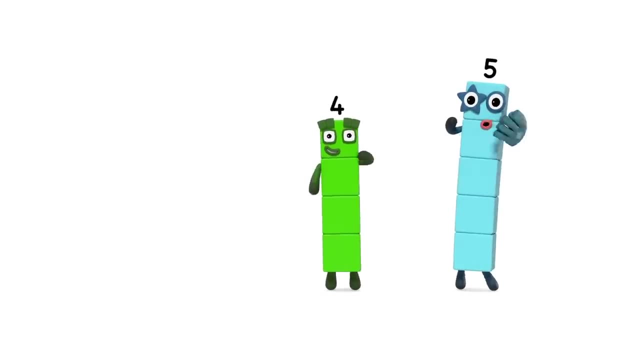 I can hide you both for sure, Peek-a-boo. We're hiding behind you, Cause I'm equal to you. no one will find you. Where have they gone? Go and give us a clue. Can you see me, Peek-a-boo? 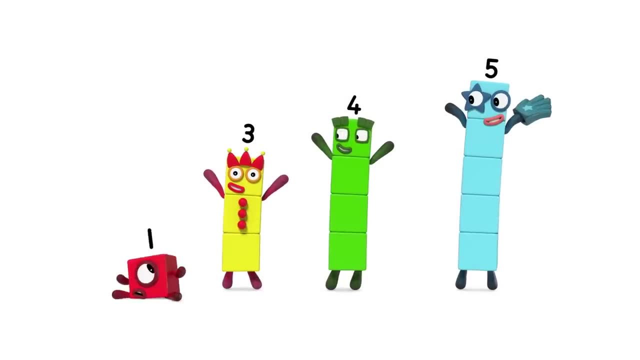 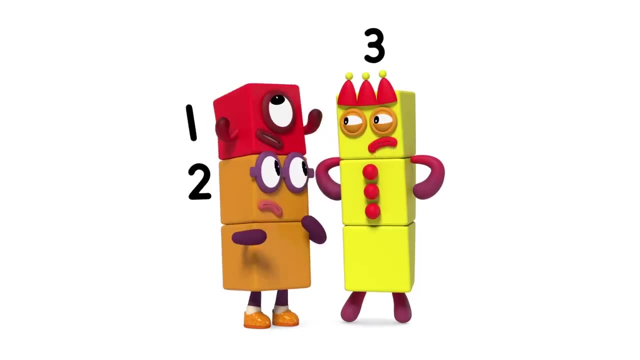 Can you see me? Peek-a-boo. Where is the peek-a-boo? It's supposed to be: two plus one is the same as three. Then you can have one and say: peek-a-boo, That's two plus one. two plus one, one one. 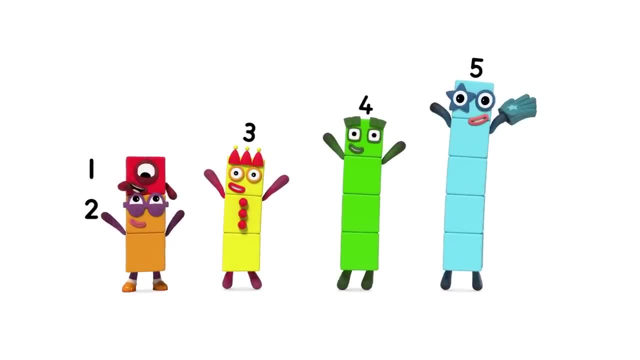 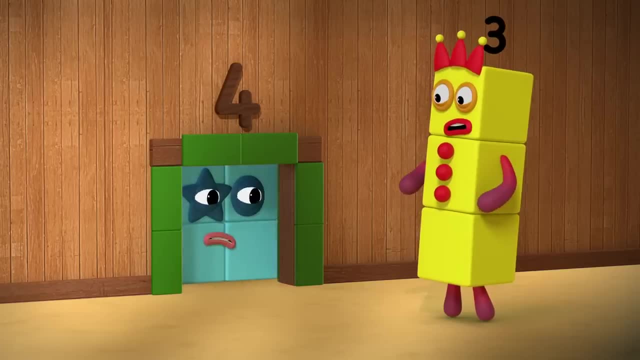 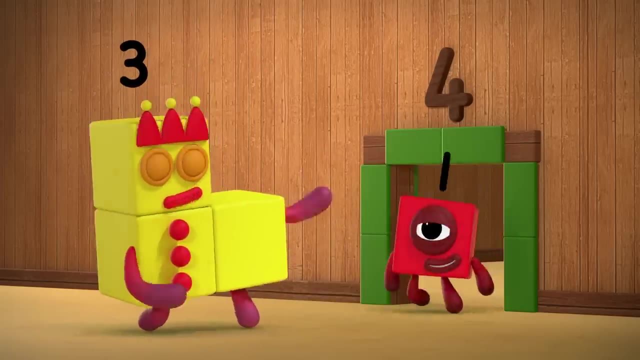 Can you see me Peek-a-boo? Five is bigger than four. I'll never fit through the door, Ow Ow Ow. Three is smaller than four. I can get through the four. Can you see me, Peek-a-boo? 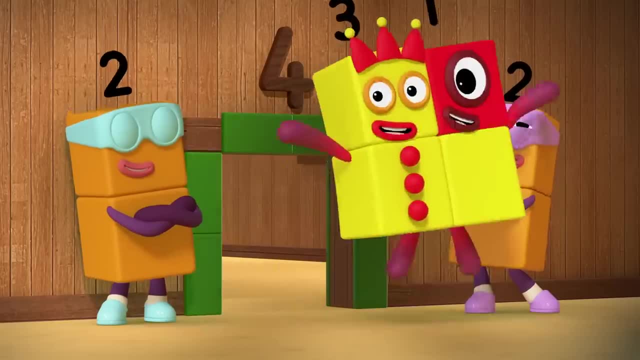 Can you see me, Peek-a-boo? Can you see me, Peek-a-boo? If you're bigger than me, you can't go that far. That's true, Peek-a-boo. Three plus one is the same as four. 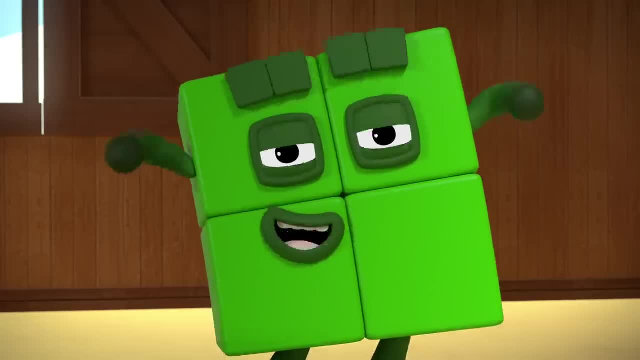 We can fit through the four door. Two plus two is the same as four. Peeking me won't up the score. Peek-a-boo, We're hiding behind you, Cause I'm equal to you. no one will find you. Where have they gone? 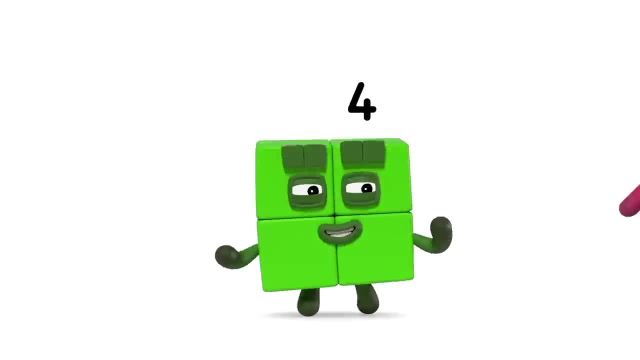 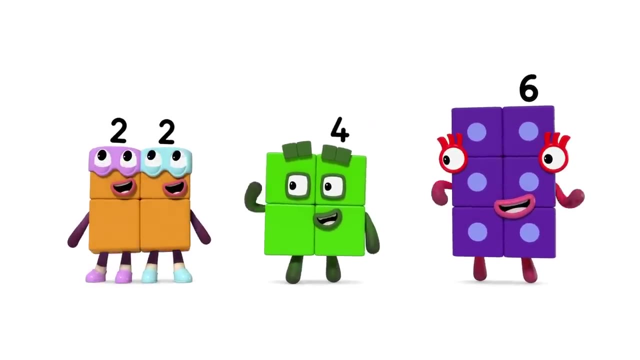 Go and give us a clue. Can you see me, Peek-a-boo? Can you see me, Peek-a-boo? If you're bigger than me, you can't go that far. Peek-a-boo, Can you see me? 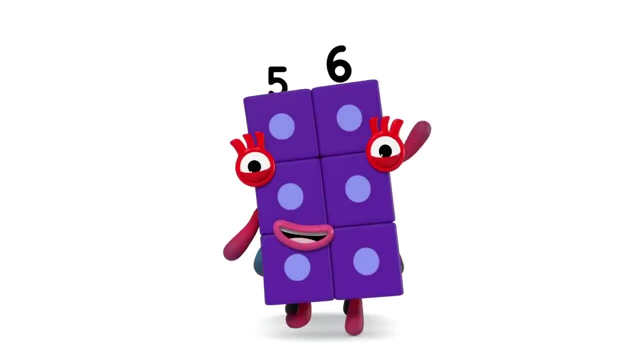 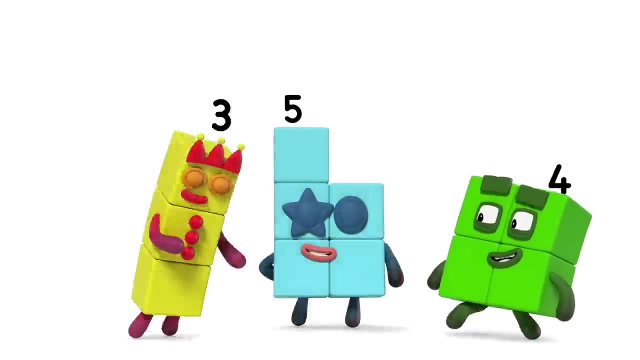 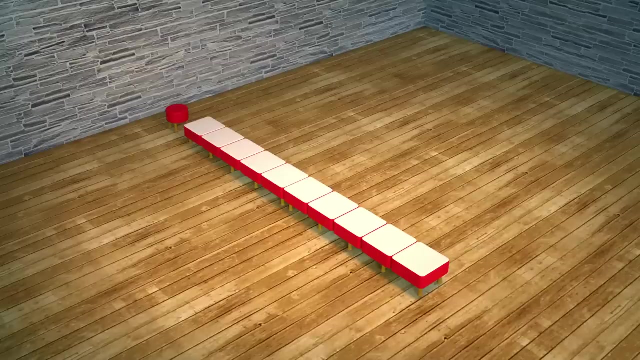 Peek-a-boo. If you're bigger than me, you can hide me As long as you make the right shape. If you're smaller than me, it'll never work, No matter what shape you make. Six won't fit into four's little bed. I can lie down in ten's bed instead. 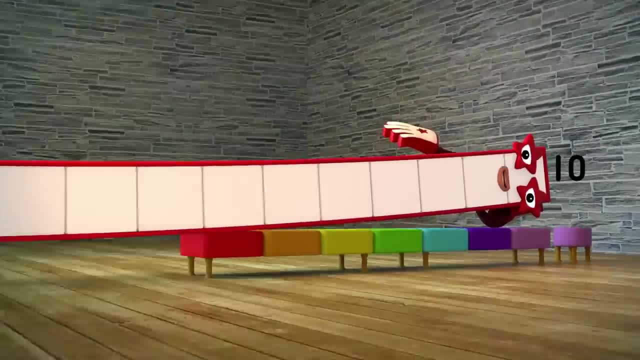 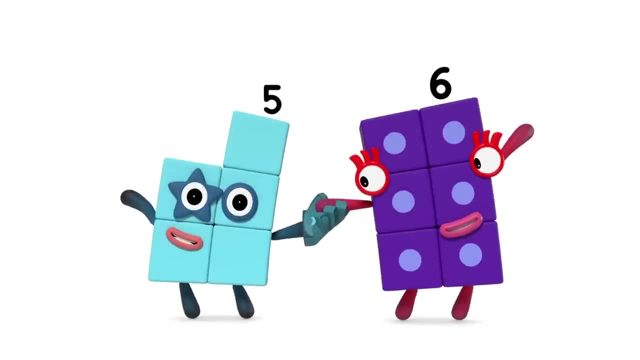 Seven's bed is too small for ten. My feet will stick right at the end. Peek-a-boo, I'm hiding behind you. If you're bigger than me, no one will find you. Where have they gone? Go on, give us a clue. Can you see me? 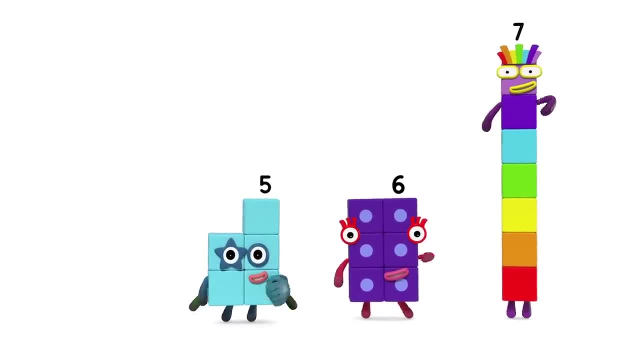 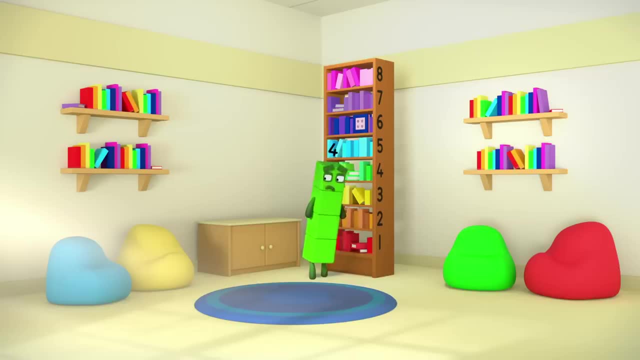 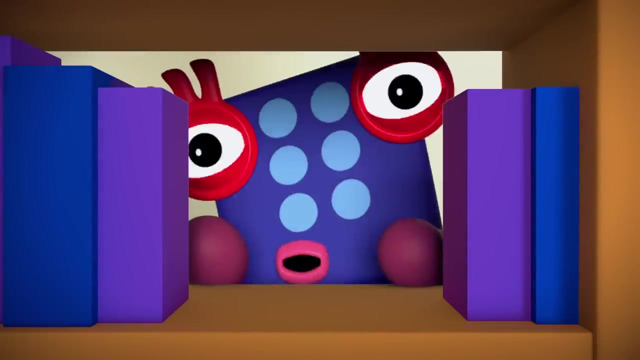 Peek-a-boo. Can you see me, Peek-a-boo? Four can't reach up to Six himself. I'll have to leave that book on the shelf. Eight can bend down to reach the book. Six can peek through. Take a look, Peek-a-boo. 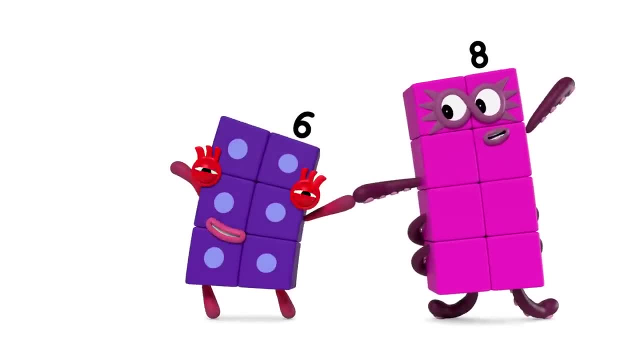 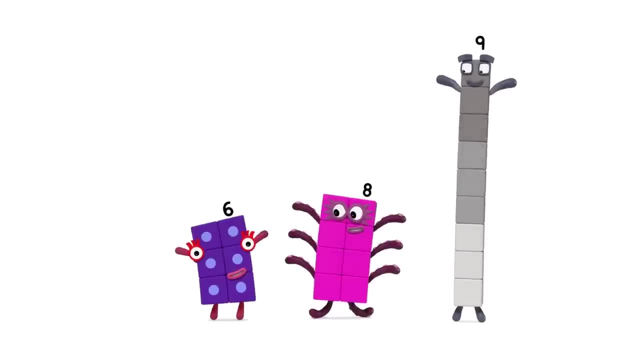 I'm hiding behind you. If you're bigger than me, no one can find you. Where have they gone? Go on, give us a clue. Can you see me, Peek-a-boo? Can you see me, Peek-a-boo? One is smaller than. 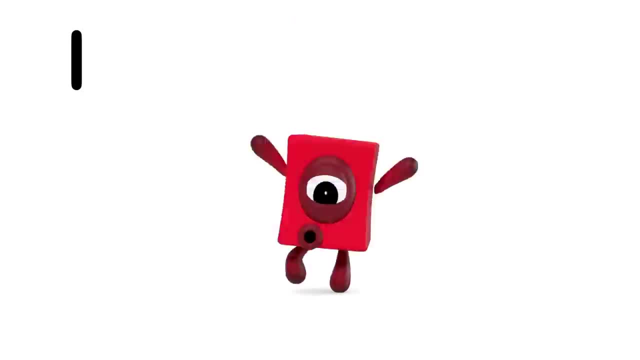 Fewer than Less than One, is less than Two, is less than Three, is less than Four, Five is less than Six, is less than Seven And eight is less than Nine is less than Ten, And ten is bigger than More than Greater than Ten is greater than Nine is greater than. 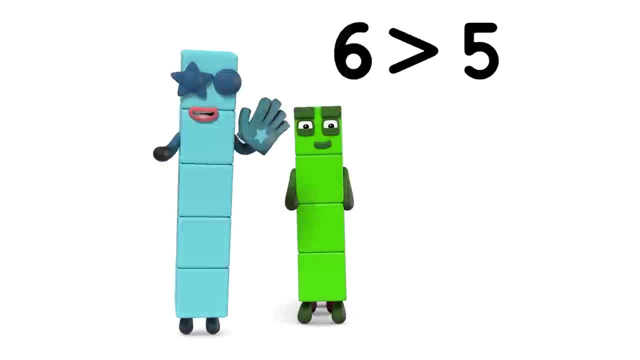 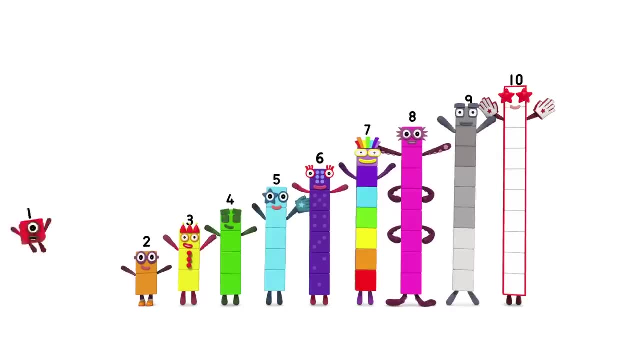 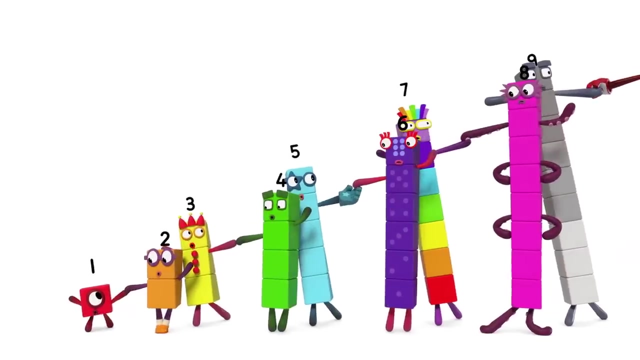 Eight is greater than Seven, Six is greater than Five is greater than Four, is greater than Three And three is greater than Two is greater than One. Peek-a-boo, I'm hiding behind you, Cos I'm bigger than you. No one will find you. Where have they gone? 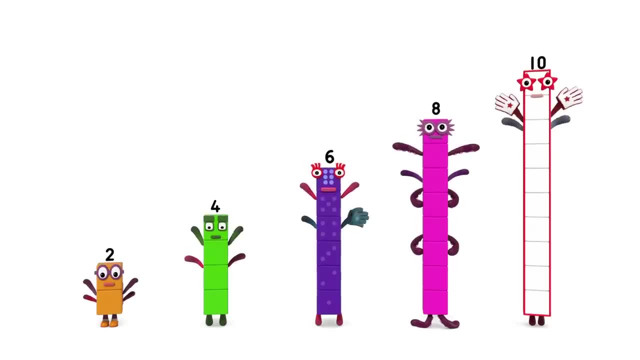 Go on, give us a clue. Can you see me, Peek-a-boo? Can you see me, Peek-a-boo? Welcome to the Numbah Block Rally. Ten riders, ten pedal-powered cars, but only one can lift the trophy. 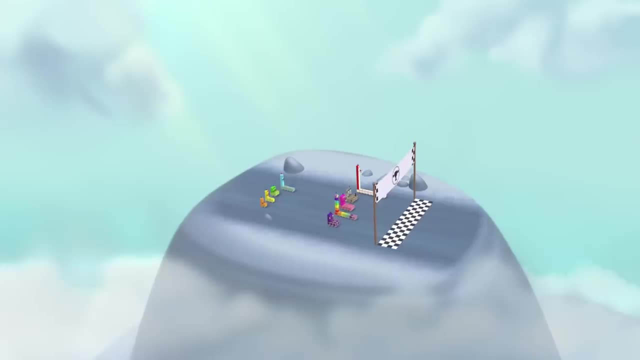 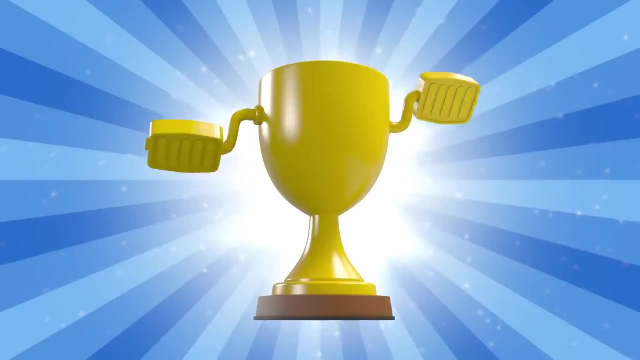 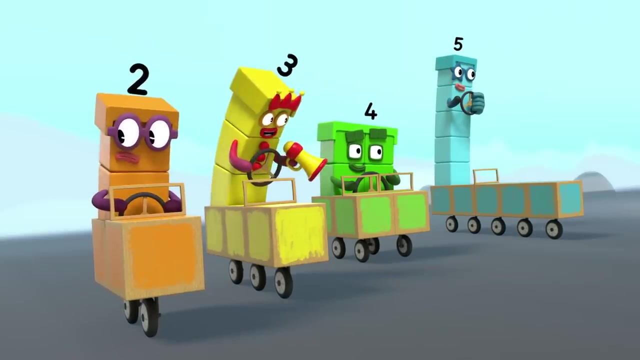 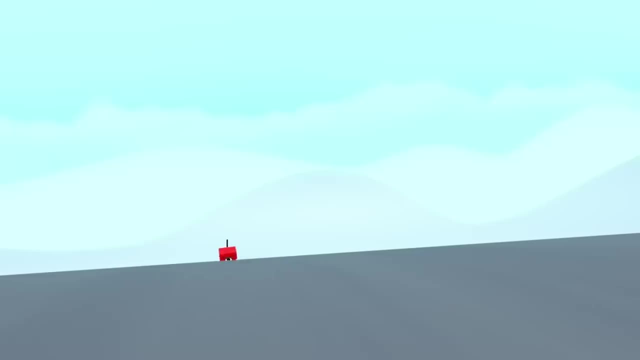 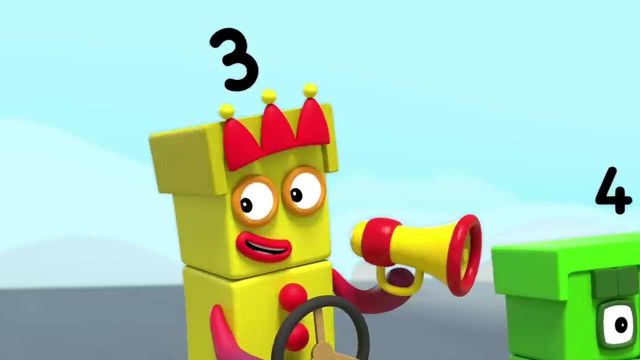 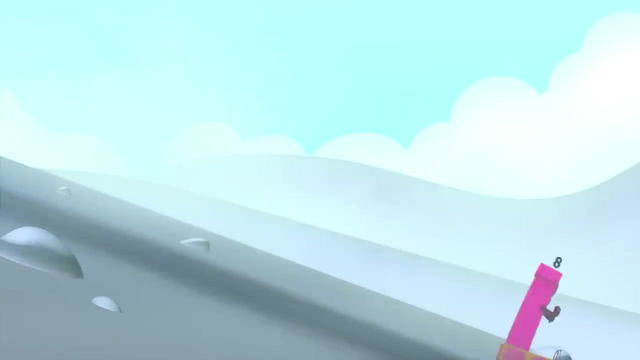 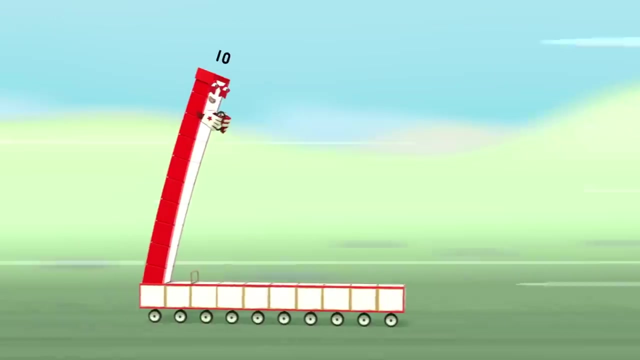 No, No, Has anyone seen it? Yes, I think we are outаетed. Two Two, Two, Two, One One, One, Two, Two, One, One, Two, Two, Two, Two, Three, Four, Three, Three, Four, Four, Five, Six, Six, Seven, Ten. Ten is in the lead with ten wheels. she seems unbeatable. 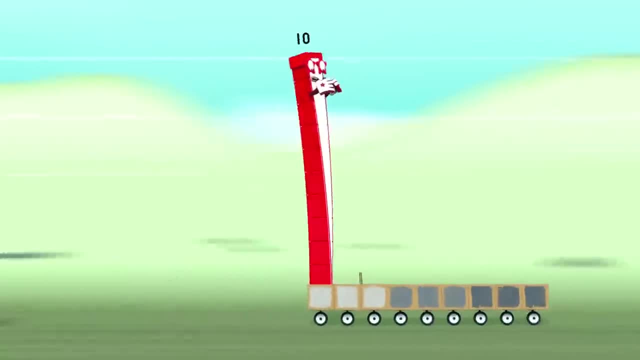 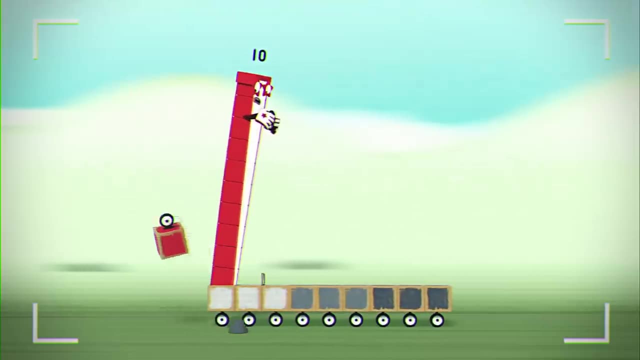 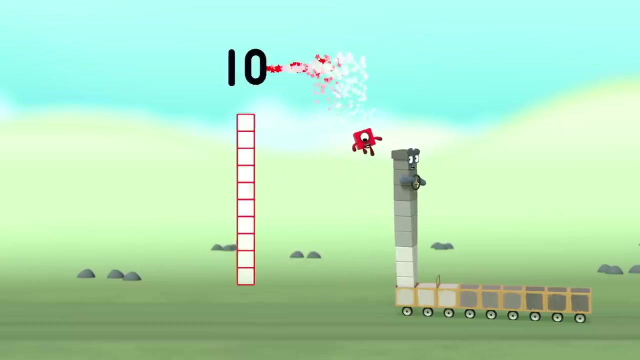 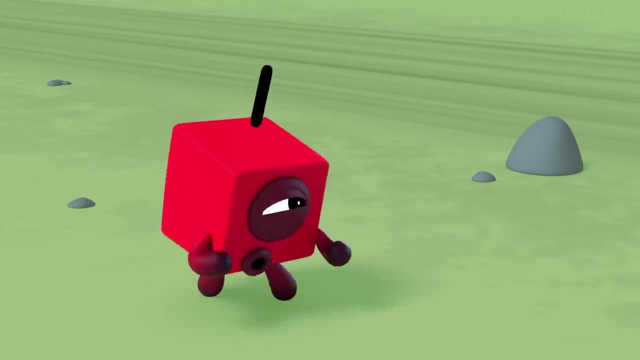 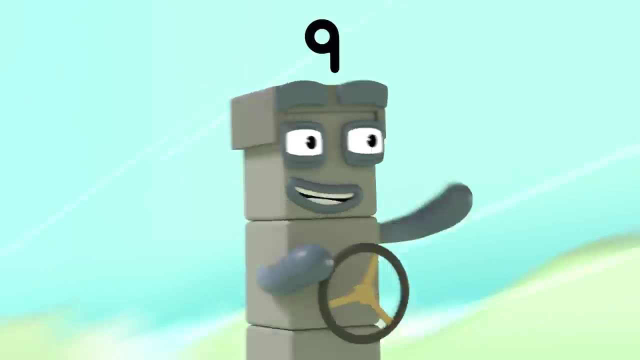 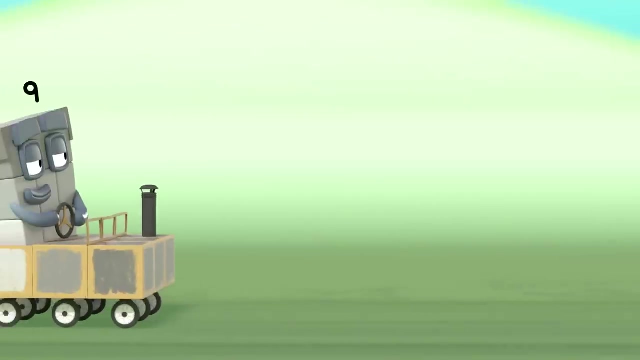 But wait, she's lost a wheel. Let's see that again in slow motion. Ten wheels minus one wheel equals nine wheels left. Ten minus one equals nine Go nine. Ten is out of the race. as nine takes a surprise lead, Nice day for it. And what makes it really surprising is that nine's in last place too. 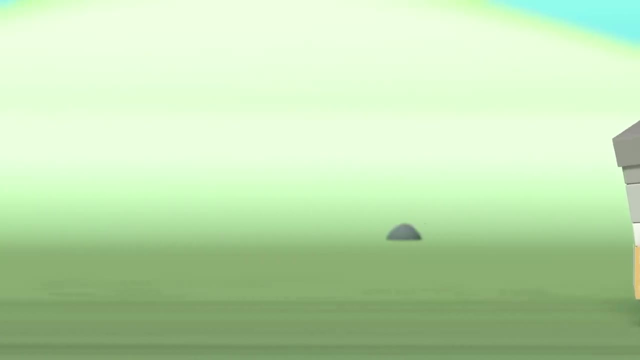 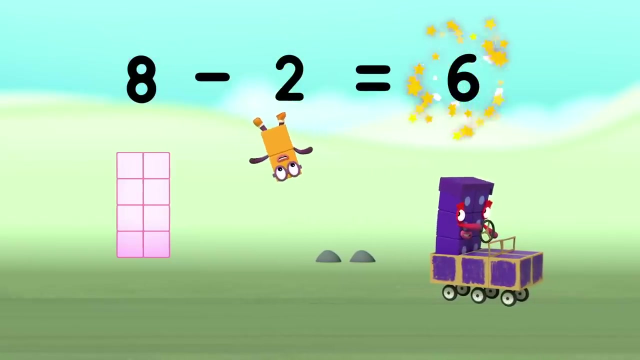 Well, next to last, Keep pedalling, Ron. Octoblock race One, two, three, four, five, six, seven, eight Race. It's in trouble. Those two crumplops are about to go. Eight Minus two Equals six, Look out. 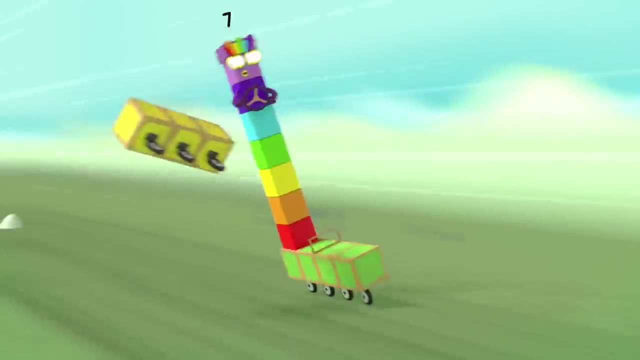 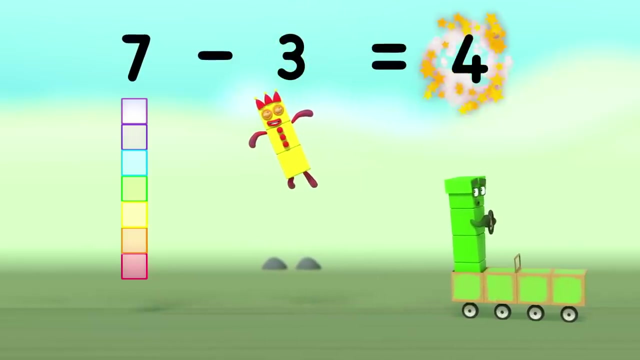 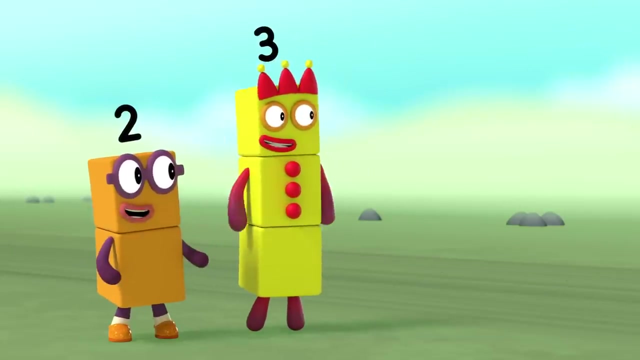 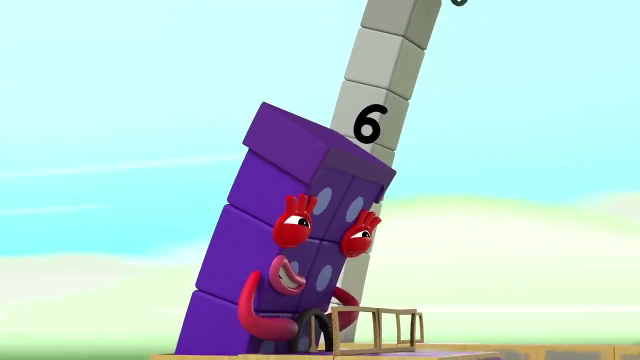 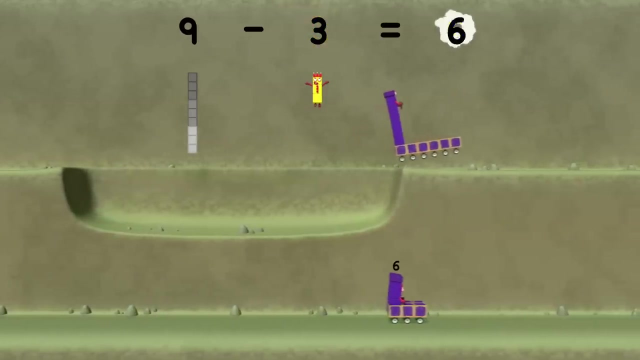 Phew, that wasn't a key. Seven Minus three Equals four. Four wheel drive: Yay, Yay, Yay, Yay Yay. Six has caught up with nine as they enter the double dipper. Mind that dip Nine minus three equals six. 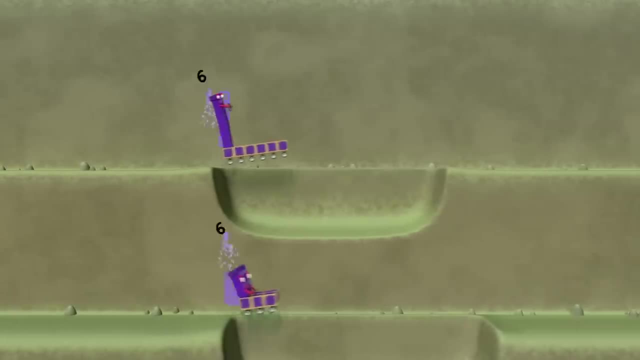 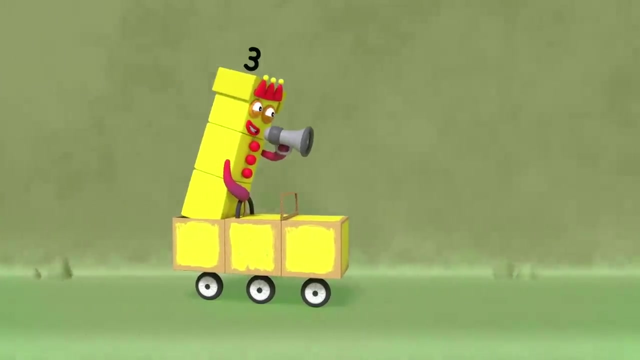 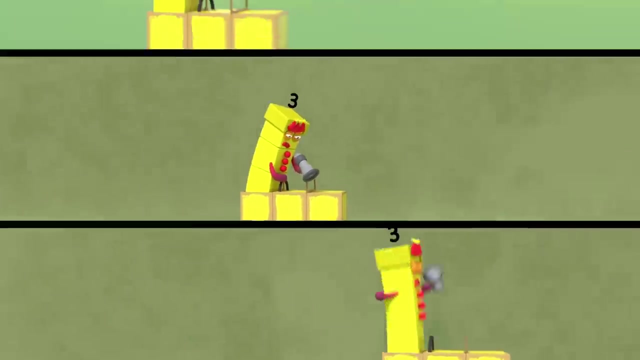 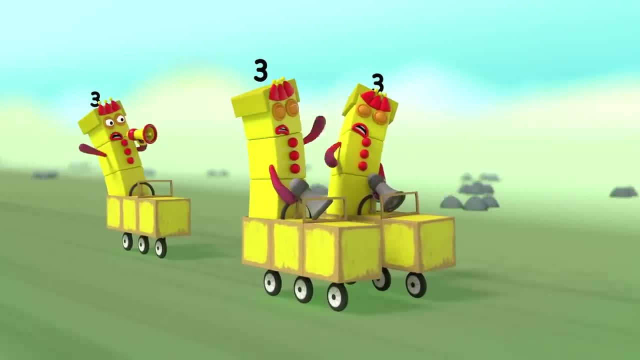 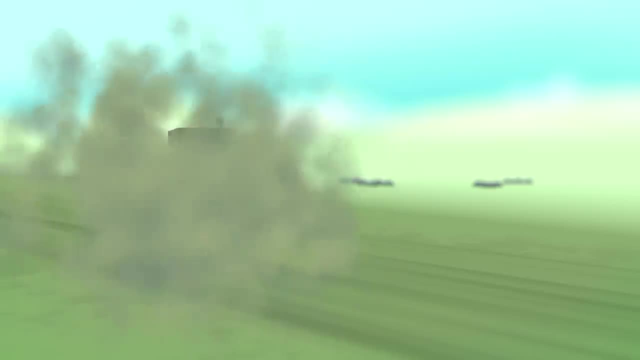 Me, me, me, Yeah, Pull yourselves together. Four plus three equals, three equals me. Oh, Uh-huh Achoo. Back in action And with the finish line in sight, It's four in the lead. Then I need a breather. 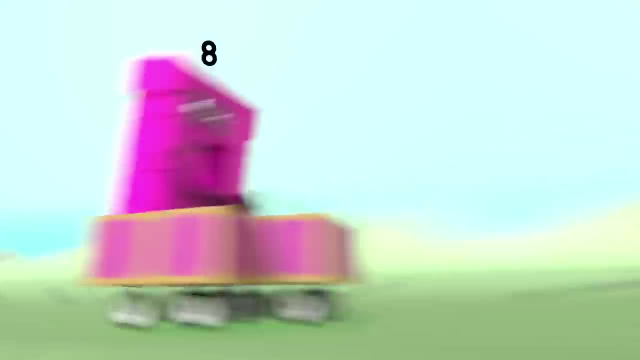 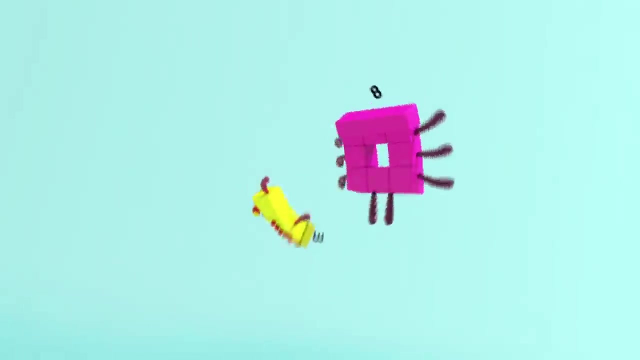 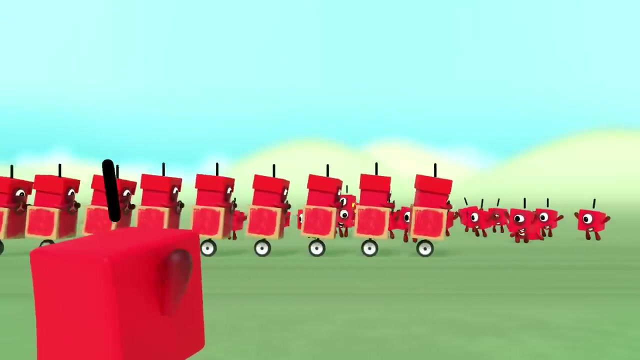 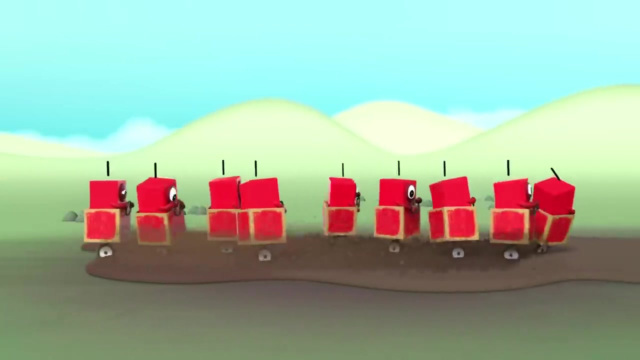 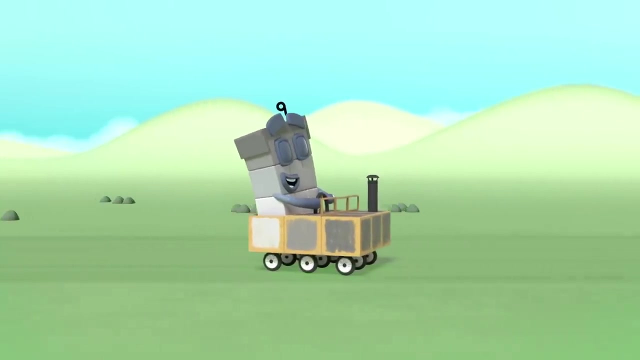 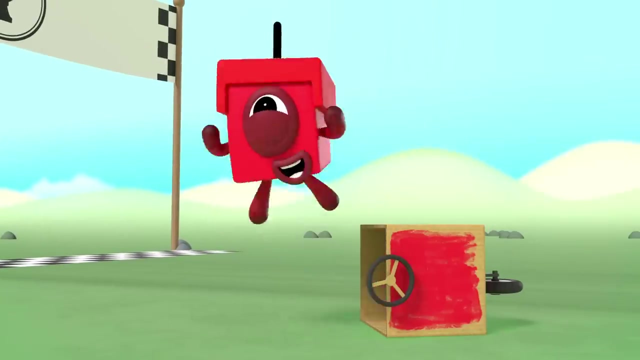 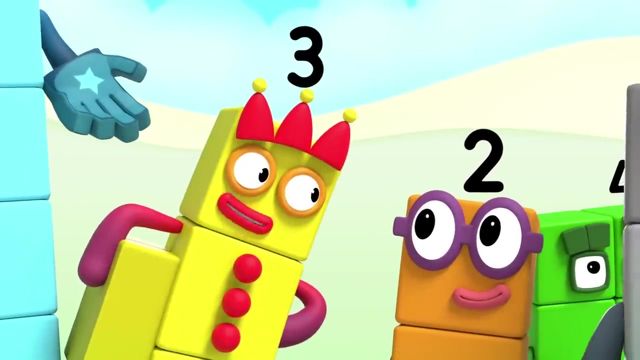 Octoblock coming through, Octoblock coming through, and it's one in the lead, followed by one, but here's one coming up on the inside. nine wolf sequels, nine, nice day for it. well, i said only one can lift the trophy, and i was right. 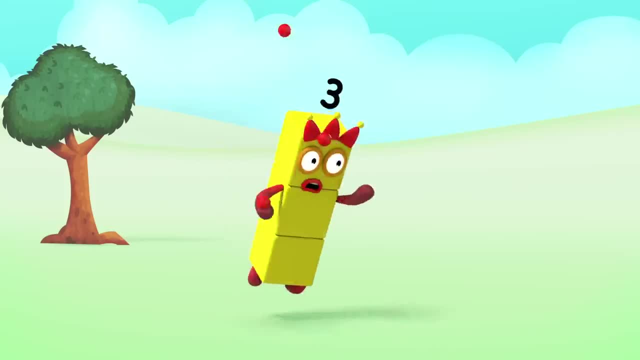 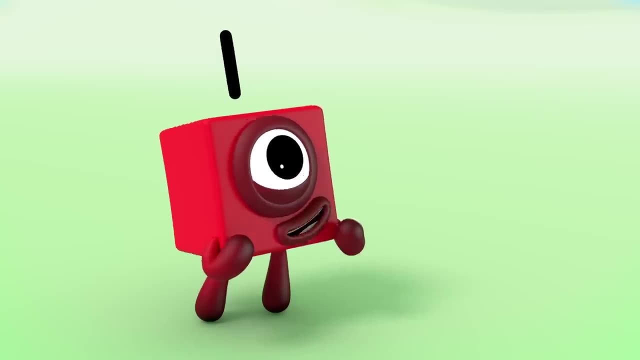 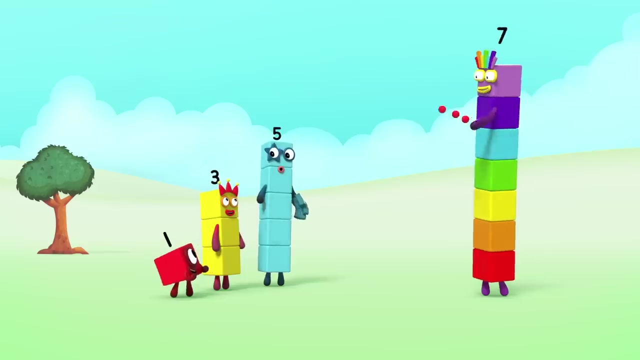 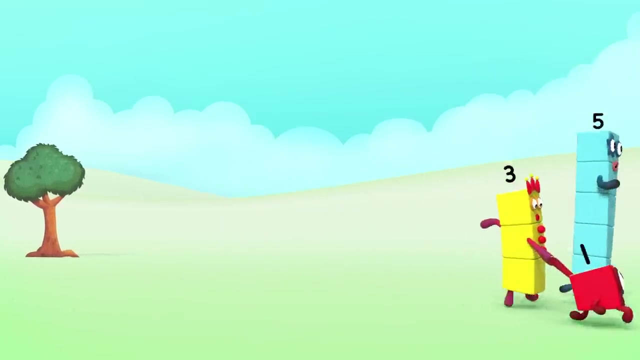 lucky catch. i wish i could be you- seven you're so. you're so lucky you can be me. just ask a friend to jump on your head. but first you have to know the difference between you and me. we all have a place, but we're different. that's very easy to see. 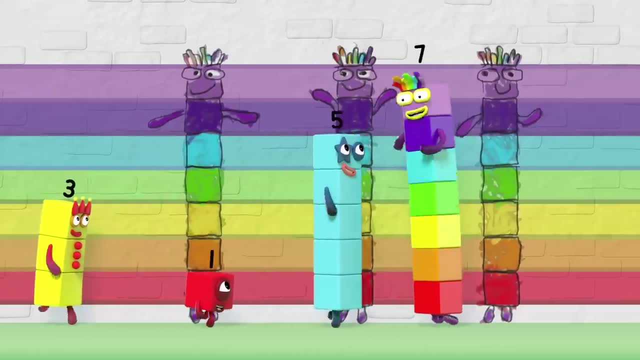 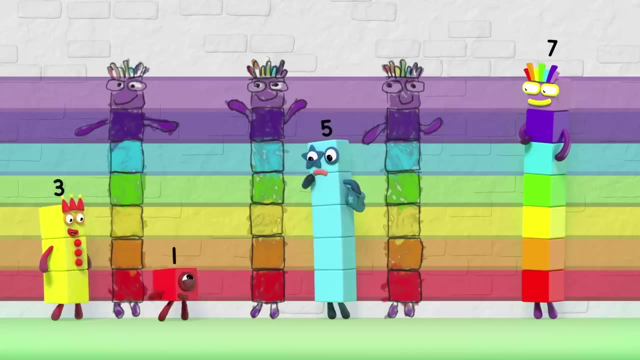 we're all friends here, but we're different. but what makes you you and not me? i'd love to be you, but i come up short. i need to add something, but what? me? i'd love to be you, but i come up short. i need to add something, but what? 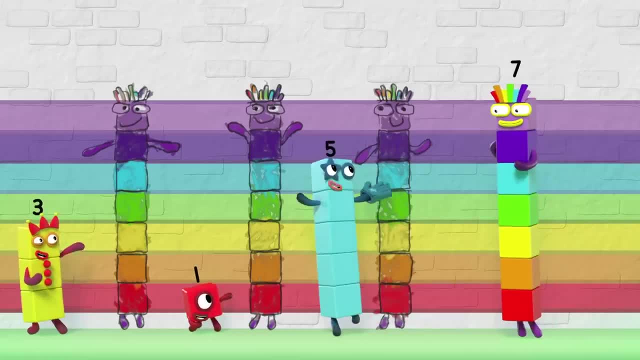 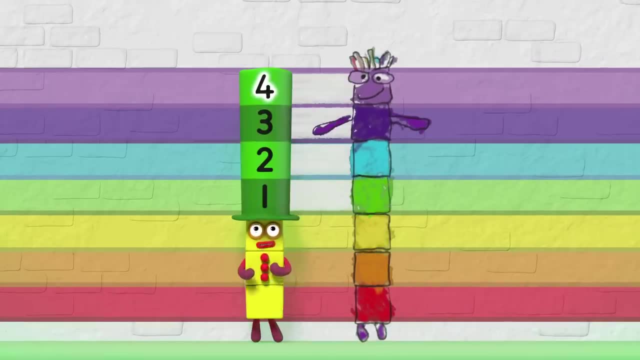 me, i'd love to be lucky like seven. me, i'd love to be lucky like seven. one of you got that we haven't got. i could try on a hat, that's the difference. or i could stand on a box, that's the difference. don't under the difference. 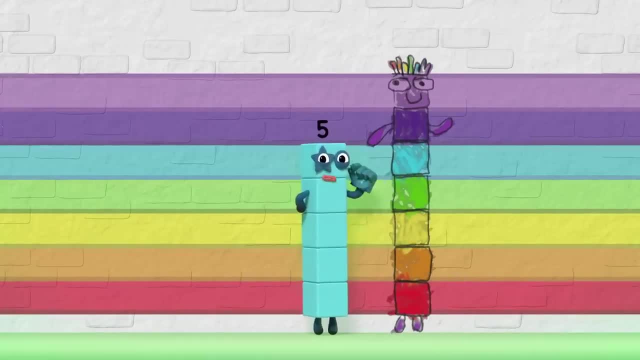 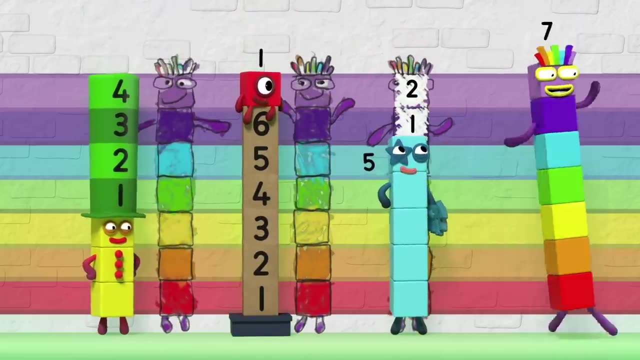 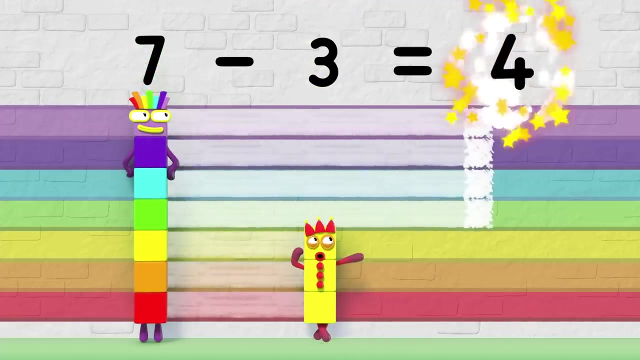 won't pop into your head. you can count the missing blocks. one, two, two. the difference is two, the difference is two. so what's the difference? so what's the difference? seven minus three equals four. that's the difference. four, seven minus me equals six. that's the difference. 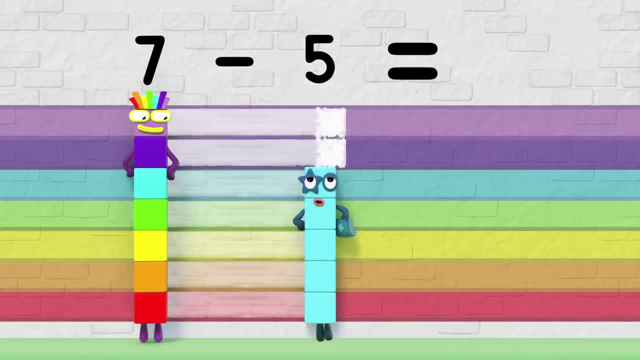 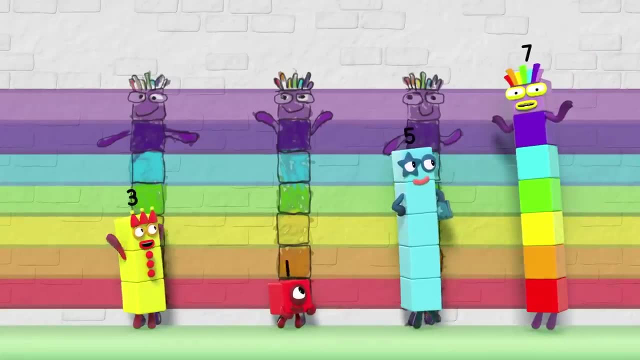 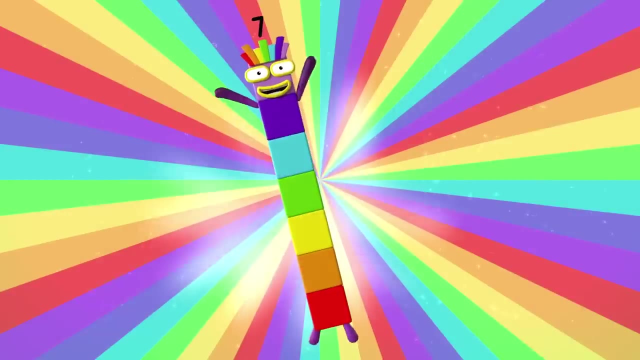 six seven minus five equals two. that's the difference. so make up the difference and everyone will see what the difference is between you and me. i'd love to be you, but i come up short. i need to add something. but what i'd love- to be stronger like nine- is 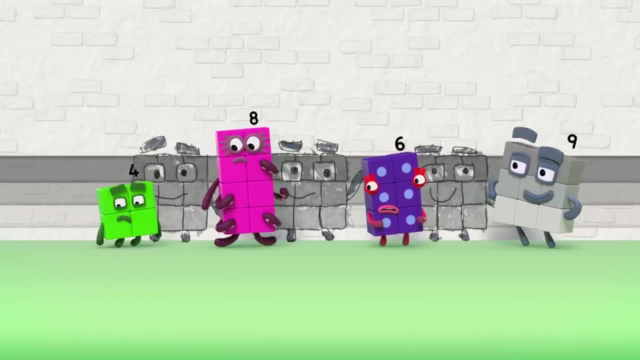 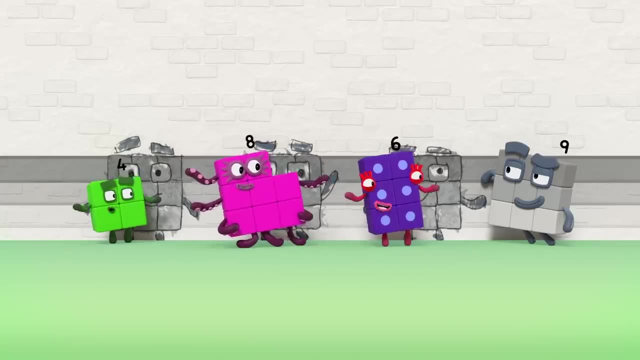 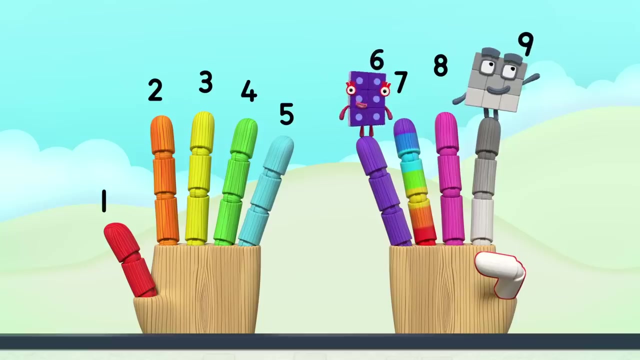 what have you got? if we haven't got, you can count on your hands. seven, eight, nine. that's the difference. three one, two, three. you can fill in the space. that's the difference. three one, two, three. you can fill in the space. that's the difference. you can fill in the space. 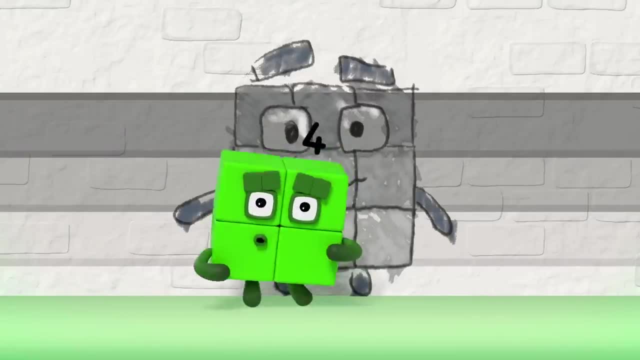 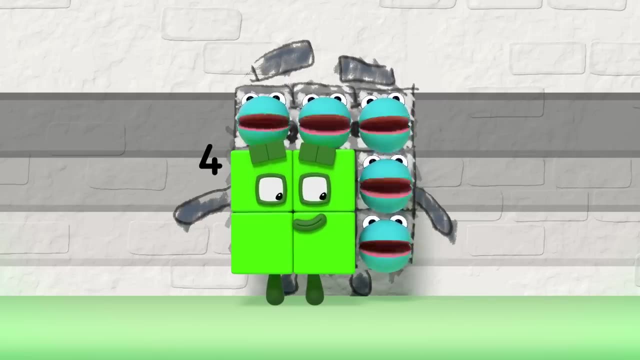 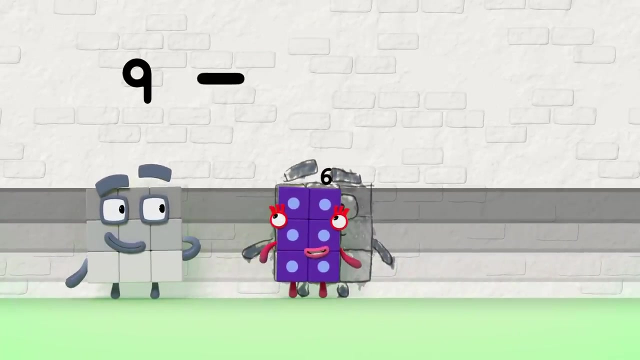 the difference one. and if the difference won't pop into your head, you can count number blocks in place: one, two, three, four, five. the difference is five. so what's the difference? nine minus six equals three. that's the difference. three. nine minus me equals one. that's the difference. 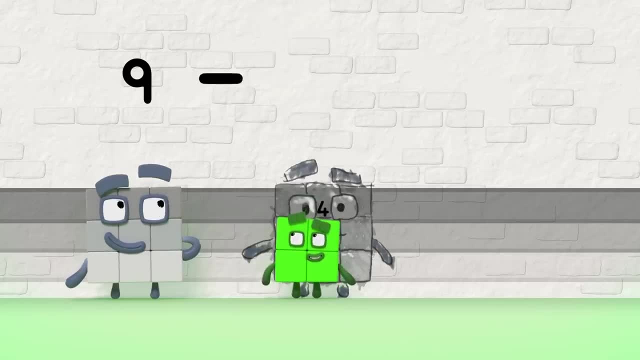 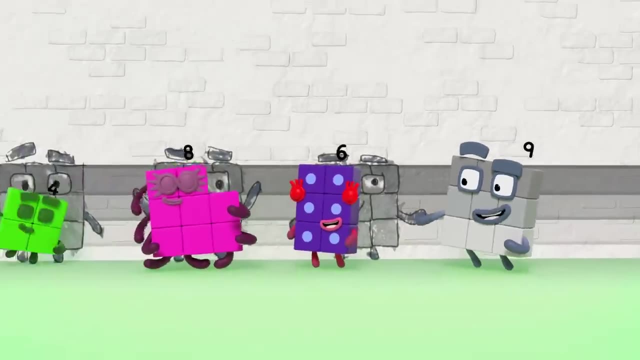 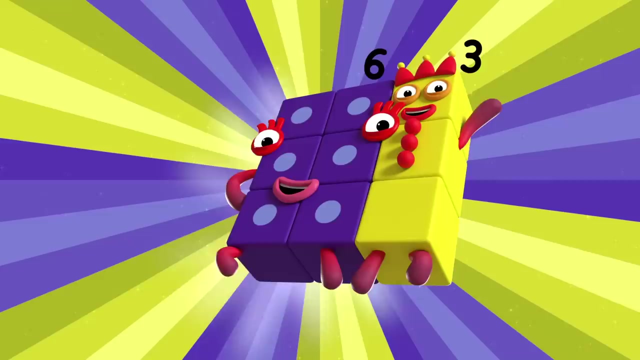 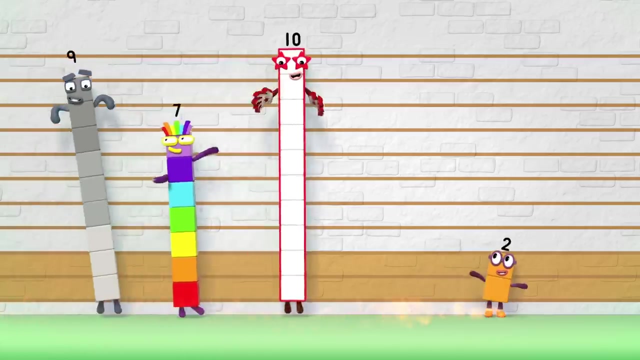 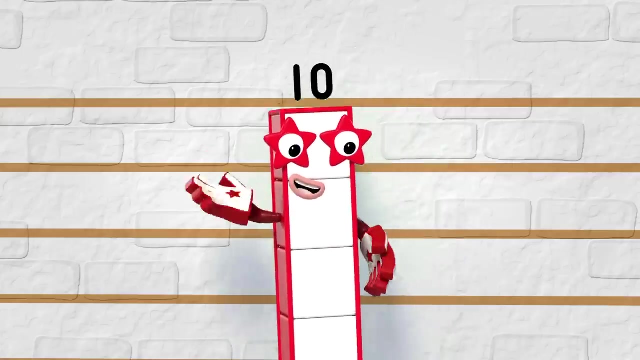 one. nine minus four equals five. that's the difference, five. so make up the difference and everyone will see what the difference is between you and me. i'd love to be you, but i'm much too big. we need to lose something. but what i'd love to have some of. 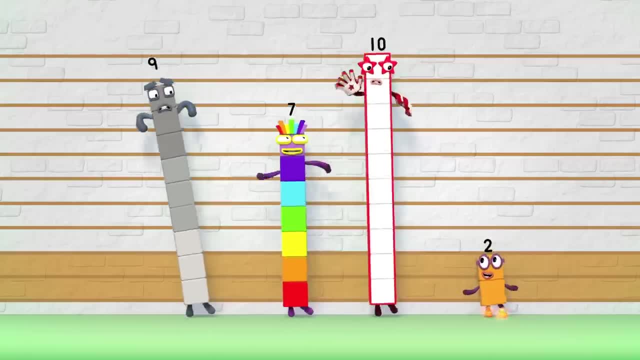 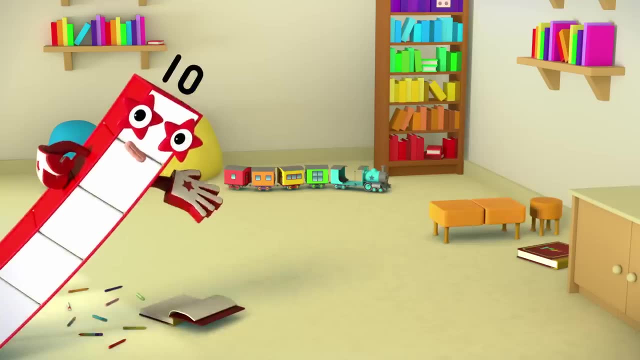 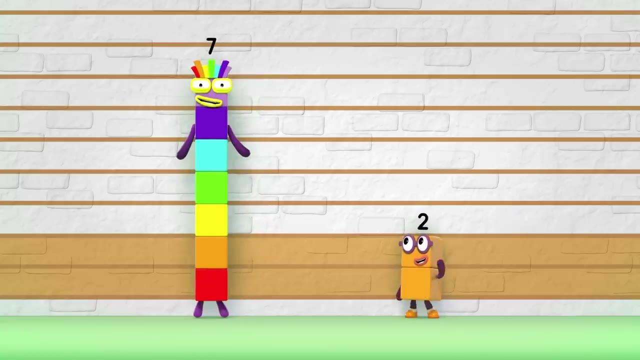 your talent. what makes you two and someone? we're not. i can walk through a door. that's the difference. i could get into bed. that's the difference. and if the numbers won't pop into your head, you can count the extra blocks instead: one, two, three, four, five. 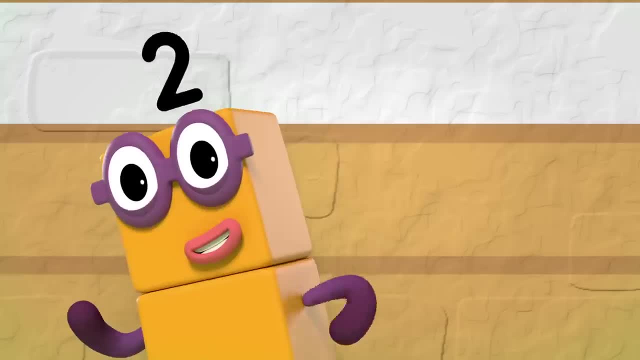 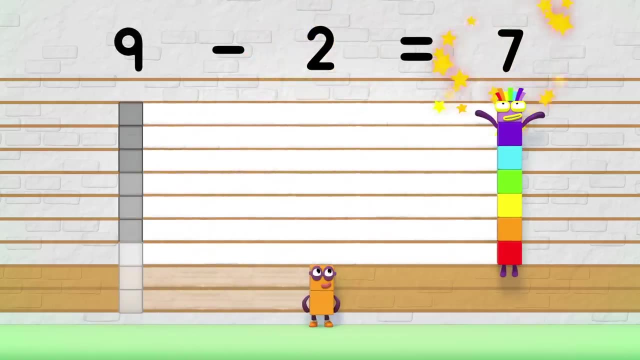 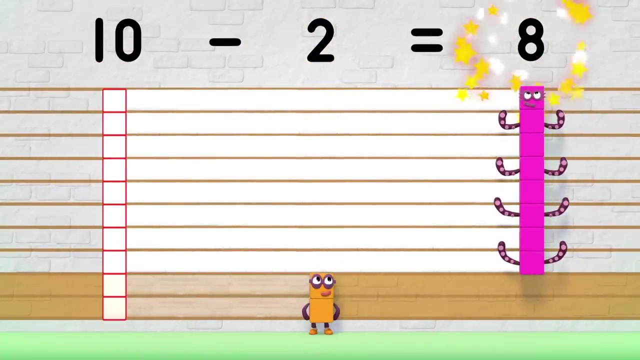 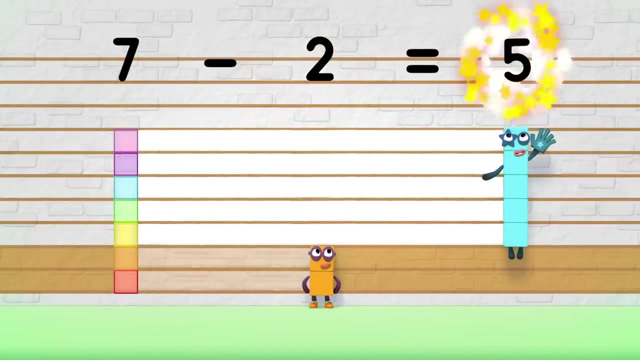 five. the difference is five. so what's the difference? minus two equals seven. that's the difference seven. ten minus two equals eight. that's the difference eight. seven minus two equals five. that's the difference five. so take off the difference and everyone will see what the difference. 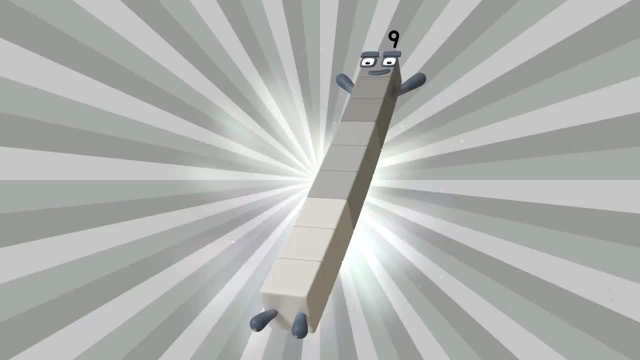 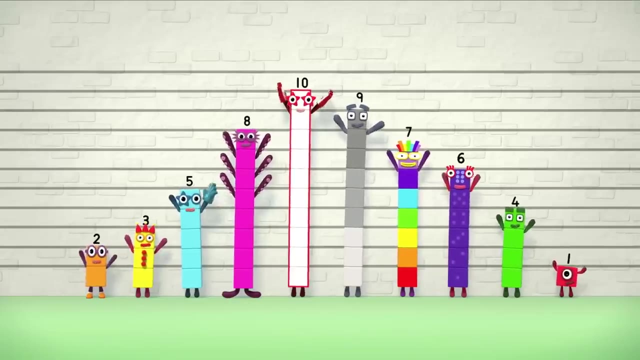 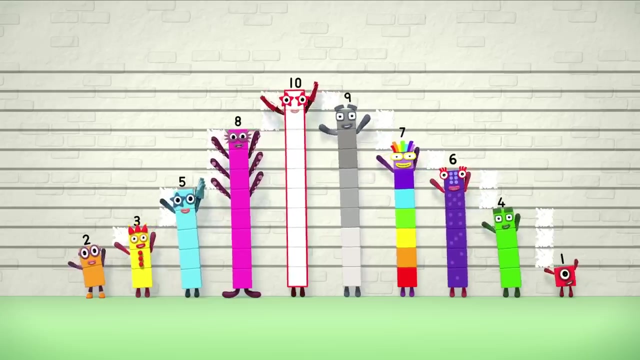 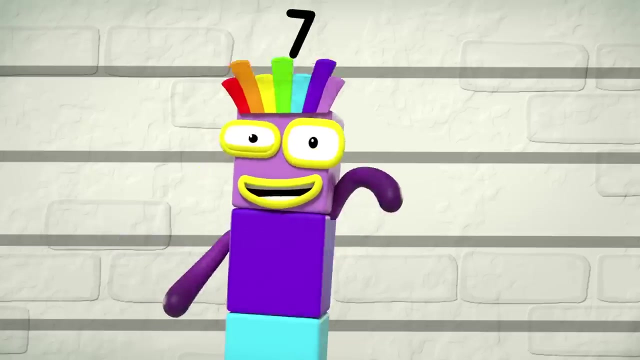 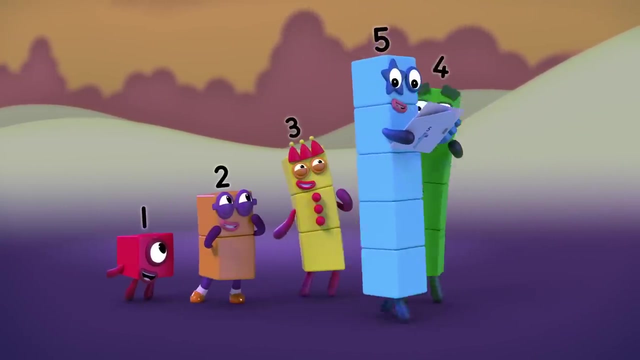 is between you and me. we all have our place, but we're different. you have to admit. we've come far. we're all friends here, but we're different, and the differences between us make us who we are now. what could this be? five and friends are invited to a five star ball. 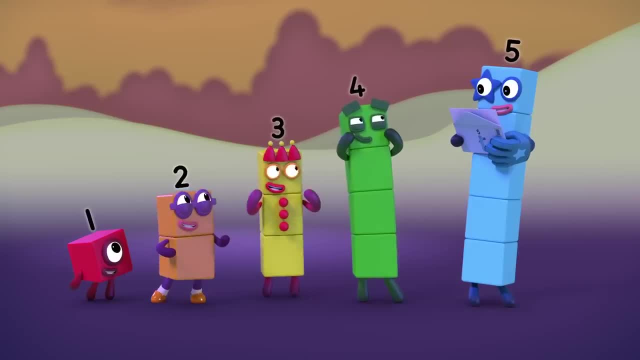 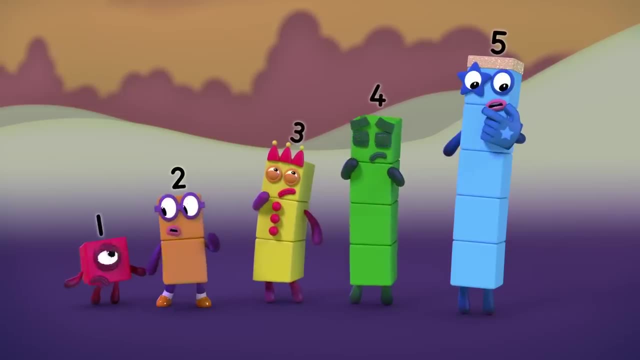 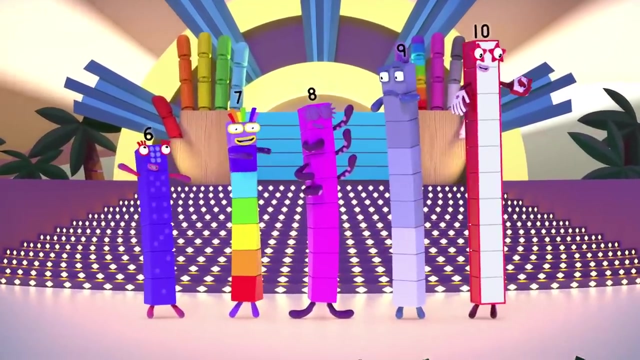 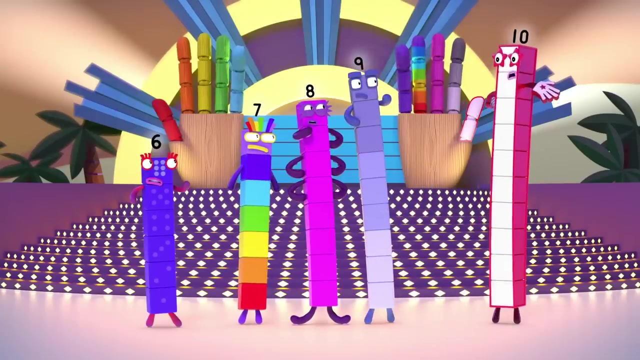 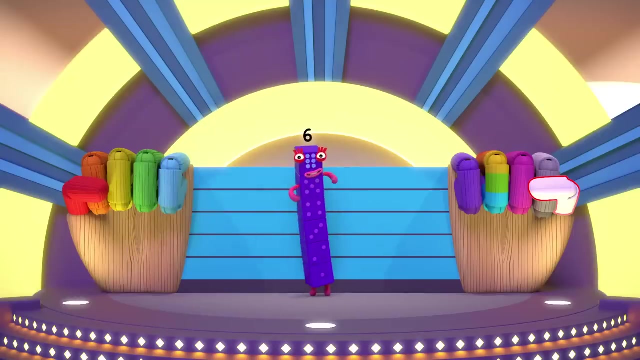 at the two palms dance floor. i can wear my sparkly headband at the two palms. where's that? um, hold on, where's five? we can't start a five and friends dance without five. why wait? just look and you will see that five is here as part of me. 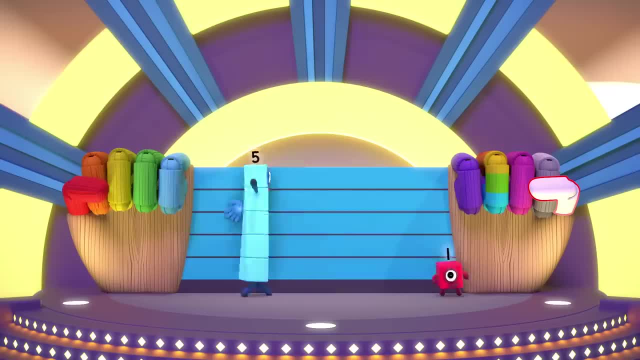 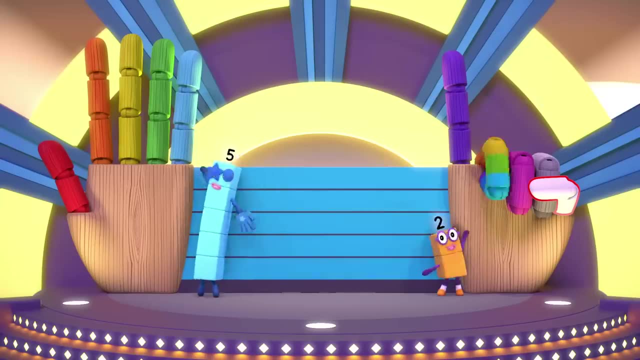 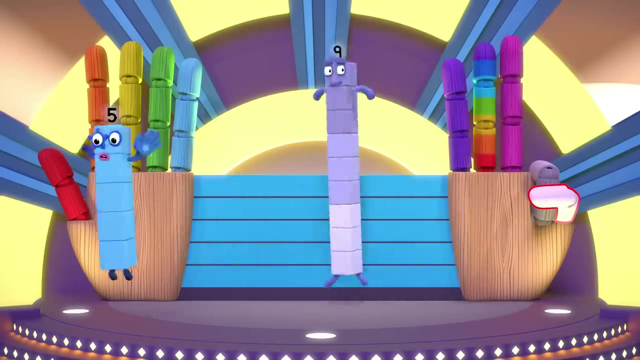 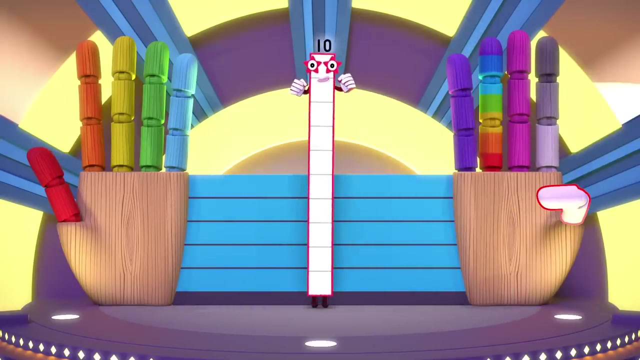 ready. i'm six, i'm five and one. i've got a five in me too. i'm seven, i'm five and two, five and two. i'm eight, i'm five and three, five and three, i'm nine, i'm five and four, five and four and i'm ten. 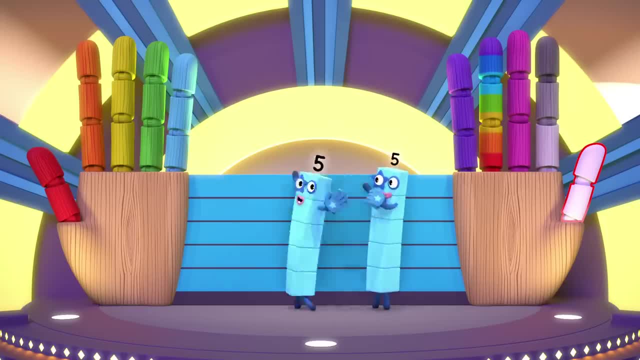 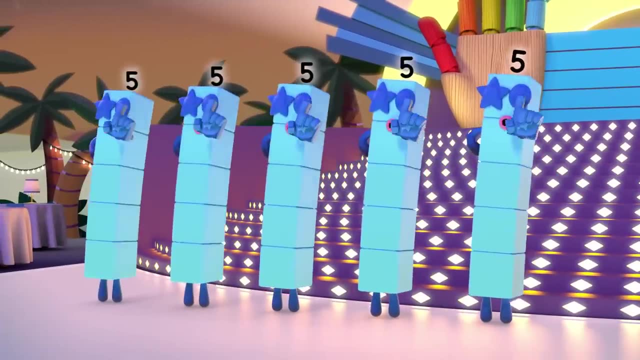 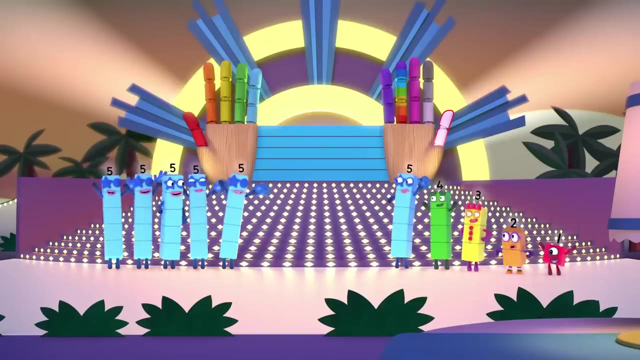 i'm five and another five, high five, five and five. hey look, five, fives, high five. ooh, to the side up above, don't go too slow. hey wait, there are loads of fives here now, but we're a, six, seven, eight, nine and ten. we can't start the dance until. 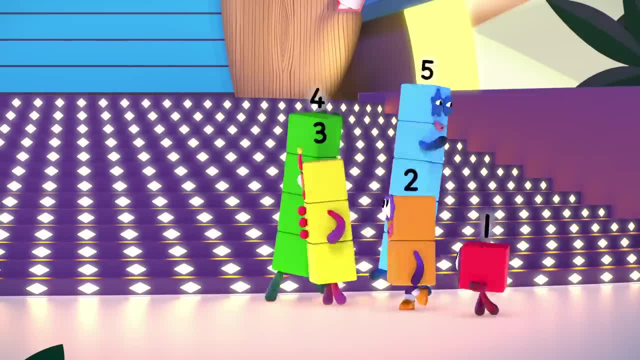 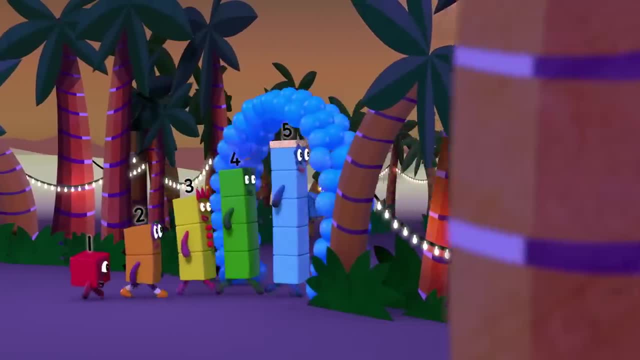 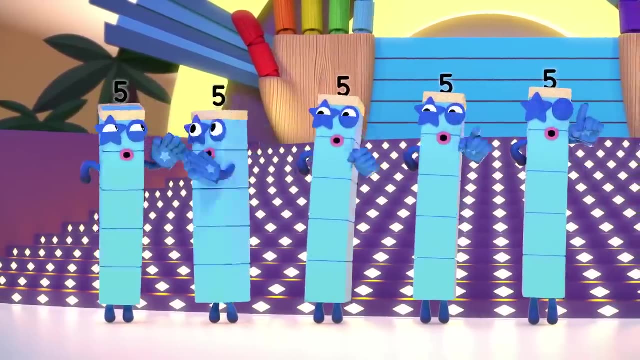 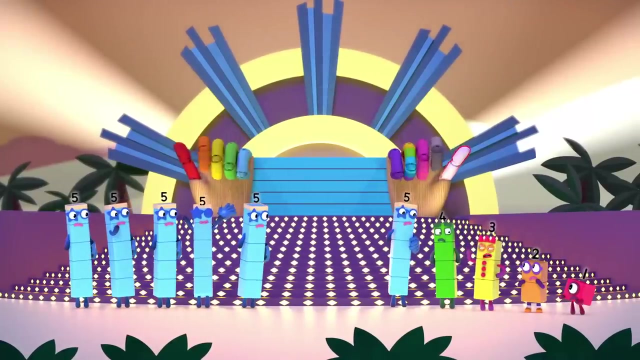 all my friends are here. let's go and find them. wow, this must be the two palms. oh, wow, and look, five, fives, oh, high five, ooh, to the side up above. don't go too slow. wait, wait, wait. where are six, seven, eight, nine and ten? 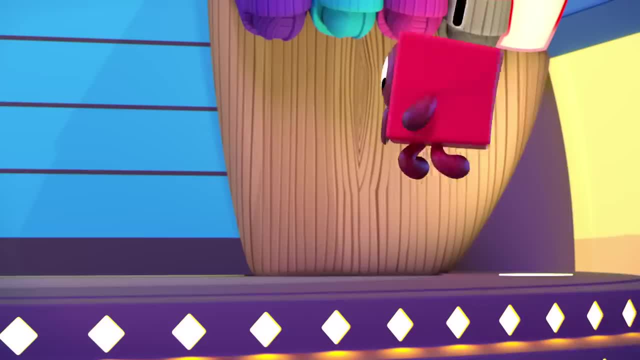 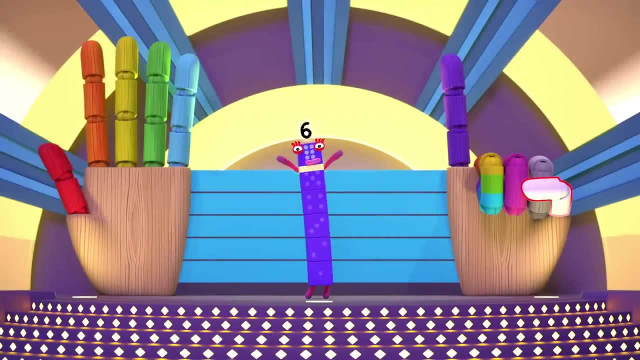 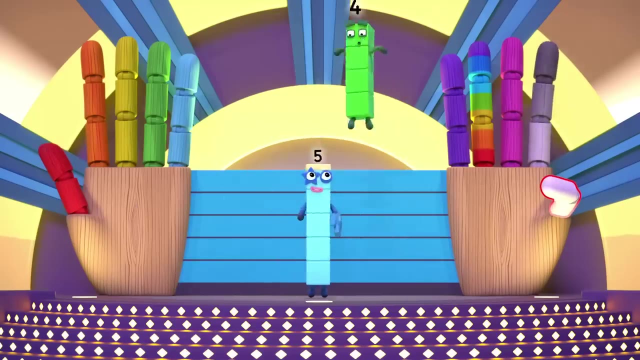 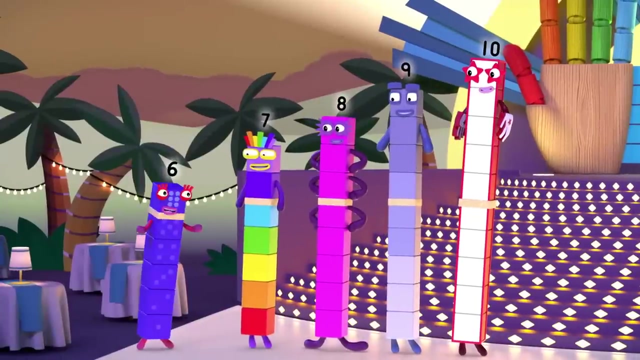 we can't start until all my friends are here. hey, we can make friends ready. five and one is six. five and two is seven. five and three is eight. five and four is nine. high five, five and another five is ten. now let's get this party started. 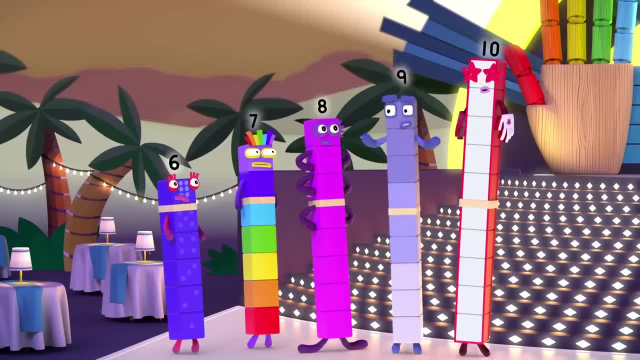 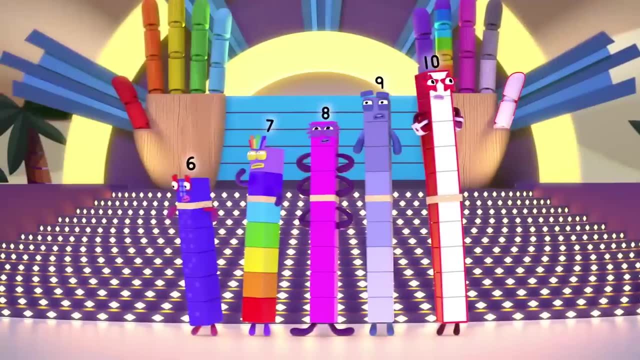 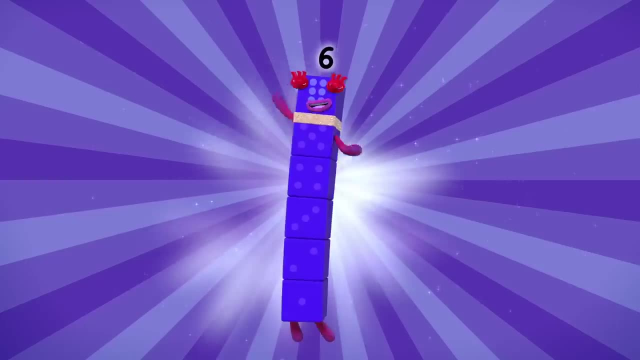 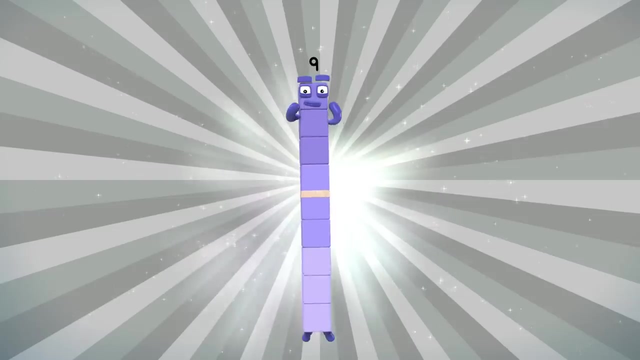 hold on. we're a one, two, three, four and five. where are they? look here, above the sparkly line. do you see who i see ready? i'm six. i'm five and one. i'm seven. i'm five and two. i'm eight. i'm five and three. 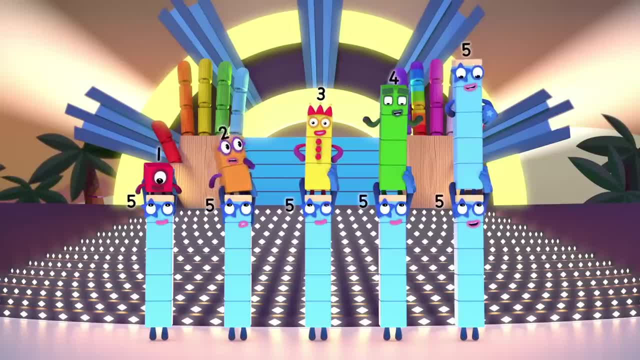 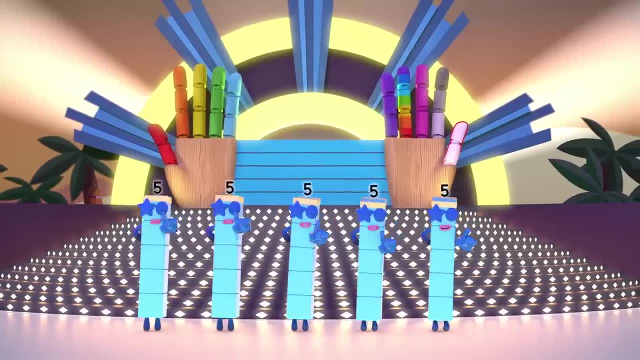 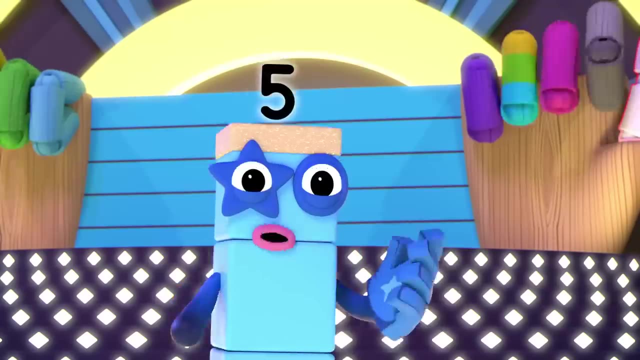 i'm nine, i'm five and four, i'm ten, i'm five and another five high five. hey wait, where are six, seven, eight, nine and ten? let's go and find them, high five. ooh, you'll see them then ready. five and one is six. five and two is seven. 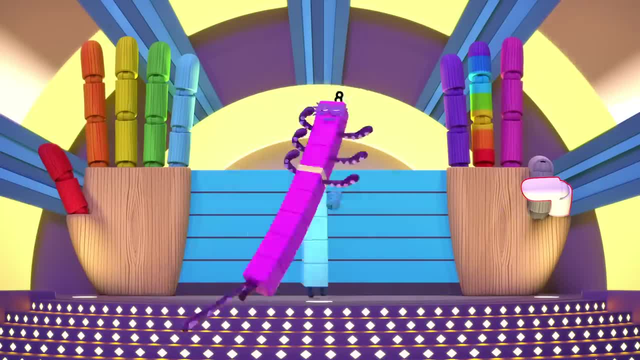 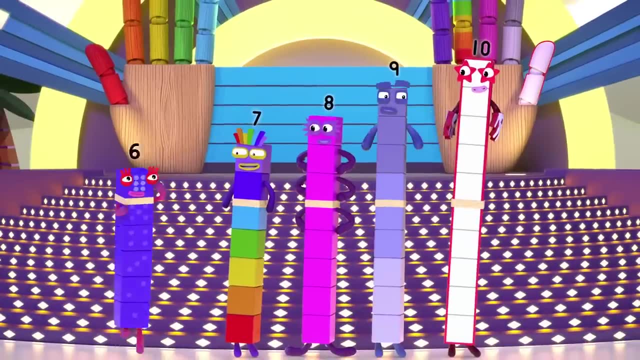 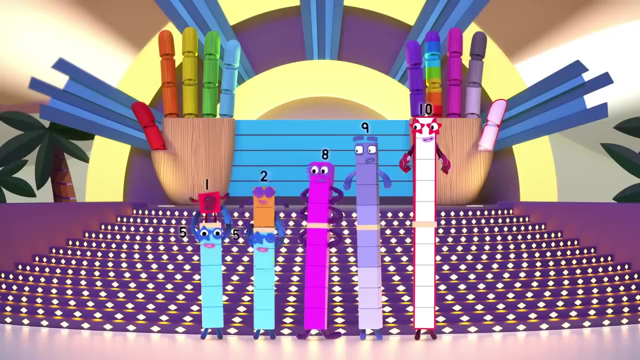 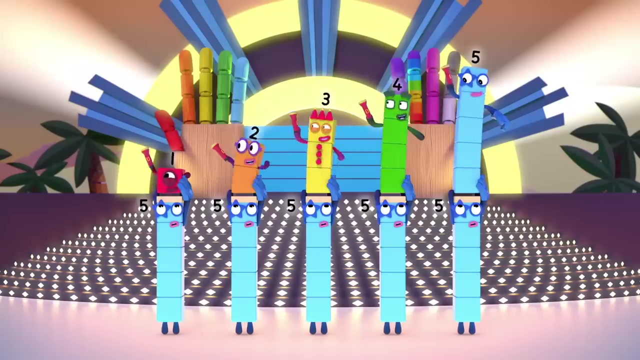 five and three is eight. five and four is nine, high five: five and another five is ten. now let's get this party started. hold on, we're a one to five: one, two, three, four, five and another five high five. hey wait, let's go look for them again. 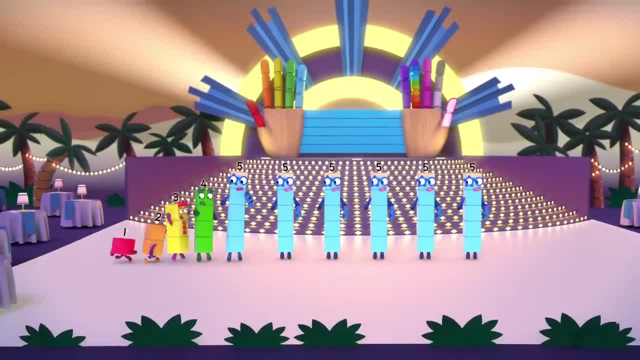 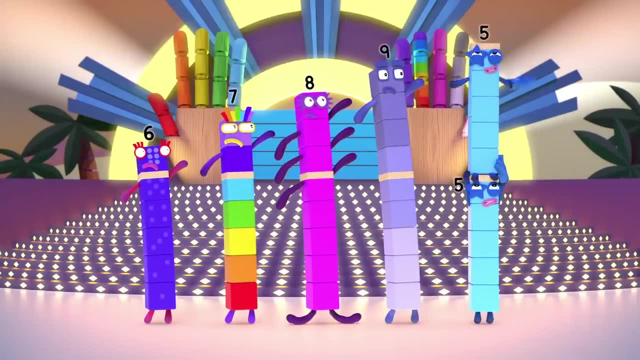 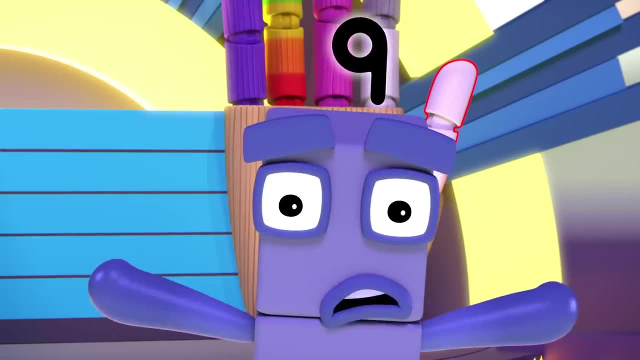 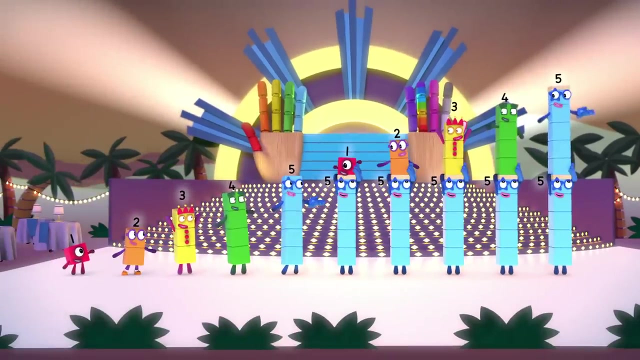 high five. ooh, we're a, we're a six to ten. why don't you jump up again? six, seven, eight, nine, five and another five is ten. let's get this party started. hold on. we're a one to five. there we are. we're a, we're a six to ten. 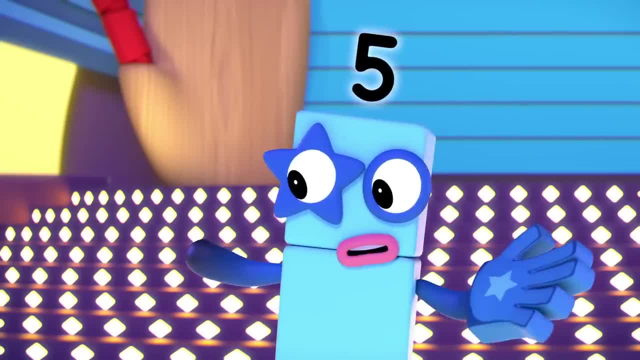 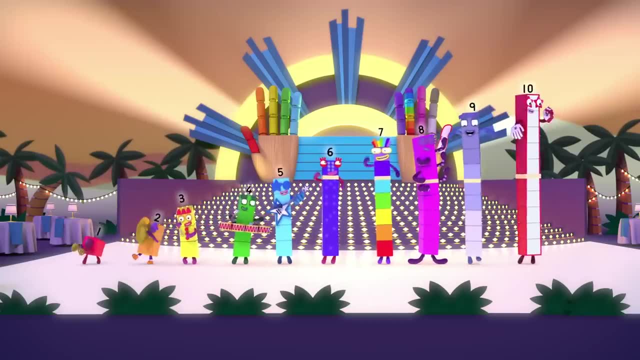 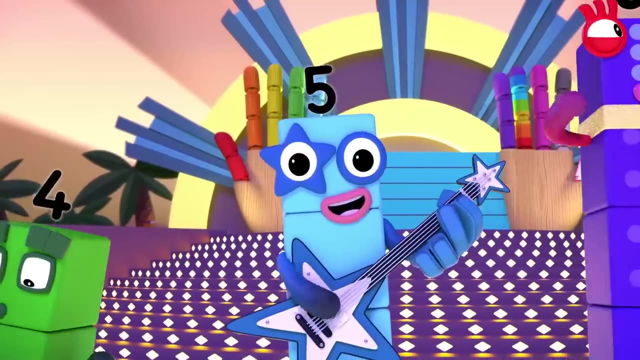 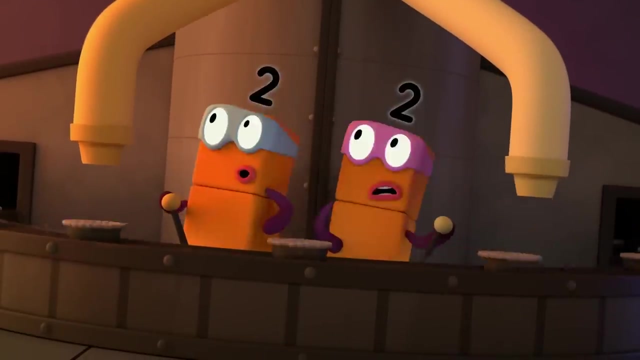 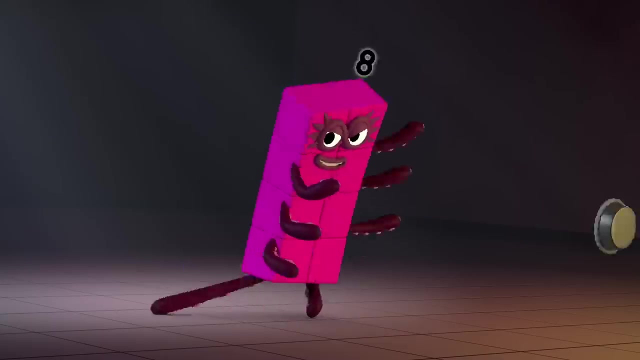 here we are. my friends are all here. let's get this party started. high five, ooh, to the side up above. don't low too slow. high five, surprise, surprise, custard pies. oops, your days of naughtiness are numbered. terrible twos. one, two, three. 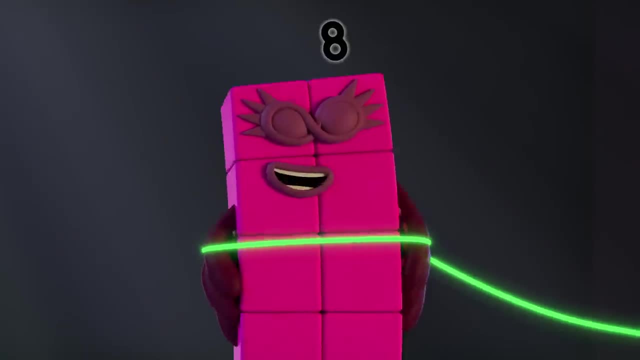 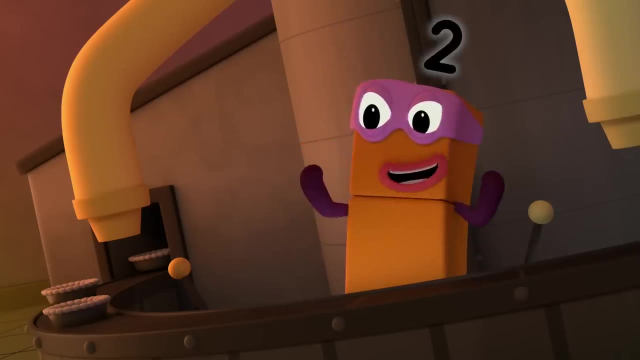 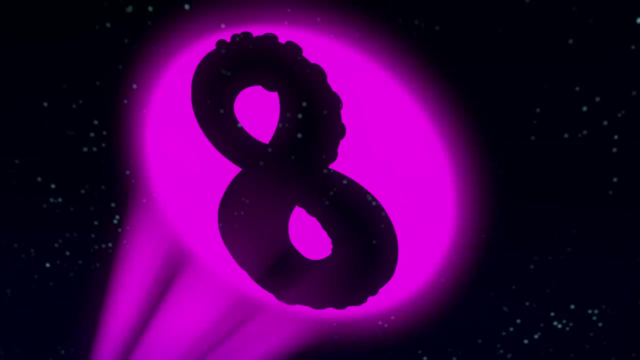 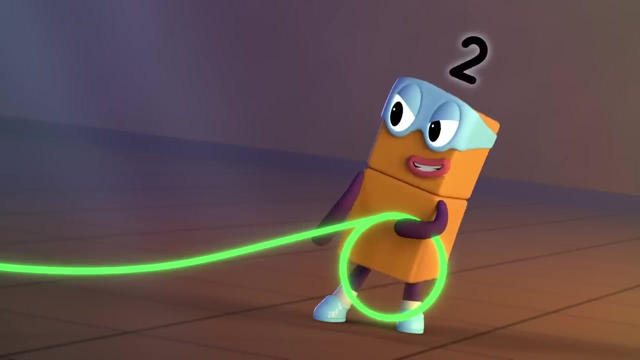 got you octoblock break rope. that rope is made from pure octonite. your powers are useless? maybe so, but i can still do this. the octo signal. my friends will be here any moment and they will fall straight into our troublesome traps. don't be so. 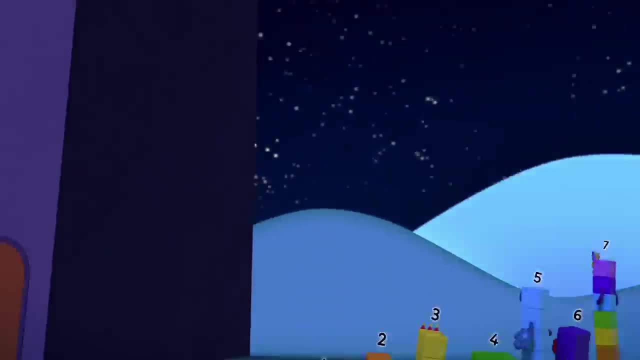 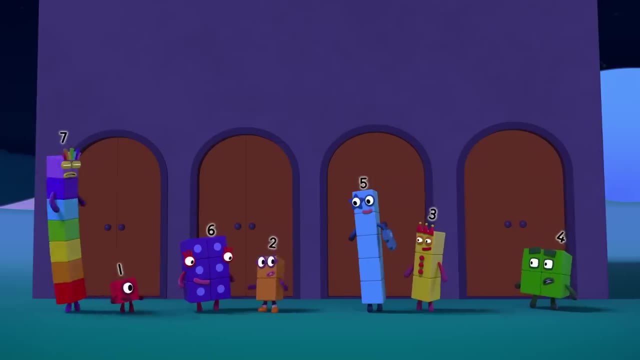 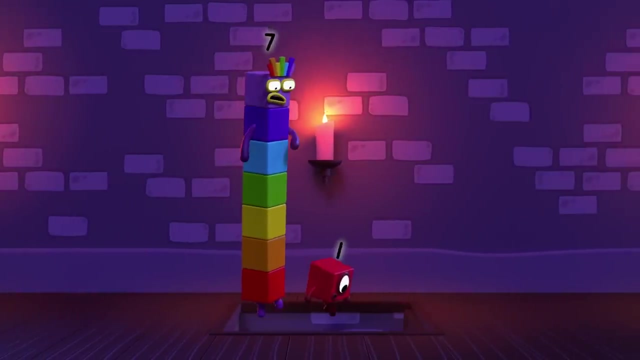 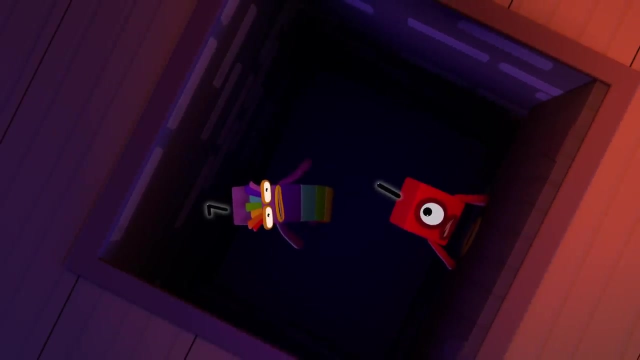 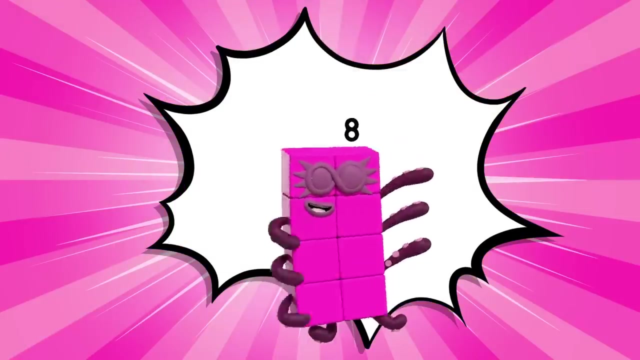 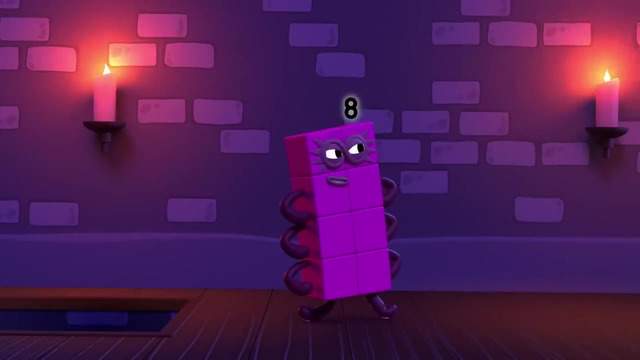 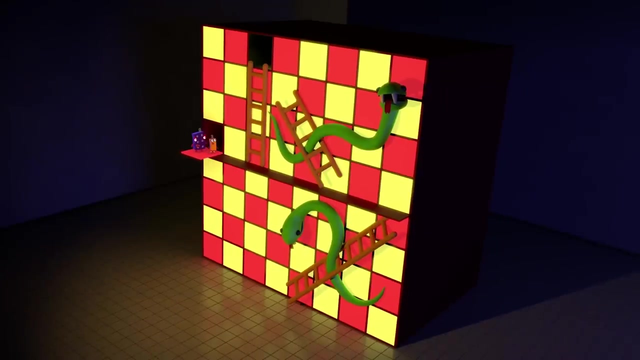 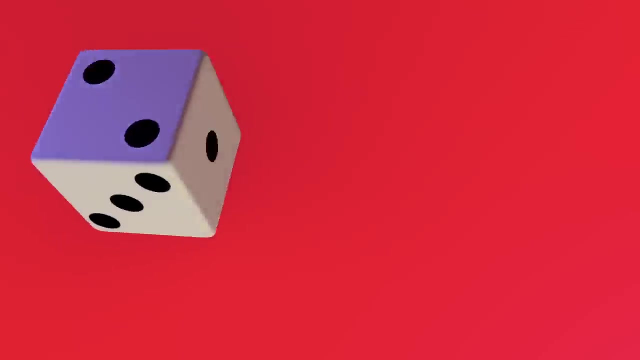 sure, octoblock leads us splitter in here. that wasn't very lucky, but that was seven. one equals eight. octoblock: leap one, two, three, four, five, six, seven, eight. leap snakes and ladders, my favorite game let's play together: two, one, two, hey, someone's. 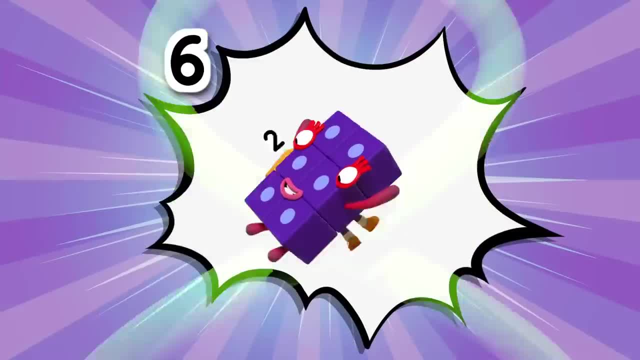 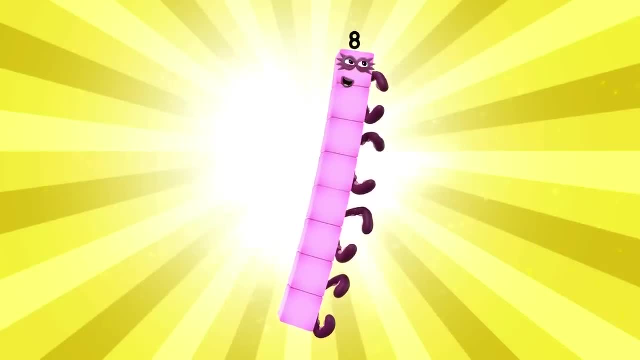 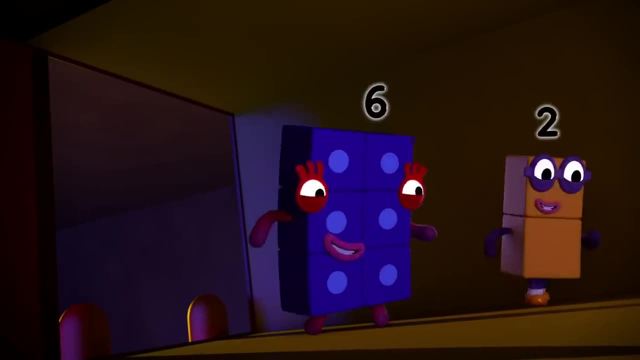 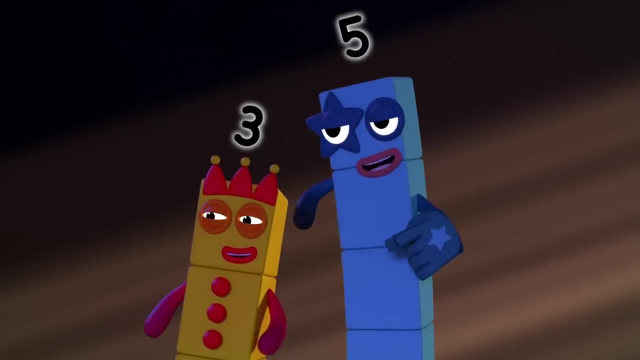 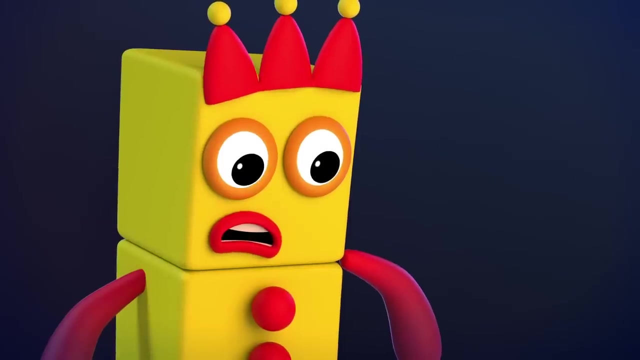 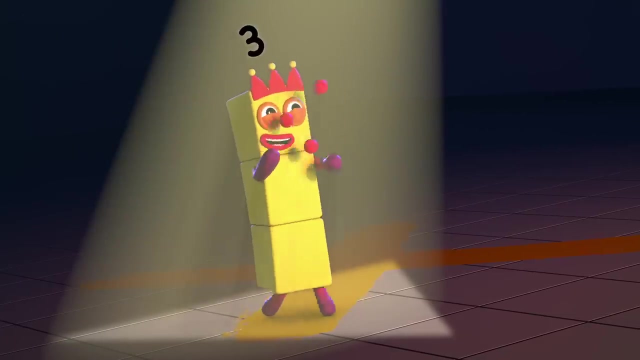 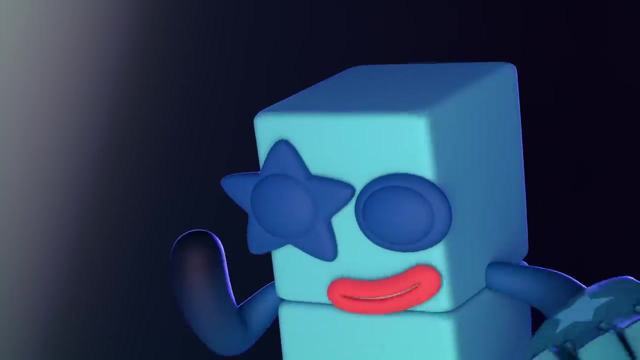 cheating. six plus two equals eight. octoblock climb. one, two, three, four, five, six, seven, eight climb. they won't catch us that easily. don't walk under the cage. i could just resist at three. i'm a star. i'm a star. hey, i wasn't finished. 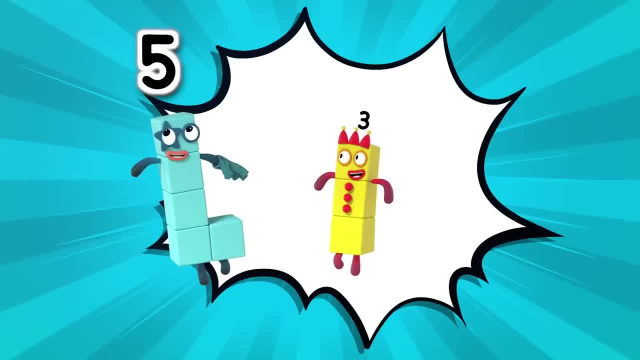 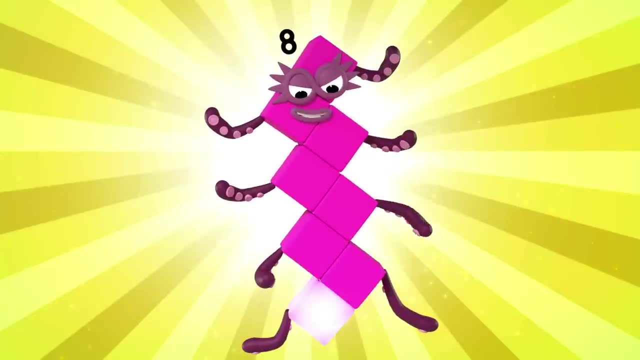 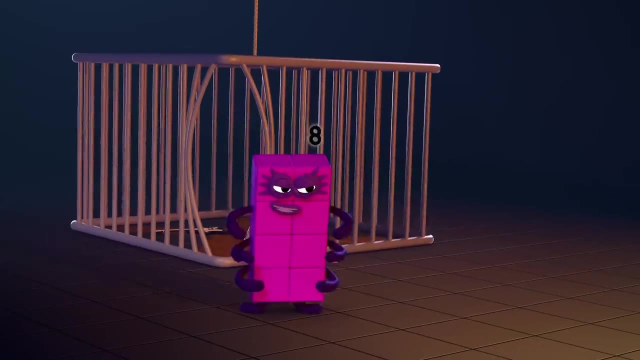 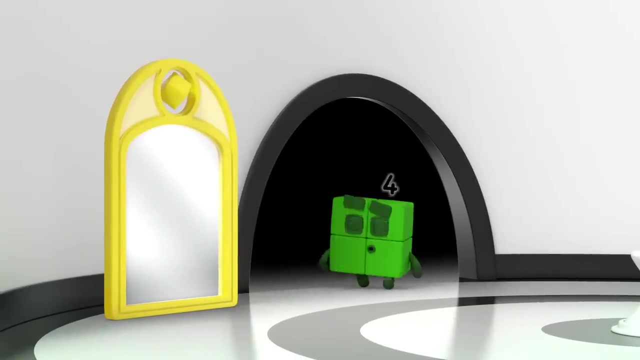 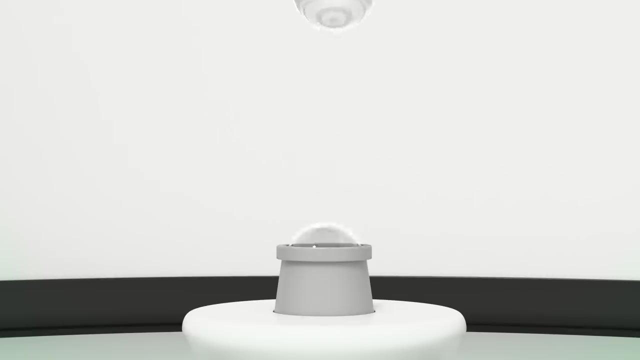 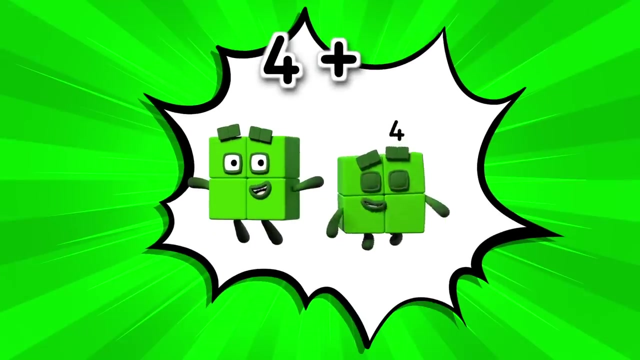 grand finale: five plus three equals eight, huh, octoblock. one, two, three, four, five, six, seven, eight. one, two, three, four, five, six, seven, eight. one, two, three, four, five, six, seven, eight. hello, hello, oh, round things, it's got us. four plus four equals eight, octoblock. 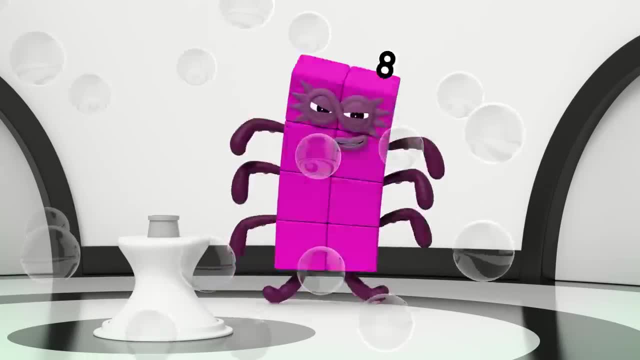 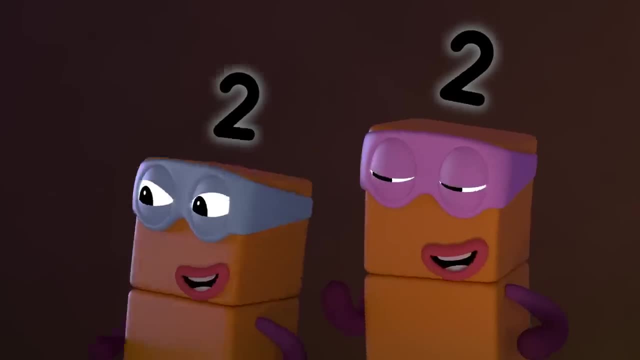 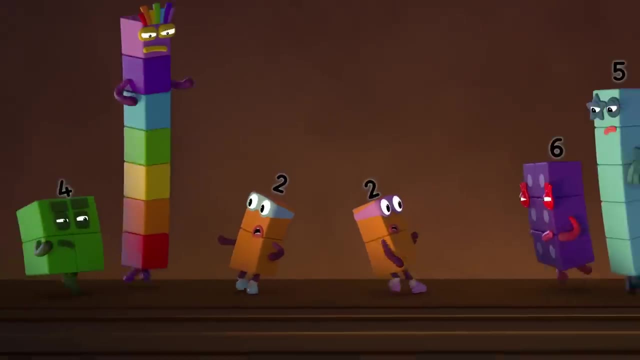 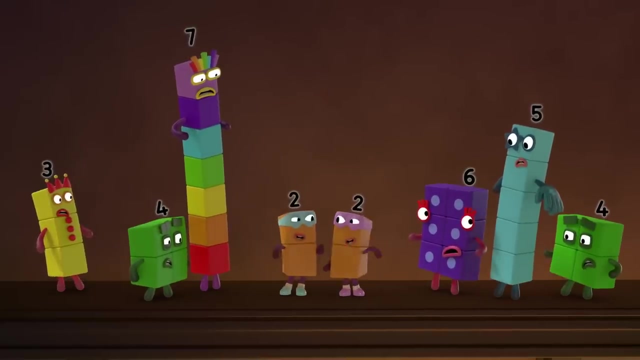 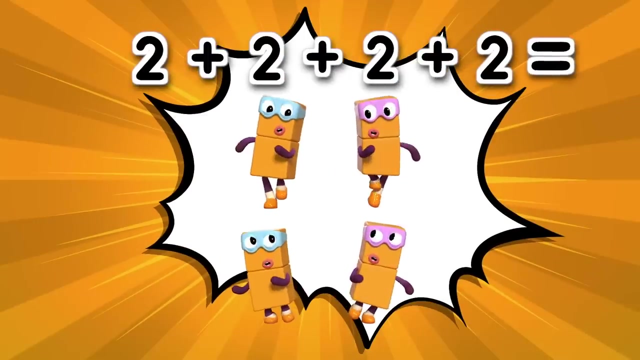 one, two, three, four, five, six, seven, eight pop, prepare to be pied spider block. stop right there. we have you outnumbered. maybe so, but we've still got a trick or two up our sleeves. two plus two plus two plus two equals eight. oh, four terrible twos. 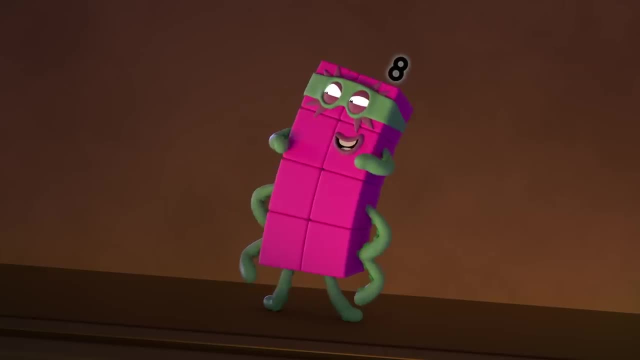 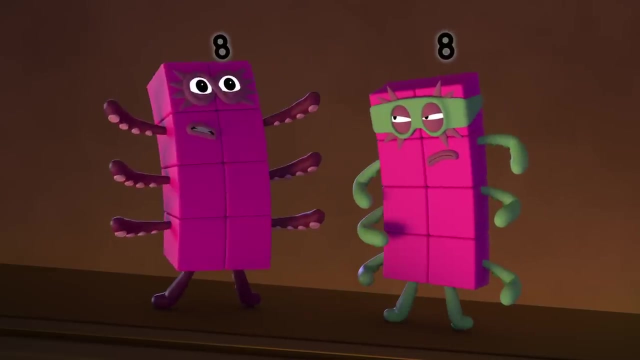 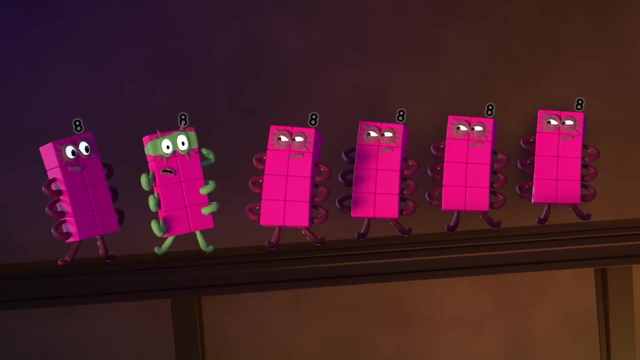 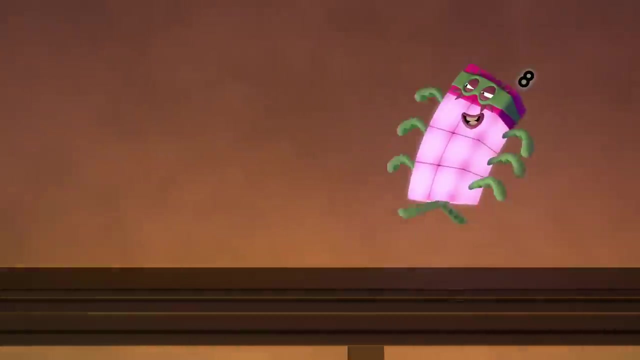 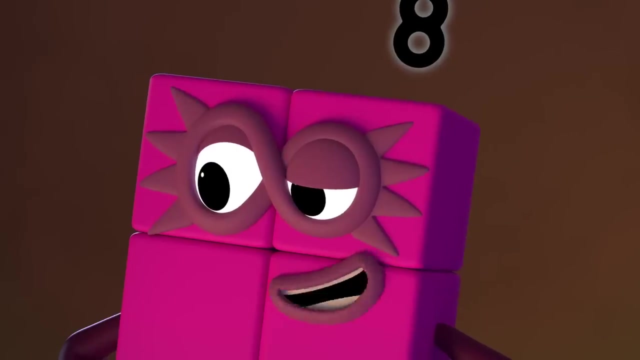 make one octonauty. you've met your match. octoblock, don't count on it. octoblocks assemble. your number is up. you'll have to catch me first. octonauty escape. eight, seven, six, five, four, three, two, one escape. oh, i spy with my. 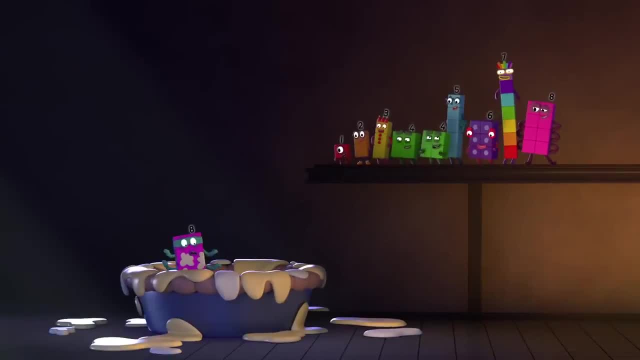 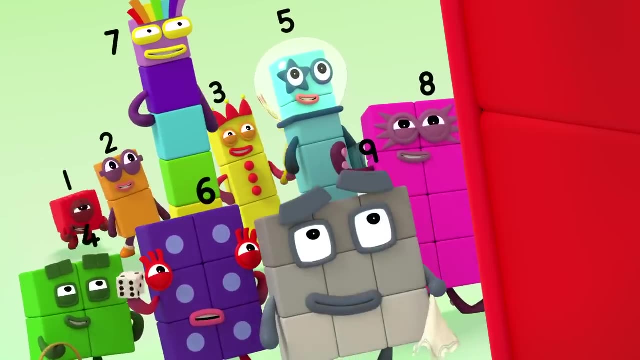 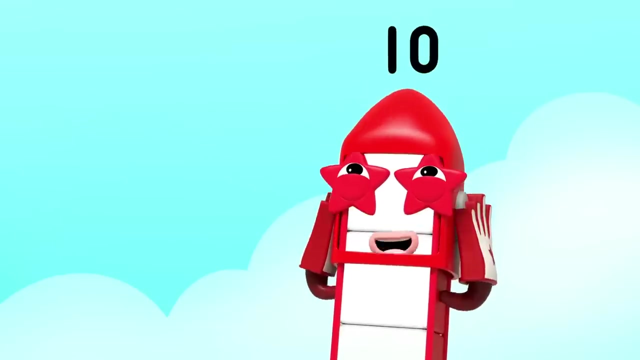 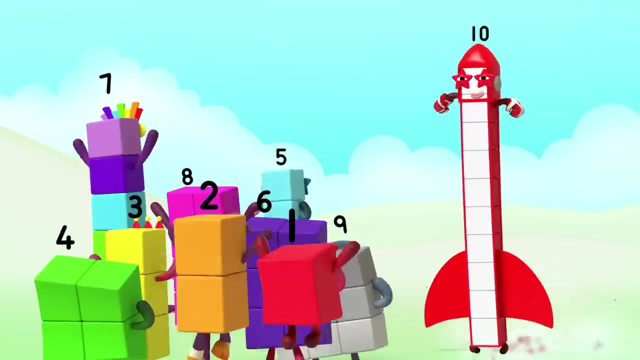 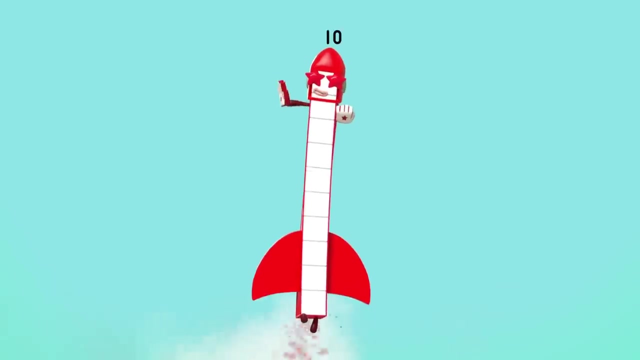 little pie, a very naughty number block. what should we do today? i said, please, please, oh okay, let's do everything. everything, yes, ready. ten, nine, eight, seven, six, five, four, three, two, one muscles. i'm ten, ten, ten. and i'm flying through the sky. i'm ten, ten, ten. 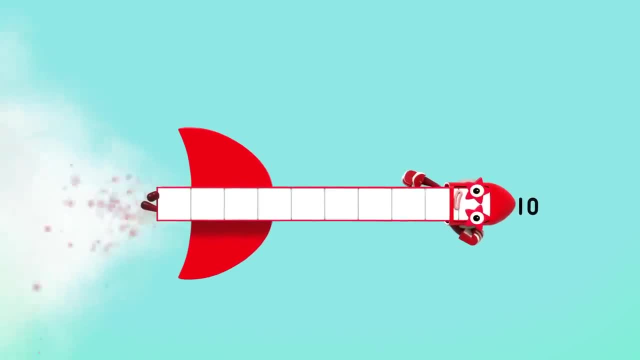 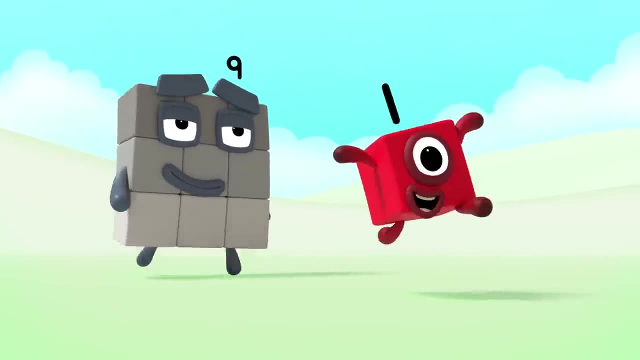 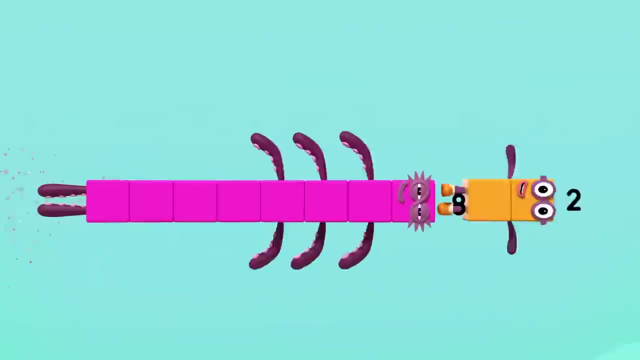 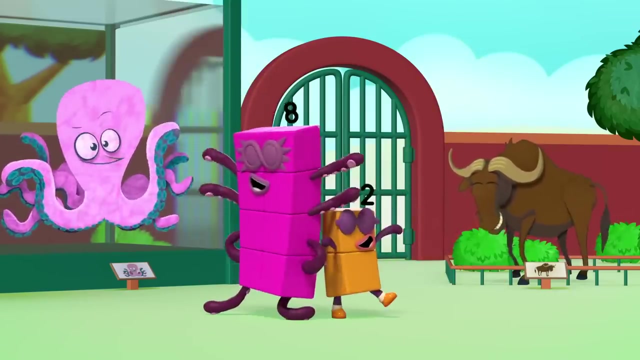 you can break me up any way you like. i can be nine plus one, going for a run trying not to sneeze, and then i'm ten, ten, ten again. i can be eight plus two, visiting the zoo, talking to the octopus and dancing with a canoe. 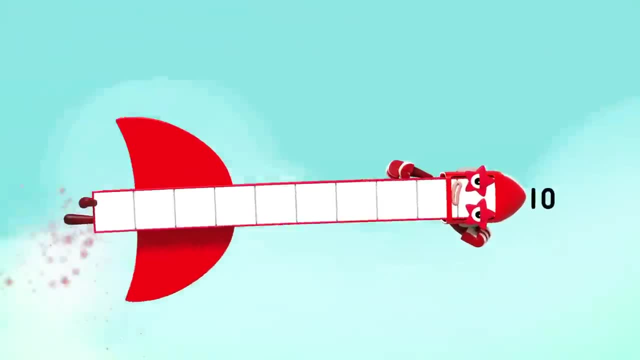 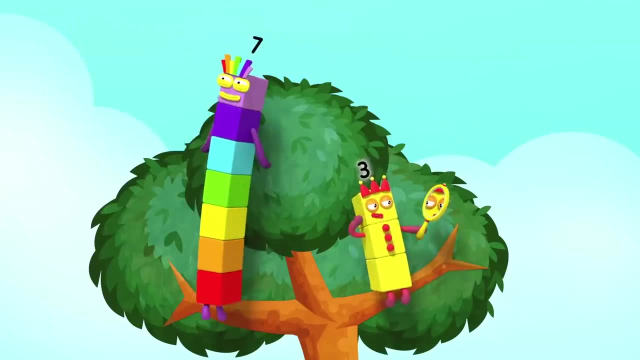 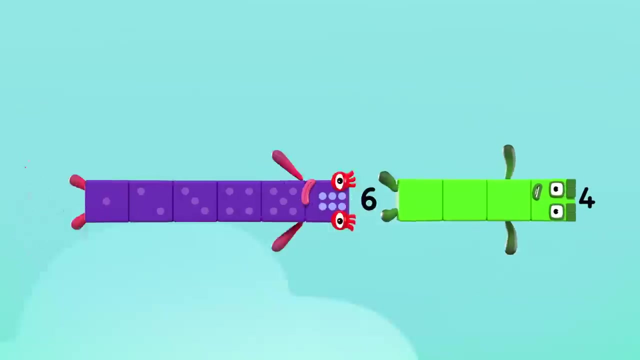 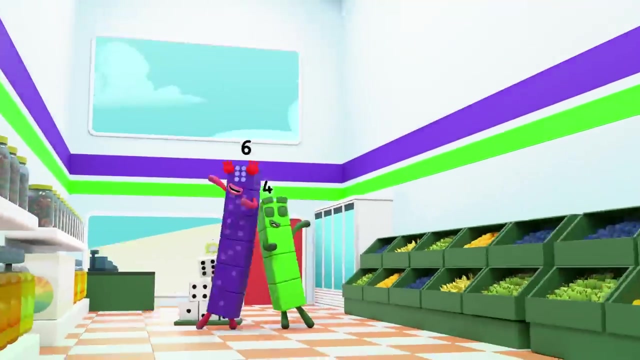 and then i'm ten, ten, ten again. i can be seven plus three, sitting in a tree making looking at me. and then i'm ten, ten, ten again. i can be six plus four shopping at the store, playing with a dice on a square tile floor, and then 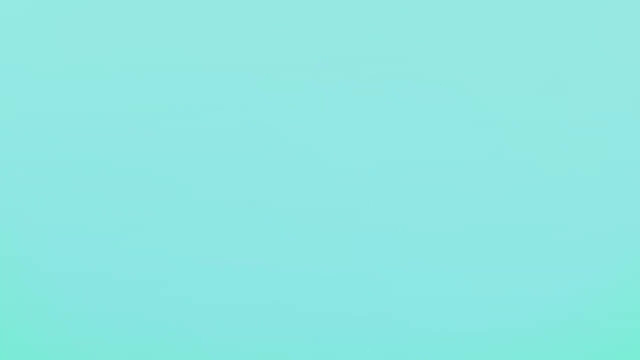 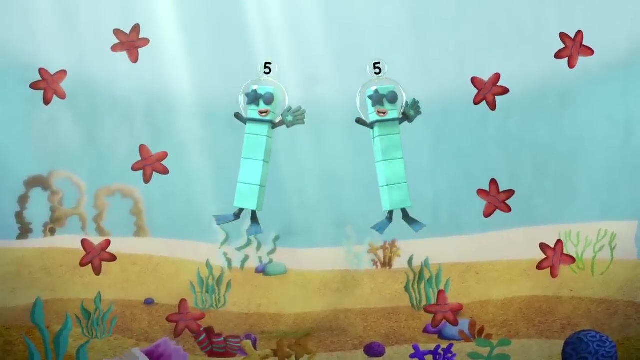 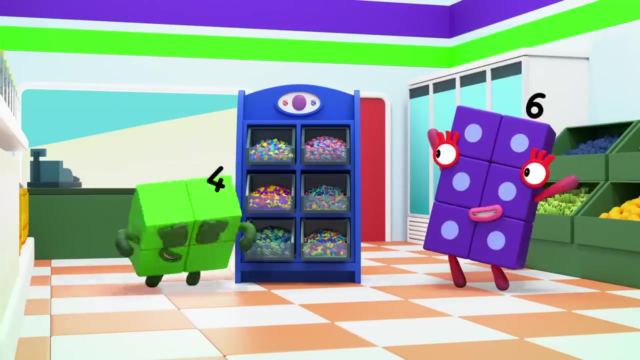 i'm ten, ten, ten again. i can be five plus five on the school dive swimming with a starfish and doing a jive. and then i'm ten, ten, ten again. i can be four plus six: pie and pick and mix, picking out the square ones and using chopsticks. 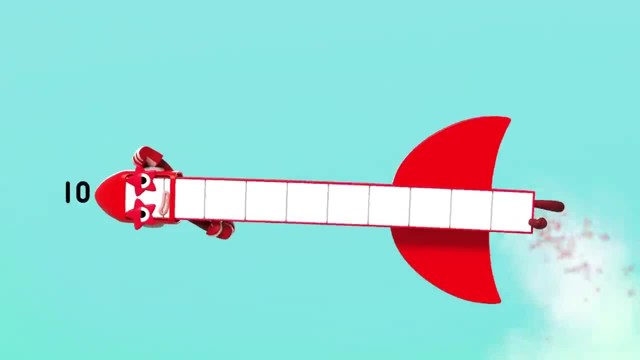 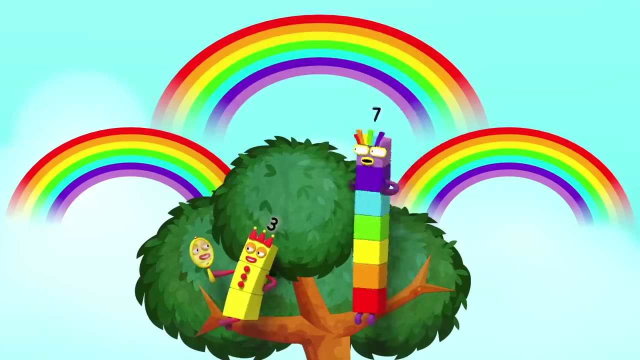 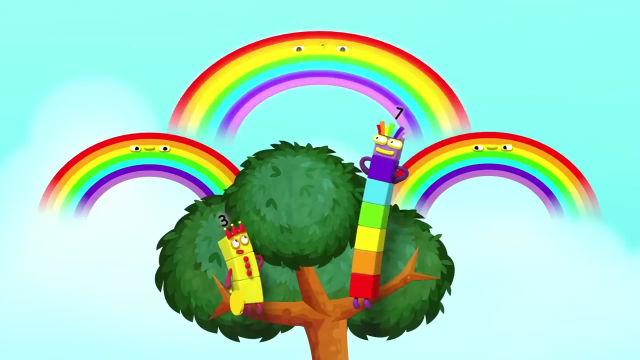 and then i'm ten, ten, ten again. i can be three plus seven, gazing up to heaven- no, looking at me- and a rainbow called kevin. kevin, and all my rainbows have names: kevin, rainbow, dina, and that's big bob. and then and then. 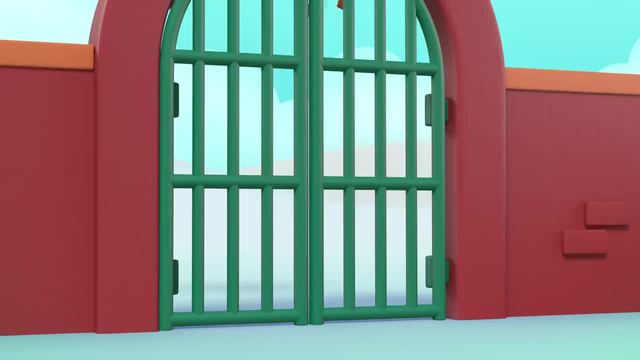 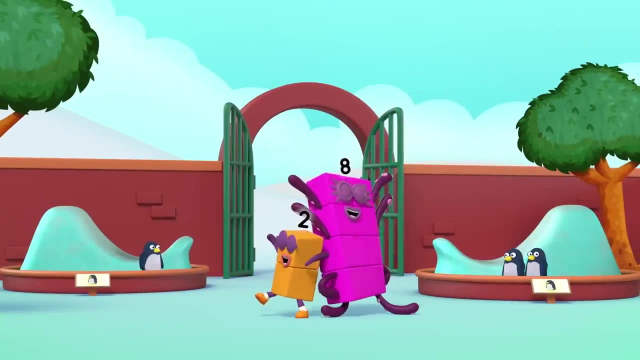 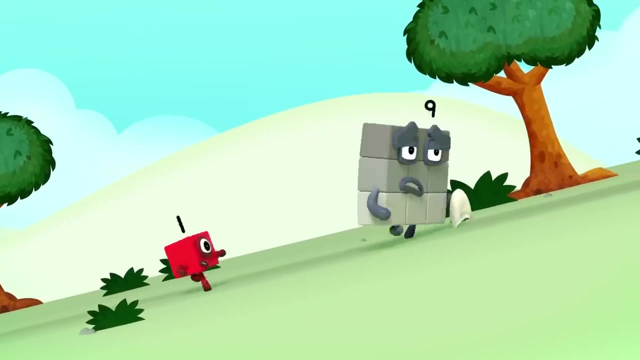 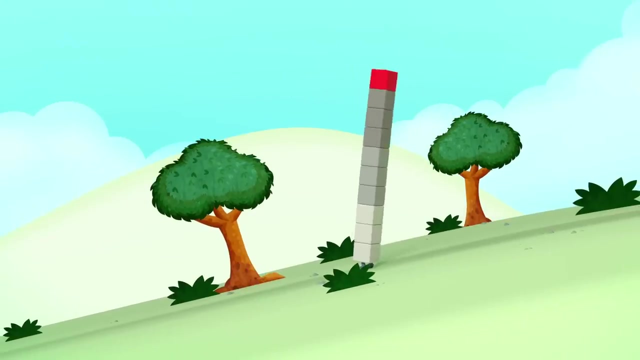 i'm ten, ten, ten again. i can be two plus eight, opening a gate, dancing with a penguin lifting heavy weights. and then i'm ten, ten, ten again. i can be one plus nine, starting on a climb, getting out of breath now, sneezing all the time. 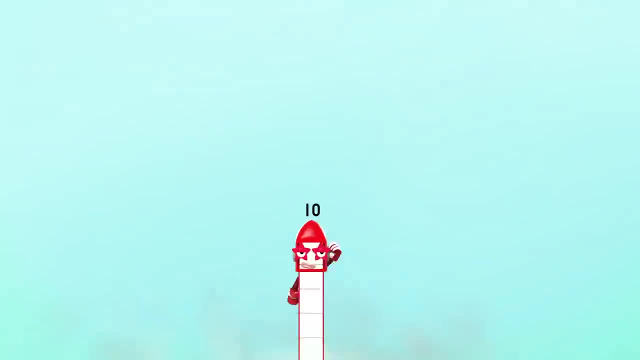 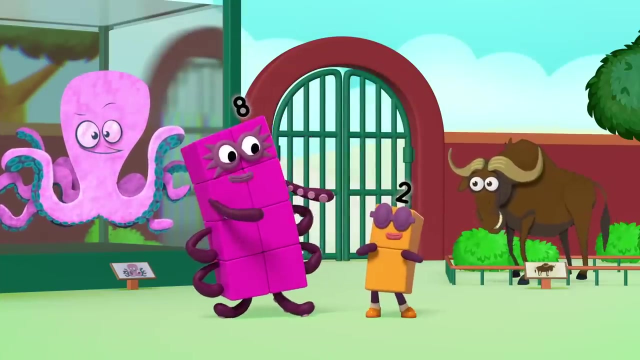 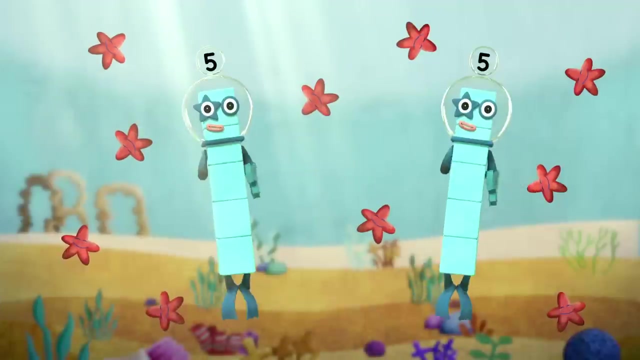 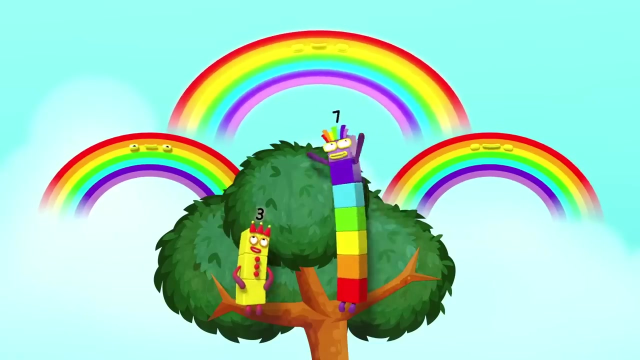 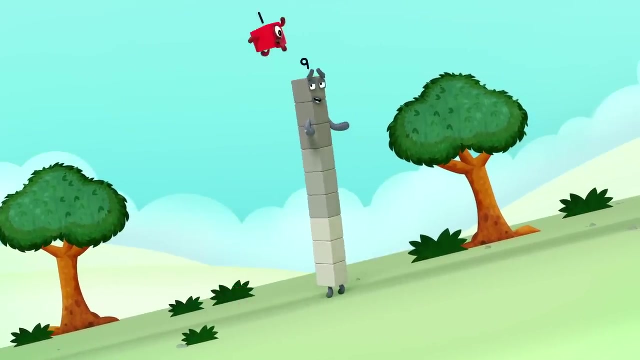 ten, ten again ten, ten, ten again again. nine plus one going for a run, eight plus two visiting the zoo, seven plus three sitting in a tree, six plus four shopping at the store, five plus five on a scuba dive. four plus six, ten again. three plus seven. 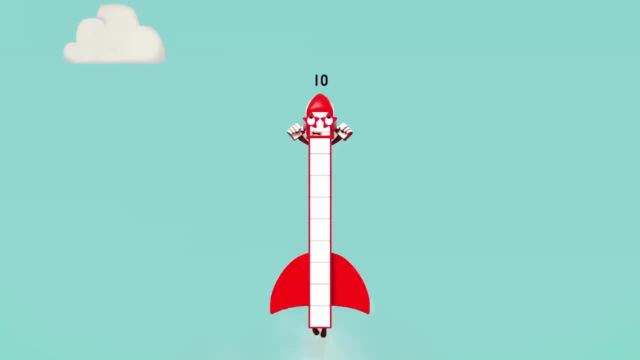 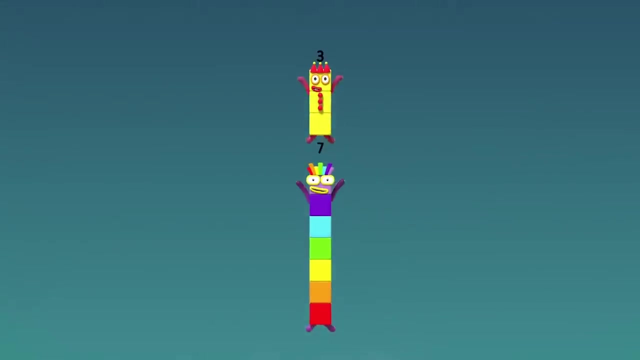 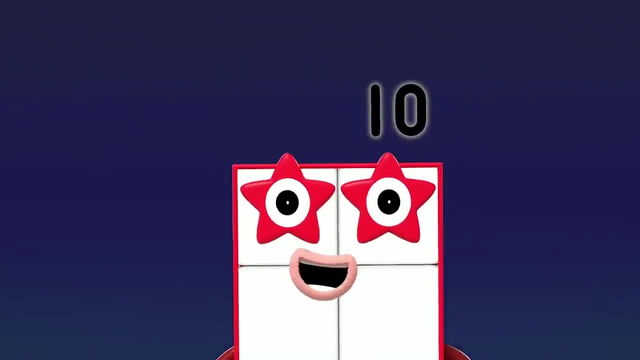 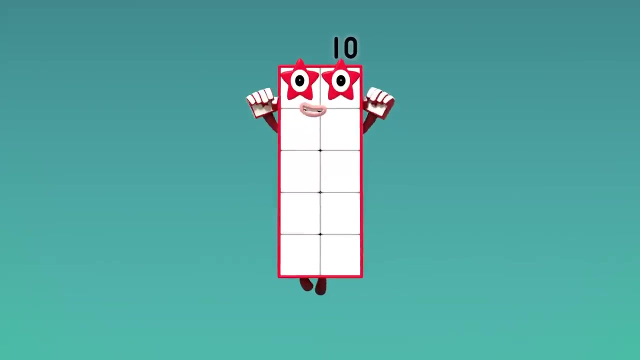 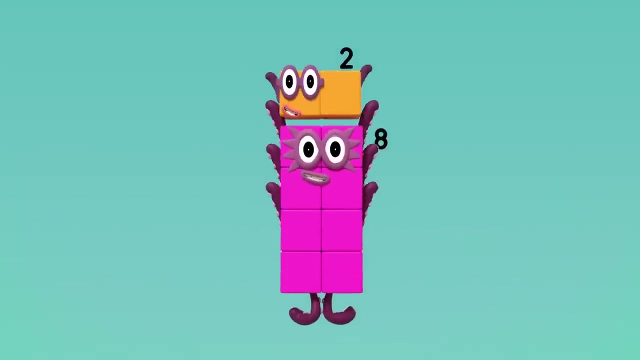 ten again two plus eight, ten again one plus nine, starting on a climb, and then i'm ten. ten. ten again again nine plus one, ten again eight plus two. ten again ten again nine plus one. ten again eight plus two. ten again seven plus three. ten again six plus four. 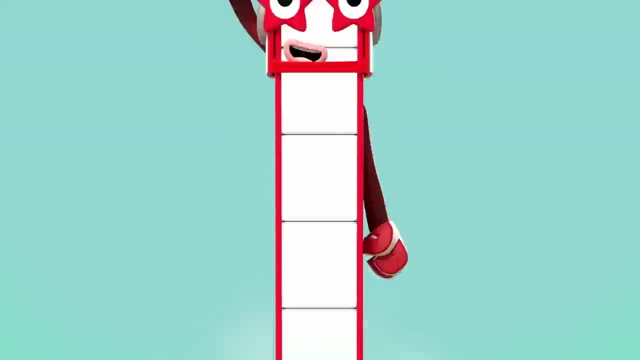 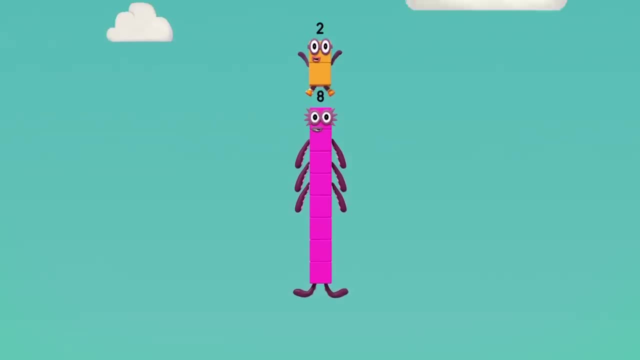 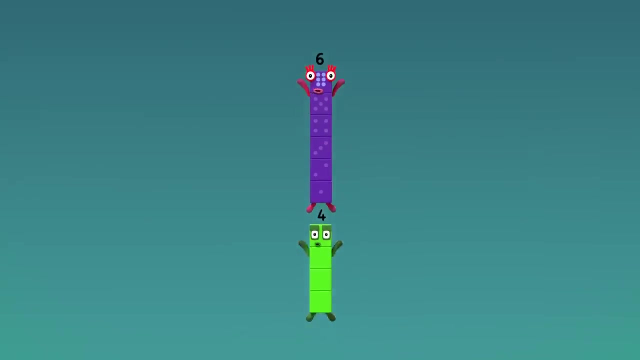 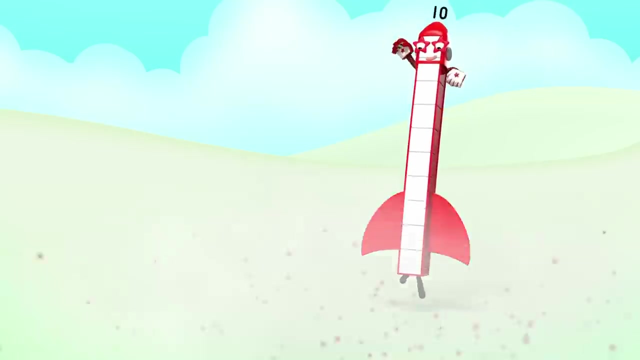 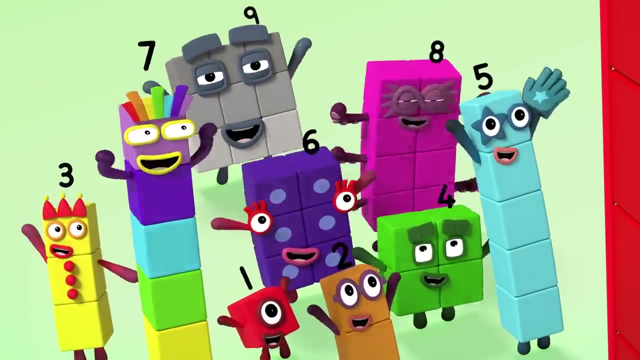 ten again, five plus five, ten again, four plus six, ten again, three plus seven, seven plus three or three plus seven, ten, six plus four or four plus six, ten, five plus five or five plus five, ten, ten, ten again. ten, ten, ten again. ten, ten ten again. and what do you want to do today? ten. 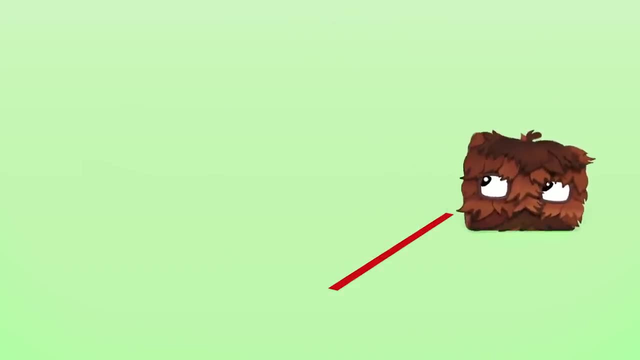 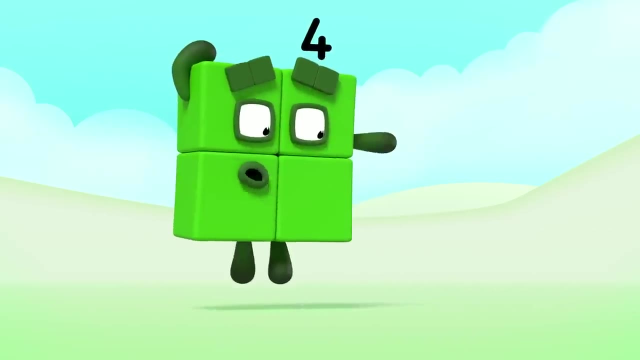 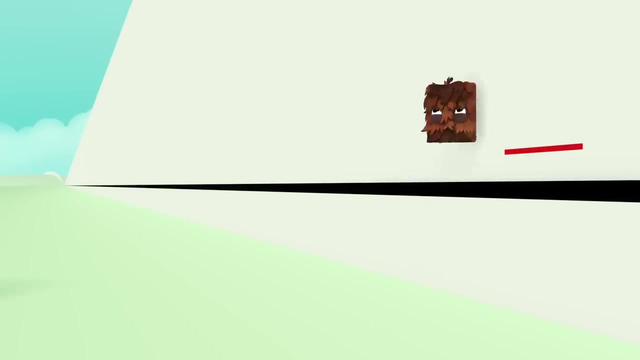 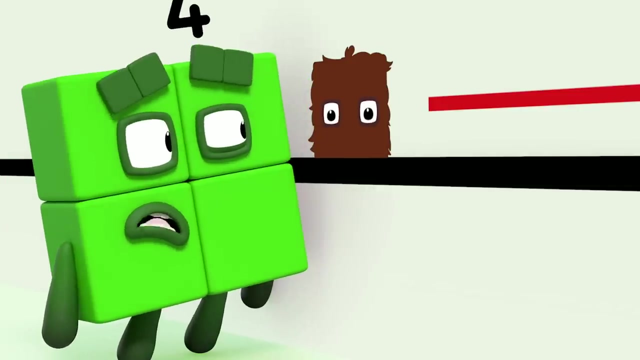 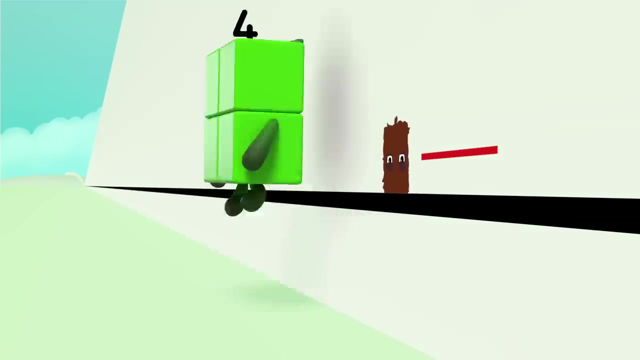 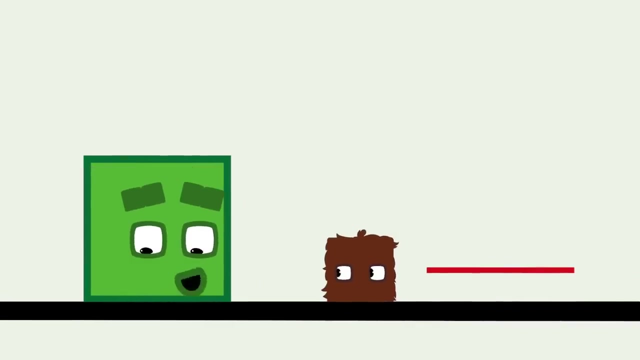 i need a nap. what is it, squirry? ooh, a stick fetch. hey, wait for me, squirry. oh, you've gone all flat. that looks like fun. hey, i'm on all flat too. i'm a square, a real square. ooh, squirry, i've a feeling we're not in numberland anymore. 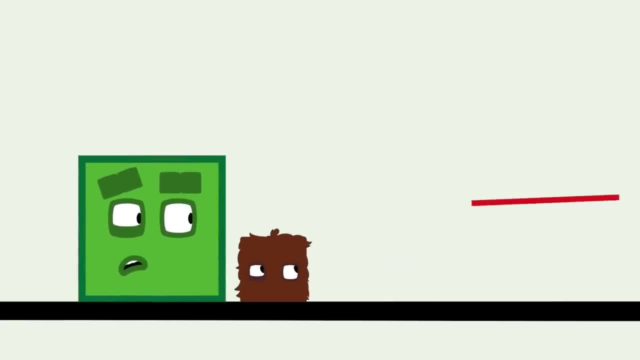 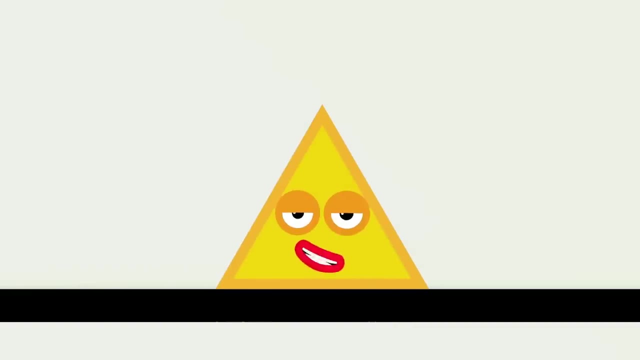 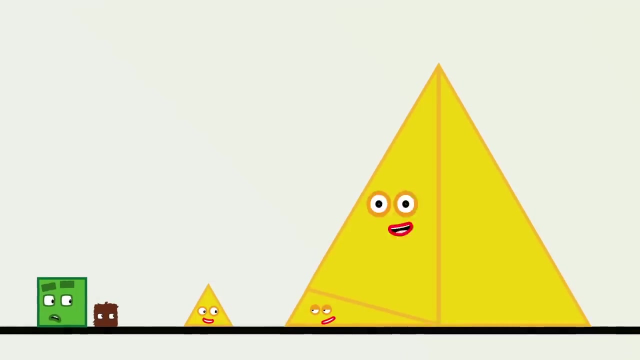 welcome to flatland, where all the flat shapes live. i am a line, one straight line, two straight lines, and when three lines join together we make a tree triangle. i've got one, two, three, three sides and one, two, three, three corners. look at me and at me. 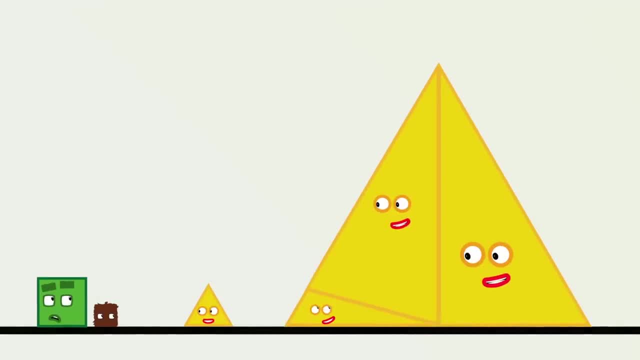 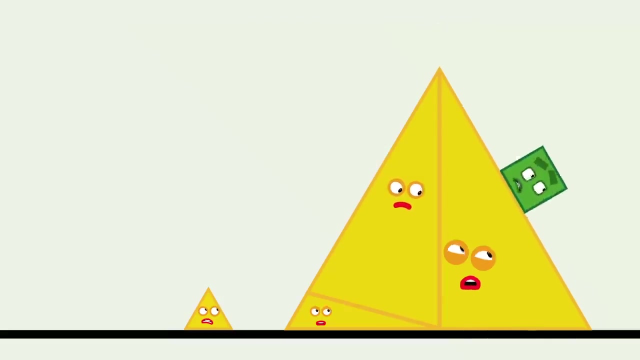 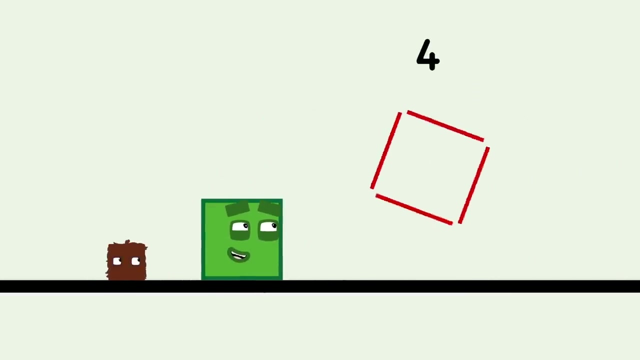 and at me, we're all triangles, wow, but you're all so different. squirry, come back. sorry, sorry, really sorry. sorry. one, two, three, four, four lines, hello, square. wait, you're not a square, no, i'm a rectangle, like you, i have four sides and four corners. 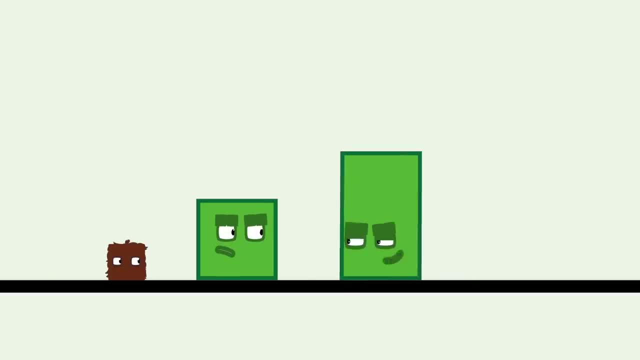 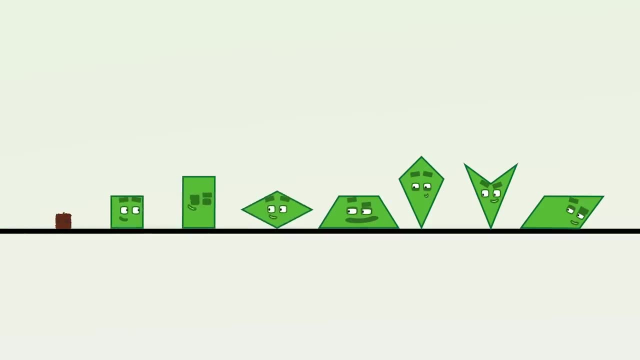 but your sides are all the same and mine are not. if i'm a surprise, you're all three turns. hello, four sided shapes. introduce yourselves. rectangle rhombus trapezium, kite square. ooh, what wonderful names and what wonderful shapes. triangle rhombus trapezium. 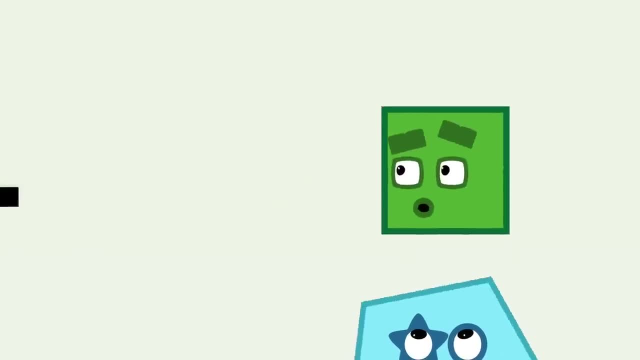 Oh, hello, Who are you? I'm a pentagon with five sides. High five, Let's have a hexagon in the mix. Count my sides and you'll find six. And, lucky me, I've got seven sides. I'm a heptagon. 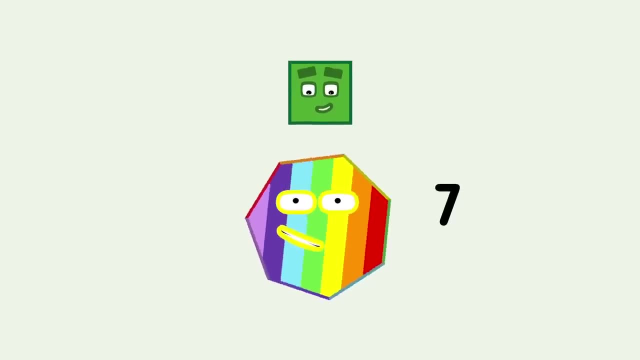 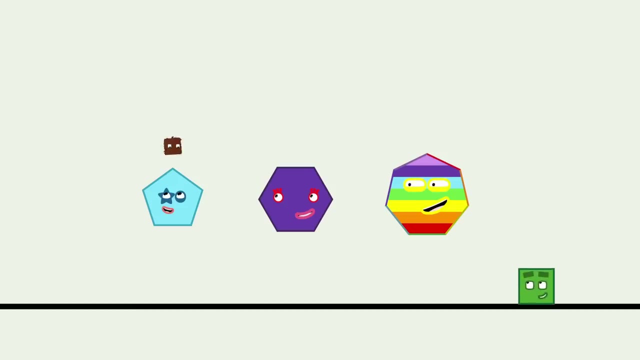 And I'm a pentagon. I've got seven sides, I'm a heptagon. A heptagon, Ooh, One, two, three, four, five sides Pentagon, Six sides Hexagon, Seven sides Heptagon. 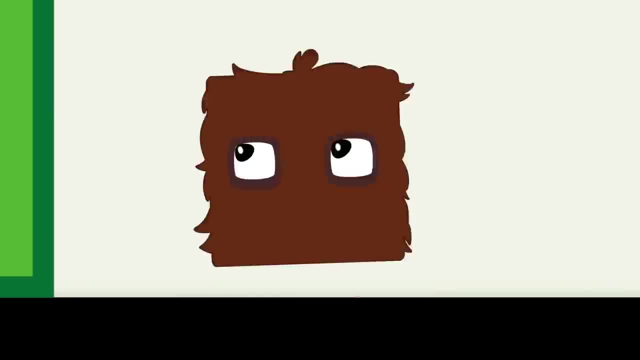 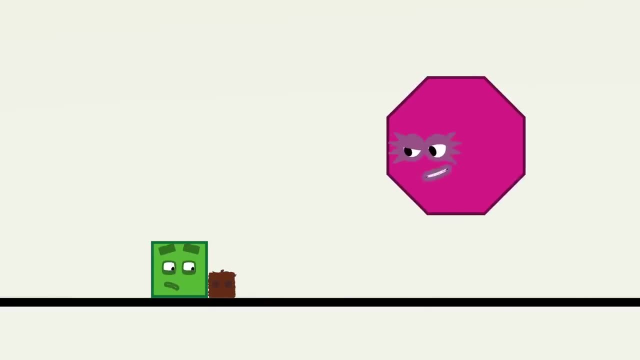 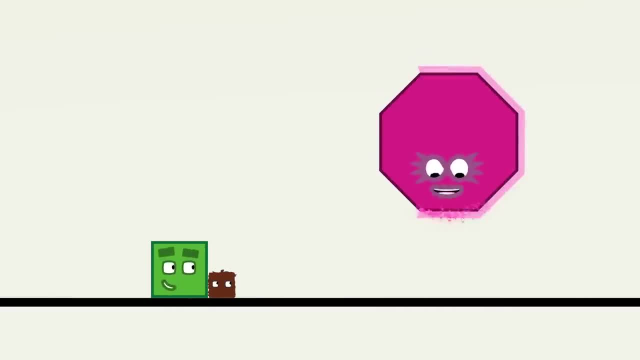 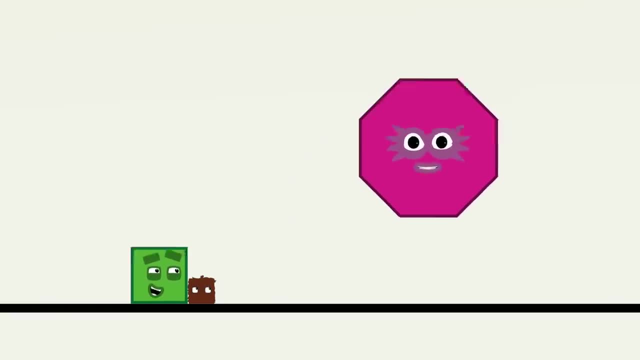 Octagon is here: One, two, three, four, five, six, seven, eight, Eight sides. I will get you home, Octagon, make an eight-sided flying basket. One, two, three, four, five, six, seven, eight. 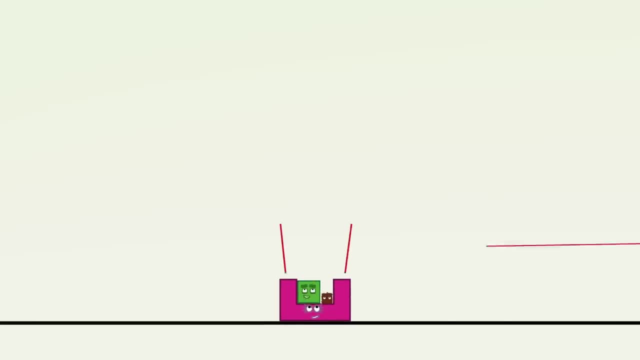 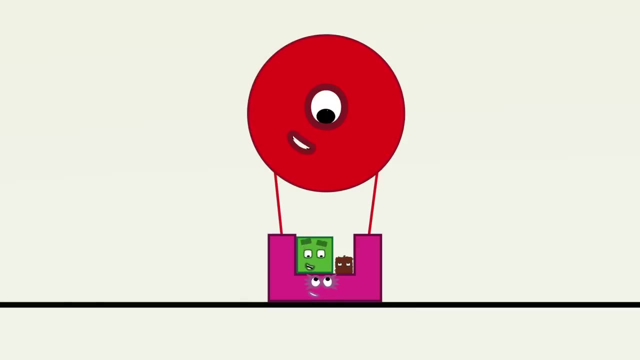 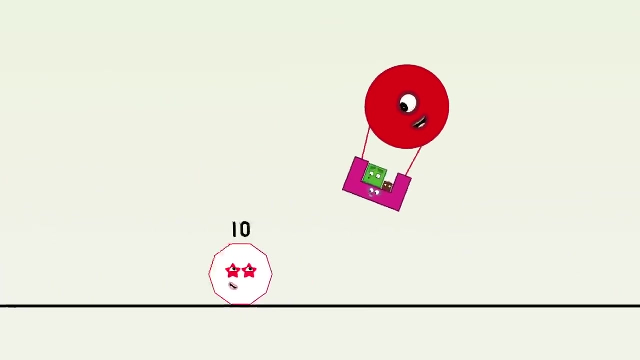 Basket. I'm a circle. I have just one curved edge. Hold tight, folks, Here we go, Whoa, whoa, hey, Ooh, Wow. Goodbye, new friends. I'm me again And you're you. 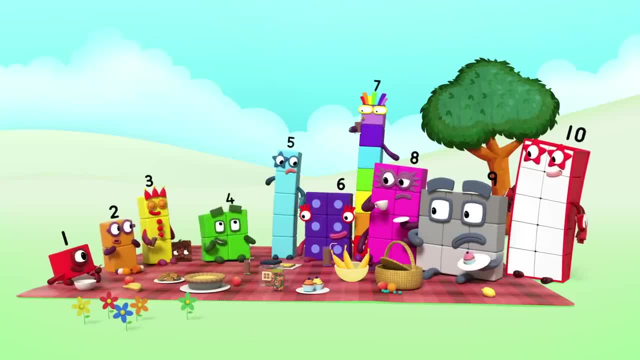 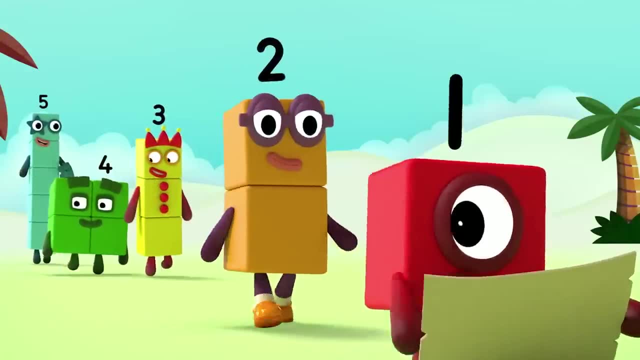 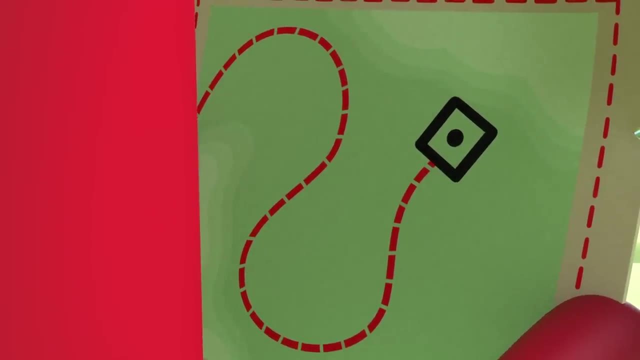 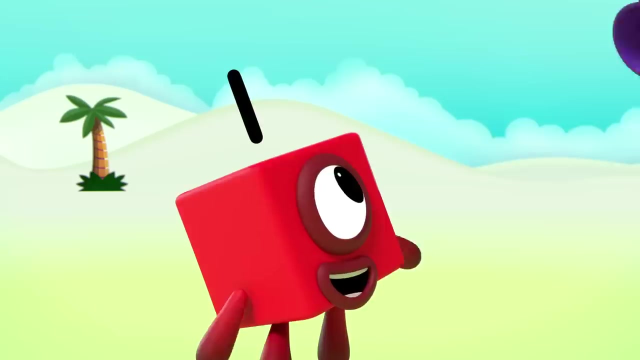 We went to Flatland and triangles were there and a rectangle and a pentagon And I was a real square. Yay, Oh, If the map is right, the Pattern Palace should be right here. Welcome to the Pattern Palace, where you can play all day. 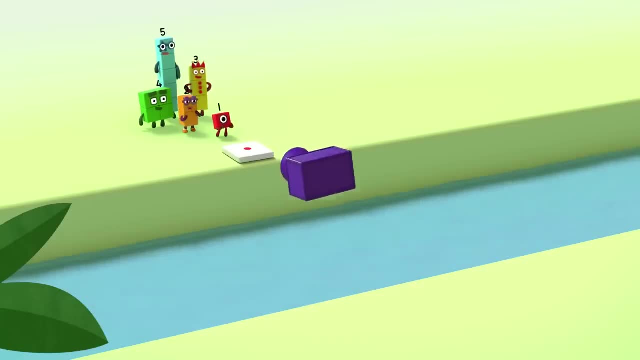 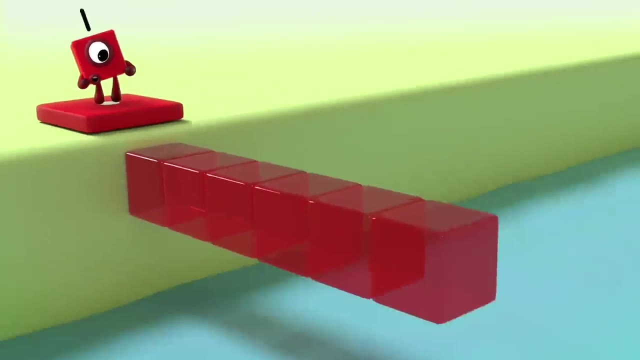 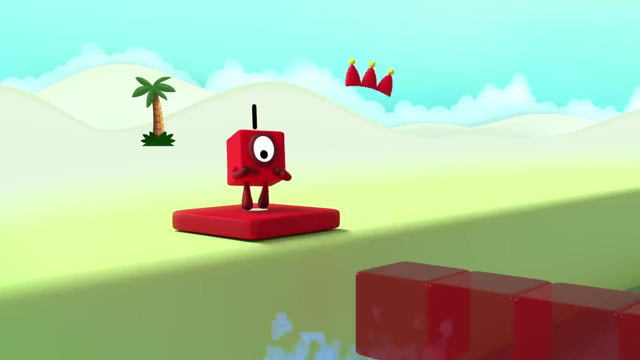 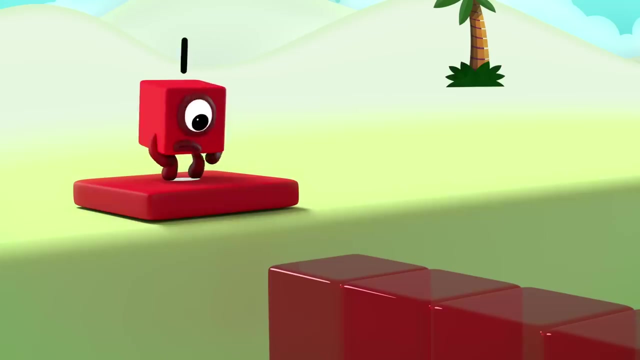 But first you must cross the Pattern Paths. Be brave and skip this way. Follow the pattern. Oh, here I come, Oh, Oh, Oh, Oh, Oh. What happened there? Um, The blocks are red, like me, so maybe I should go first. 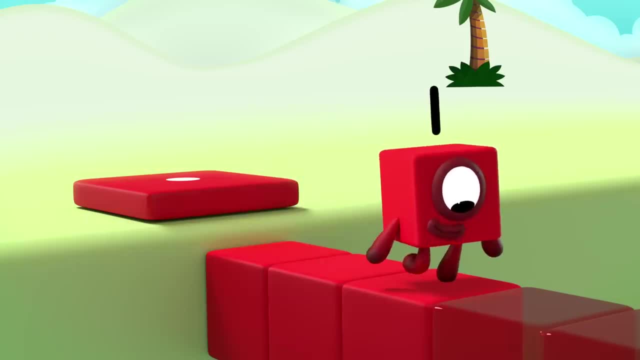 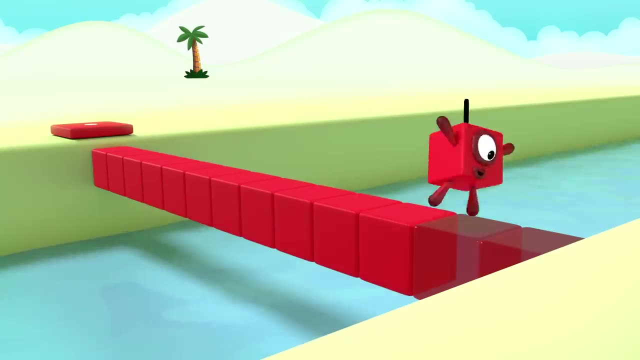 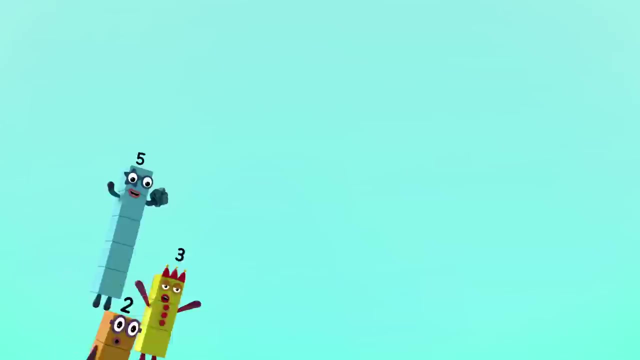 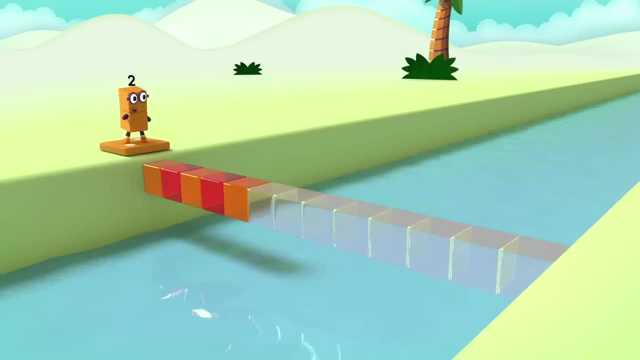 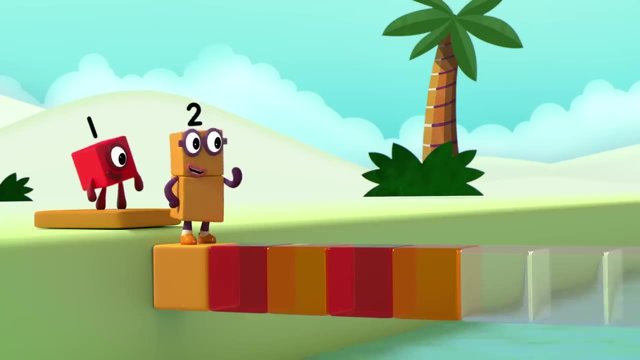 Uh, who is it Red Red Red? Uh, who is it Red Red Red, Red Red Red? Whoo-hoo, Whoo-hoo, Whoo-hoo. Two dots, Oh, My turn. 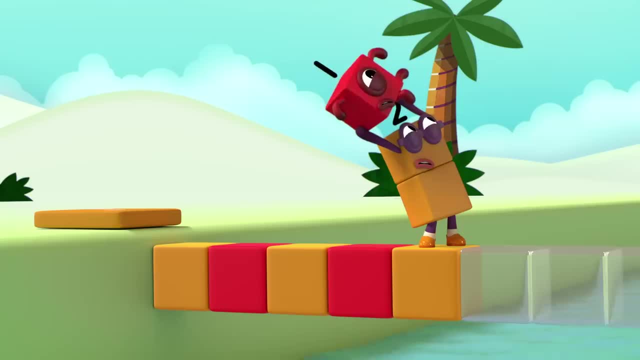 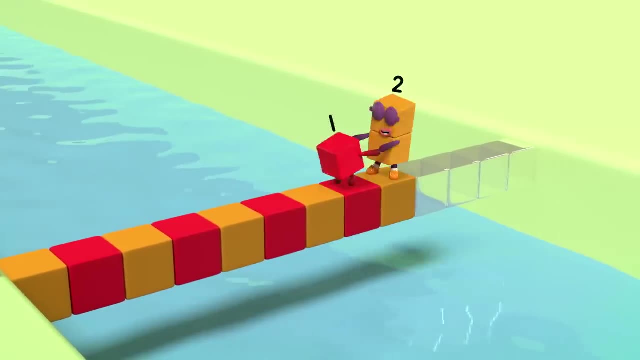 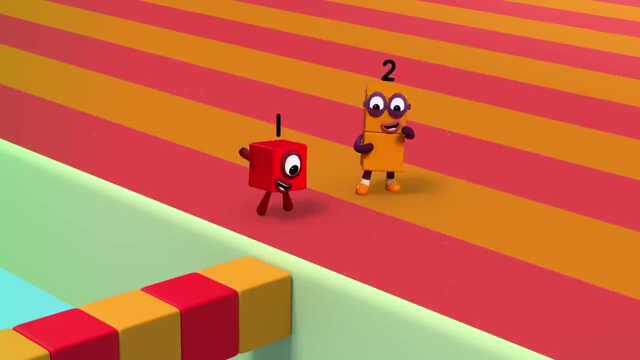 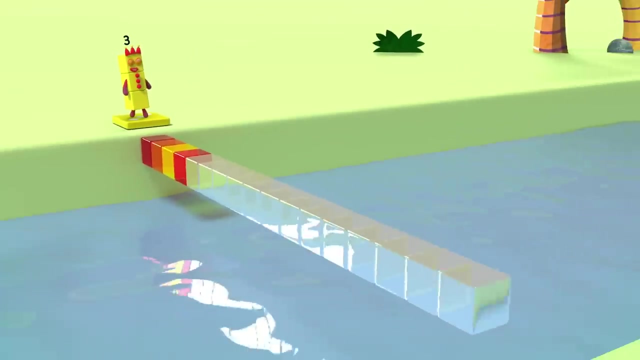 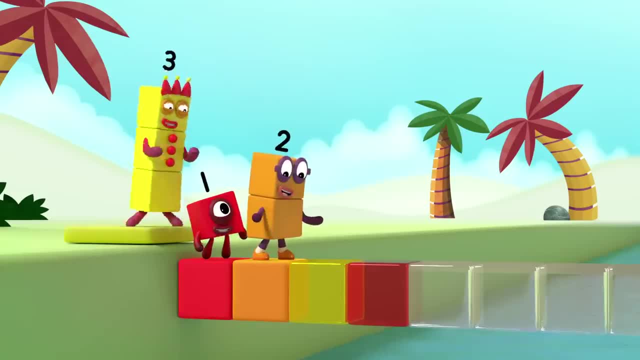 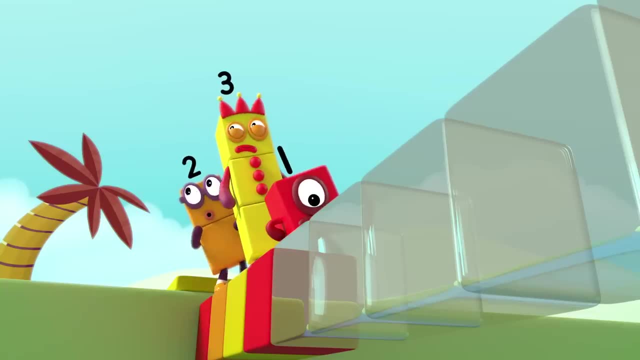 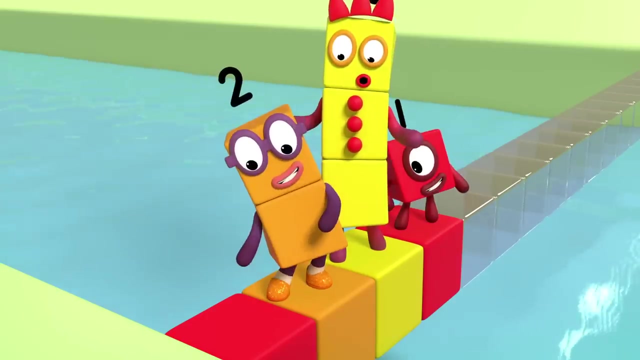 Red Orange, Oh Yellow, Yellow, Oh Red. Stop, Who's next? Ooh, Ah, Um, It goes. Red Orange, Yellow, Red Orange, Yellow, Red Orange, Yellow, Red Orange. 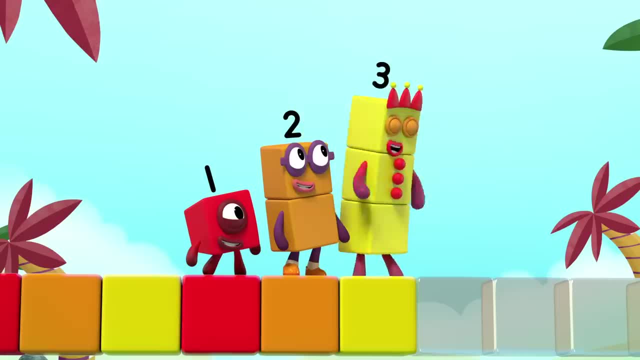 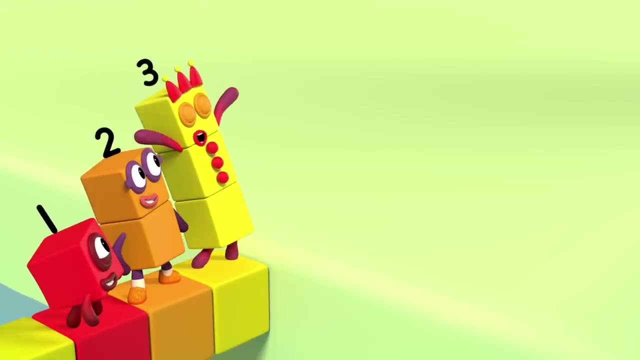 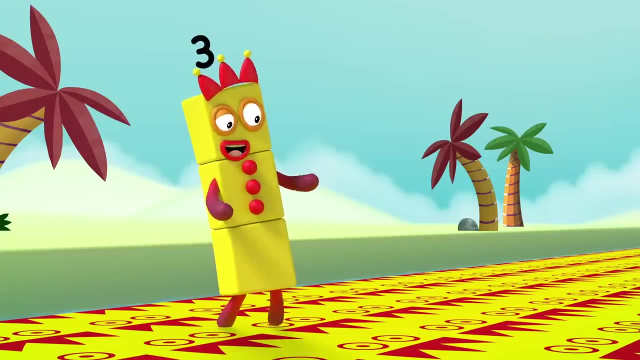 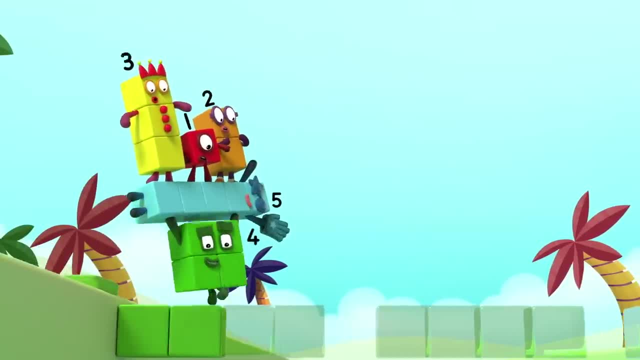 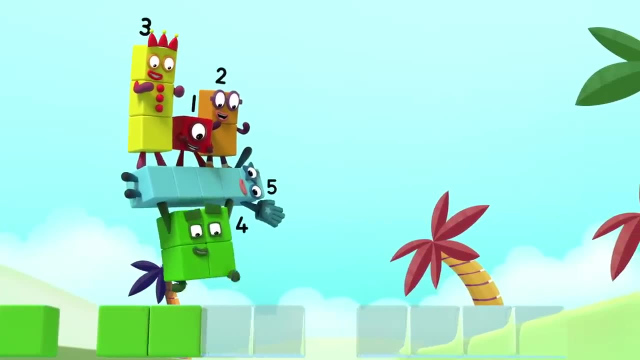 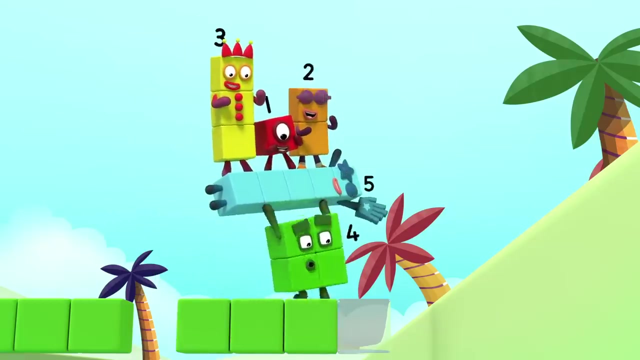 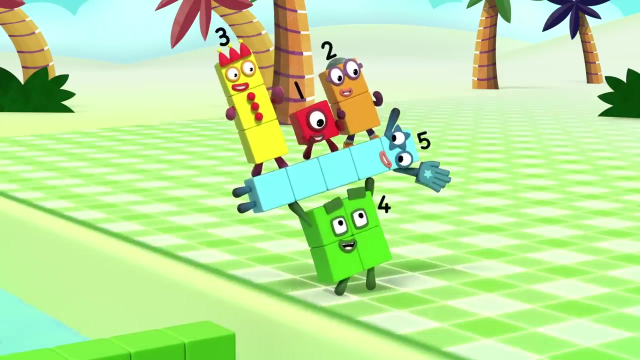 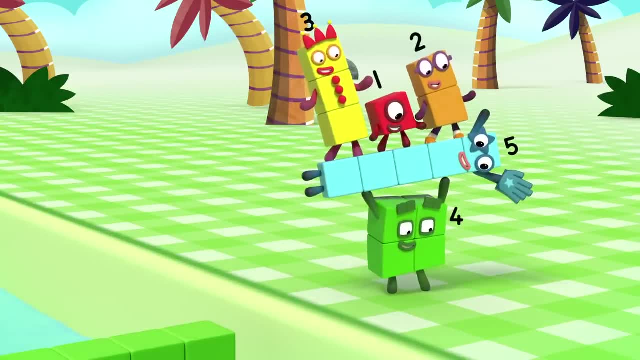 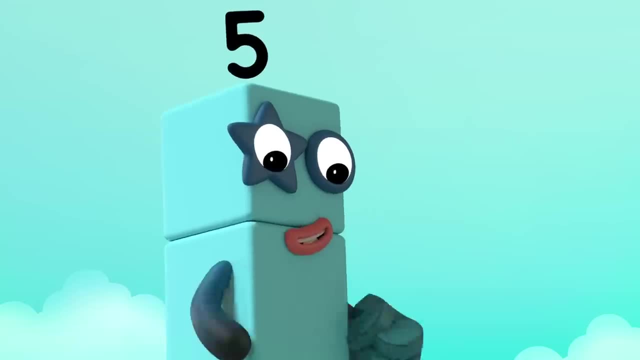 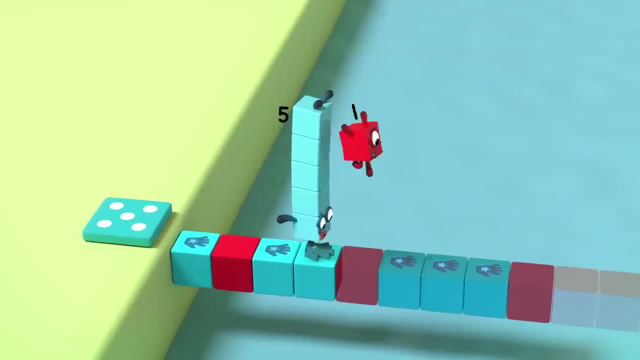 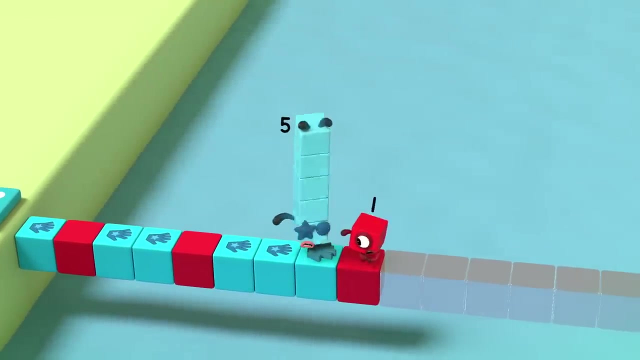 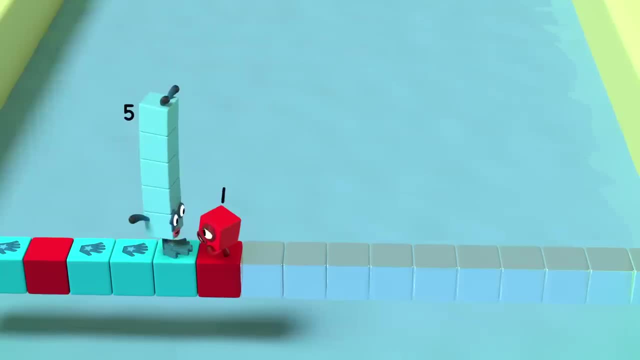 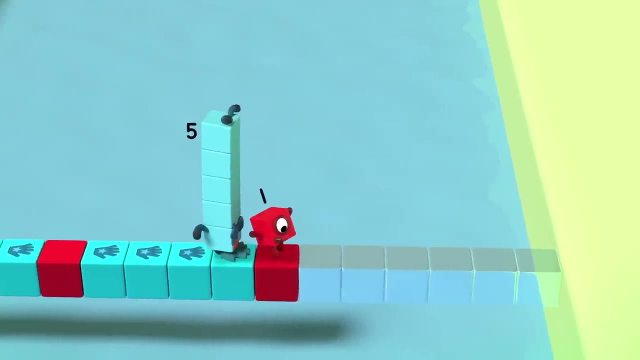 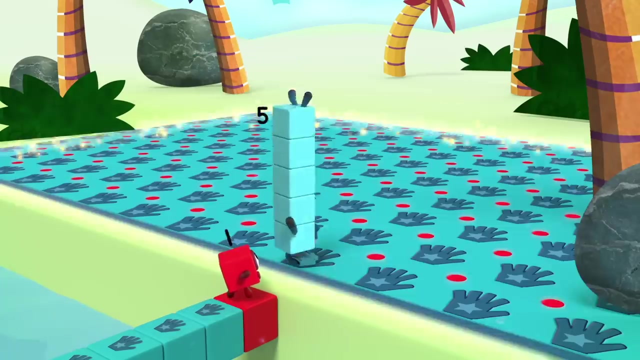 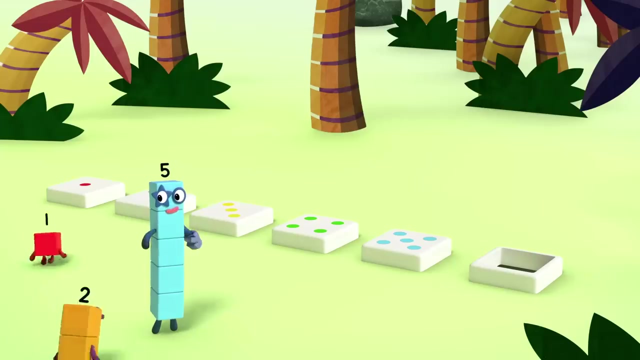 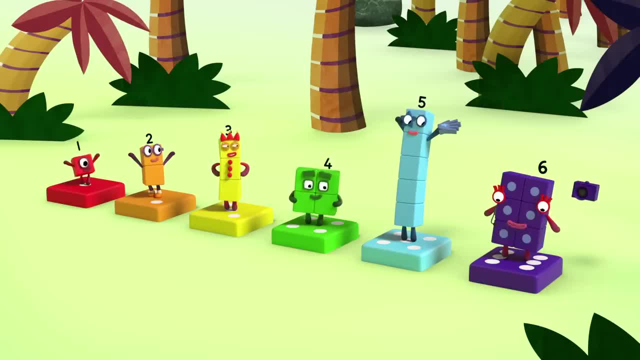 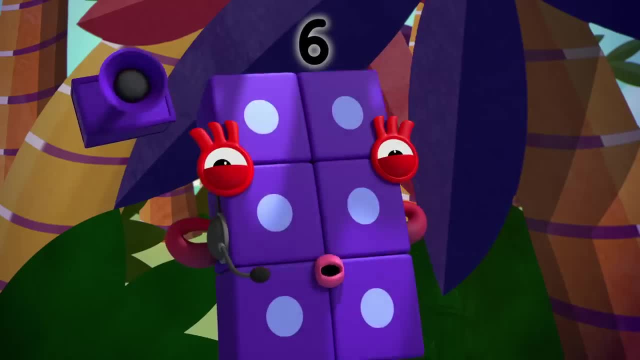 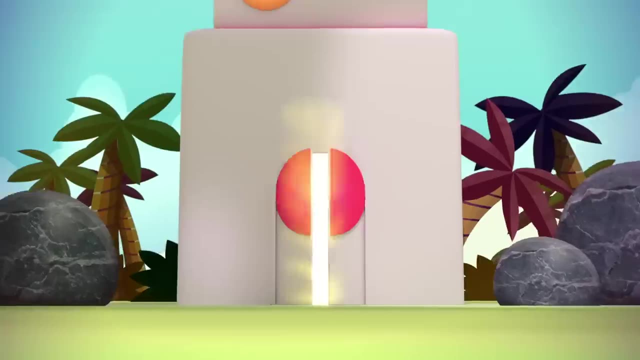 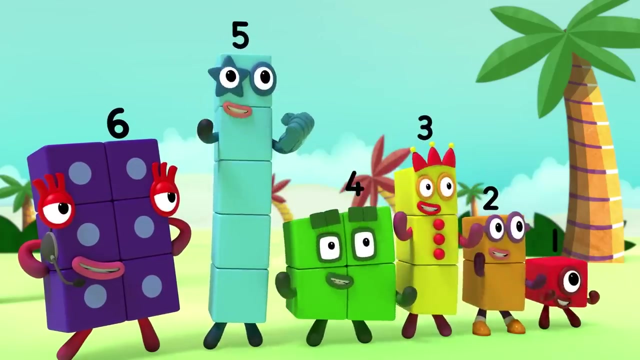 Pattern unlocked. You got across my pattern paths. Well done everyone. Now step into my pattern palace and let's all have some fun. Pattern palace unlocked, And next I'll show you the long gallery. Keep up everyone. Oh, what's through there? 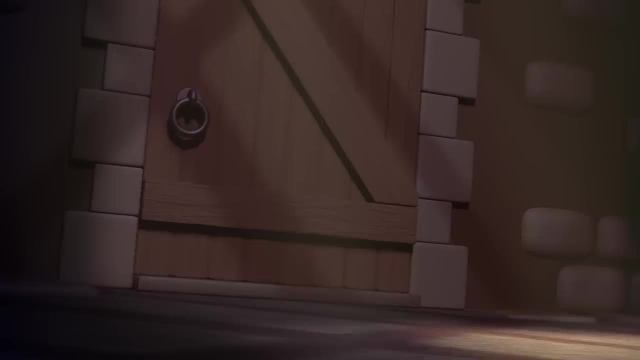 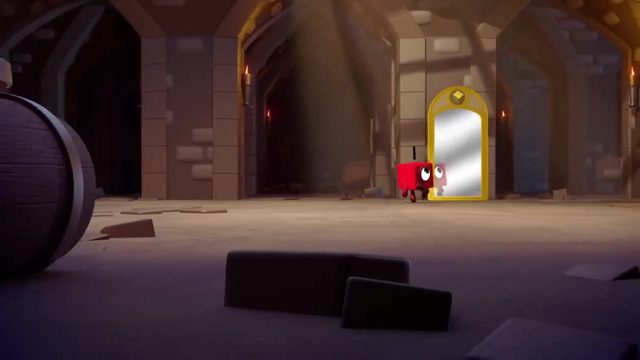 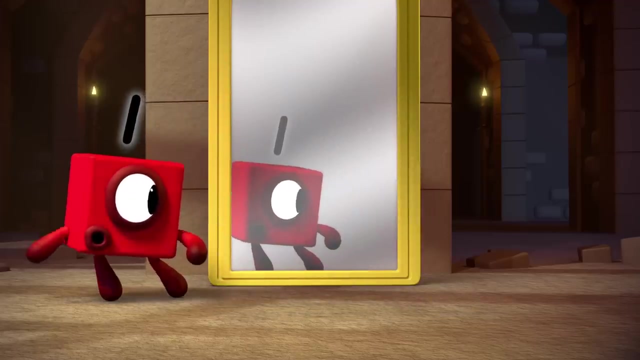 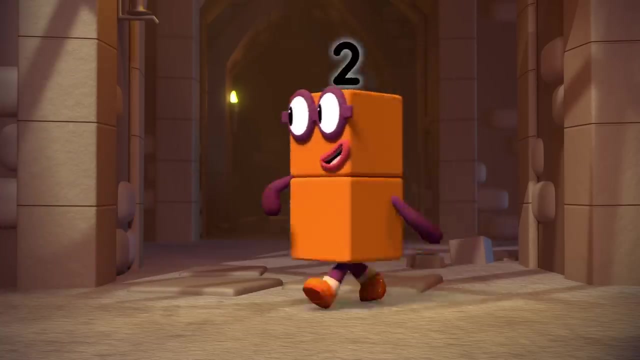 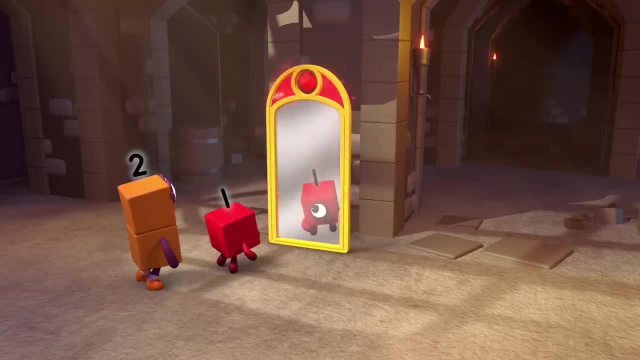 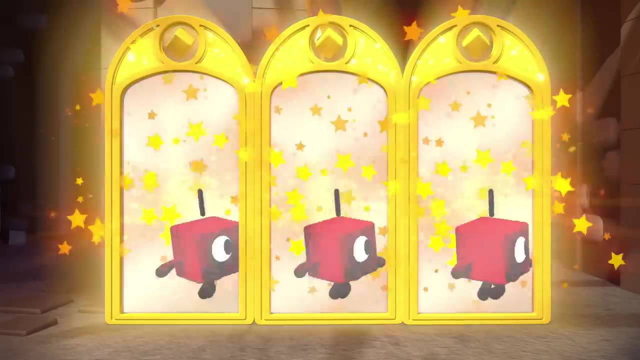 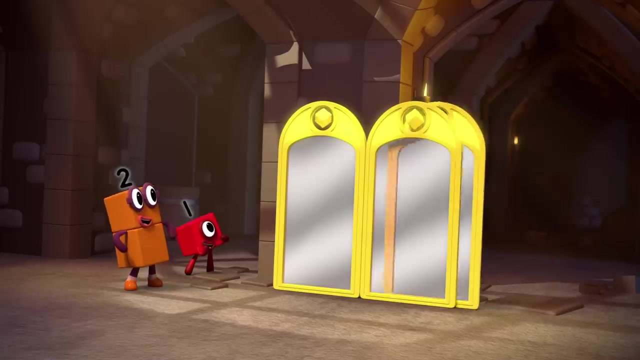 I wish you could make three of me. Your wish is my command. Oh, Wow, Three, lots of me, One of one. Ha ha, ha ha. One plus one plus one equals three. Ooh, My turn, My turn. 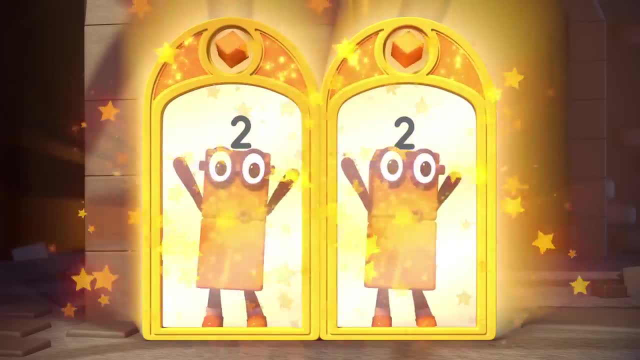 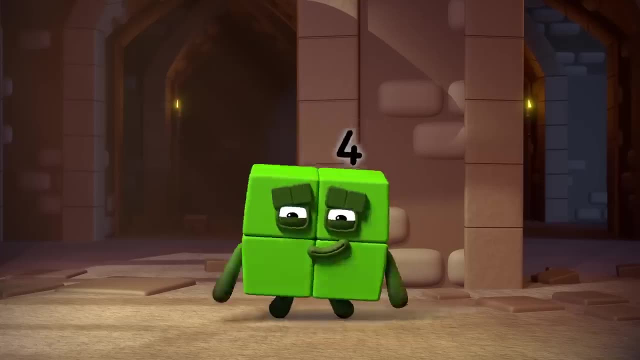 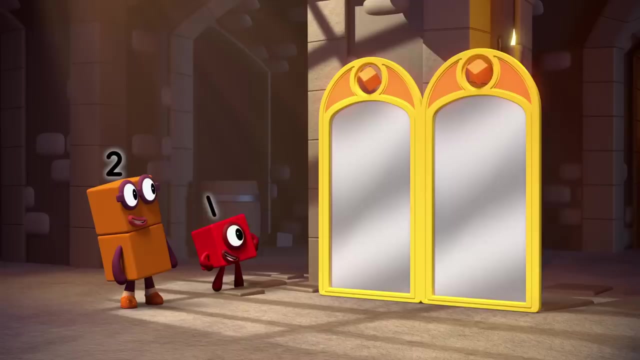 Two lots, please. Two lots of two. Two plus two equals four. I'm four. I'm Two lots of two. The terrible twos. Hee, hee, hee, hee, Ahem, Ah-ha. 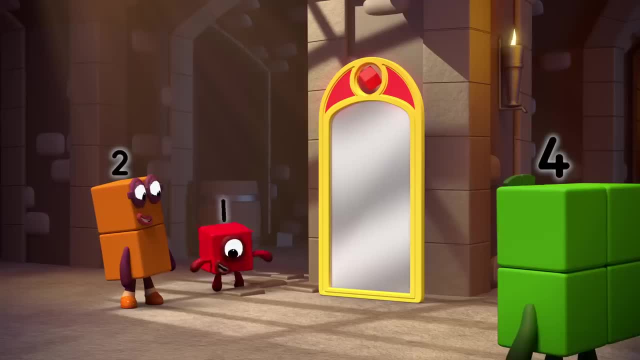 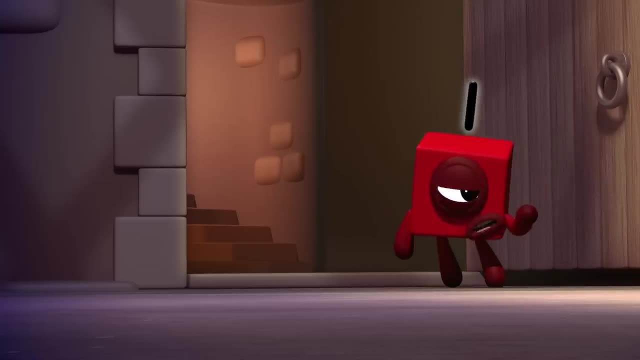 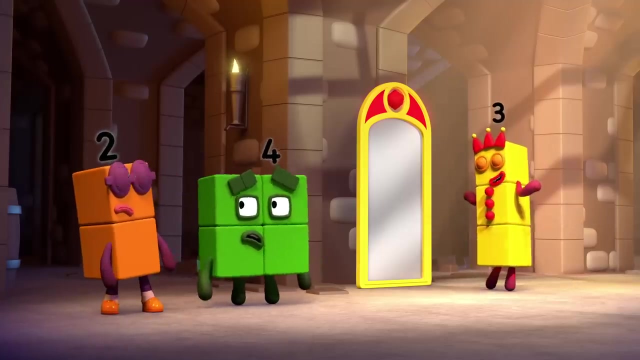 The magic mirror is even more magical than we thought. Oh, the others will want to see this. Keep an eye on it while I'm away and don't mess around with it. Right, my turn. One said not to. Oh, go on, it's only fair. 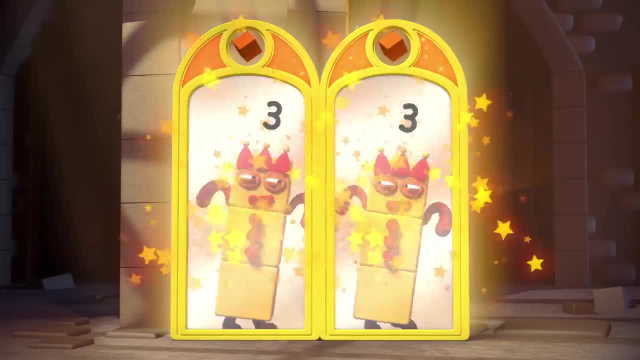 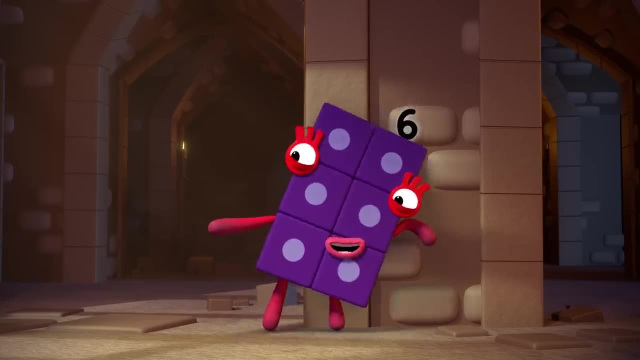 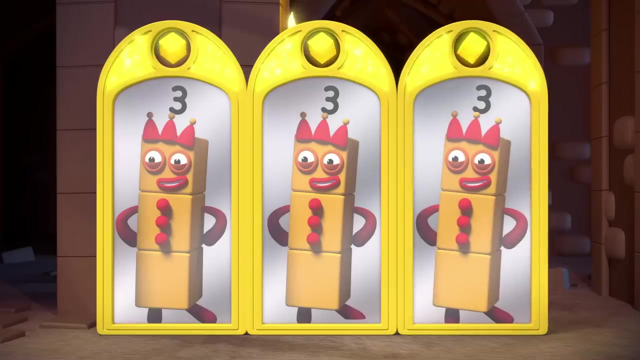 Two lots please. Two lots of three is six. Number six is on the floor. Don't be shy, let's have some more Good idea. Three lots, please. Ha ha, ha ha. Three lots of three. 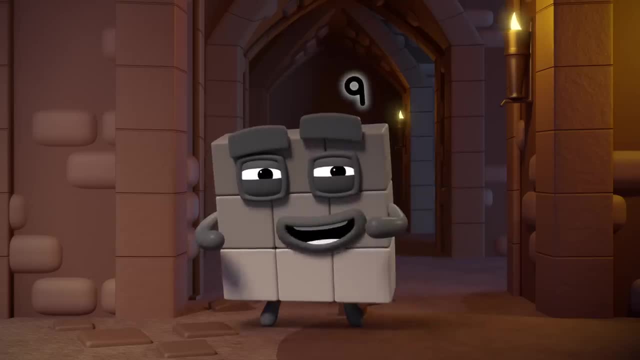 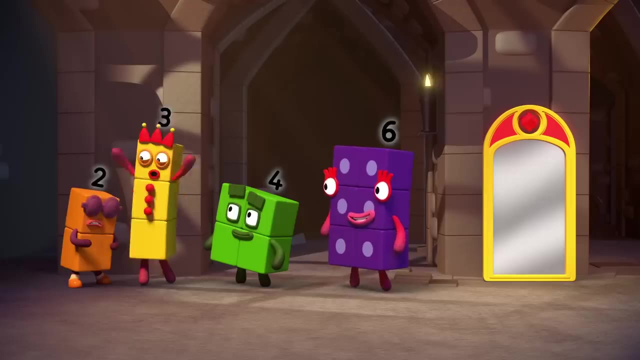 is nine And three, threes, see Ha Yay Ooh, We should probably stop now, But look, There are so many of us here already. Wump wouldn't be surprised if she comes back, and everyone's here. 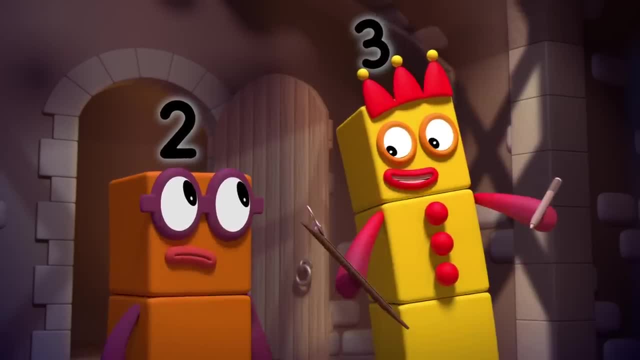 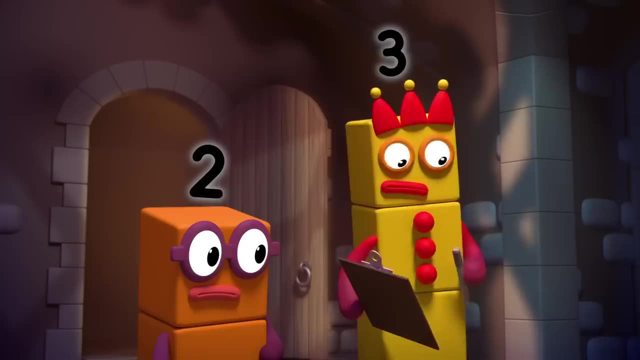 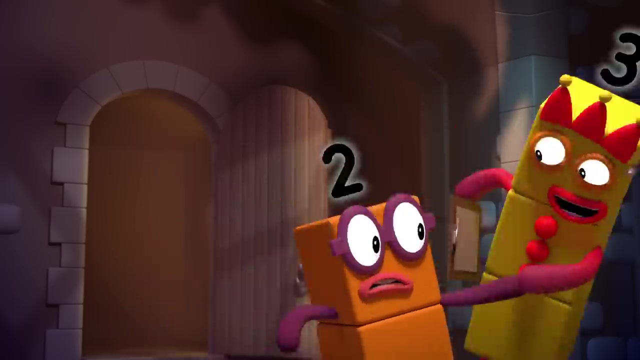 Hmm-mm-mm. All right, then We've got two, three, four, then six. Oh no, We're missing five. How many lots of? who is five? Hmm, let's try you. Ooh, Three lots, please. 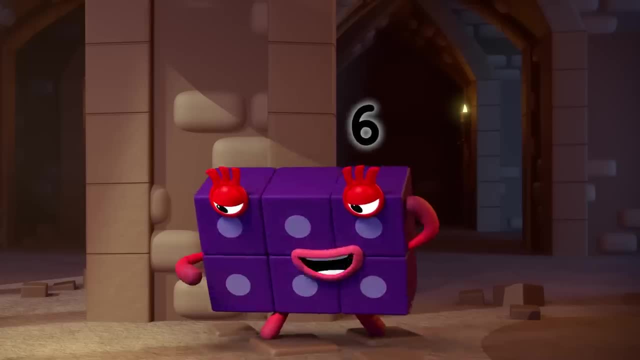 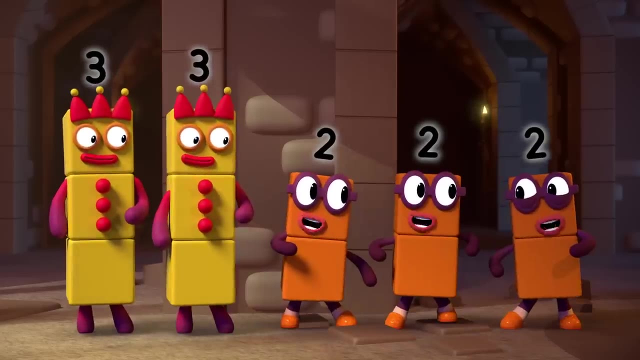 Three lots of two is six. Number six is on the floor. Have I said that before? Ha ha ha ha. Two lots of three, three lots of two. Ha ha ha ha, Yay Yeah. 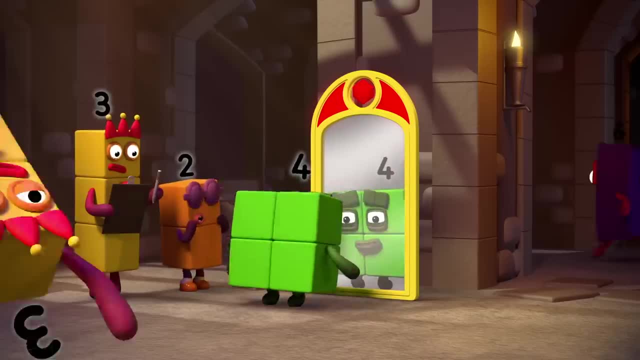 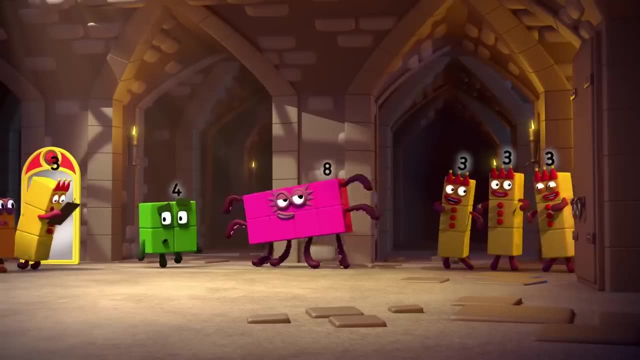 I was hoping for a five. Maybe I can help. No Two lots, please. Ooh Ha ha ha. Two lots of four is eight. No, no, no. We need a five And we're missing seven and ten. 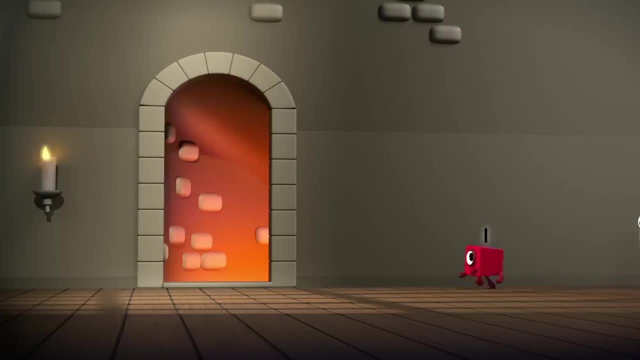 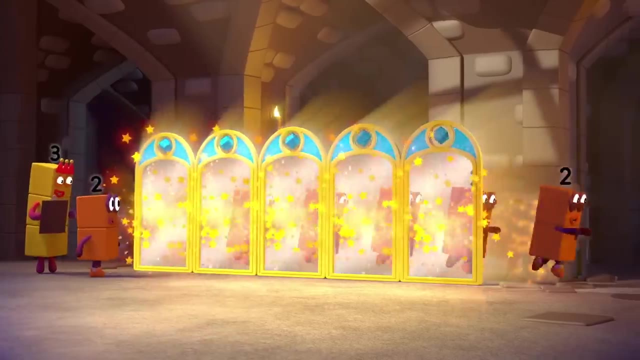 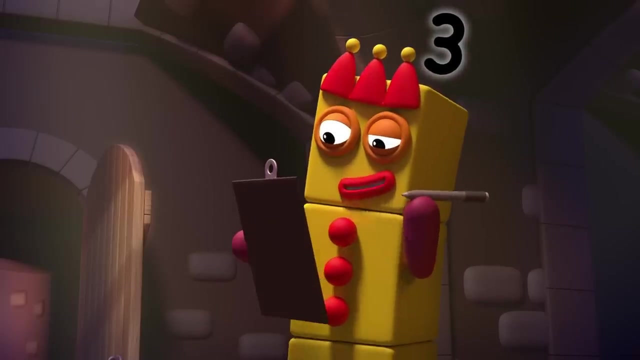 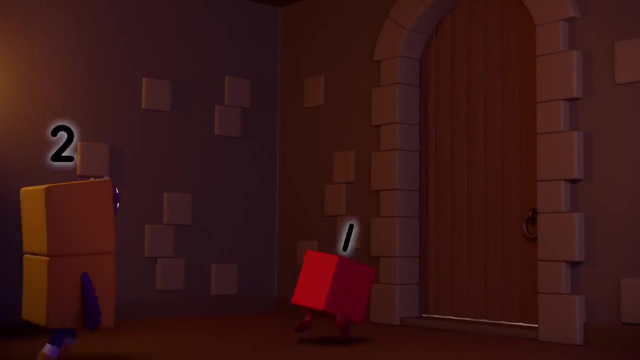 Who wants to try next? Ooh Ooh, It's a big surprise. Ooh Five, lots of two is ten. That's ten sorted. All we need now is five and seven. Next, Get ready for a really big surprise. 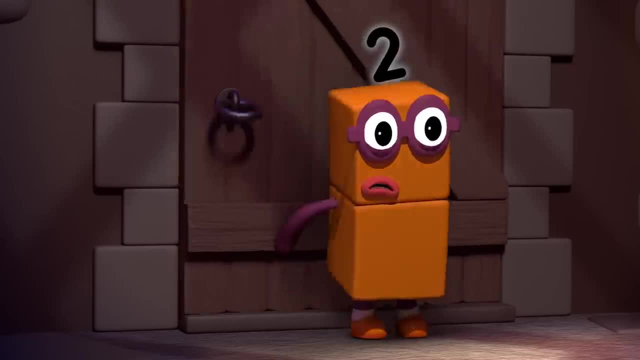 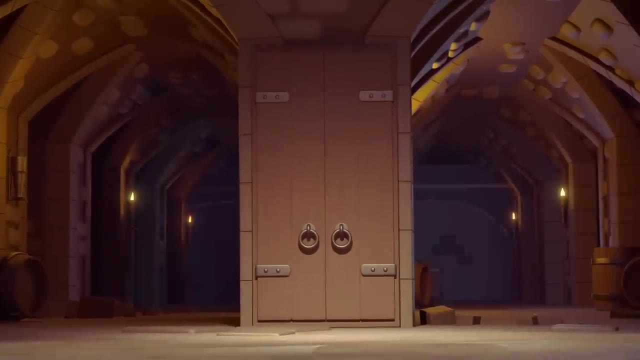 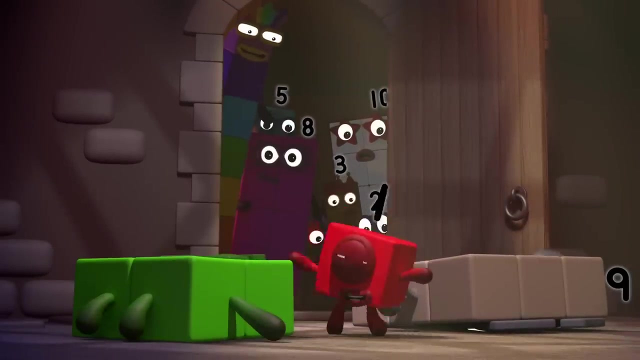 Huh, Ooh, One's coming Hide. Can we make five and seven? Ooh Ha, ha, ha, ha, Ooh Ooh Ooh. Whoa There Surprise, Ooh Ooh. 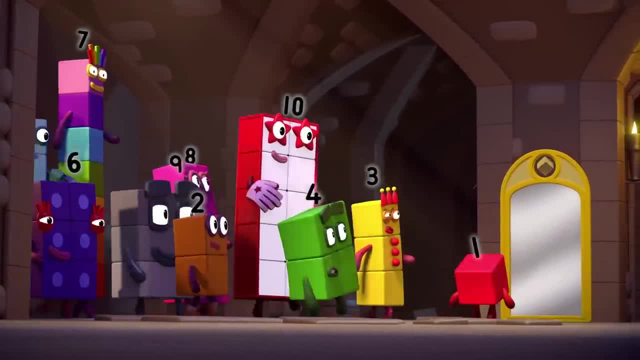 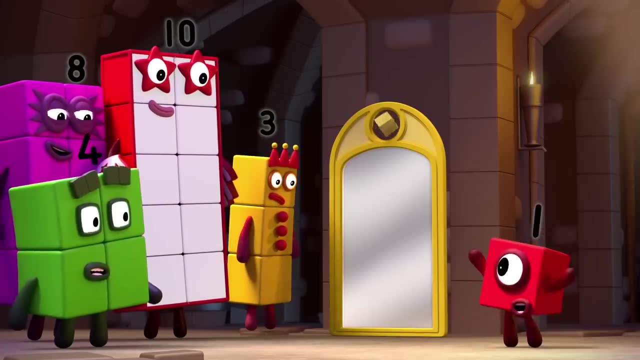 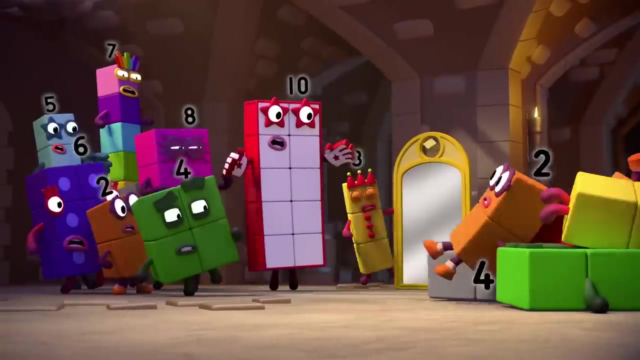 Ooh, A magic mirror, Some big surprise. Ooh Ah. But what if I said I could make lots of number blocks appear all at once? Now, that WOULD be a surprise. Ooh, Ooh, Ooh. 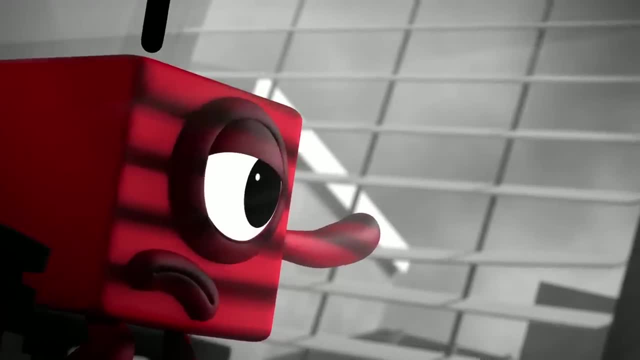 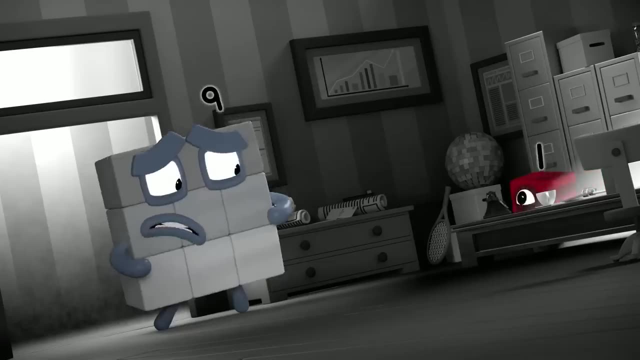 Ha ha ha. Surprise. That was a great day in the big city. I was wondering where my next case would come from, when You've got to help me one. It's gone, Everything's gone. Slow down. Nine. 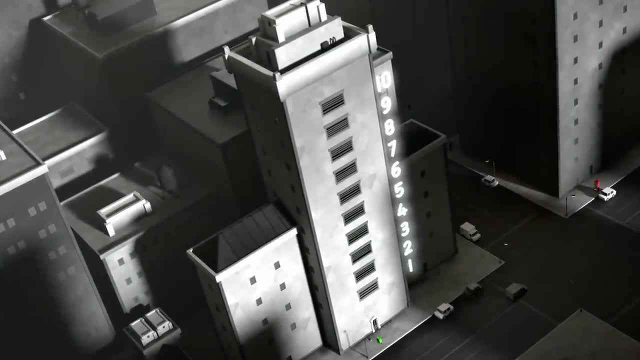 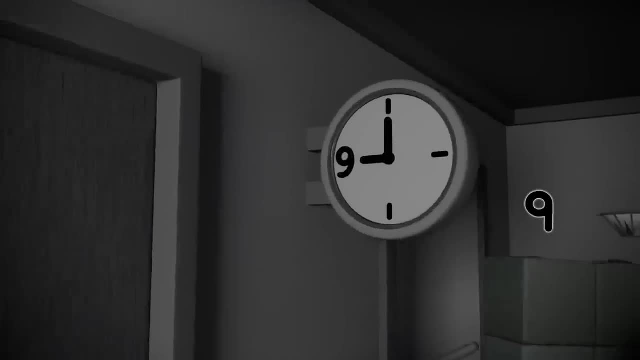 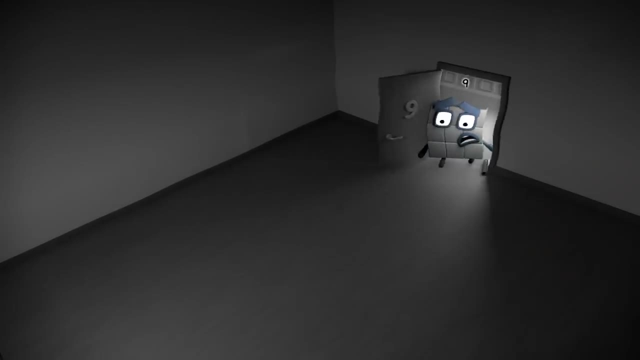 Tell me what happened. I live in apartment nine on the ninth floor of numerical towers. I left home this morning at nine o'clock to buy a newspaper. When I came back nine minutes later, the door was open. Everything was gone. A mystery indeed. 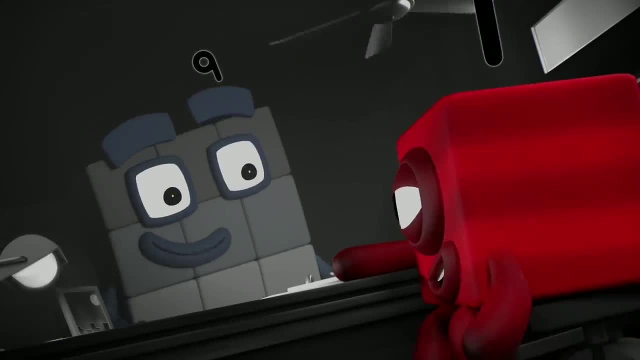 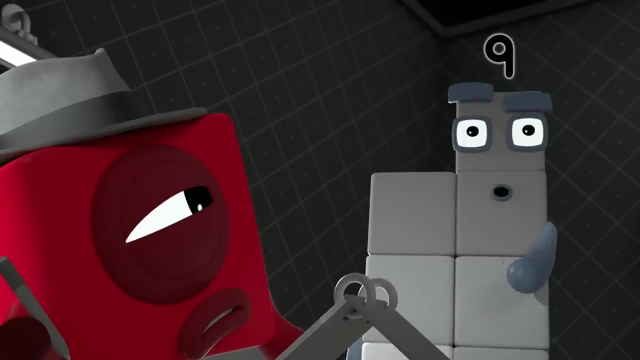 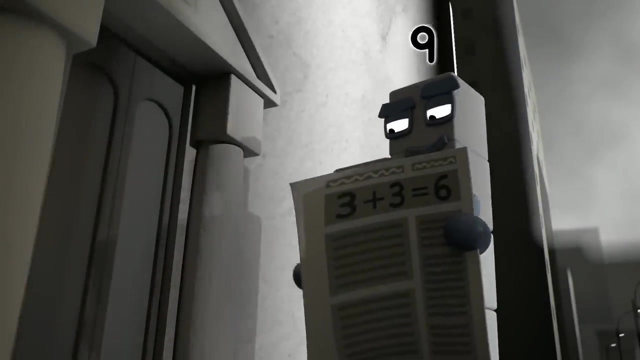 I'll take the case. Let's look for clues. Did you notice anything strange or unusual when you got back? Er, no, nothing. Oh, there was one thing: A suspicious, shadowy stranger in a coat and hat pushed past me and ran out of that door. 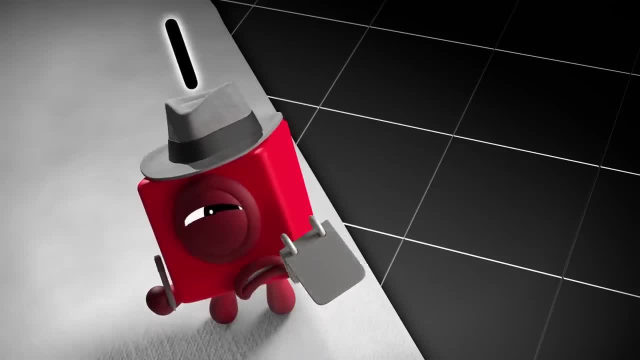 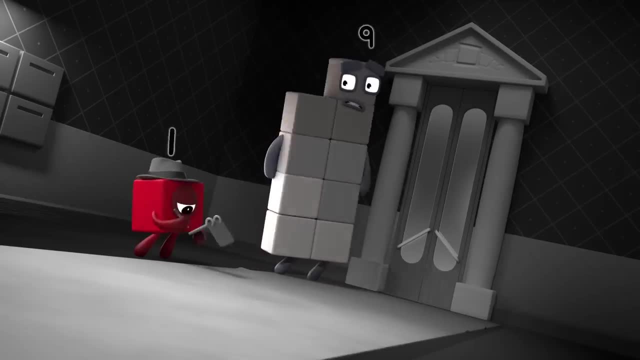 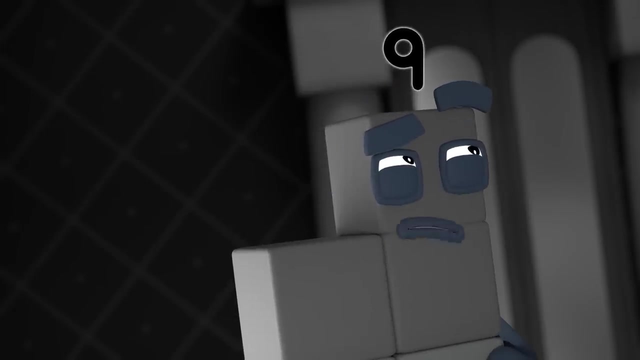 But apart from that nothing. Can you describe this stranger? They were as wide as the door, so two blocks wide with a flat head. Clue, one flat head when standing two blocks wide. Anything else I could see over their head when we were both two blocks wide. 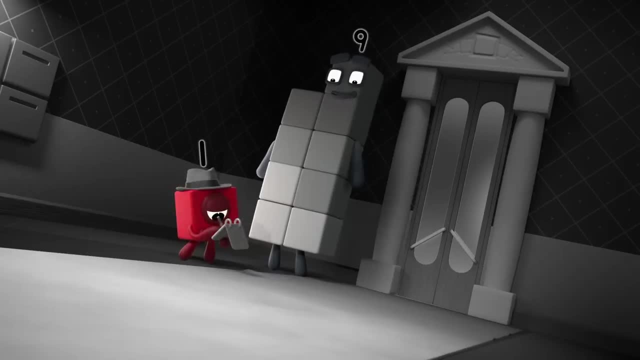 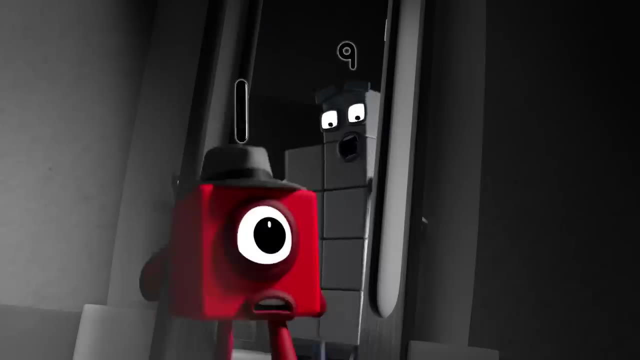 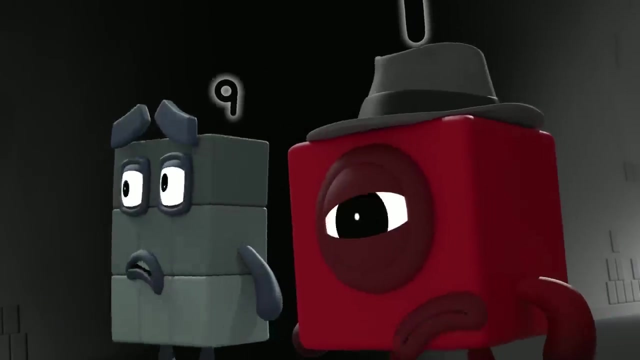 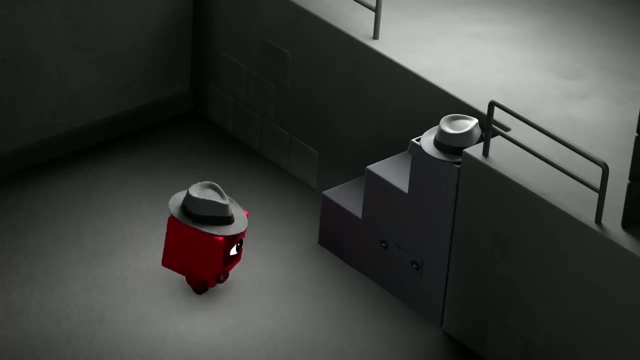 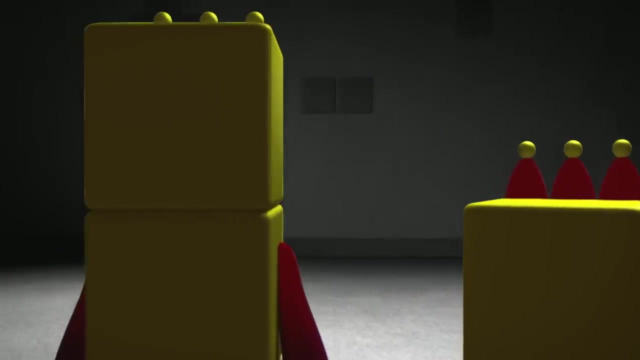 so they must have been smaller than me. Clue two, smaller than nine. Hmm, Hat Coat, It's them. After them, quick There on the steps. The hat, These aren't steps, it's. Did either of you see a suspicious? 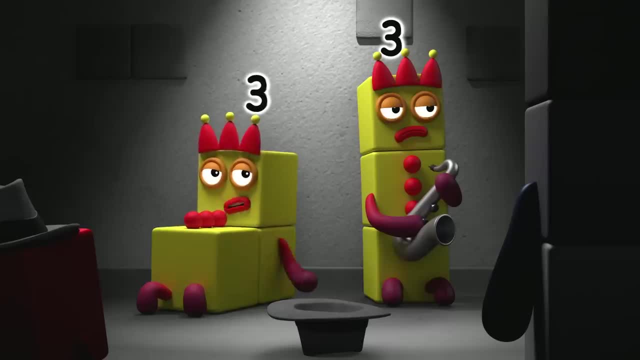 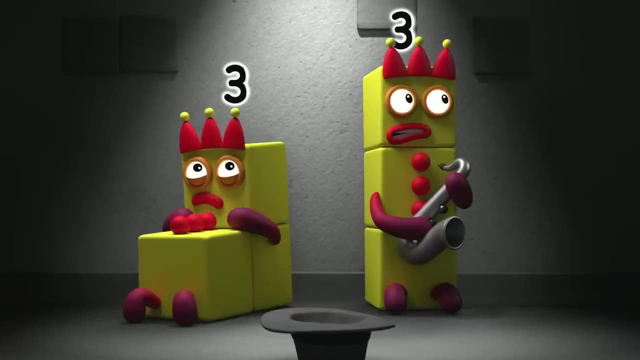 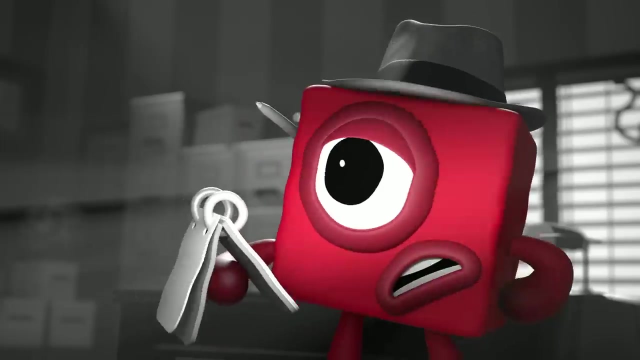 step-shaped figure in a coat and hat. Sorry, friend, No-one else down here, Just us. Something didn't add up, Or did it? Let's look at what we know. Clue one: The suspect had a flat head when standing two blocks wide. 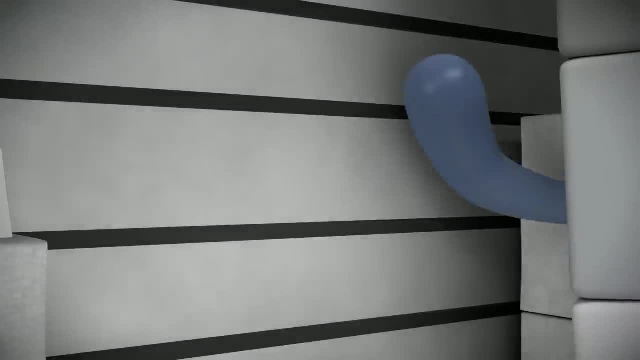 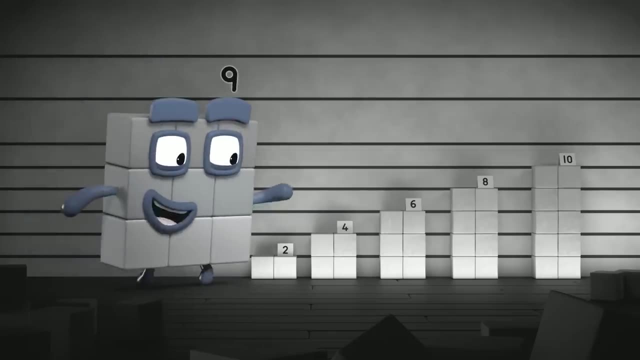 so it can't have been three, five, seven or nine. And it wasn't you, Because you can't stand two blocks wide. Two, four, six, eight, ten. The suspect must be an even number. Bingo, And remember clue two. 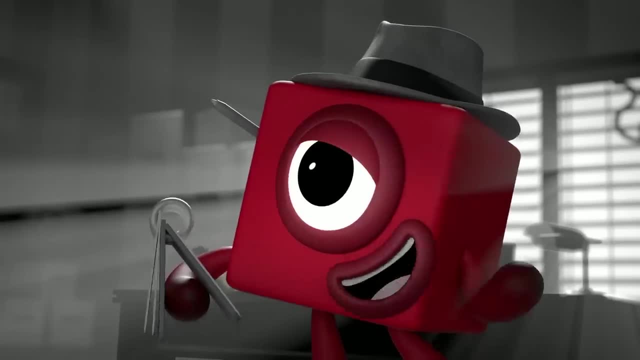 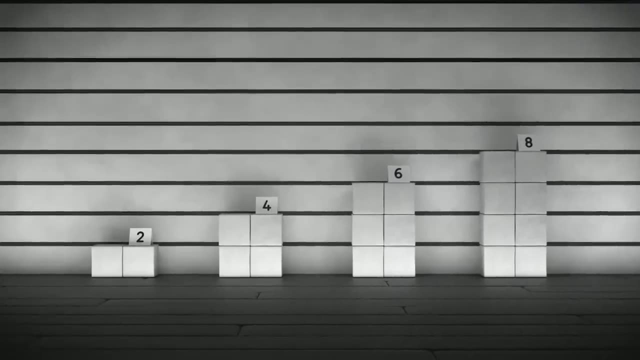 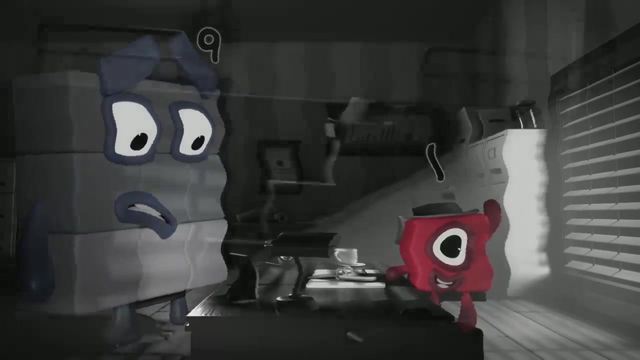 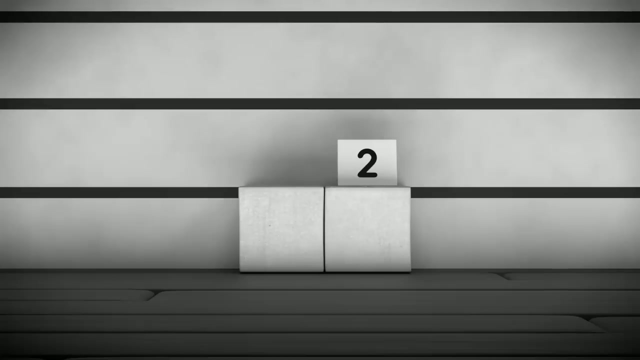 The suspect was smaller than nine, so it can't have been ten. That still leaves two, four, six and eight. But which was it? Wait, There's one more clue. we nearly forgot. The suspect can make a step shape, Not two or four or eight. 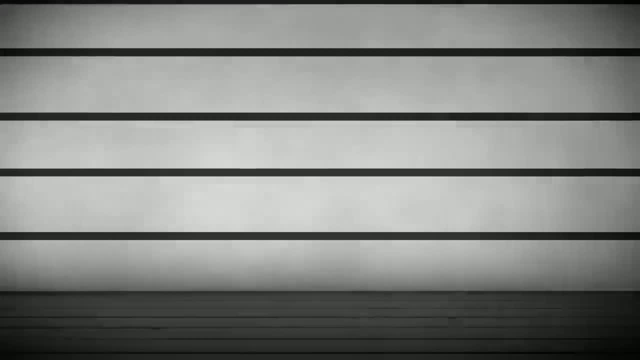 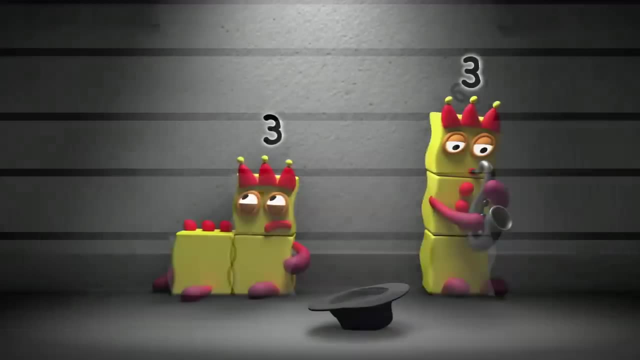 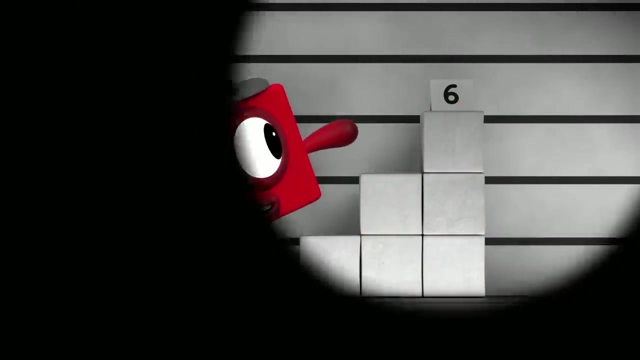 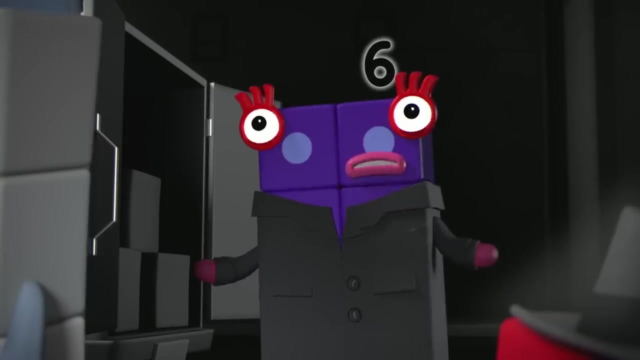 So it must have been Six. And who did we meet in the alley? Three And another three Equals six. Stop, Thief. Ha, I'm not a thief, I'm a thief. You've got it all wrong. Oh, where to begin? 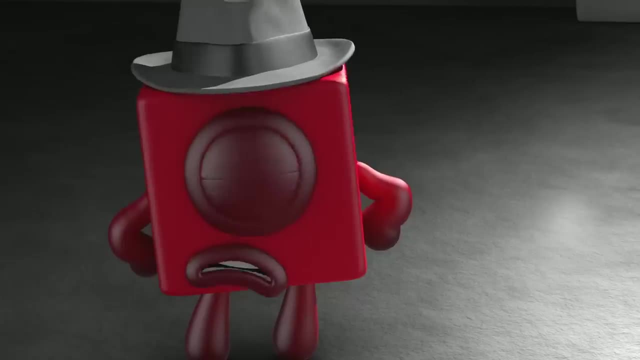 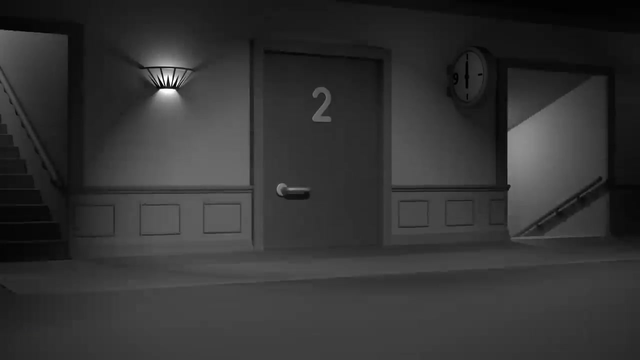 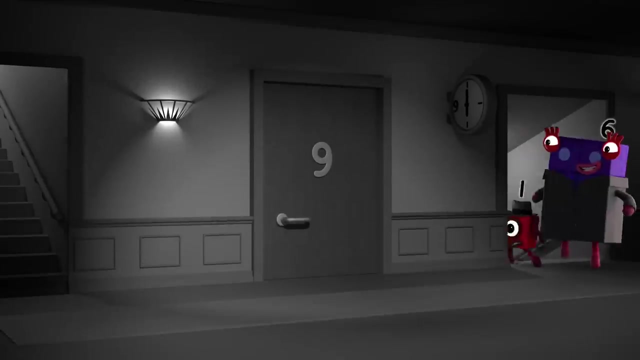 I'm not taking these things, I'm moving them in, Moving in. Come up and I'll show you One, two, three, four, five, nine. Wait, Nine doesn't come after five. This isn't apartment nine. 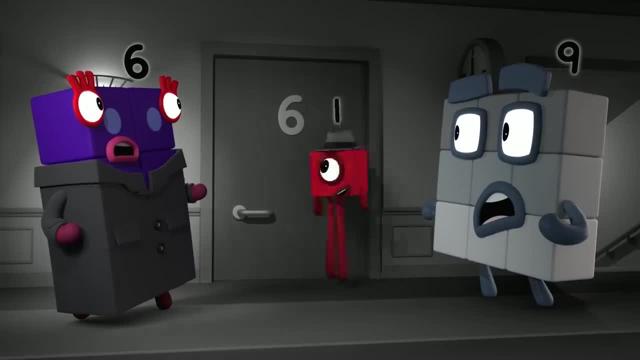 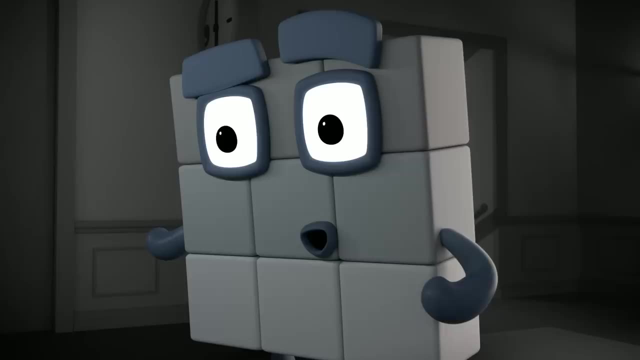 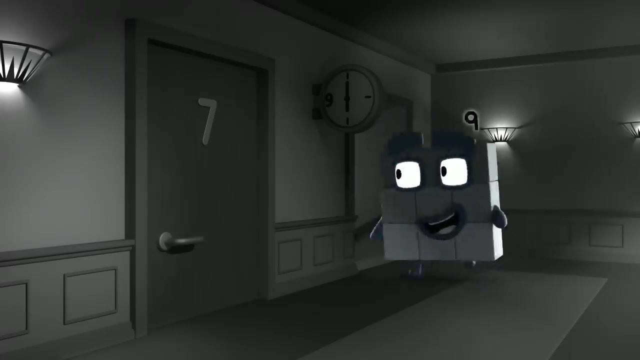 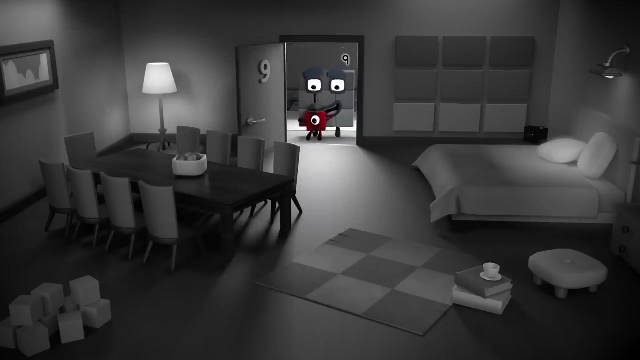 It's apartment six. Look number six. turned upside down looks like a number nine. Oh, No one stole your things. Nine, You went into Six's empty apartment, So my things must be Right where I left them. Case closed. 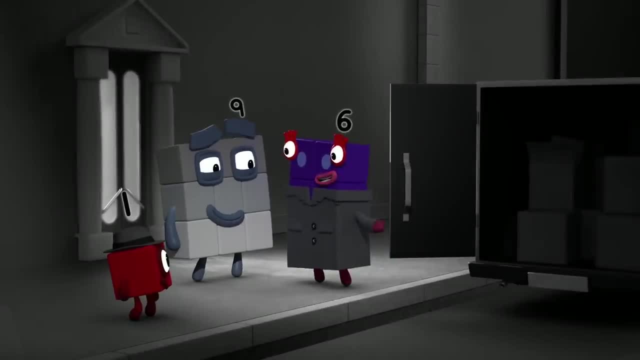 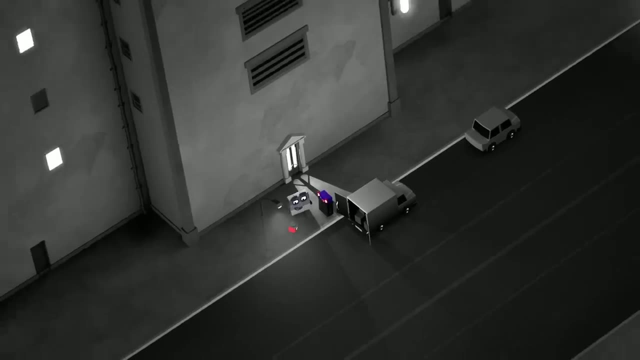 Sorry, we chased you Six. I thought that you were after me. That's why I hid. I hid as three plus three. Let's make it up to you by helping you move in. Welcome to the big city. Phew, It's cold up here. 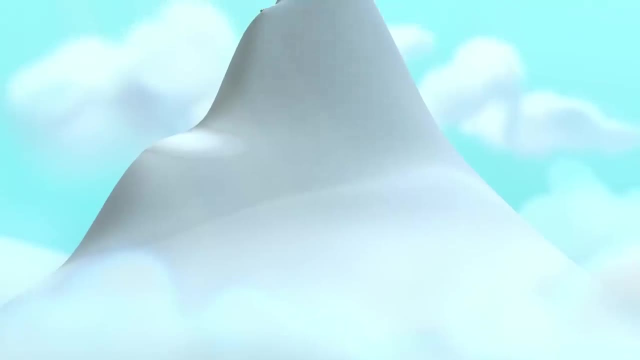 Keep going, everybody. We're near the top of Blocky Mountain. Ooh, If we're really lucky, we might spot the legendary Big Tum Ha, A big hairy monster with a big hairy tummy who loves puzzles. Don't be silly Seven. 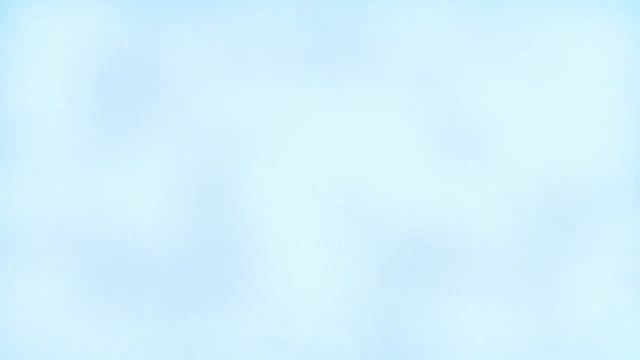 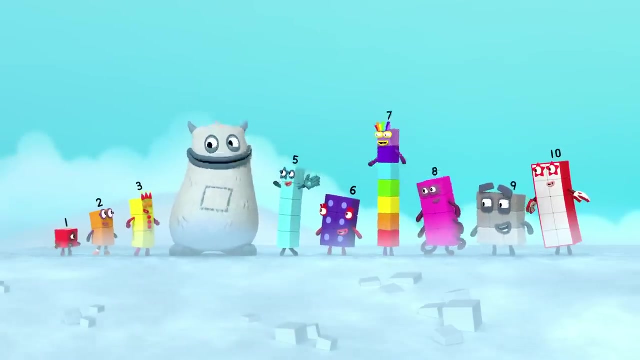 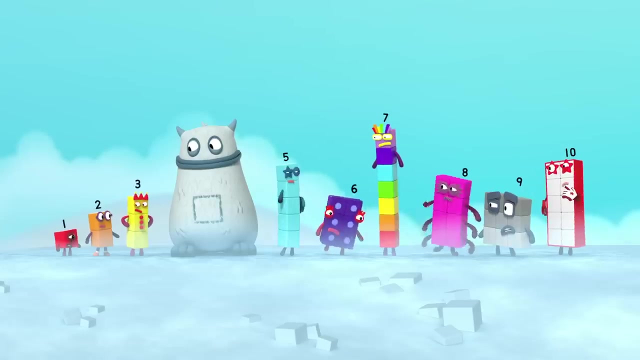 We're going to find him. Yum, What was that? Yum Big Tum. Yum yum, Who's in my tum? Who's in Wait? Is one of us missing? Huh, Ooh, Everyone. call out your number. 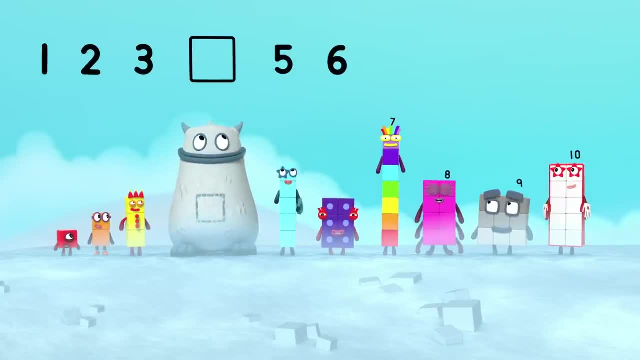 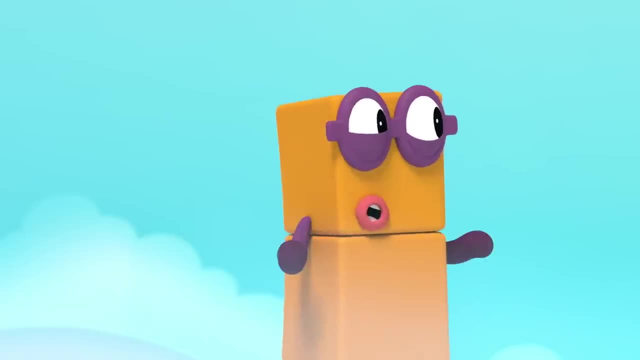 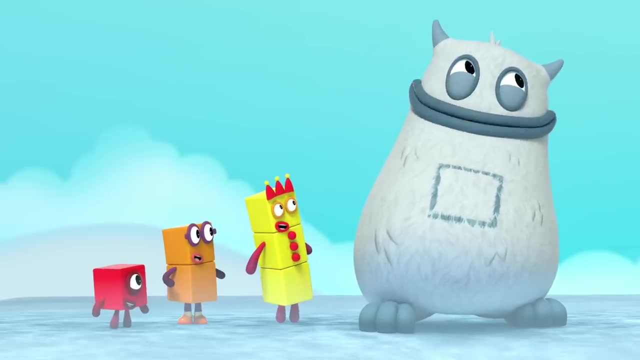 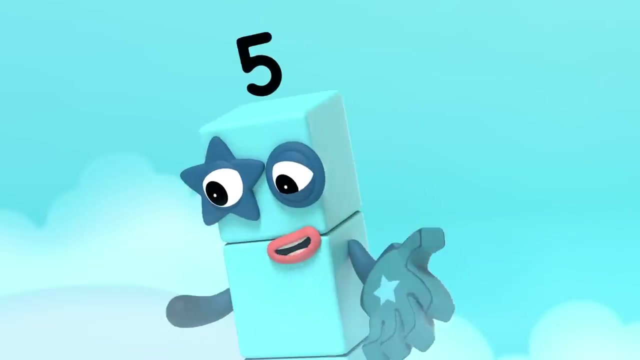 One, two, three, five, six, seven, eight, nine, ten. Oh, Hmm, Where's Four, Four's missing, Four's in your tum. Yum, yum, Well done. Oh Ooh, Are you feeling OK? Four: 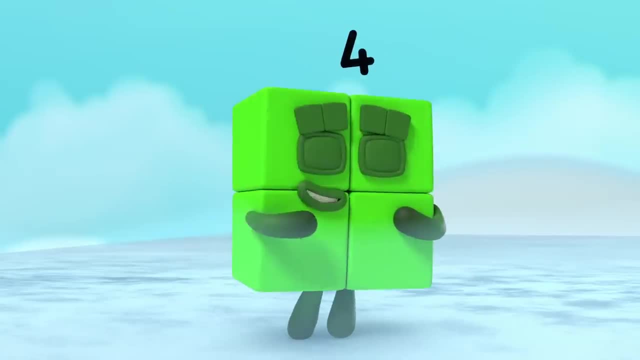 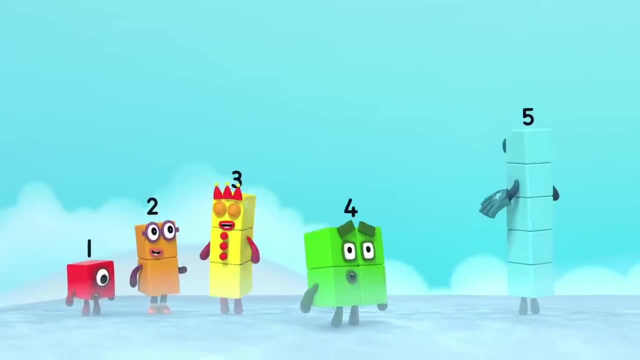 Oh, I'm fine, thank you. It was warm and snuggly in Big Tum's tum. Huh, Oh my God, Come and get me Game on. I'm coming Ready or not? Ooh, Ooh. 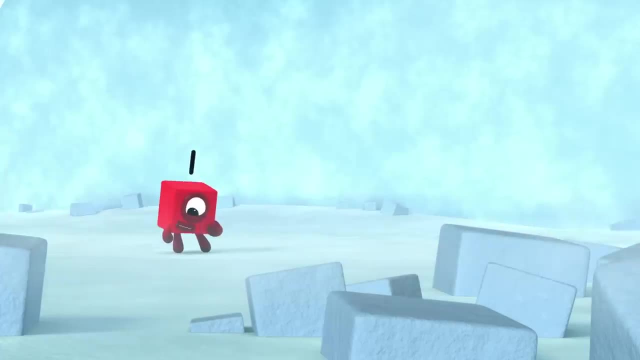 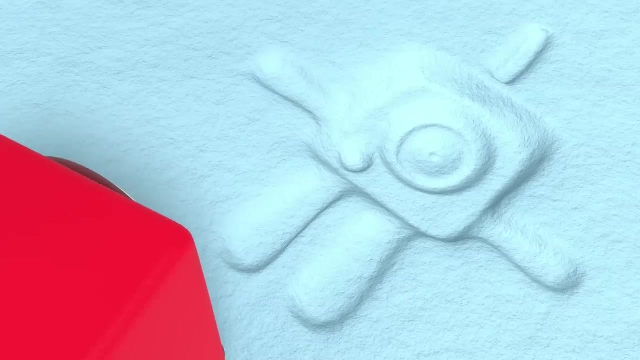 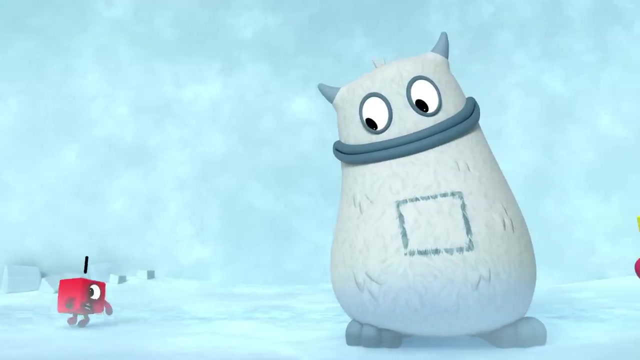 Ooh, Look, Nine, Nice smooth snow. Yum, Oh, Oh, Ooh, Yum, yum. Who's in my tum? Nine? Oh no, Where are you? It was me, I was Nine. 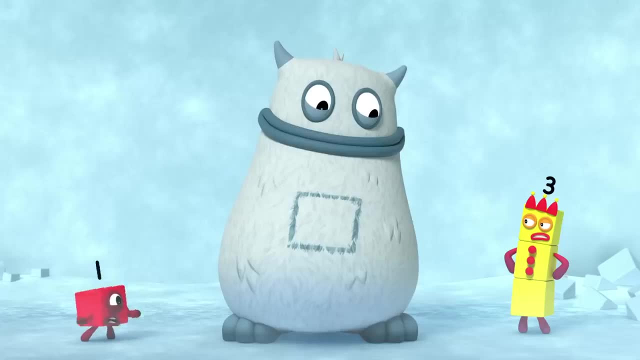 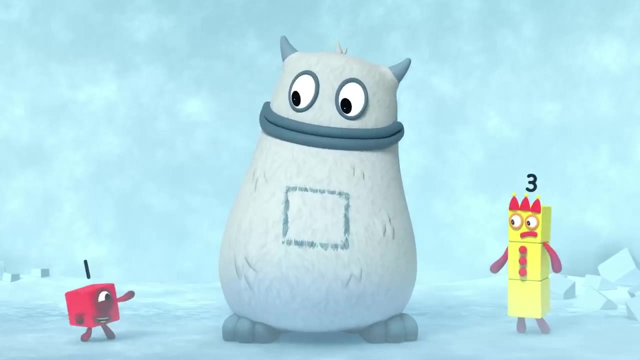 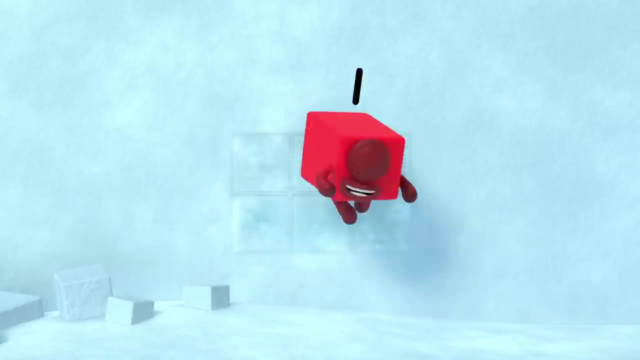 And Big Tum gobbled up some of my blocks- How many, I don't know. I had my eyes shut, Oh, I know. Here goes One, two, three, four, five, six, seven, eight, nine. 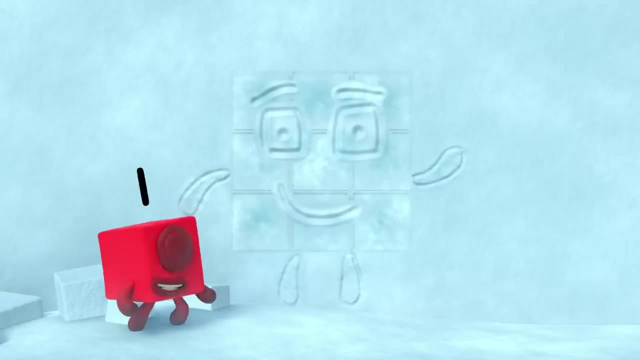 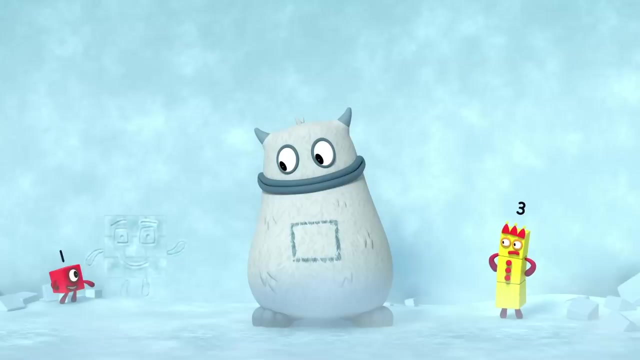 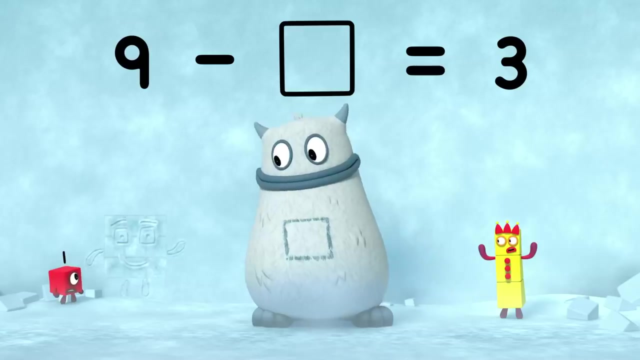 Uh-huh, Huh, So Nine was here. Then some of his blocks were taken away and that left you three, which means Nine minus Yum equals three. So what's missing? Hmm, Come over here. Three. 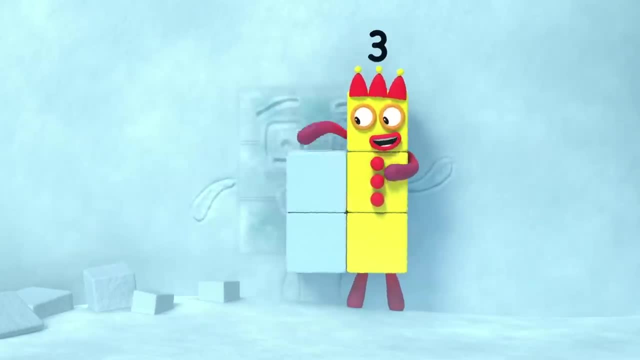 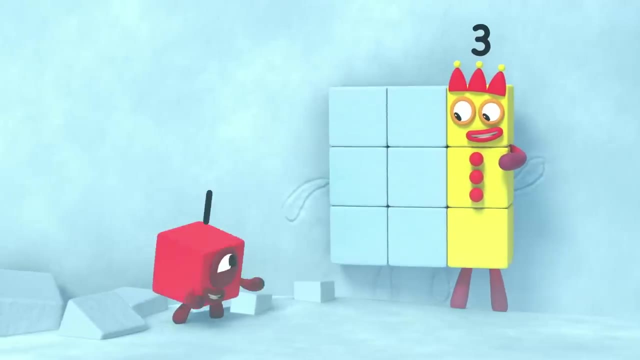 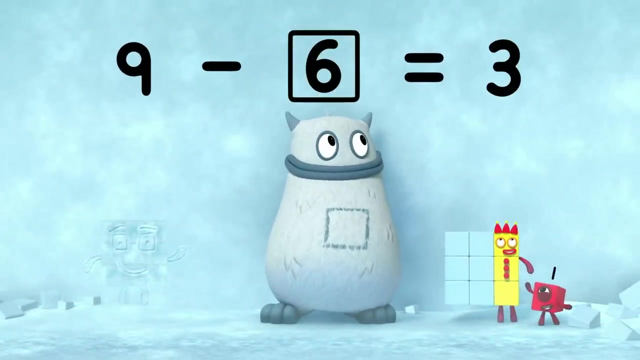 Hey, Brr, That's one, two, three, four, five, six There. So that's what's missing. Nine minus six equals three, And six is in your tum. Yum-yum. Well done, Hooray. 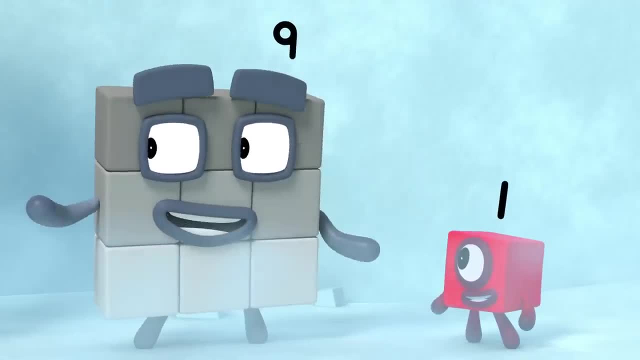 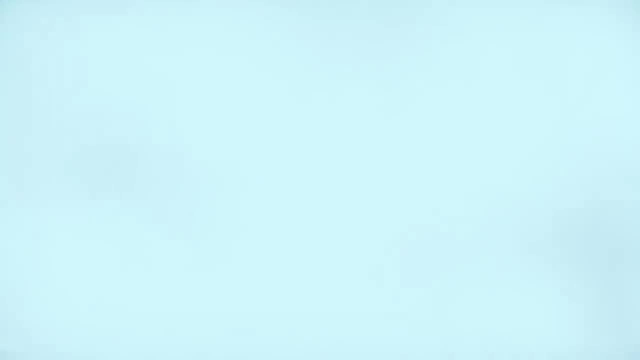 Ha-ha, It's good to be back. Where are the others? Octoblock sledge, Yum-yum-yum-yum. Everybody stay close. No need to panic. Oh Um, What's wrong, friends? Why don't you? 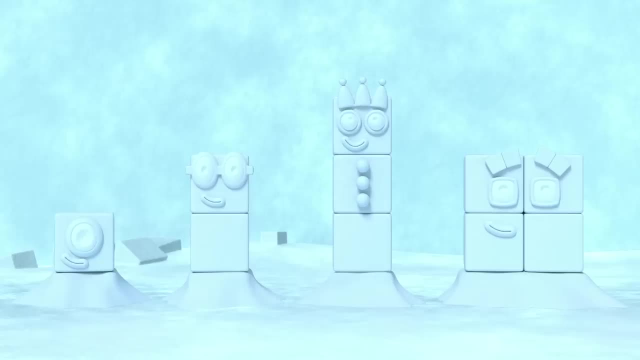 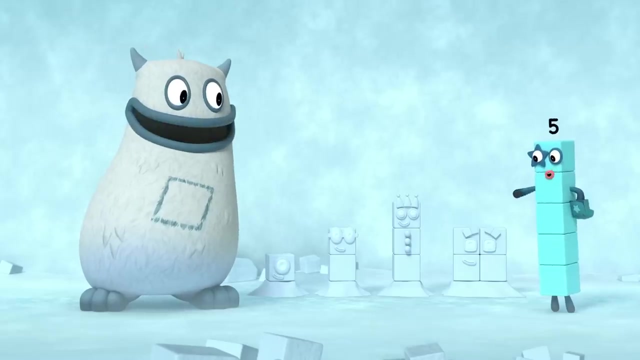 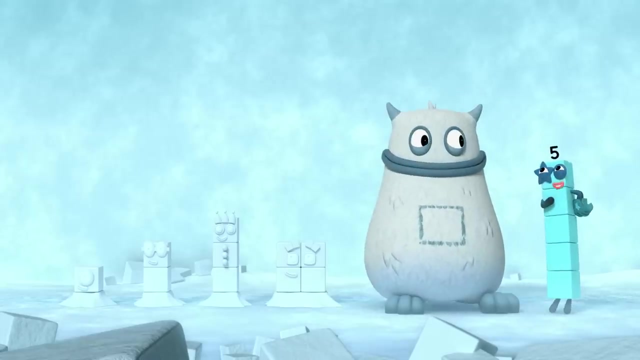 Oh, they're made of snow, Snow, Yum-yum. Who's in my tum? That's easy. The real one, two, three and four. No, They're all together now. So what do they make when they're all together? 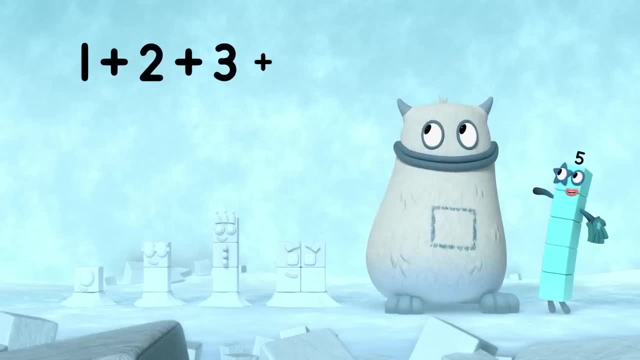 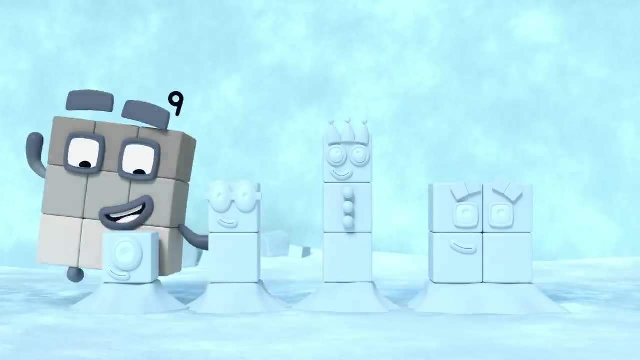 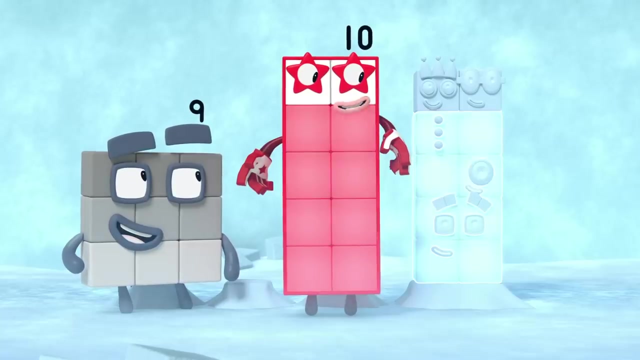 One plus two plus three plus four equals Yum. Let's try adding the snow blocks together: One two, three, four. One two, three, four, five, six, seven, eight, nine, ten, Ten snow blocks. 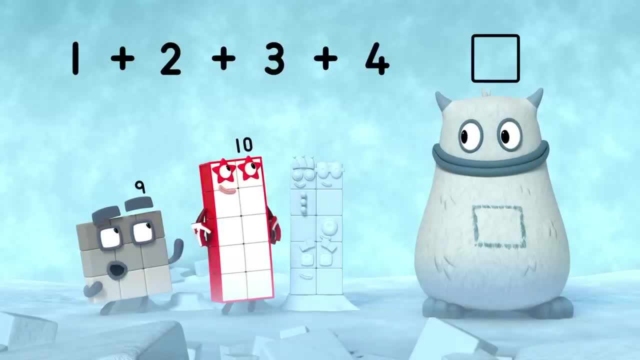 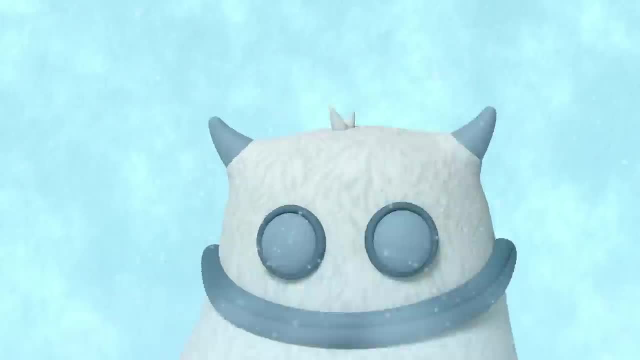 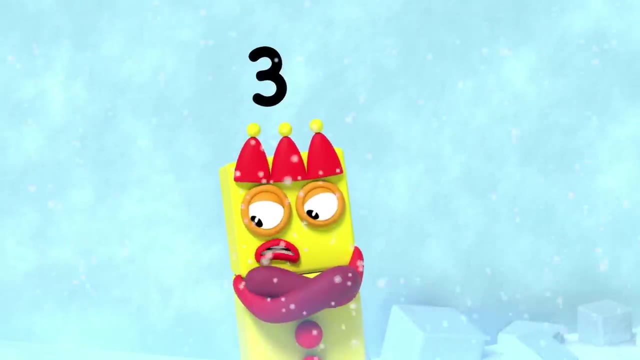 So one plus two plus three plus four equals ten. There's a ten in your tum, Yum-yum. Well done, Woo-hoo. It's nippy out Much warmer inside. Can we all come in until it stops snowing, please? 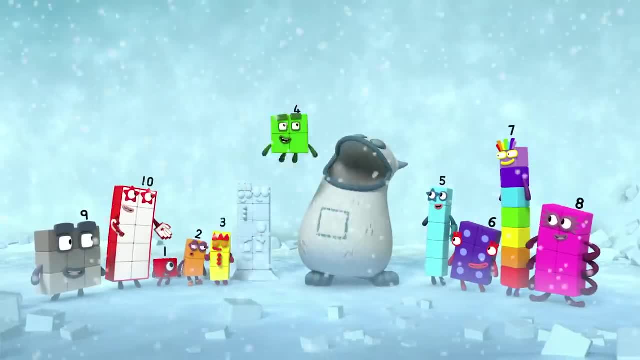 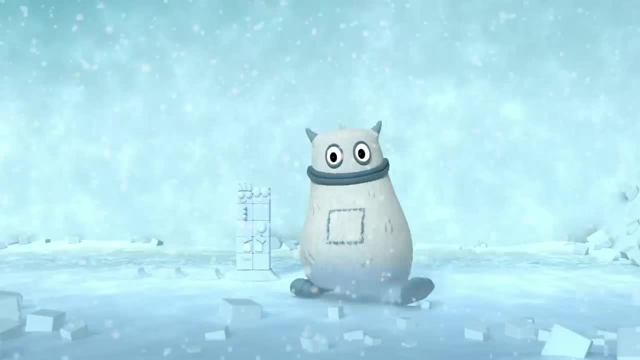 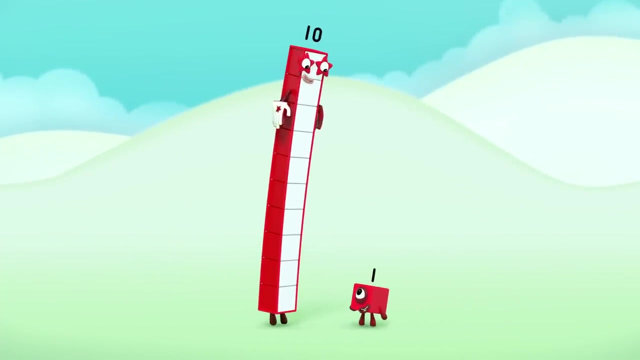 No problem, Hooray, Hooray, Hooray, And plenty of room for you too. Yum, Hello ten, Hello one. What shall we play today? Oh, Ooh, Um, Hmm, Oh. 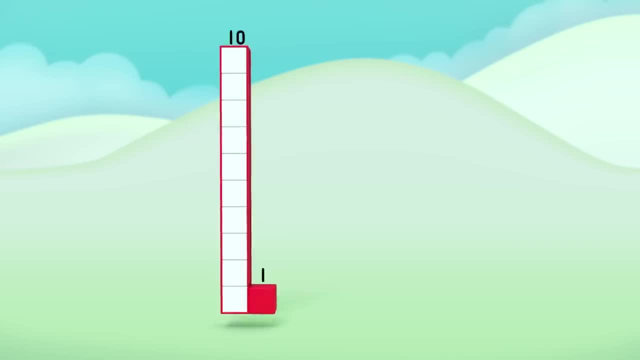 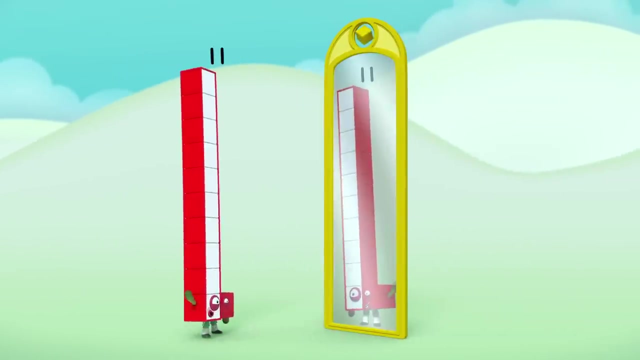 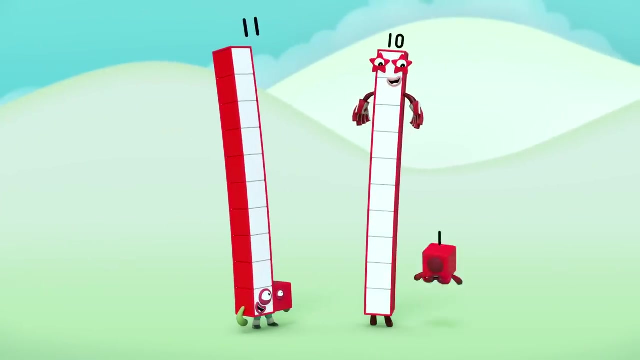 What was that? Who was that? A new number. block Ten Plus one Equals Eleven. Hello, I'm eleven, So am I, And I'm ten and one. Oh, WHISTLE BLOWS, Um Huh. 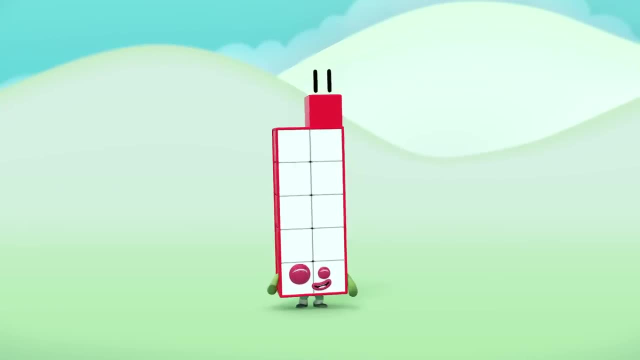 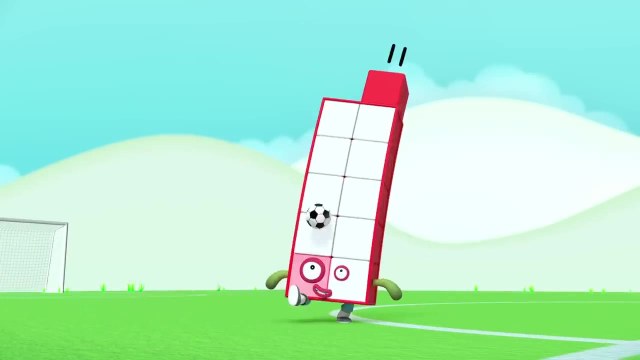 Yeah, That's better. Ooh, WHISTLE BLOWS Whoa. One, two, three, four, Five, six, seven, eight, nine and ten, And one more is eleven. I am eleven And I love football. 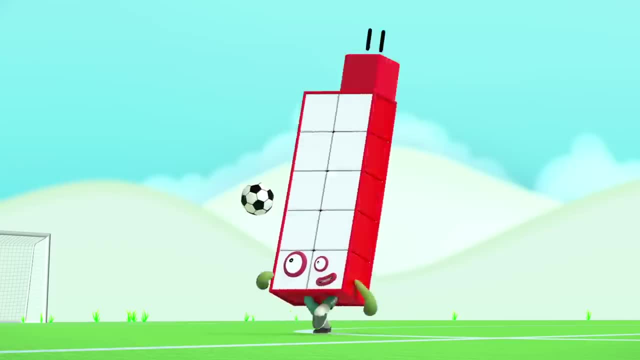 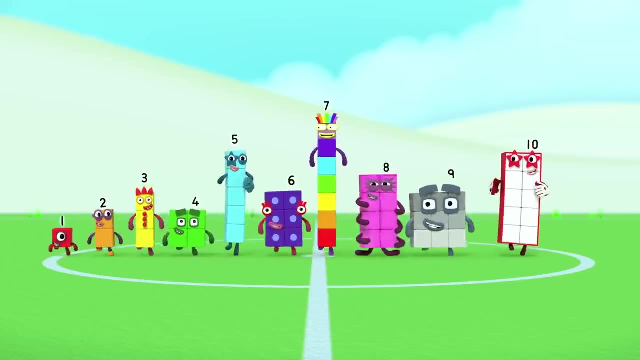 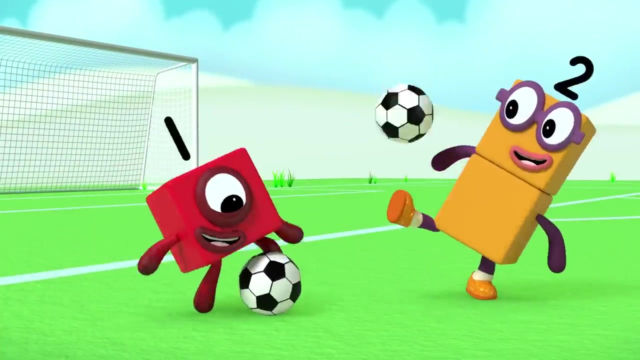 Yeah, Wow, Let's play football. Hooray Hooray. One, two, three, four, five, six, seven, eight, nine and ten. One more is eleven. WHISTLE, BLOWS. We're on our way to victory. 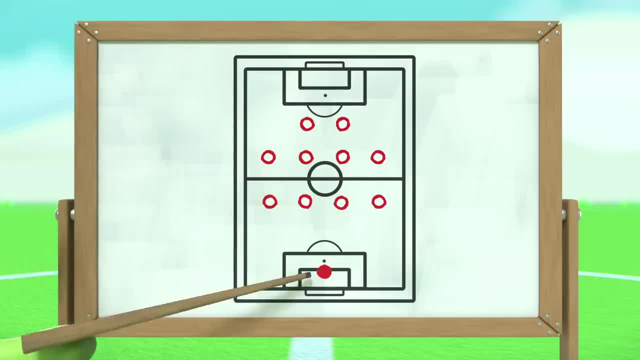 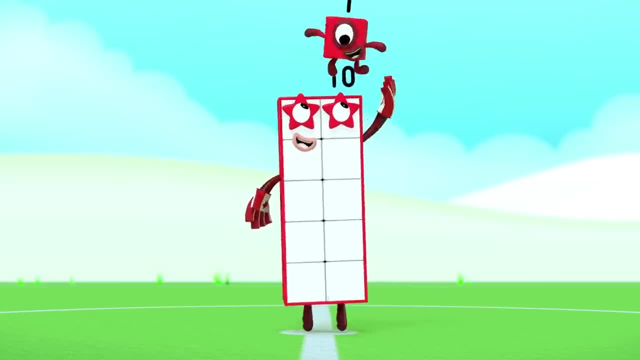 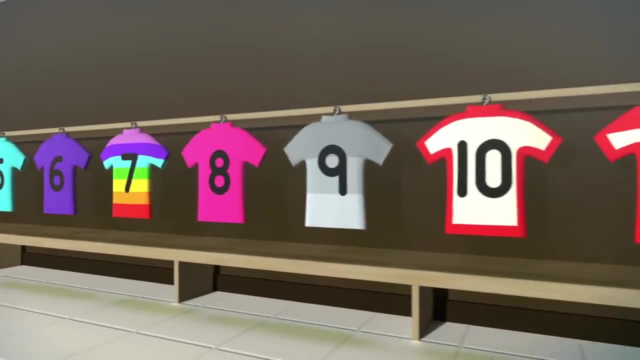 We're on our road With ten on the pitch and one in goal. We will never be denied. We'll take it in our pride With ten and one, ten and one, eleven, on our side. Football shirts, Football shirts. One for every number block. 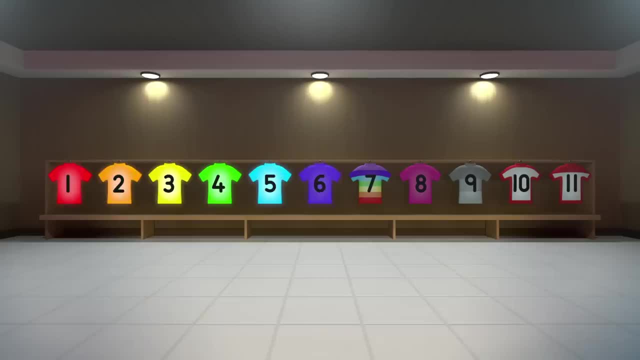 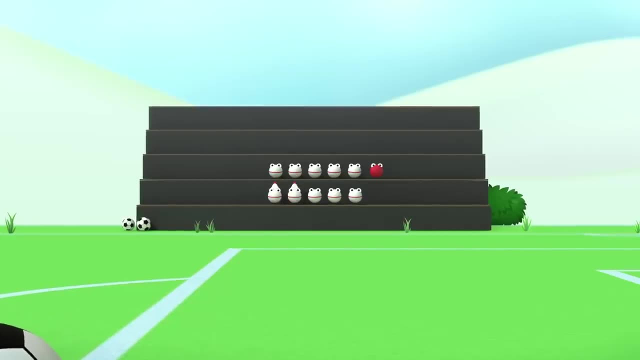 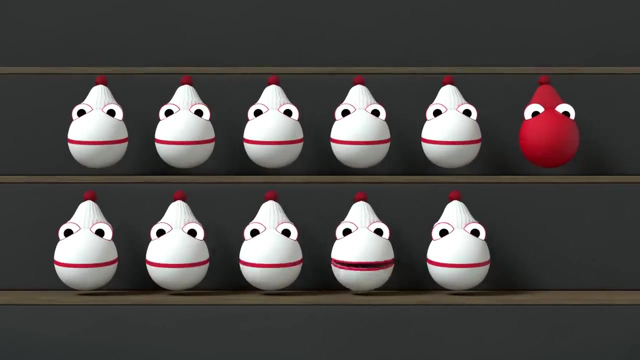 Football shirts: One, two, three, four, five, six, seven, eight, nine and ten, And one more is eleven, Hooray. Bubble hats. Bubble hats, One for every number. block Bubble hats: One, two, three, four, five, six, seven, eight, nine and ten. 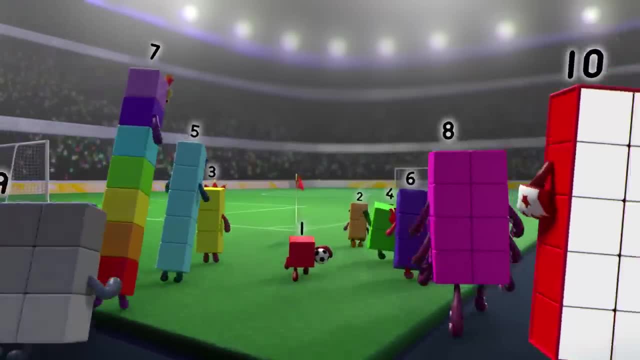 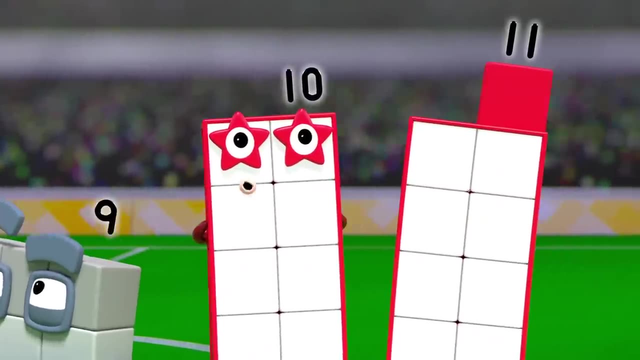 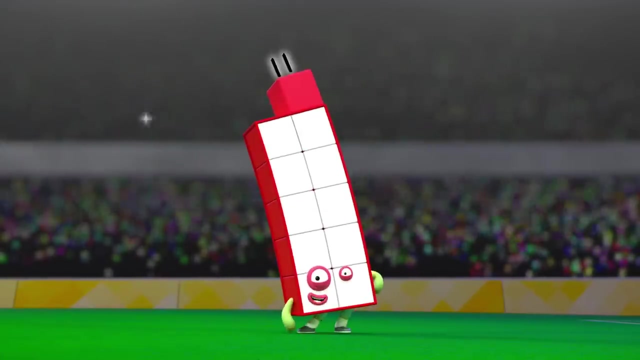 And one more is eleven. Hooray, We're on our way to victory. We're on our road With ten on the pitch and one in goal. We will never be denied. We'll take it in our pride With ten and one. ten and one, eleven on our side. 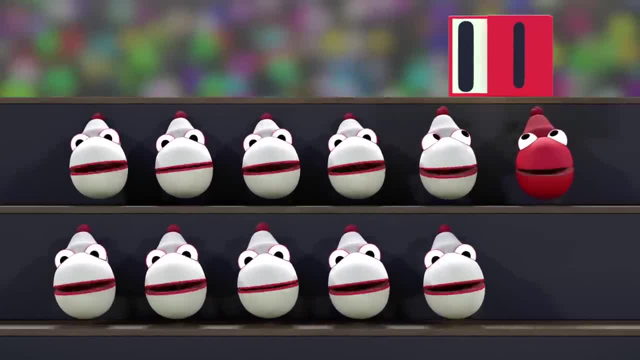 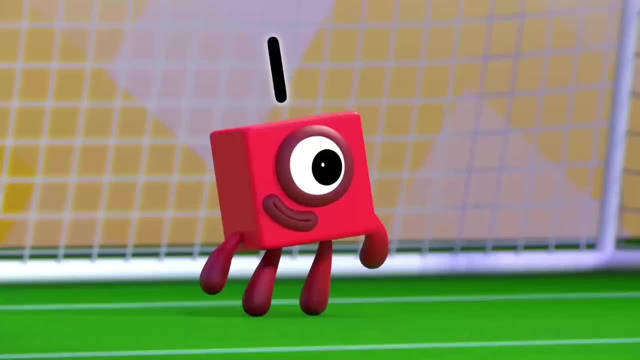 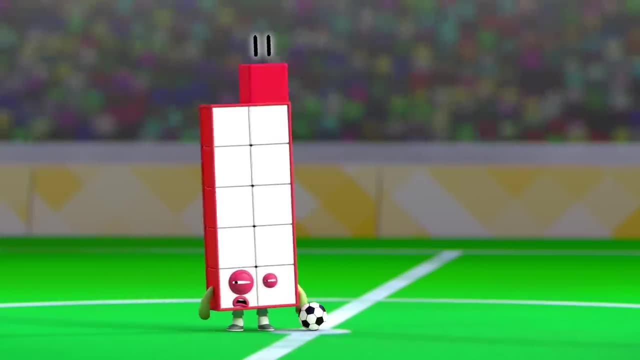 One ten, One one Ten and one Eleven. One ten, One, one Ten and one Seven. Hooray, The number blocks are out on the pitch for the big match And their captain, Eleven, looks ready to lead the team to victory. 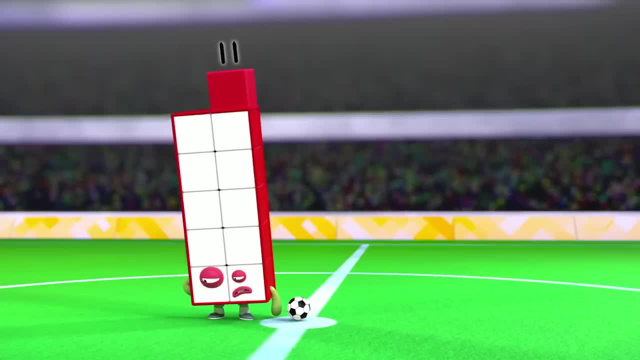 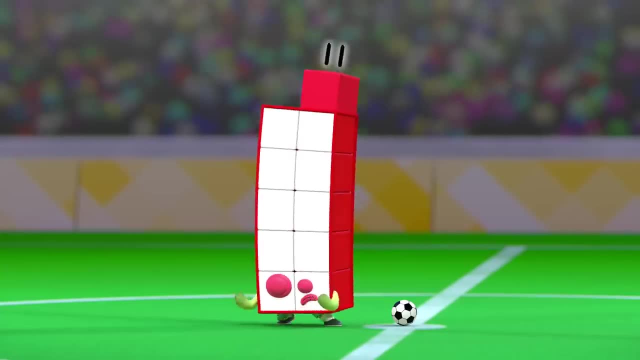 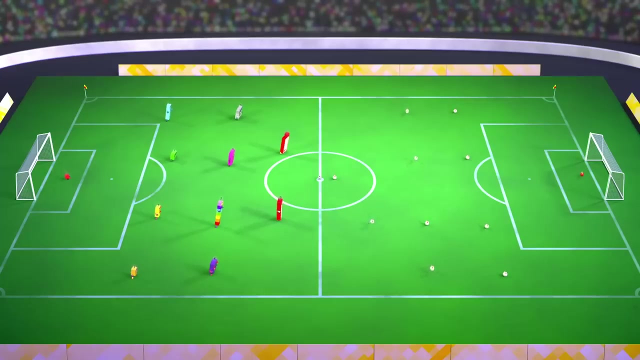 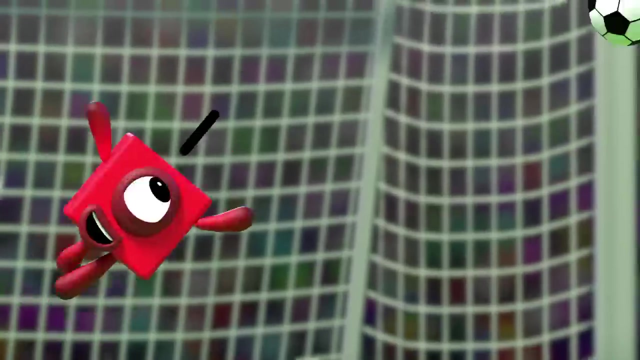 Something's wrong. What can it be? I've forgotten something. The other team. We need eleven more players. Number blocks: Hooray Game on And the number blocks have kicked off. It goes high towards the goal And saved by one. 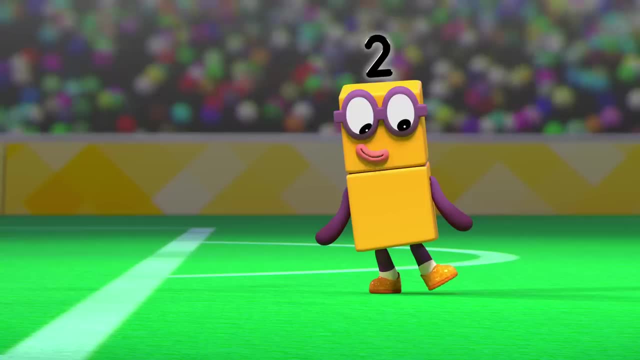 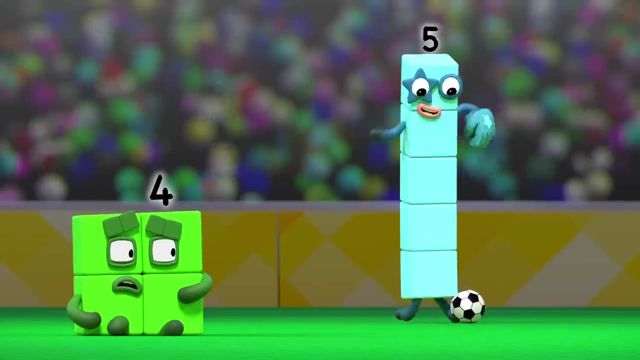 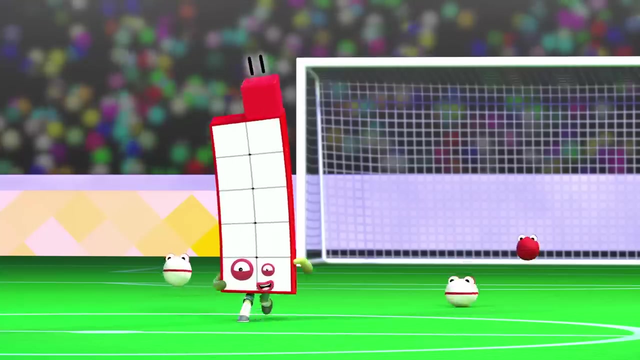 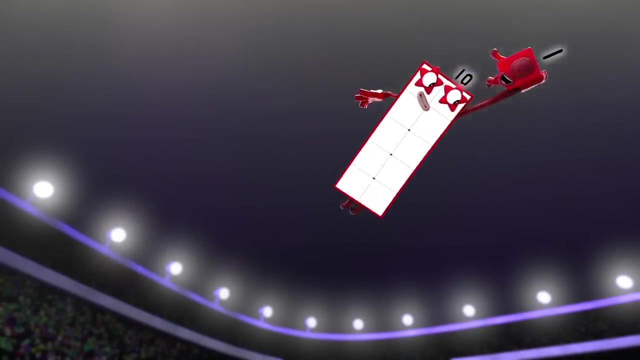 Take a bow, one, One throws it down to two. Who passes it? That's right to three, four, five, six, seven, eight, nine and ten. Now pause it to eleven. Ten passes, Eleven leaps for the header and, oh my, splits into ten and one to reach the ball. 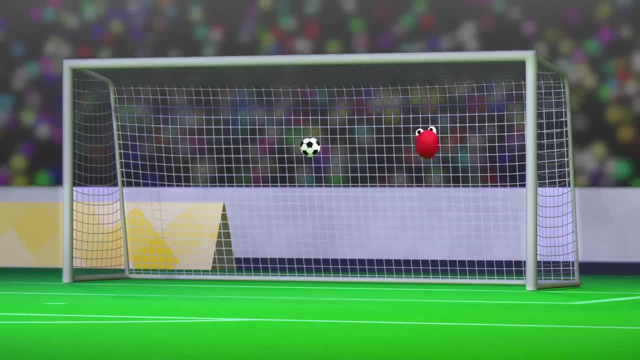 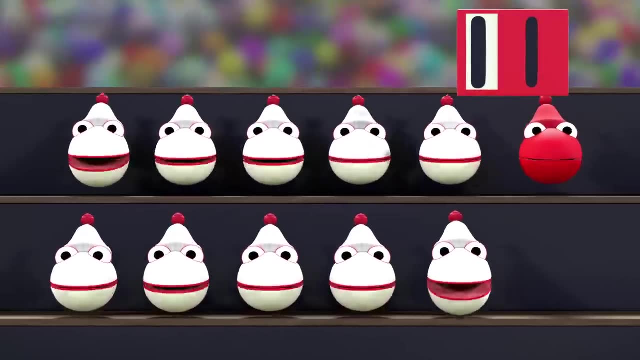 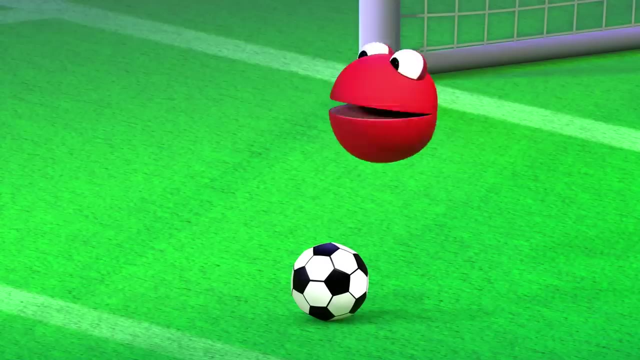 Incredible, And It's a save. What a save. Cut it up to eleven. You're louder than the rest. Ten and one. ten and one eleven is the best Number. Blob passes to Number Blob. Who finds Number Blob? 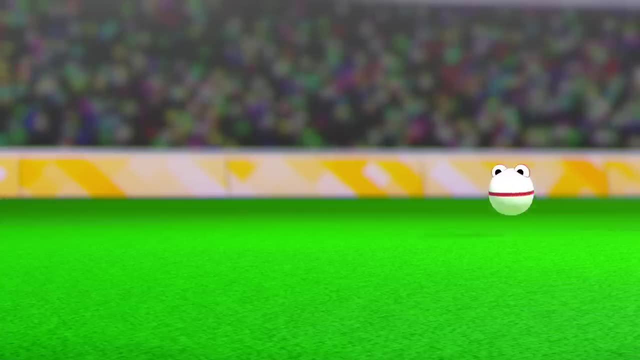 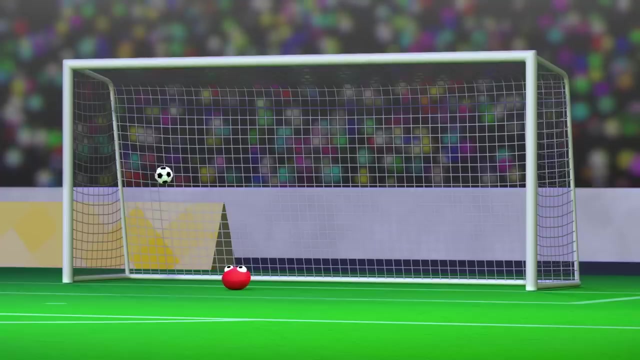 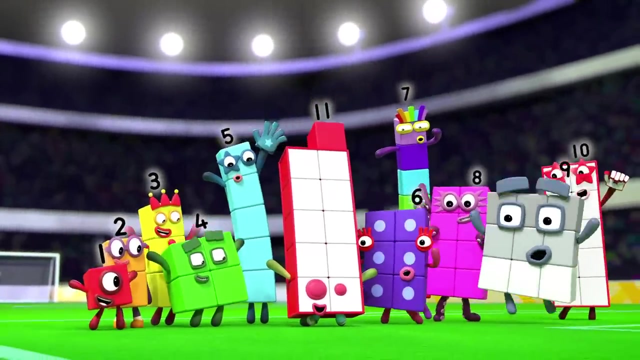 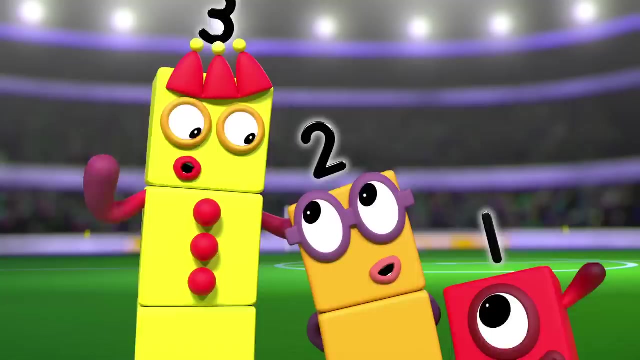 And a lovely header there to number block Eleven. Who hits it to eleven? And it's eleven, Eleven, Eleven. Oh yeah Woo, We're on our way to victory. We're on a roll With ten on the pitch and one in goal.